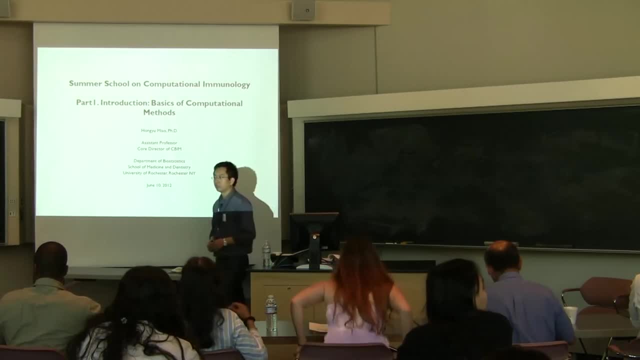 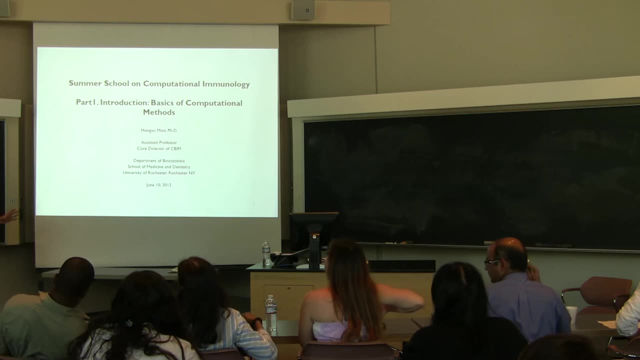 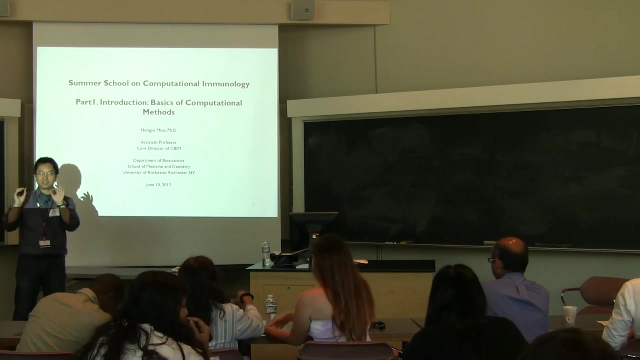 And some of you may already notice that I didn't actually talk too much after the class. Don't misunderstand that. I'm a social person. I talk a lot, I talk fast, But I need to actually keep talking six hours tomorrow, so that's why I have to save some voices today. 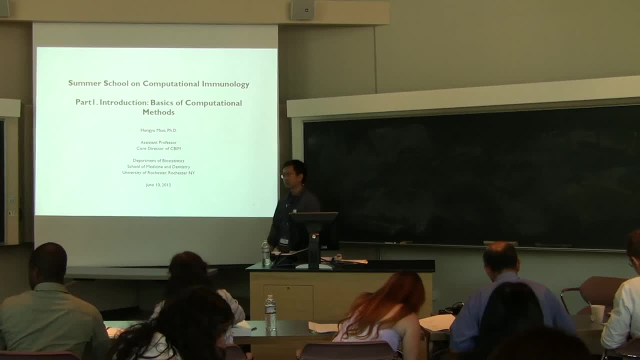 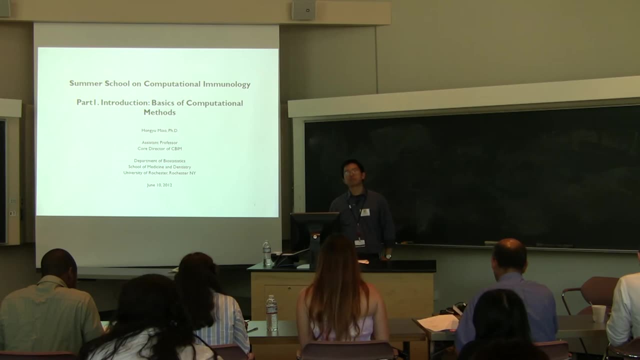 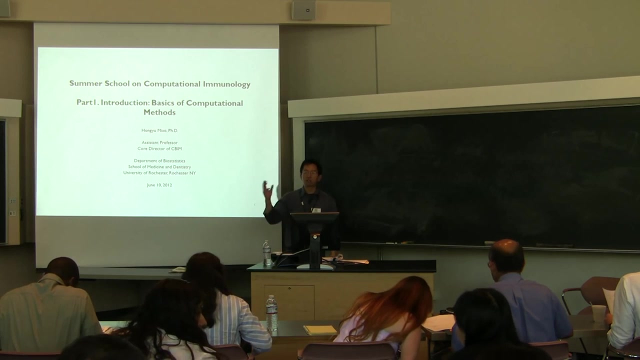 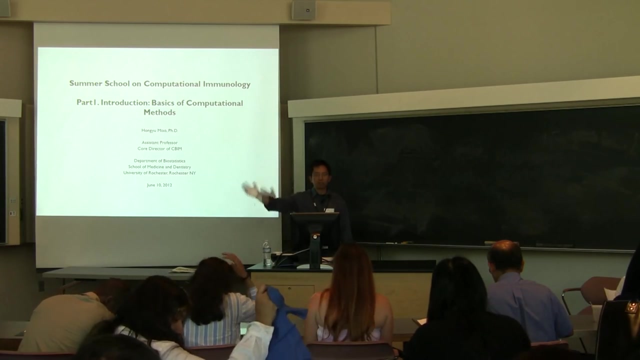 So after the introduction this morning, I actually would like to go ahead with the computing method instead of model construction, Because the whole procedure, including model construction, sensitivity analysis, benefit analysis and model selection, that will be a whole procedure which will be covered tomorrow. 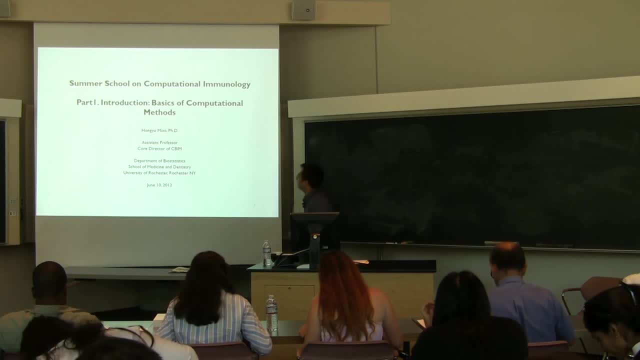 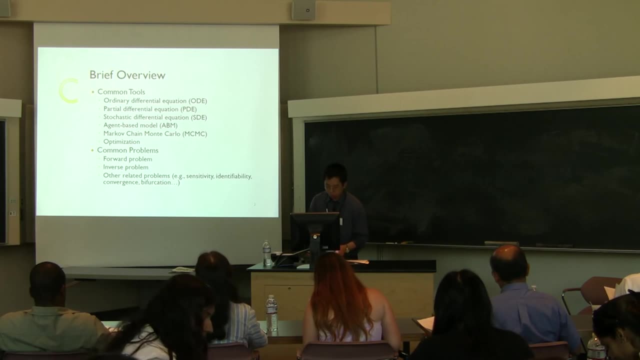 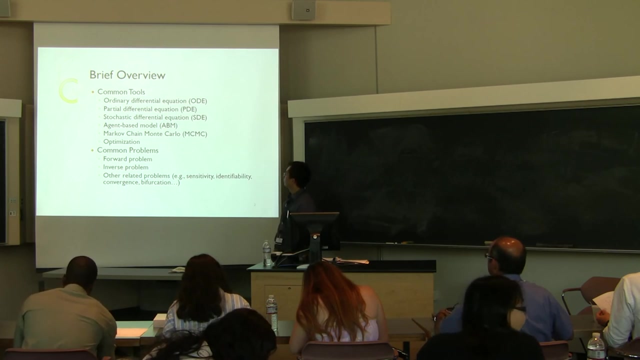 So now let's switch, Switch the gear. okay, a little bit Computing method. So we have talked about some commonly used tools in mathematic modeling. okay, including the ODE model, PDE model, SDE, aging-based model, and Monocarlo Markov chain, Monocarlo and optimization. 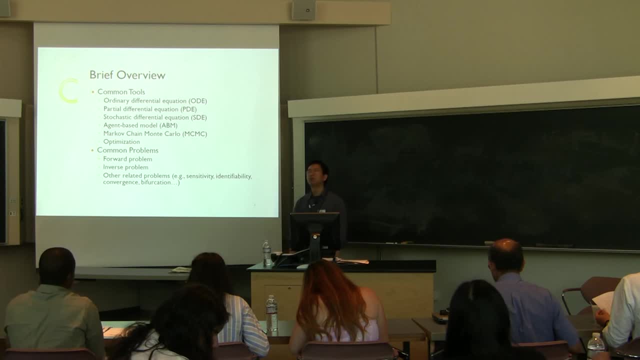 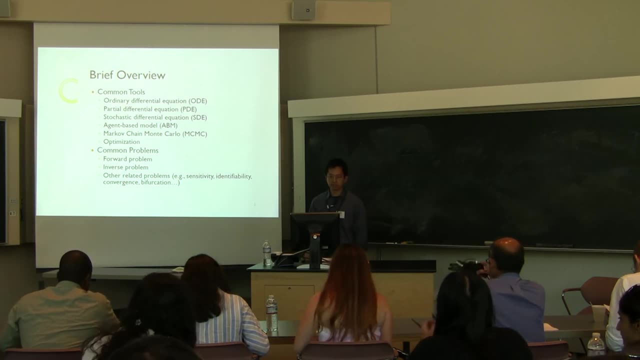 We already sort of know what's ODE- okay, And the PDE we already know PDE can actually take the spatial difference into consideration. That's one advantage of PDE, SDE- we know that it includes randomness or stochasticity into the model. 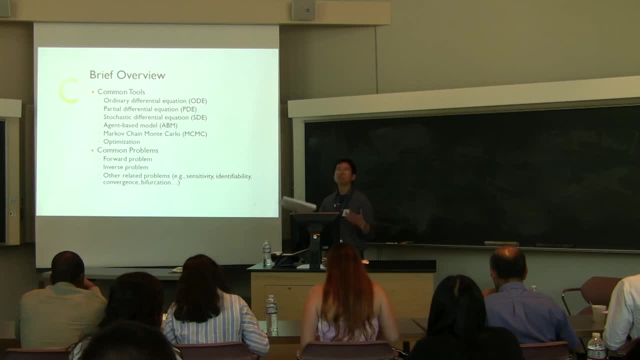 Aging-based model is more like a stochastic simulation tool, which Catherine from Canada will actually spend the whole day with you, with Tom Kepler actually talk about the aging-based model, So I will not talk about that Either today or tomorrow. Markov chain is more like a conditional probability model. 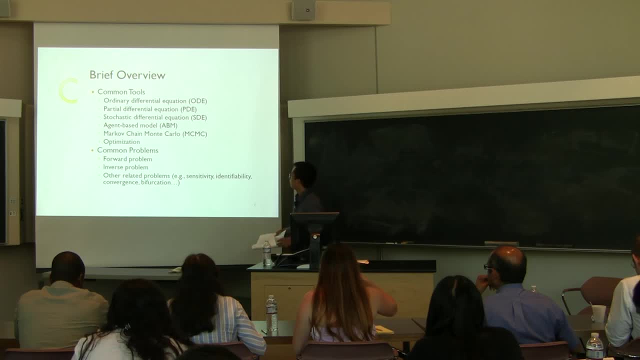 For now, probably we don't care about what it is And, by the way, we will actually talk about optimization, which is actually of extreme importance. okay, to modeling. I'm going to explain why. And now we definitely cannot actually cover all these different, you know, tools and how to. 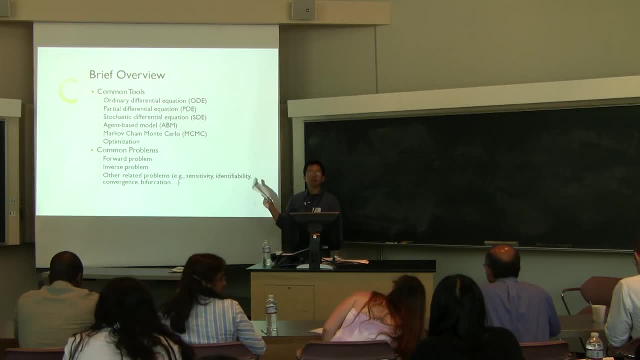 how can you deal with them? What we can do actually is: I selected ODE, PDE and some stochastic simulation algorithm plus the optimization algorithm. okay, For the rest, topics are very interesting. Wednesday: that's about aging-based modeling. 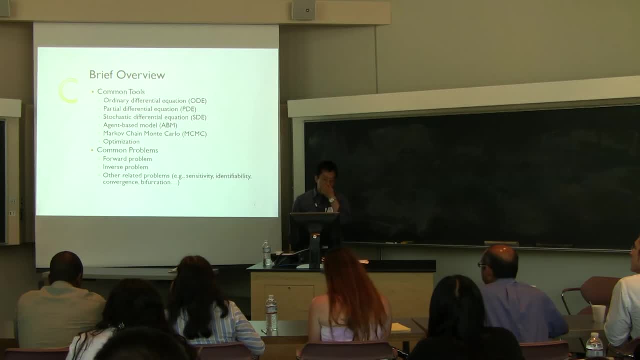 And unfortunately we don't have anybody to cover the MCMC. okay, Although it's a very important tool In general. okay, when we use this, mathematical models okay, or modeling tools, there are two categories of problems we want to solve. 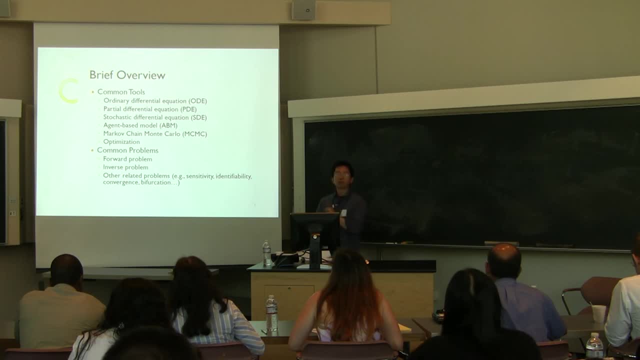 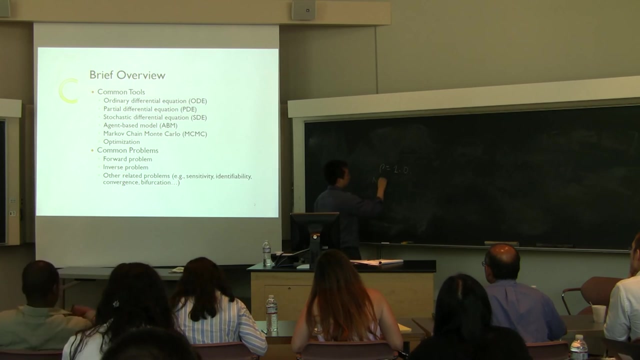 One is called the forward problem, The other one is called the inverse problem. So actually this morning we already talked about the forward problem. We mentioned that if we give a parameter value and if we also give initial condition, for example 100.. 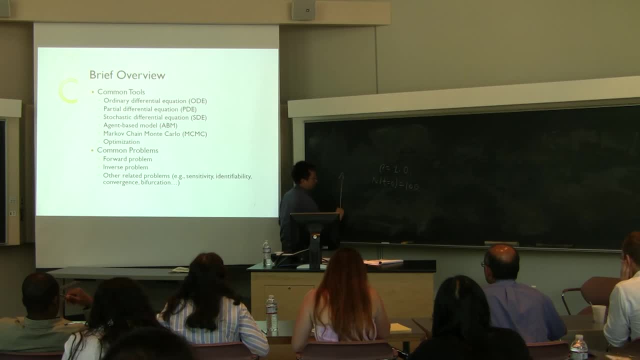 Okay, Then we solve the ODE to get the complete trajectory. of course Depends on what model you're considering. If it's an exponential growth model, you want to actually know every detail about this curve, okay, So that's called the forward problem, okay. 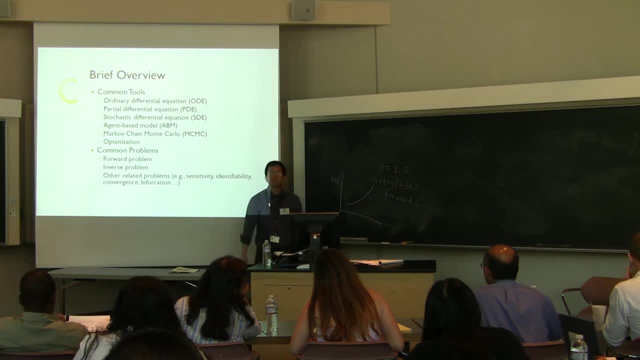 Okay, Which means giving parameter values, giving initial conditions. then I predict what happened afterward. okay, So it's called forward forward in time, okay. So, however, inverse problem is not mean, does not mean that I want to solve this problem. 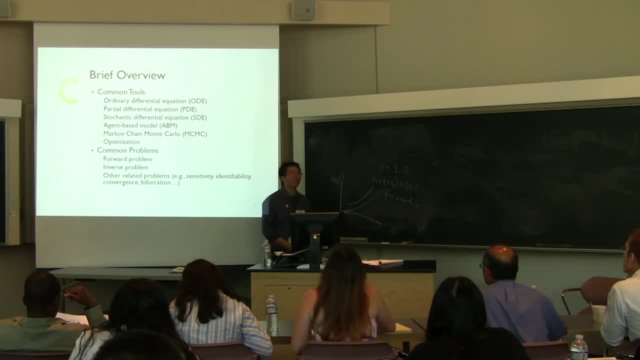 backward in time. okay, That's not a meaning of the inverse problem. Inverse problem is that I don't know the parameter value. okay, However, now I have data With noise- right, I have data. Now I want to infer the value of this parameter from data. 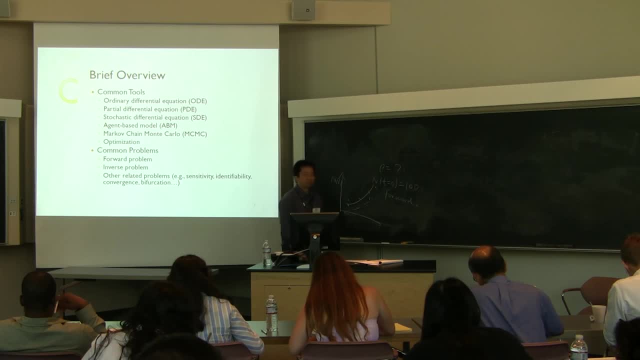 Okay, that's called the inverse problem. Okay, So clear. Now there are many other related problems, okay, For example, the sensitivity, identifiability, convergence, bifurcation analysis. Unfortunately, we don't have time to talk about all of them. 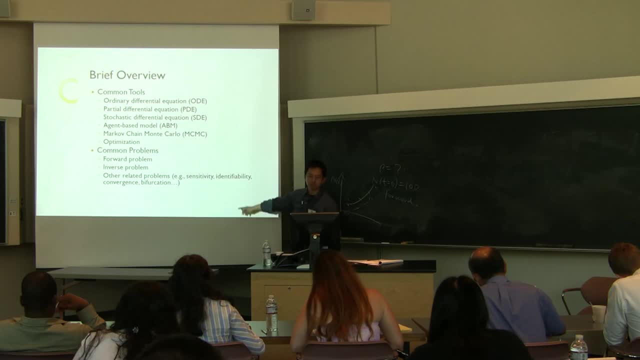 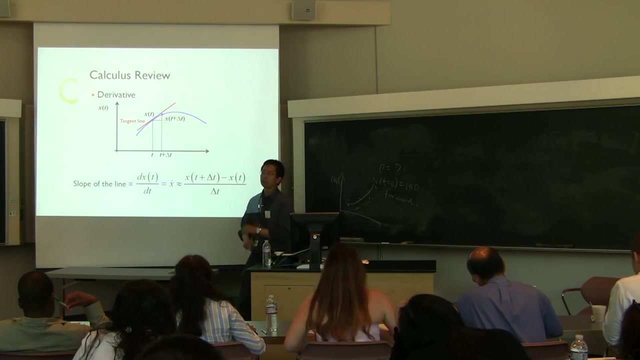 but we will cover the most important and basic one, okay, Sensitivity and identifiability. So that actually is directly related to your model structure. So now let's actually spend like five minutes to finish the first grade undergrad course of calculus, okay. 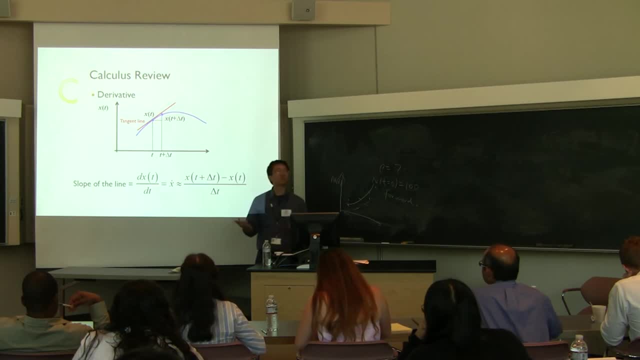 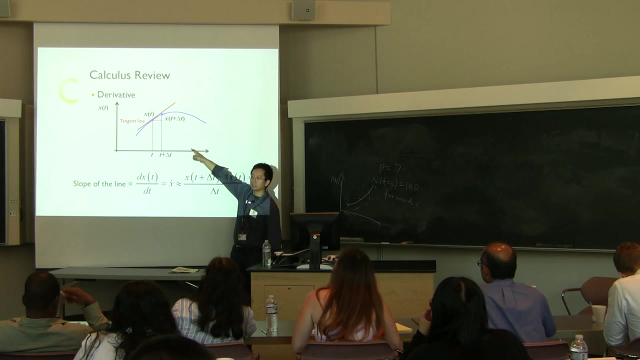 Just two slides. One slide is derivative. okay, We talked about it this morning. right, We say that the derivative is actually the change per unit time, or equivalently, that's the rate, or equivalently, that's the slope of the tangent line. okay. 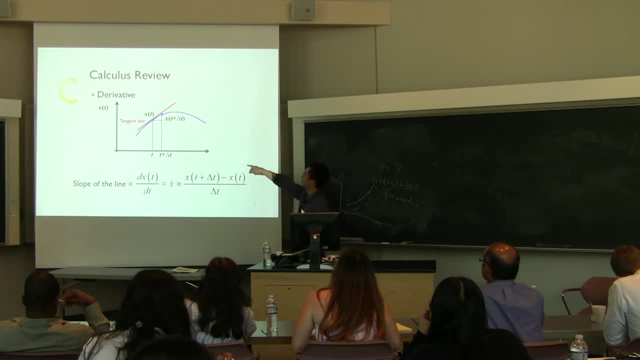 So there are the same thing, if you just look at this plot- okay, Giving a time interval. you look at the- let me see if I can use it. Okay, you look at this distance. This is a change, okay. 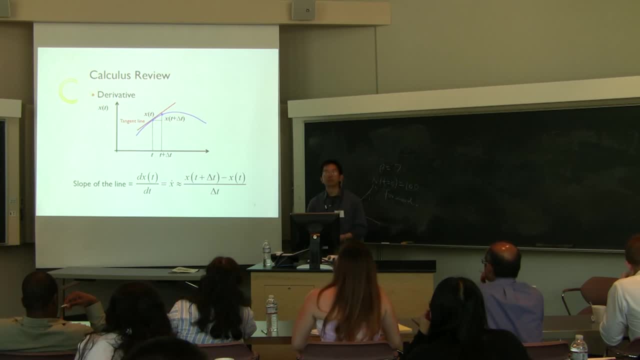 This change divided by the time interval. that's where you get the derivative, Okay, Okay, So your lecture will need like 10 courses to explain this idea, but we finished it in like a half minute and I'm gonna spend another half minute. 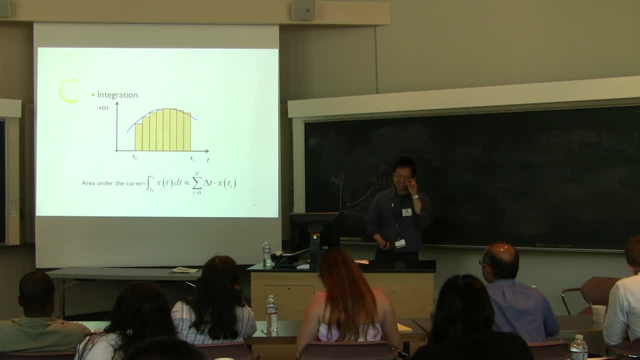 to explain the idea of integration. okay, Integration comes from the problem that we want to calculate the area under the curve. okay, So this is my curve, the blue curve is my curve, okay, And if this is a straight line, okay. 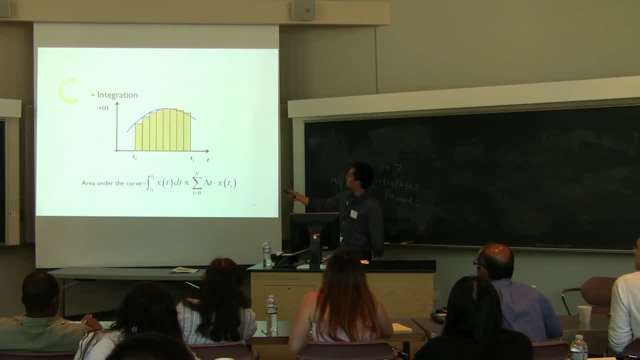 the area under the curve is easy to calculate. right And now, if it's an arbitrary shape, okay, how we do the calculation? calculate the area under the curve. So the idea actually is also simple, Since I cannot directly calculate the area under the curve. 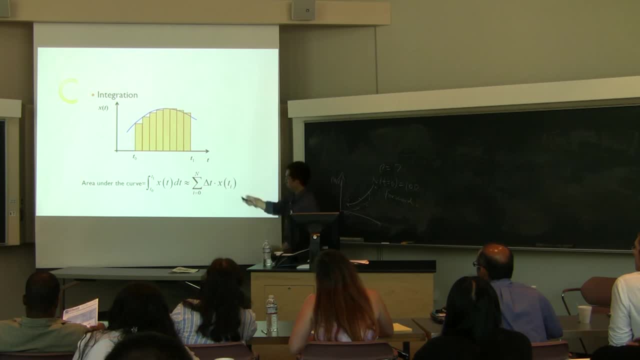 let's divide that into small pieces, okay, And within each interval. okay. I use a rectangular bar to approximate the area under the curve within this interval, okay. So of course there's a approximation error right here. We actually didn't cover that part, that area, okay. 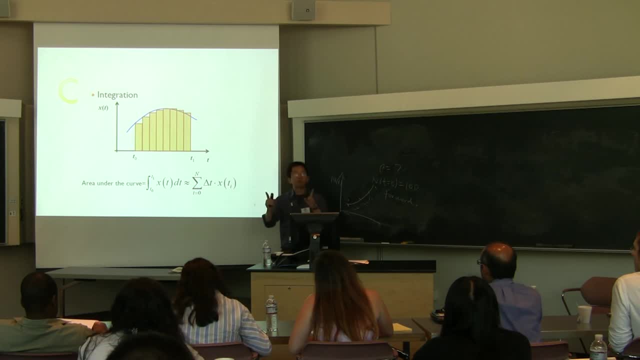 But it's okay, Why, If we keep dividing this into smaller and smaller interval, the approximation will be better and better, right? So eventually, okay, I can calculate, okay, the area under the curve using the summation of the area. 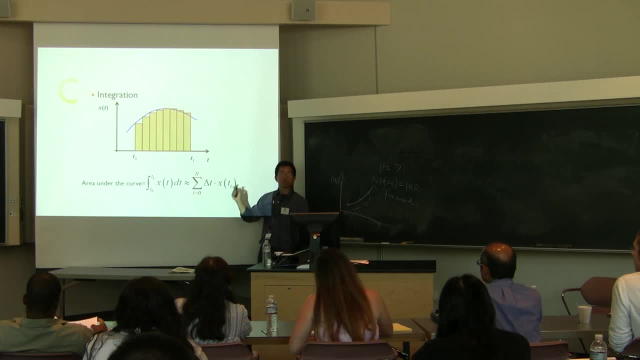 of all the bars, right, And once we have enough bars, or divide the whole interval into much, much smaller intervals, okay, the approximation actually will be very accurate, okay, So you don't need to worry about, of course. 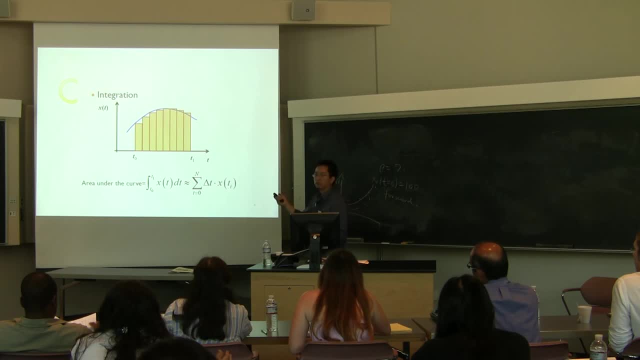 all the numerical algorithms, they have errors. okay, If the error is very small, then we don't need to actually worry about it. So that will be the idea of integration. So the notation will be- I don't know how to call it. 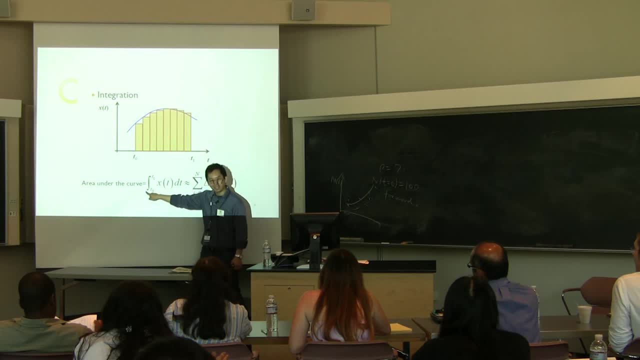 okay, doesn't matter. So you have an integration operator. This means the integration operator, And this is the starting point, this is the end point, okay, which means from here to here, okay, And this x is your full curve. 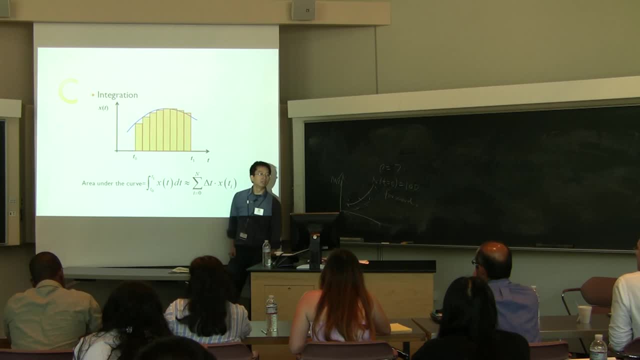 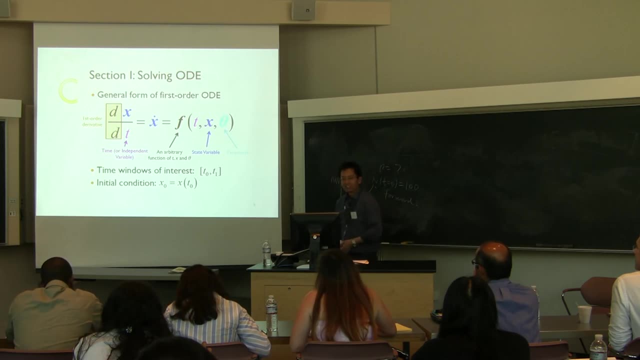 And this just give you the area under the curve. okay, Half minutes, finish the calculus course. okay, So now in the first section, I want to talk about how to solve ODE models. okay, That's the what we just talked about. 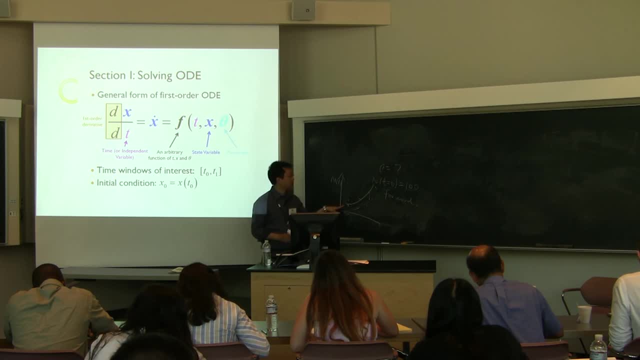 Give the parameter value, give the initial condition, how actually numerically solve to get the whole trajectory? okay, Again, here is the terminology we should get familiar with And we're gonna use this kind of terminology tomorrow. okay, So we again we know that D is the derivative. okay, 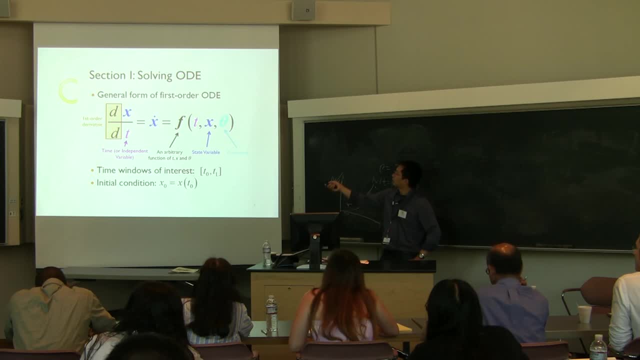 means that differentiation, okay, operation X is a dependent variable or state variable, T is an independent variable or tan, simply quite. And we can write it this way: These two are equivalent. okay, And T again x, theta. here I use theta. 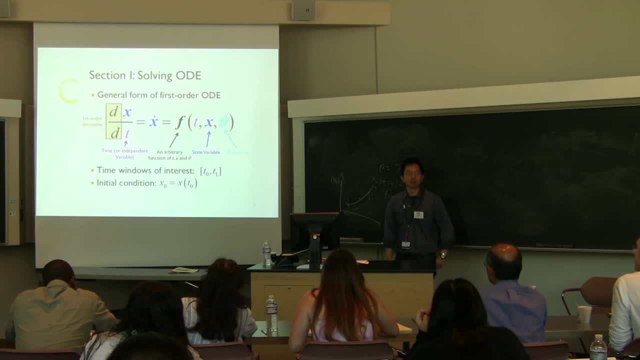 to denote the parameter, all the parameters. So one model can have more than one parameters. okay. One model can have 10 parameters. If you're talking about a network model, you probably have thousands of parameters. okay, So this theta doesn't mean it's a one-dimensional, okay. 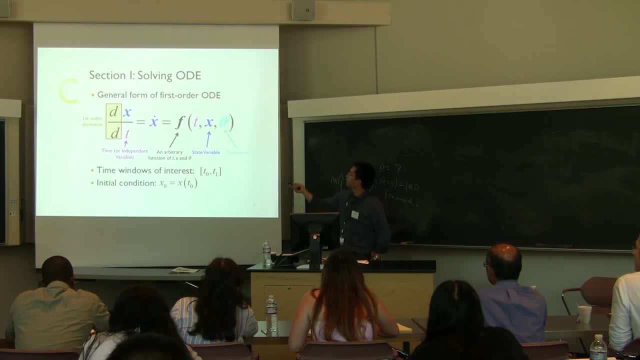 It can be one-thousand dimensional, okay. F here is actually an arbitrary function of T, x and theta. So that would be the general structure of ODE model. So now, if we need to solve ODE, we also need to specify two other things, okay. 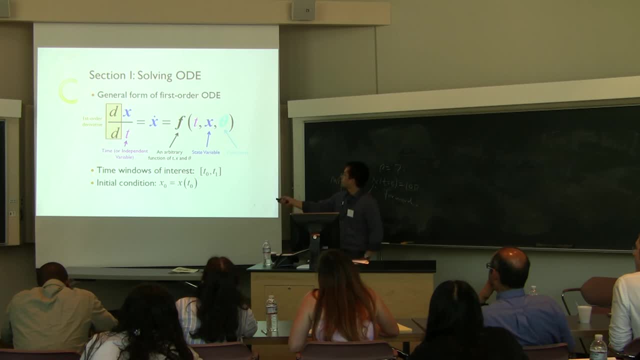 The first one is the time window of interest. So from T zero to T one. So why can't we go to infinity Instead of from T zero to T one? we can go from T zero to infinity, right, But usually we don't bother to do that, okay. 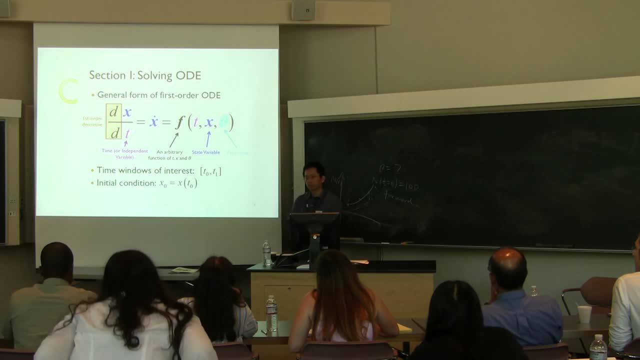 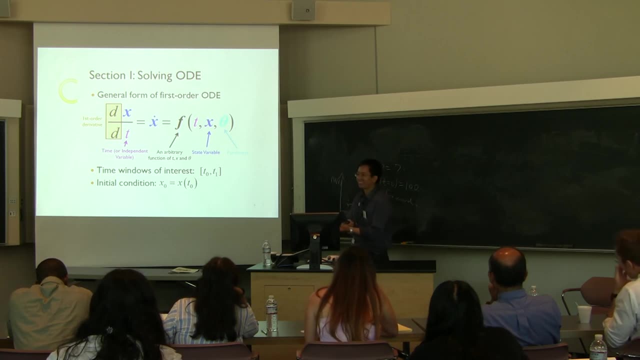 First, in experiments you cannot actually observe things okay after infinite time. okay, So it's too long. Nobody gonna find you okay to do that. Secondly, even if we want to understand the system behavior at infinite time, 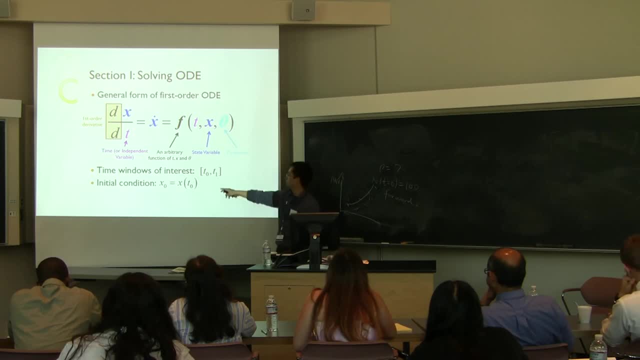 we have other method, okay, which okay. we have other method, okay, which okay. we have other method, okay, which okay. we also will talk about which is called. that you already call the steady state, okay. 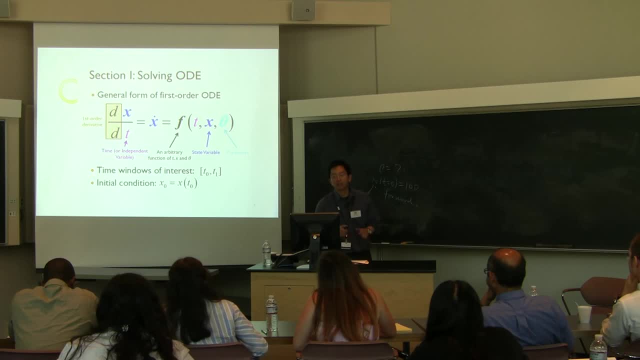 So there's alternative methods to deal with that, So you don't have to worry about it for now. Initial condition: of course we need to know We are starting with 1,000 cells or 10,000 cells- okay, in my culture. okay. 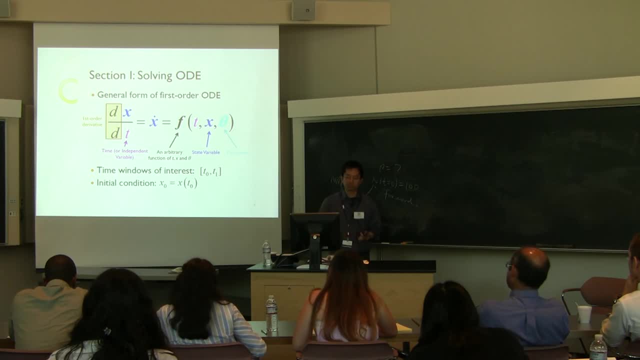 So that will give you a different- you know curves, trajectories, okay. So of course, like I mentioned before, theta has to be specified. okay, If you don't know theta, you cannot solve the ODE, okay. 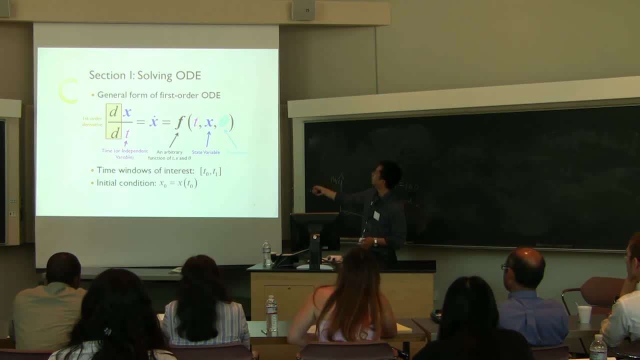 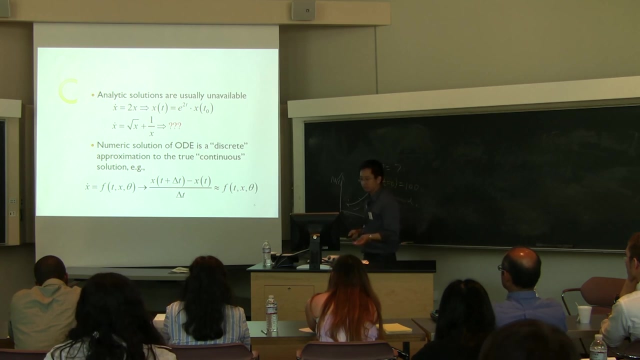 So actually you need to specify three things: Theta, T0,, T1, and the initial condition. Then you can solve ODE. okay, This is a forward problem. Now let's look at the, the necessity of a numeric solution to ODEs. 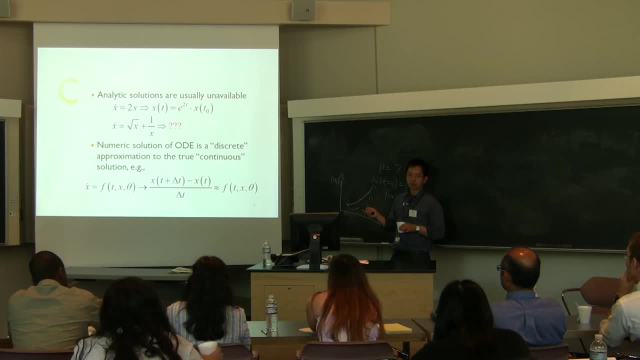 So, if we consider this very simple exponential growth through a growth model- okay, we talk about this morning, right, I just replace the row, or replace the row with a two okay, of a specific number. Then we have an analytic solution like this: 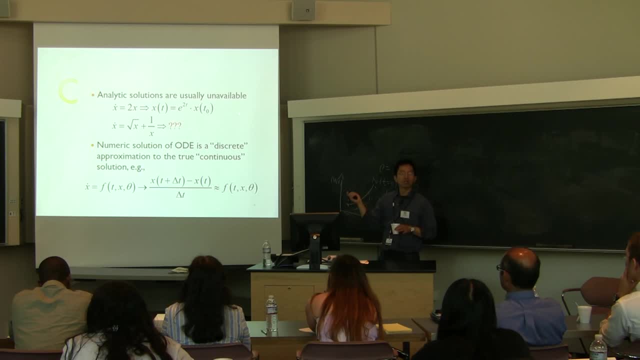 which actually looks simple. okay, This one is simple. However, if I just somehow manipulate this equation a little bit, put a square root of x and add a one over x here. So what's the solution? Can you get a closed form solution or any way? 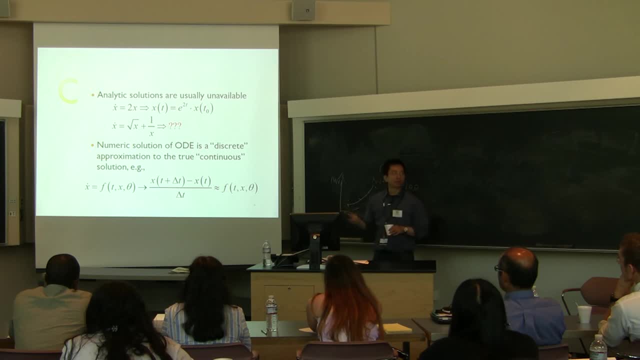 Okay, well, actually you can. I tried this one using Mathematica. You know Mathematica can do, you know the package Mathematica can actually do this symbol, symbolical computing. okay, And the results: actually is three lines long. 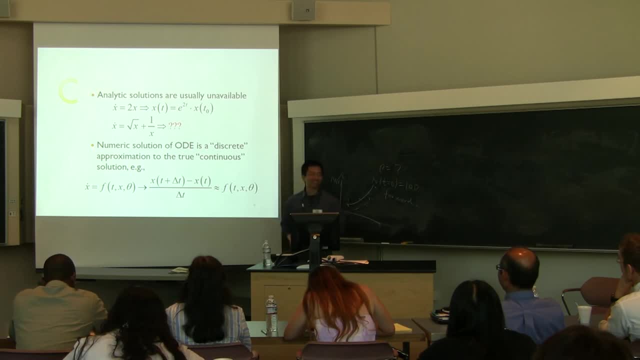 You don't want the father to use that long solution, okay, They give you lots of struggling, okay. So that's why people actually use a numeric solution, okay. So for this simple solution, okay, you could use, you know. 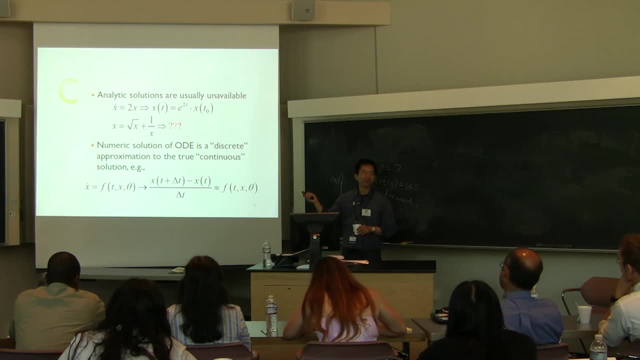 three lines long, okay, So that's what people actually need. This is actually also a simple, you know ODE model, So, but even for this one, okay, you probably will consider numeric solution, okay. However, numeric solution is a discrete approximation. 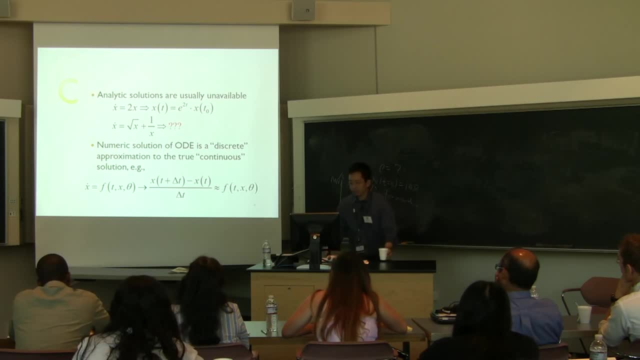 okay to the continuous solution. Remember, if I have a we talked about this morning, okay, NT okay is continuous. okay, So when we solve it, okay, we cannot actually calculate every point, every single point on that trajectory. 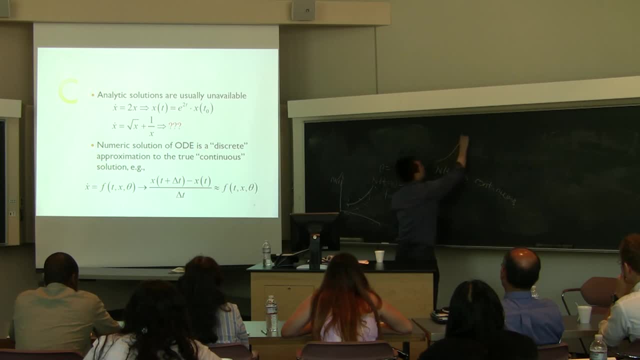 What's the reason? So, if I have a curve like this, how many points are there on this curve? Infinite number? right, because they are continuous. You can divide, divide, divide this into smaller, smaller, smaller interval and you still get one point. okay. 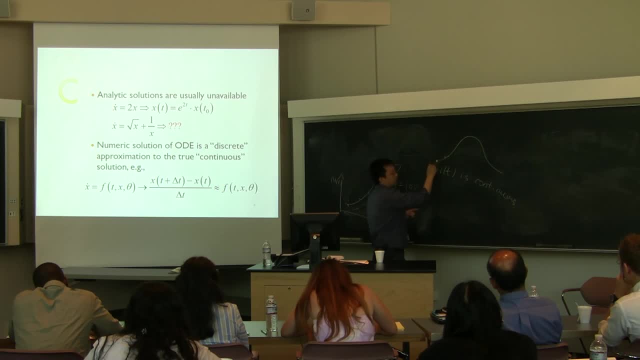 That's why when we solve the ODE, okay, we can't do that, Okay, we only solve at a certain distance. For example, if I start from here, I can jump a little bit. then I get a predictor value here. 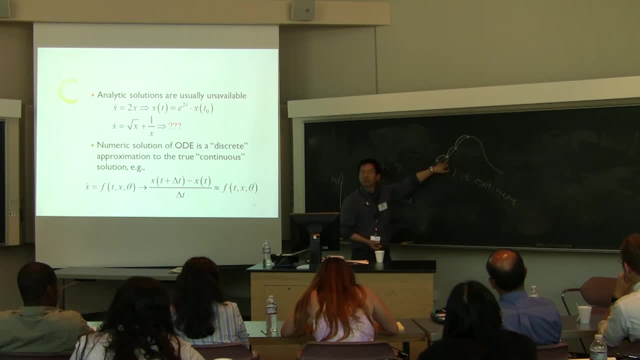 and then I jump to here, then jump to here. okay, So that's what I mean by discrete approximation. okay, So you will not get actually every point. okay, It's not possible. However, if you are really interested in this point, 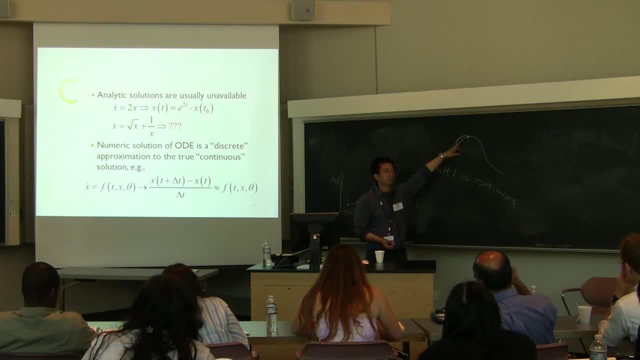 which is not covered by any of the points in a solution. there is a way, okay, to calculate the spike. Okay, the algorithm actually will handle that, So you don't have to worry about, you know, this problem, this sort of problem. 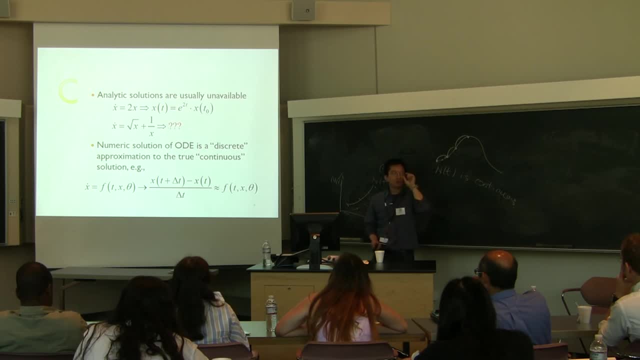 Now let's actually look at how to actually solve, numerically solve, the ODE. okay. So let's start from the equation. okay, This is our general ODE equation and remember, when we derive the derivative, we actually start from this approximation. okay, 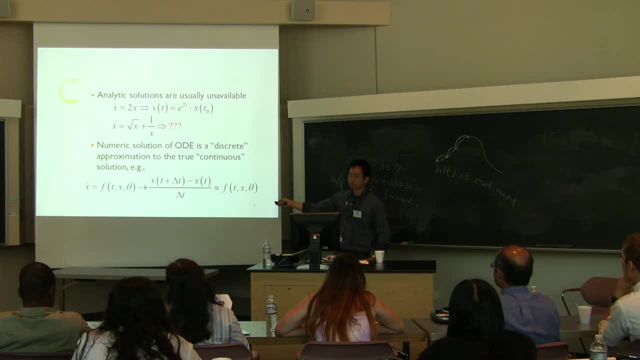 We start from the difference divided by the interval. right Now, when we solve it, we actually go back to this approximation. okay. So instead of the exact derivative at one point, okay, we go back to this approximation. Now, if I plug in this approximation into the left-hand side, 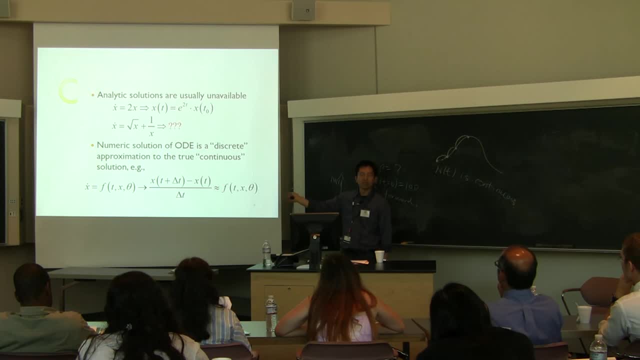 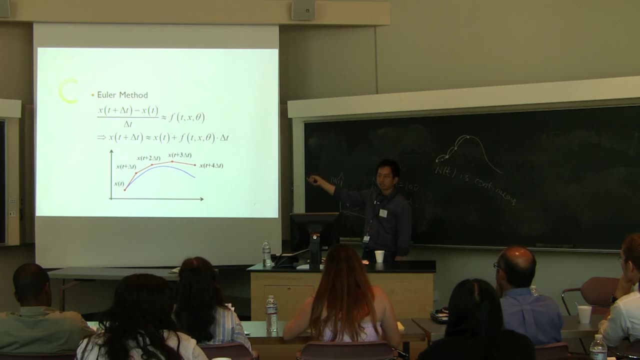 you will get this equation right, Okay, so next step: we just multiply delta T on both sides and move actually back to the right-hand side. So we're doing what are we doing This morning? we're actually doing, you know. 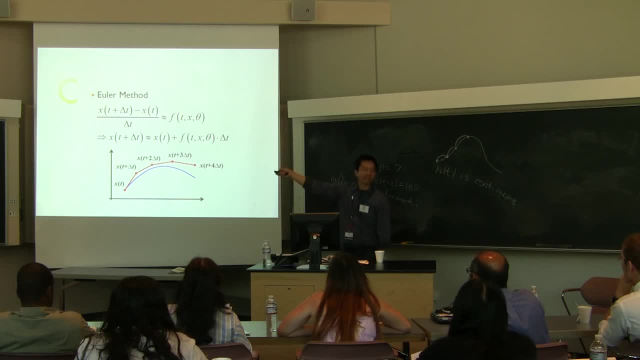 the opposite direction, right, We start from here and then go back to this equation, and then go back to, and eventually we get at this equation right. So when we solve it, we actually, you know, follow an opposite direction okay. 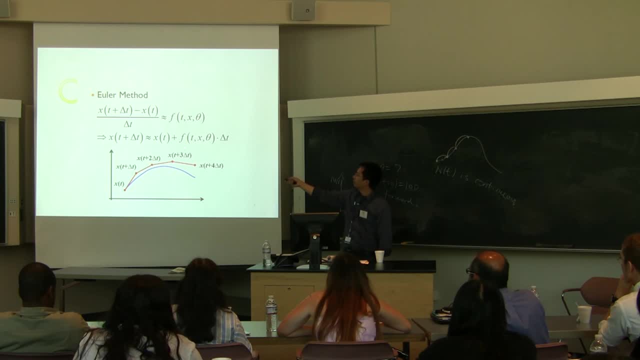 So once we get to here, then one good thing you can tell is that if I know the value of x at time, t okay, and also if I know the time interval I'm looking at, then I can actually predict the value, approximate the value at t plus delta t okay. 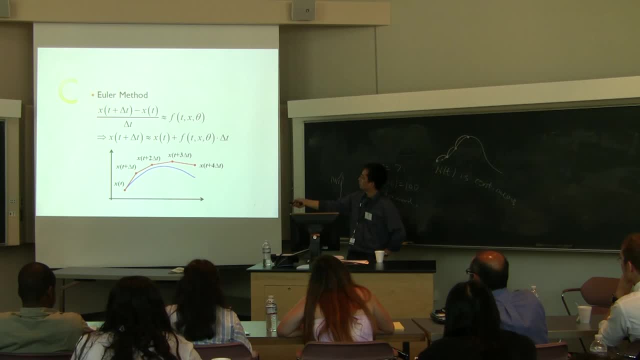 So that's the idea. So once I know this one, I can predict the value here. Once I know this number, then I can use this formula again and predict the value after two delta t and after another delta t. okay, 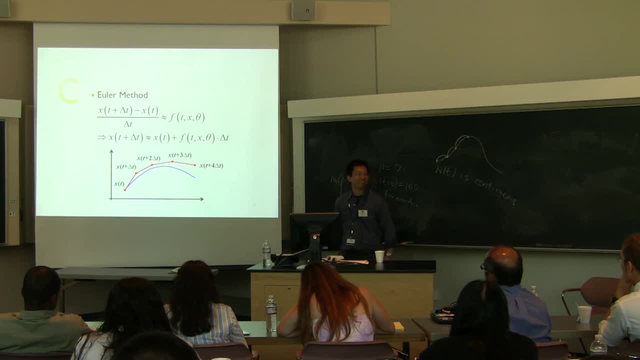 So that's our famous Euler method. okay, So every numerical algorithm book will talk about this Euler method. okay, But the basic idea is actually extremely simple. You start from one point and predict the next value- okay, And then predict the next one. 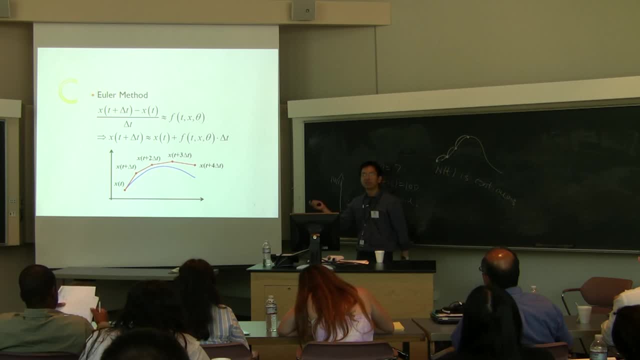 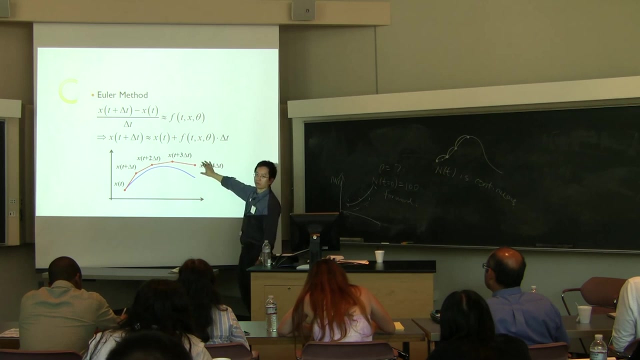 So what's the immediate problem? you can see from this slide. So blue curve is my true trajectory. However, my Euler method is shooting away right from the true trajectory, So that's something called the numerical error. okay. 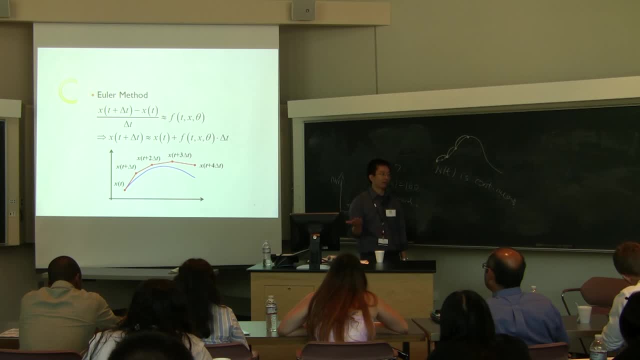 Remember, when you use a numerical algorithm, okay, you always get you know a numerical error. But again, if a numerical error is small, then you don't need to worry about it And algorithm actually has many strategies to control that numerical error. okay, 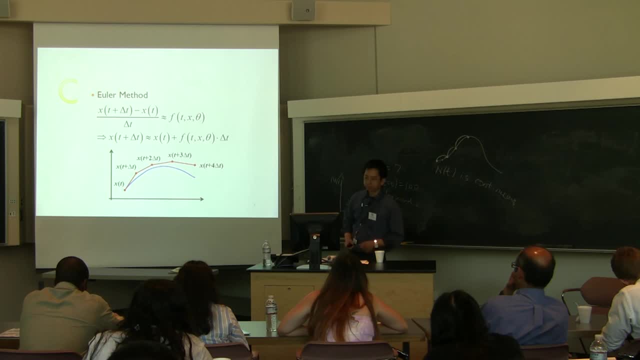 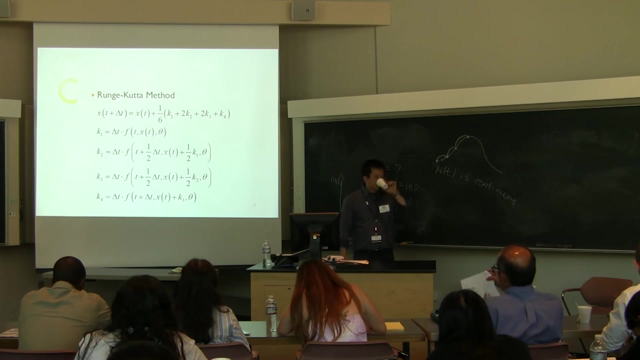 So, anyway, I have to say Euler method is not a very accurate algorithm, okay, as you can tell from the plot. That's why people also derive the so-called Rangokuta method. So Rangokuta method- okay as I, this is actually a much more accurate, okay, algorithm. 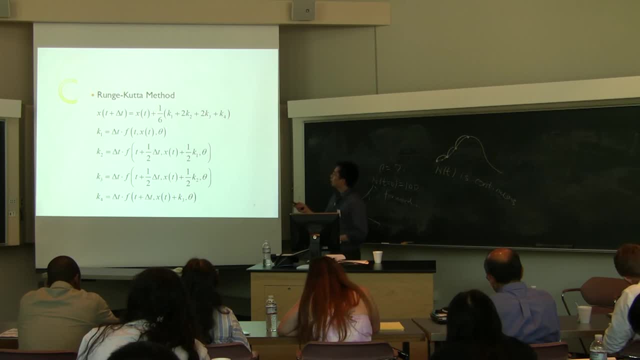 than the Euler method. So if you look at this equation, okay, now again we're trying to predict the approximate error. Okay, the value of X at T plus delta T from the value of XT. okay, But what changes is here? okay, 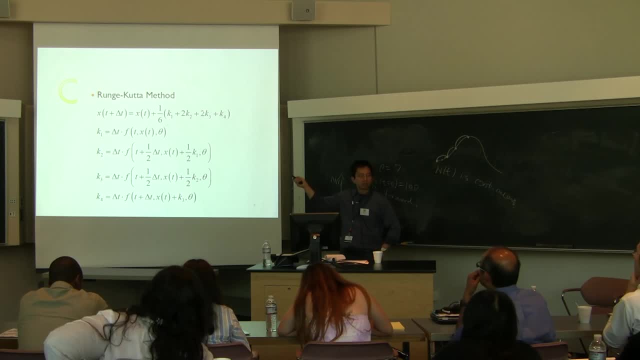 Instead of F multiplied delta T. I have a little bit more you know sophisticated term here, So it's K1 plus K2 plus K3 plus K4, okay, So if you look at K1, K1 actually is the exact same term as in the Euler method, right? 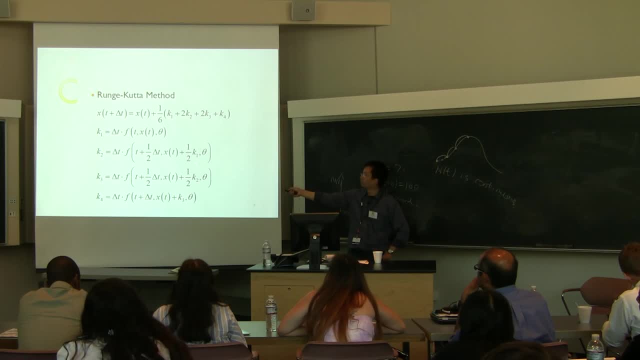 And K2, actually I use what I calculated okay for K1 here, Plugged it in and update my prediction. Then I use this prediction, update this prediction again, I get K3.. And finally, I use this prediction to update K4. 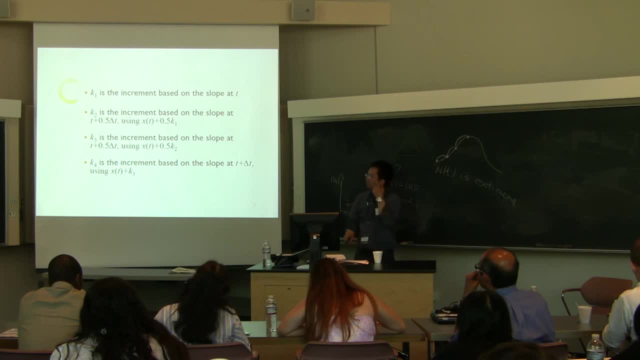 So what I'm talking about right now is a little bit difficult to understand, but if you go to this slide, okay, this will tell you. K1 is actually the increment based on the slope at T. We know slope is actually the derivative at T. 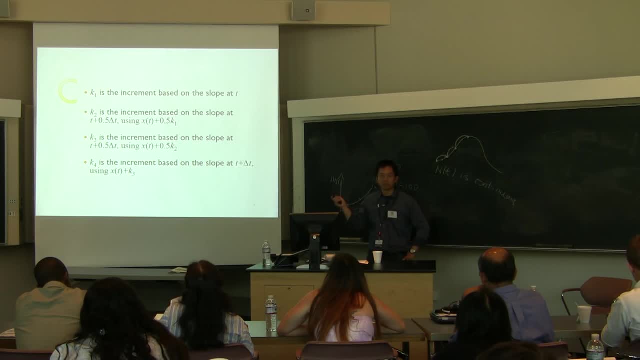 Okay, Slope derivative: they are the same thing. Okay, We have talked about this for quite a few times. So again, K2 is an increment based on slope at T plus half of delta T using XT plus half of K1.. 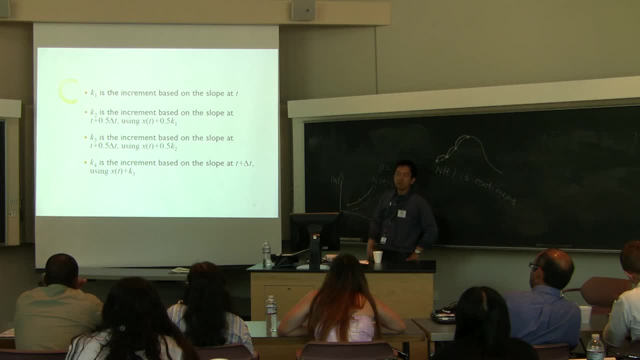 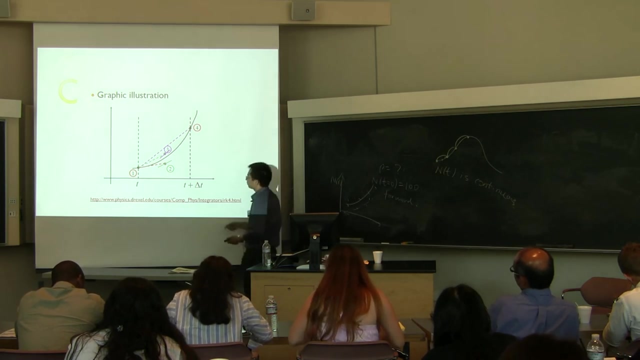 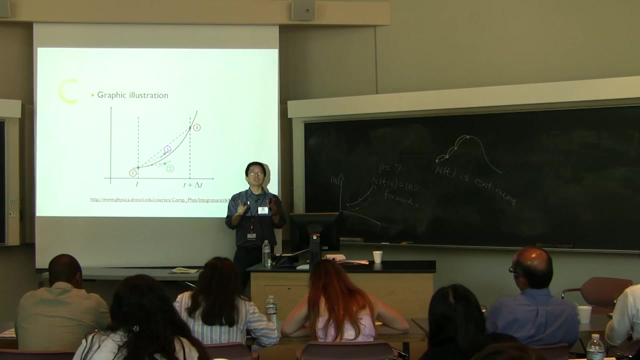 Similar for K3 and similar for K4.. So if you are saying that I still don't know what you are talking about, okay, here is a slide. That's why I have this slide. okay, So remember, when we start from K1, okay, K1 is actually the slope at time T. okay, 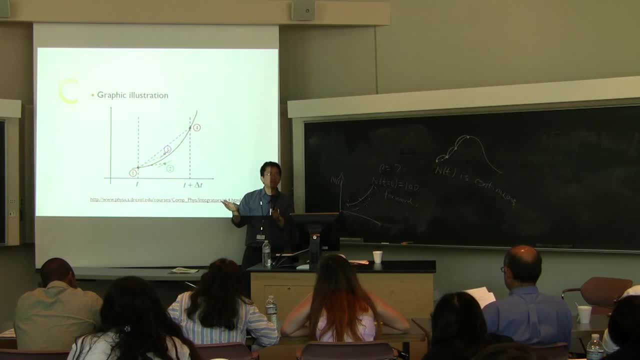 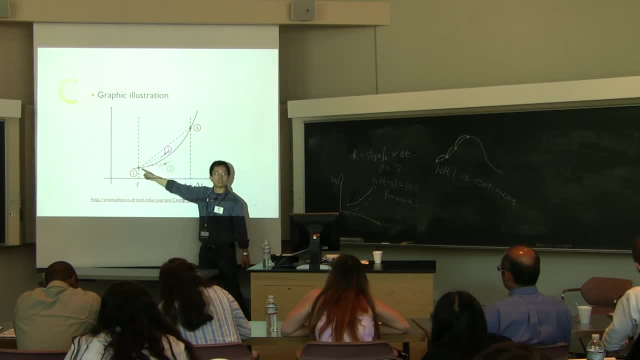 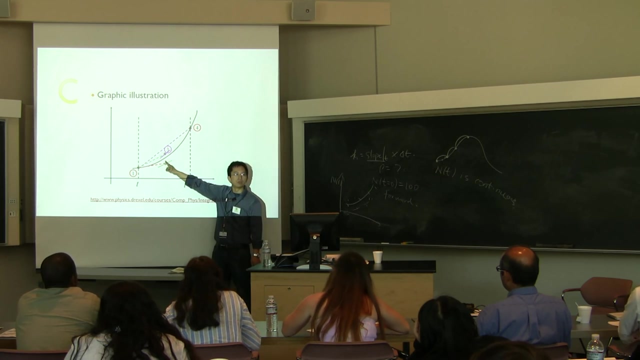 Where is the slope? This is a tangent line. okay, The slope of this tangent line is what you saw here in K1.. So I start from K1 and then I predict what the value of this curve will be at the middle. 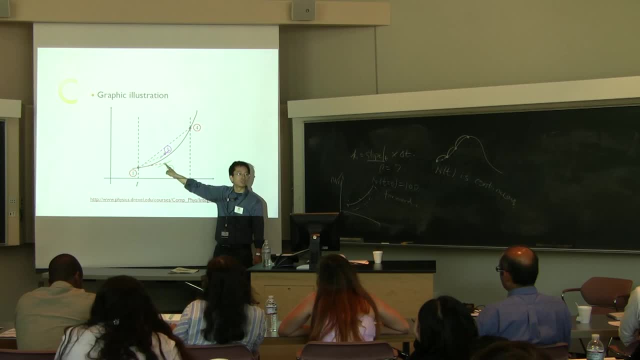 in the middle. okay, That's why you get K2, okay, And at K2, I calculate this slope again And I use this slope to calculate the K3. So these two lines they are parallel, okay. And the reason I do this is because I suspect if I only use the slope here, the results 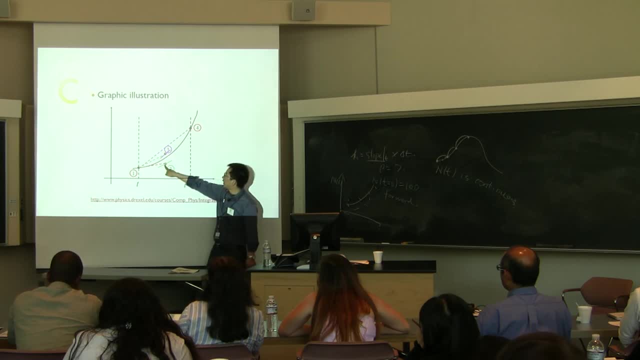 may not be correct enough, accurate enough, Then I do some correction. okay, using this prediction, do some correction. So I hope that to improve the accuracy. Same thing here When I get the slope here, I'm not sure whether it's accurate enough, so I do a correction. 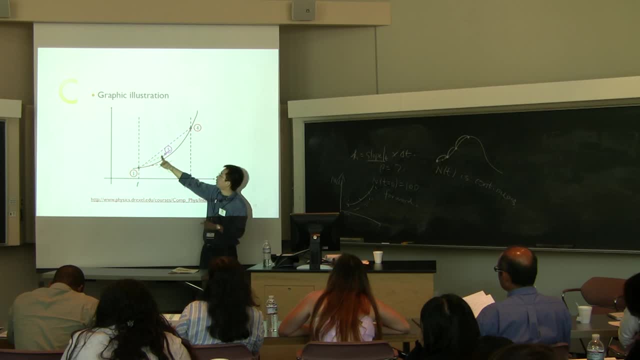 again. That's how I calculate the K3.. And finally, I use the correct correction again to actually calculate K4.. So these two lines are parallel because they are using the same slope. okay, So that's the idea behind the wrong quota method. okay. 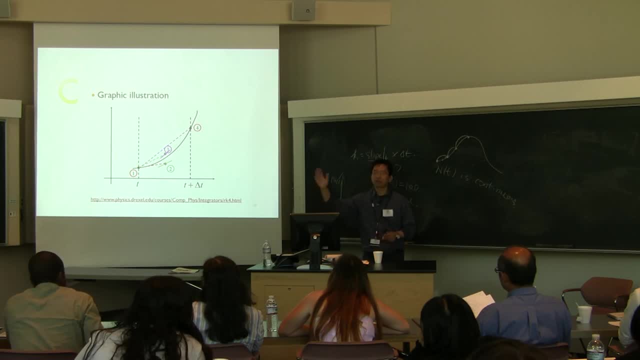 You predict once, but you improve it by correction, okay, Okay. So if you go back to here, you will see that's what I'm talking about. okay, You do a correction here, you do a correction here. So eventually you add them together and mathematically actually you can prove that. 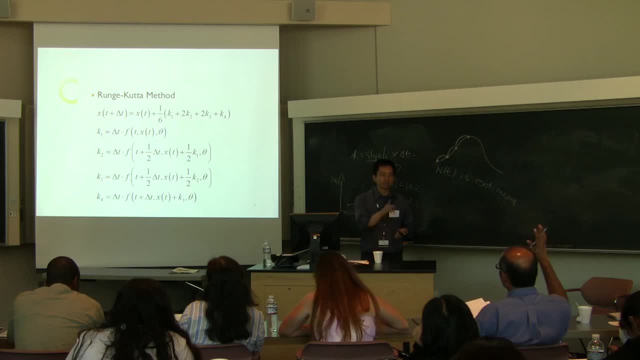 the numerical error actually will become much smaller. okay, But you could make it better if you do one-third or one-fourth, right, That's a good question. So actually I can a little bit extend that, Okay, Okay. 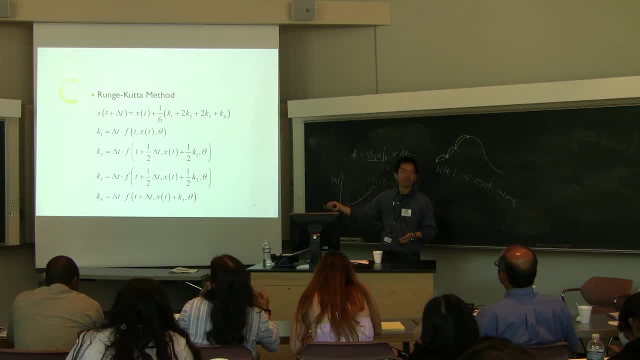 Okay. So that equation means: why don't we just use K1, K4? Or why don't we just use K2, K3?? So when people derive this kind of formula, okay, eventually they will derive a term. 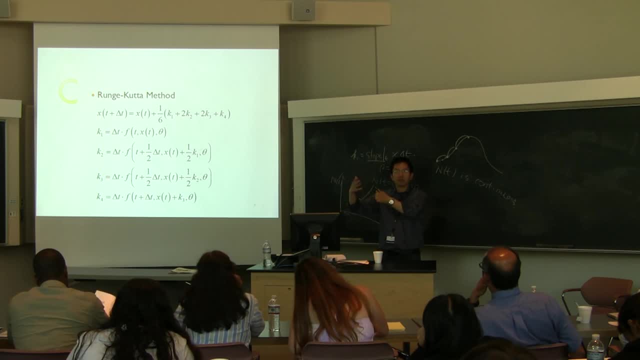 to approximate the numerical error. So this turn out to be a best balance, okay, And that's why you put a two here, put a two here and divide it by six. So there's actually an optimal balance, Okay, Between these four terms. 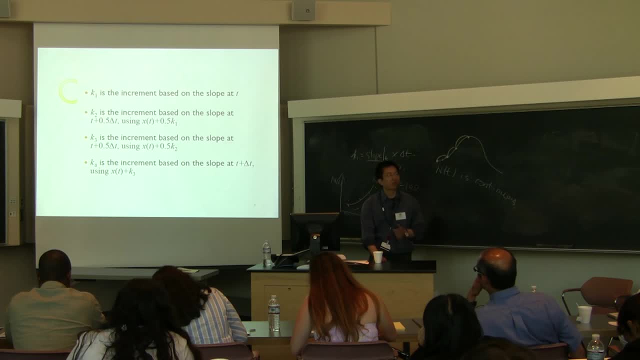 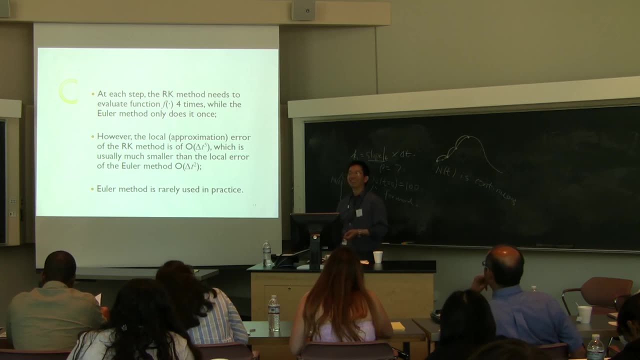 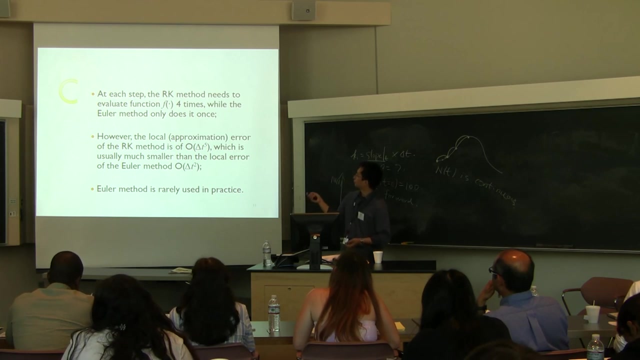 Okay, Any question? Good, Okay, Oh, no question. could be good, could be bad, Okay, So I hope it's not the latter one, Okay, So So if, after we derive the you know Run-Kutta method at each step, okay, we actually need. 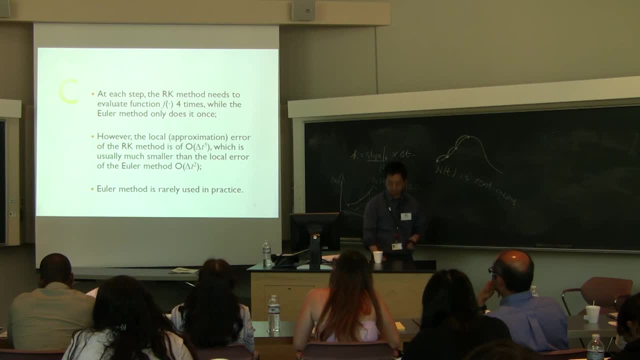 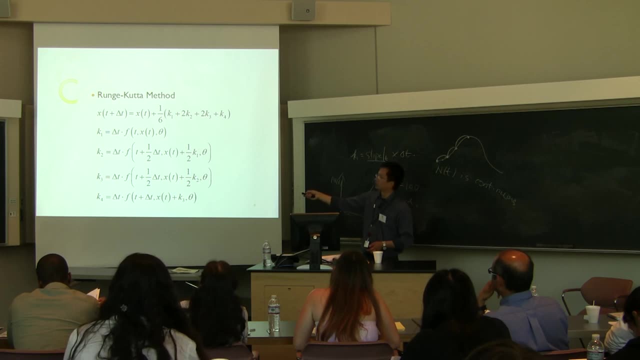 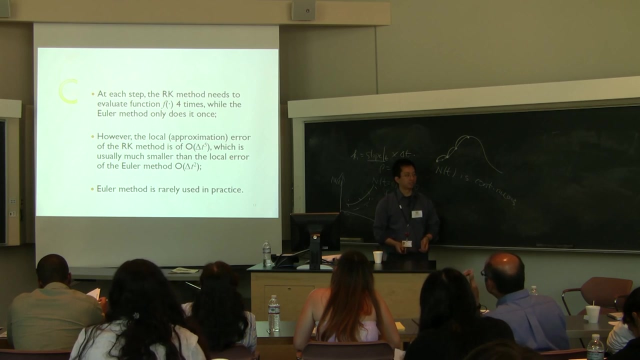 to evaluate the f function four times. Okay, Right, Because when we calculate the K1, when we calculate the K1, we evaluate this function once, Then K2, another time, another time and the fourth time. So computationally it's much more expensive than the Euler method. 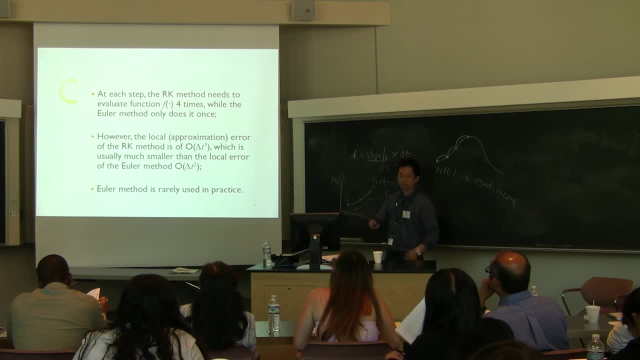 Right. However, the local error, like I mentioned before, the local error of the Run-Kutta method actually is of the order delta T to the power of five. We know that if delta T, You don't need delta E, You only need delta E is small. 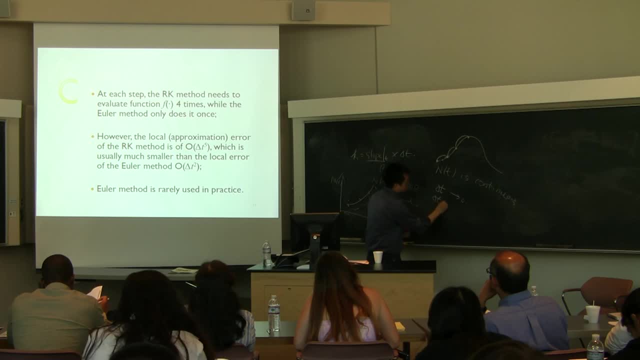 Okay, Close to zero. And if delta T, for example, is 0.1, then delta T to the power of five is equal to one. Right, So for the same delta E, okay, but the local error of the Euler method actually is to the. 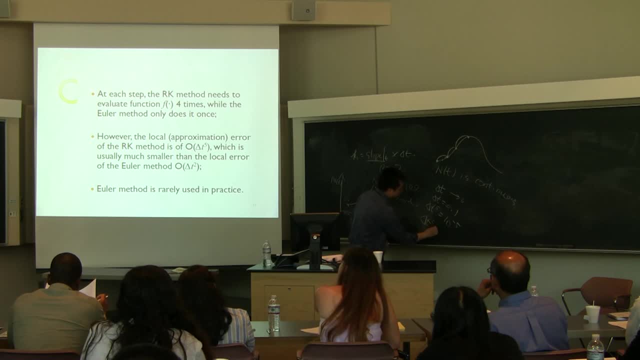 power of two. So for the Euler method, this local error is actually 10 to the power of negative two. Okay, So this one is actually much greater than okay 10 to the power of minus five. That's why, actually, in practice, I will strongly recommend not to use Euler method. 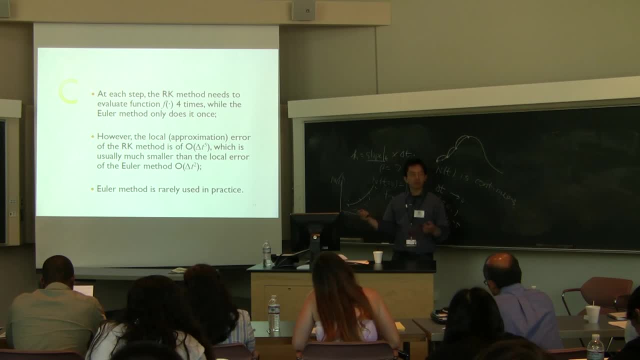 Okay, And if you use the Euler method- although you use it quick, but you, it's very likely you will get the wrong answer. Okay, And in my opinion, okay, accuracy should be prioritized as the first you know, because 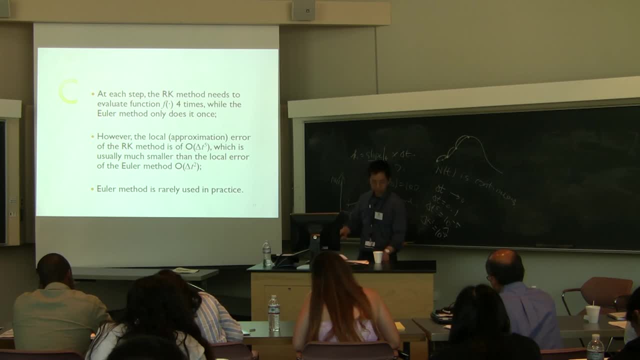 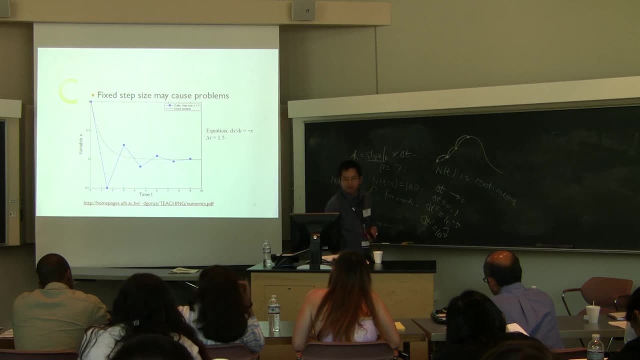 if you get the answer wrong, it doesn't matter how quickly you get your answer. Okay, You first need to get the answer right, Okay, So now, since we talked about the fixed the step size: okay, delta, T, okay, delta. 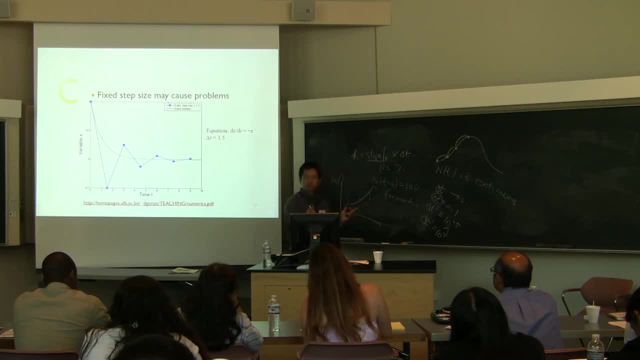 T is actually called a step size, which means the length of the interval we move from one point to the next one. Okay, Like here: Okay, This is delta T, This is delta T And this is delta T. Okay. 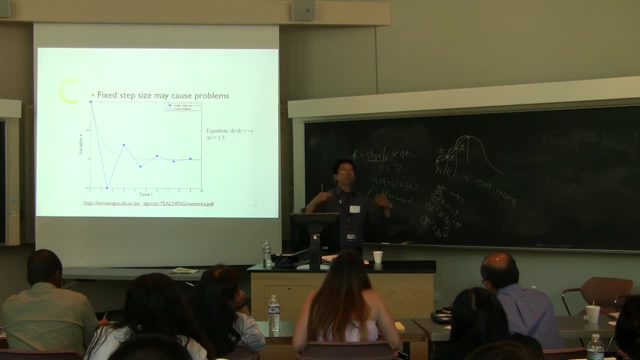 So it doesn't matter the Euler method or Runge-Kutta method we just described. Okay, We always can use a fixed step size in a solution, which means I fixed it to 0.1.. Okay, For you know, between all these points, 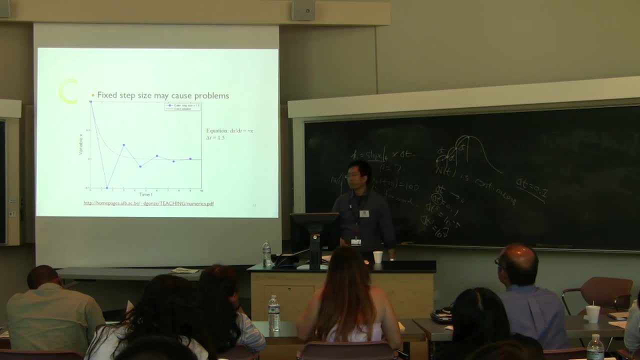 Okay, Fixed the interval at 0.1.. However, if you look at this plot, okay, I just used 0.1.. I just used the Euler method to solve this equation And I used a fixed step size. Okay. 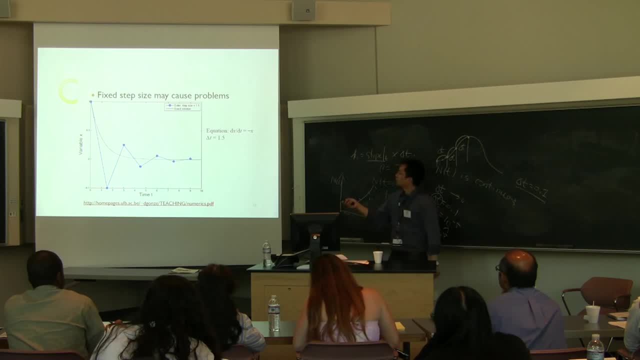 This is called a fixed step size. if this one is a constant, The problem is the approximation could be very wrong. Okay, Especially in a steep region. Okay, Right, But if you look at the tail region looks okay. There are some small error, but it's okay. 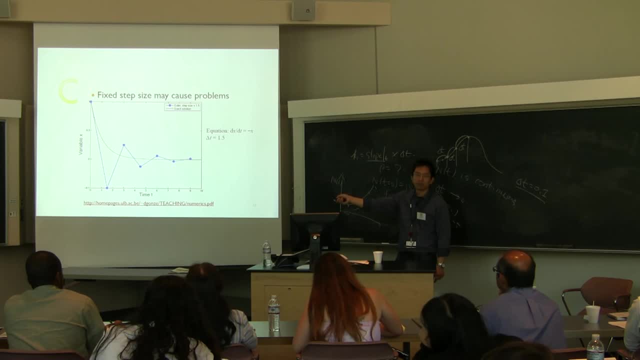 Acceptable, probably, But here it's too far away, Okay, From the true solution, And here it's also bad. Here it's also bad. So that's actually a common problem if we use a fixed step size. 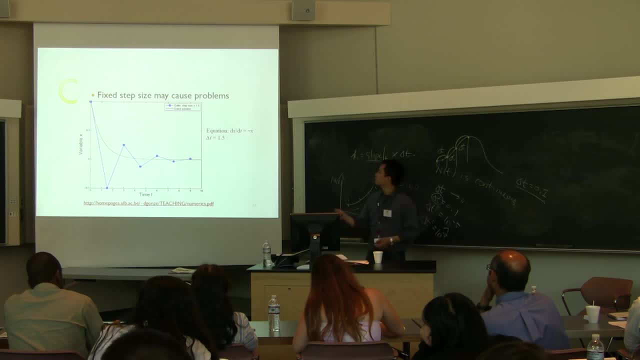 Okay When we solve the ODEs. So what do we want actually? What's the ideal step size we want? So we would like to have a strategy that can automatically reduce the step size So I can better approximate the steep region. 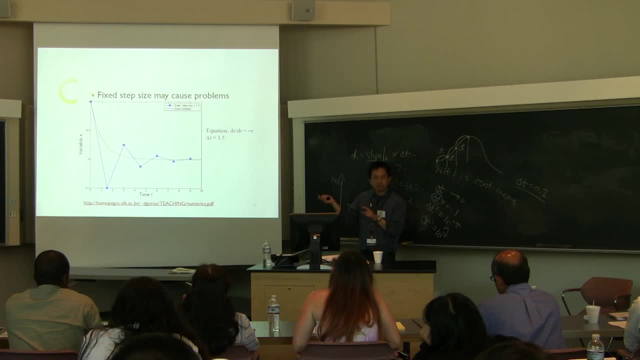 However, I don't mind to have a longer step size, Longer or bigger step size in the fried region, Right, That way I can get accurate approximation to all the you know all the parts of the trajectory, Right. So that's, that would be ideal thing. okay to do. 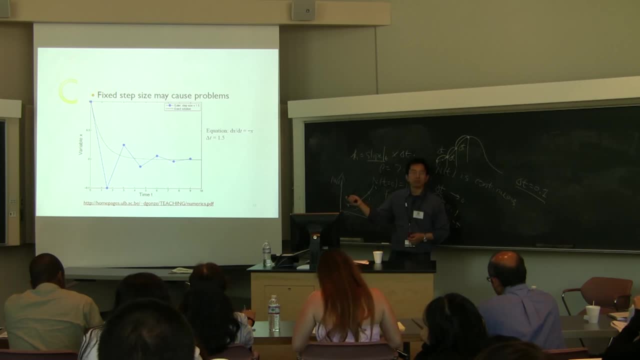 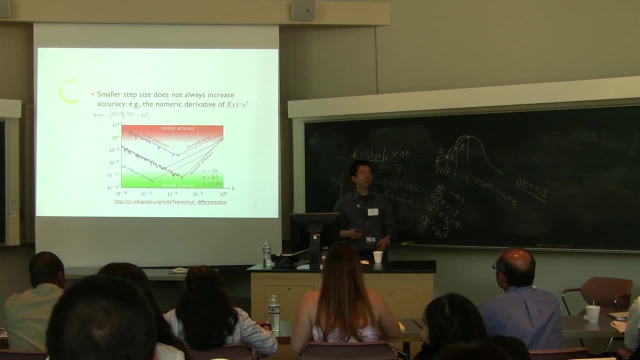 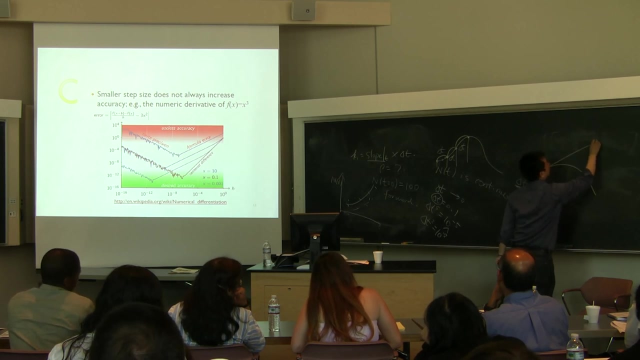 And also one serious problem associated with fixed step size is that we actually will expect that If we reduce this step size, we will get more accurate results. Is that true? For example, if I use a big step size, then I should far away from the true trajectory. 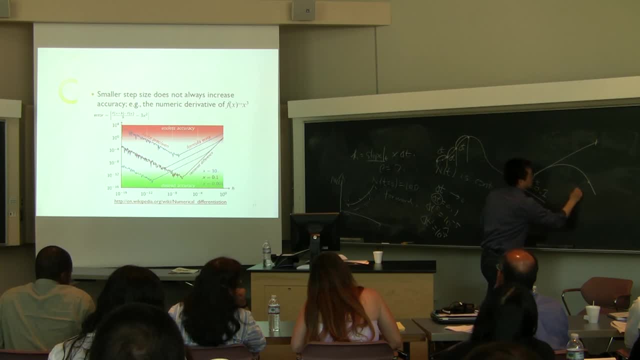 Right, If this is my T plus 30. Okay, If the step size is too big, Then I should. I should, far away from you, know the true solution Now if I reduce the step size to here: Okay. 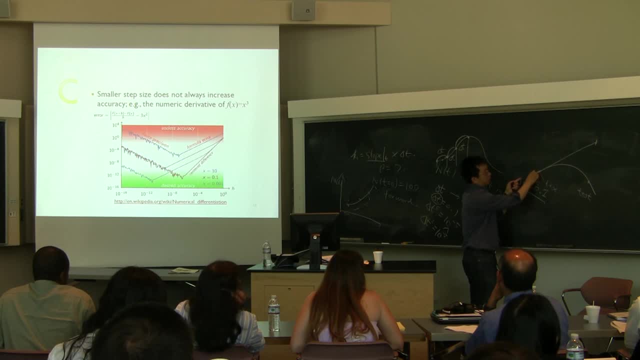 If my T plus 30 is here, Then the approximation looks okay. Right, So I can do the same thing here If I reduce my step size here, Just to use this small time interval and to approximate the value. update the value here. 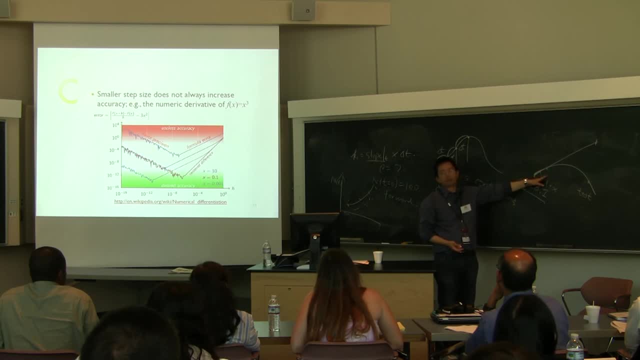 Looks still okay, Right. So intuitively, you will see that if the step size is smaller, then you will get better solution or more accurate solution. Unfortunately, okay, this is not always true, So here is actually an example. 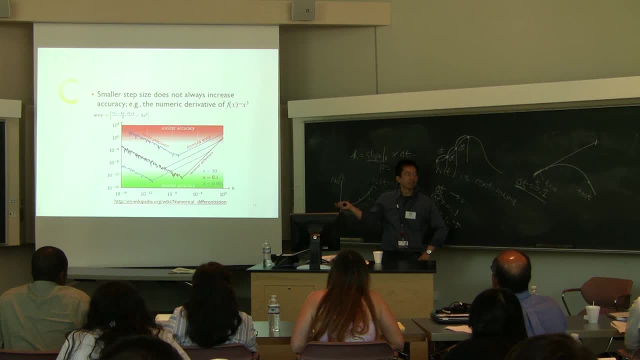 We just H. here is the actually delta T. Okay, Notation changed a little bit, Sorry about that, But here H actually is the delta T, Which means if I change the step size, Okay, What will be my approximation error? 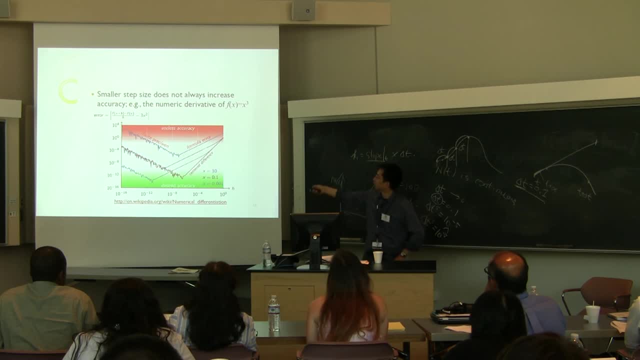 Originally, we expected that this curve should be a monotonically decreased line if H gets smaller. Okay, I'm looking at it in this direction. Okay, However, you see, you actually will jump back. So why is that? The action is. 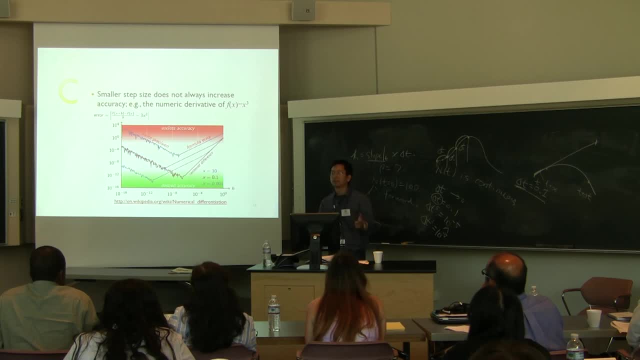 The action is because the computer- Okay, Computer- cannot store infinite digits of number. Okay, After computer has precision also. So after a certain digits it will cut off the rest of the digits. That's called rounding error, Okay, 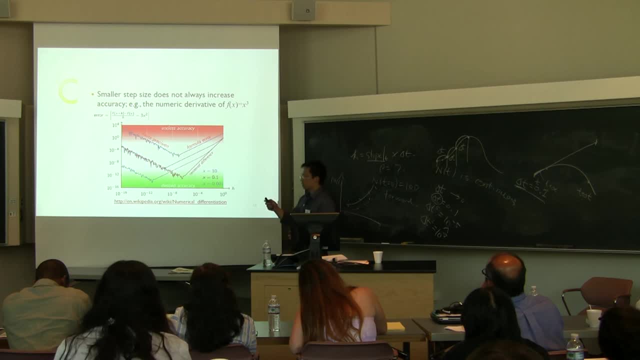 And once you cut that off, then you will get a small error. Okay, So you only need two. Okay, If you ask a computer to store number two in a memory, what indeed it stores is not two. Okay, 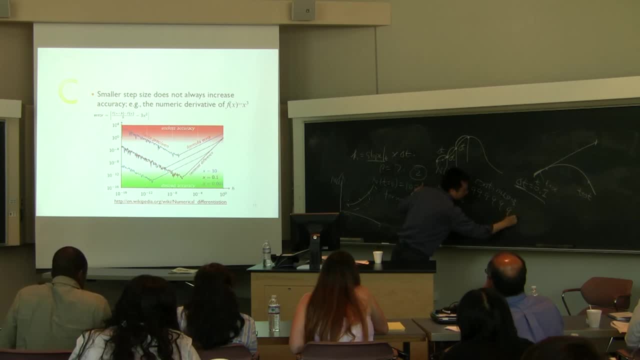 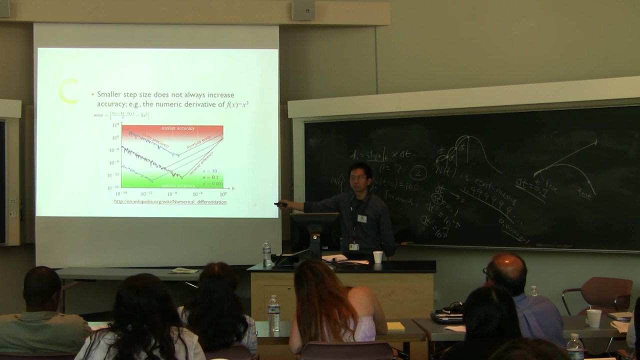 You only need to store is Okay, So you will loss a small digit. Okay, For example, like this: And this one, you only doesn't matter, Right, This one, you only doesn't matter. However, here you also want your delta t becomes very small. 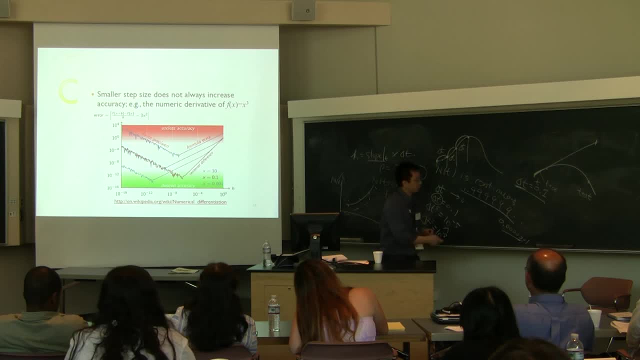 Once these two actually become comparable, for example, your h also becomes this small, Now small number. divide another small number, You actually could get a larger number Right: 10 to the negative 10 divided by 10 to the negative 20.. 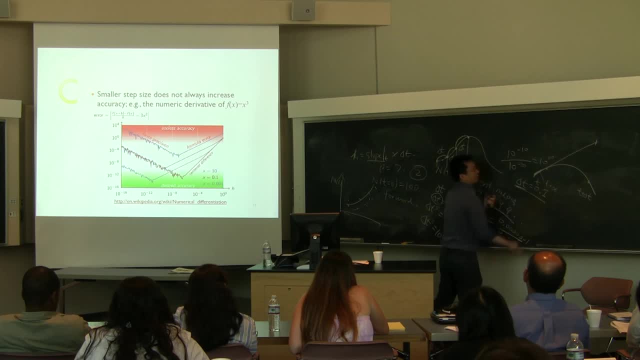 What's the result? 10 to the power of 10.. So you will get a very large number. So that's exactly what happened here, Okay. So if you make your time interval too small, okay, this kind of rounding error will kick. 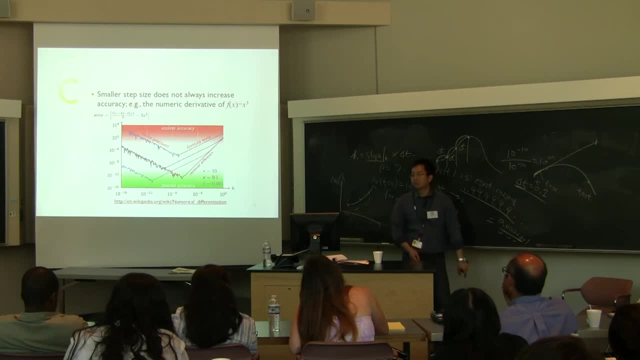 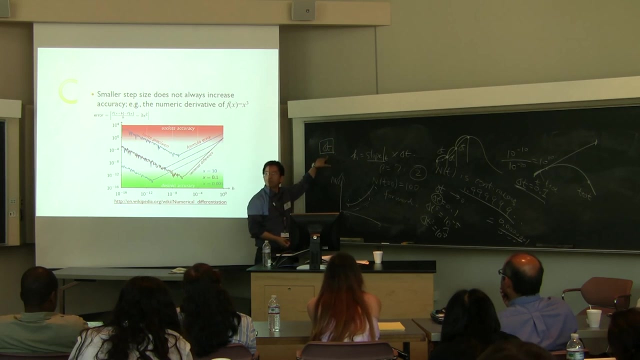 in and you will get totally wrong answer. So that sounds like a big problem, Right? So I first, if I solve ODE. okay, I want to pick. Okay, I want to pick a reasonable delta t. 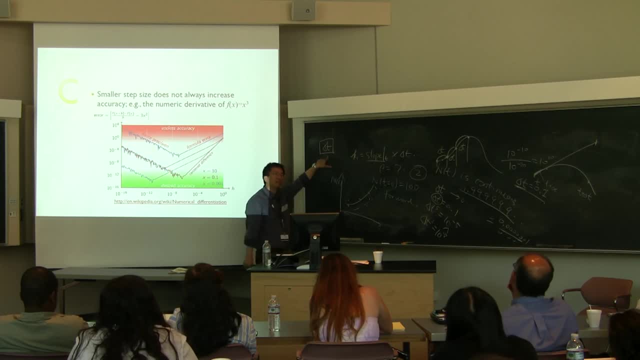 Reasonable delta t, which means it will give me a solution that has acceptable error. Okay, But how? How to choose this delta t? Unfortunately, the answer is not depends. Okay, So there are some strategy we can actually control. 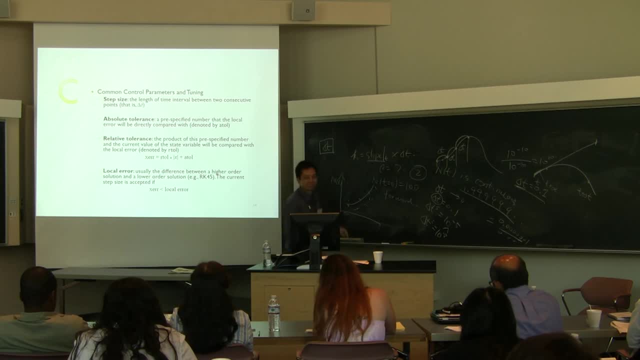 We can automatically select the delta t. okay, step size. So if you're using ODE solver, okay, we call the numeric algorithm or functions that solve ODE solver. Okay. If you use a solver in my lab or any other package you like, sometimes the solver will. 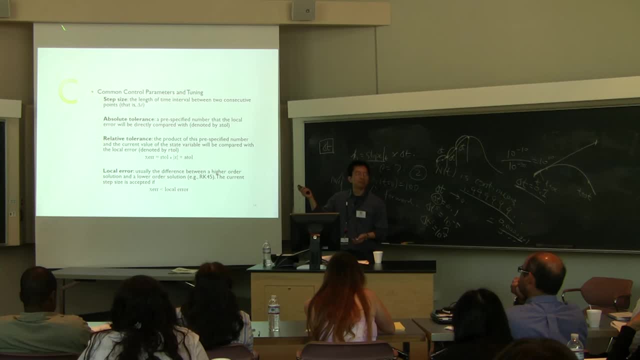 provide you a control parameter named step size. Okay, So you can actually manually specify the step size, but I will not recommend do that, Okay, So here is. here are two other actually control parameters actually we usually use. 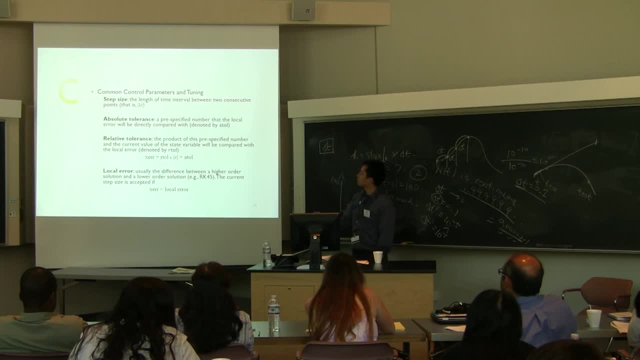 to automatically determine delta t. Okay, The first one is called absolute tolerance. The second one is called relative tolerance. The first one is more like a pre-specified number that a local error will be directly compared with And the solvers in my lab or in ddiscover- that's our own package- will give you a default. 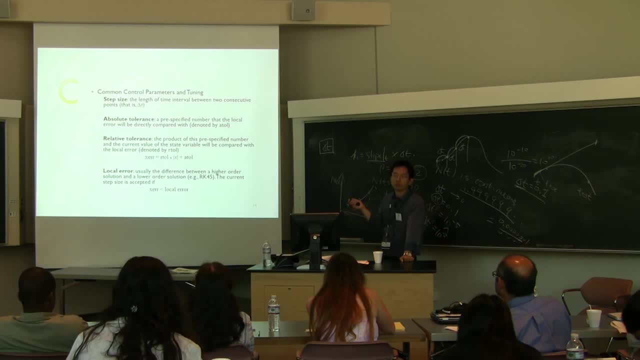 value: Okay. So if you don't know what to what value to use, you can just start with the default value. Okay, Same thing here: Relative tolerance. it will have a default value And the product of this number with current value of state variable will be compared to. 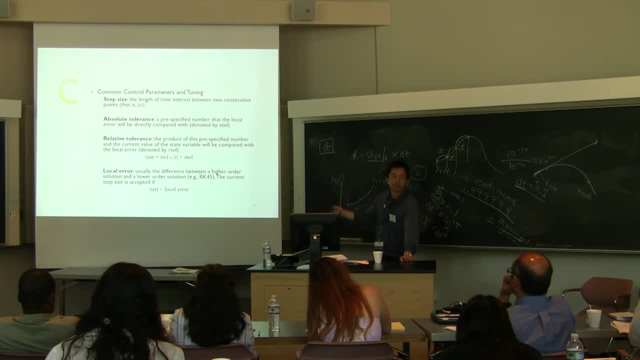 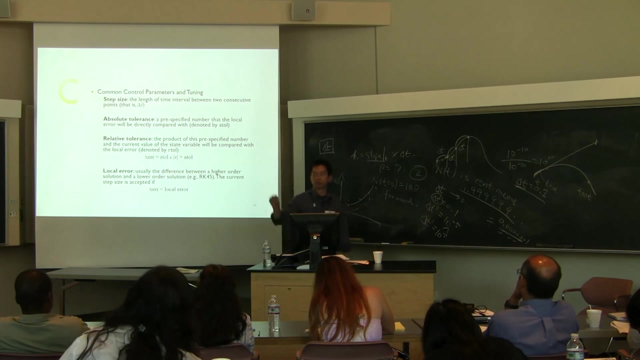 a local error. Okay, So that's actually the formula we are using to control the local error. So the relative error tolerance multiply the current value of x now plus the absolute value, absolute tolerance, Okay, And that's our total error we want to control. 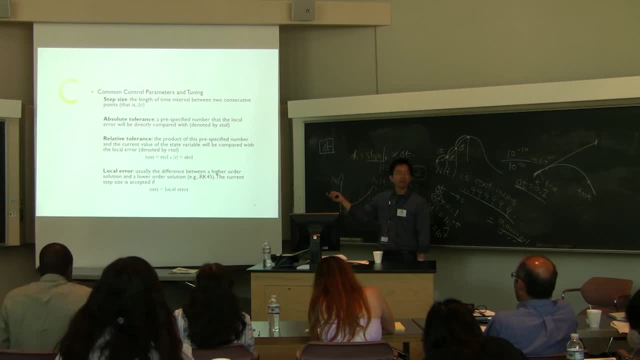 Okay. So, by definition, if I decrease the absolute tolerance and the relative tolerance, will I get a better solution or worse solution? Okay, Error is smaller, which means the solution is better. Okay, So if I decrease these two numbers, I will expect to get a more accurate result. 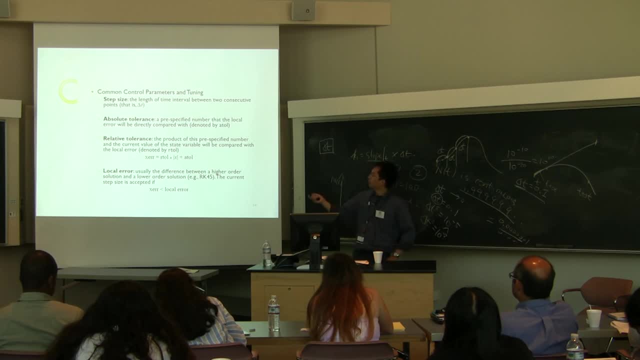 Right Now. so why people use this kind of, you know, tuning parameter or control parameter instead of just directly control the step size? Because the problems in practice, okay, have many, many different timescales. Okay, If you are modeling the long-term infection, you probably use a unit of the time of unit. 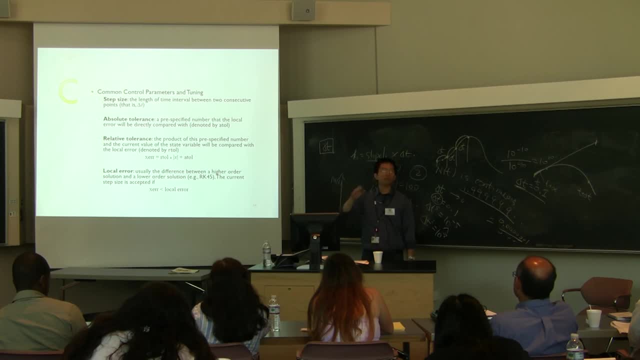 probably will be a year. But if you are looking at you know the molecular interaction. the unit will be like a microsecond. So in essence you have to use a very different for problems of different timescales. 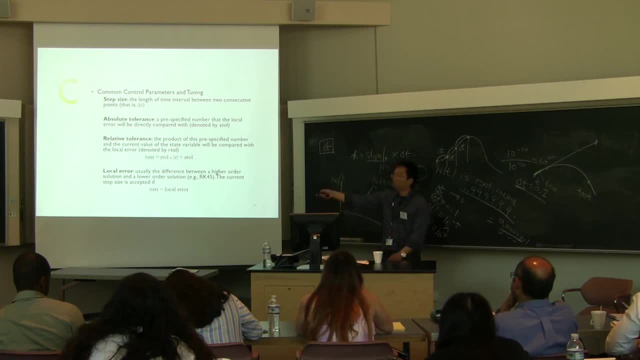 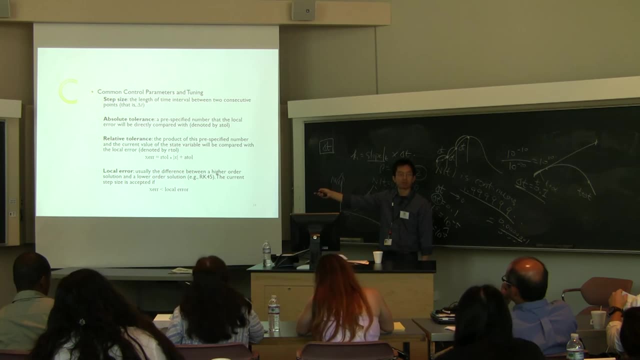 So to save that kind of trouble, you can actually just control this. two numbers, Okay, And for all the you know problems of different timescales. So that's one convenience, Okay. So another thing I want to talk about is that here we have this error actually is. 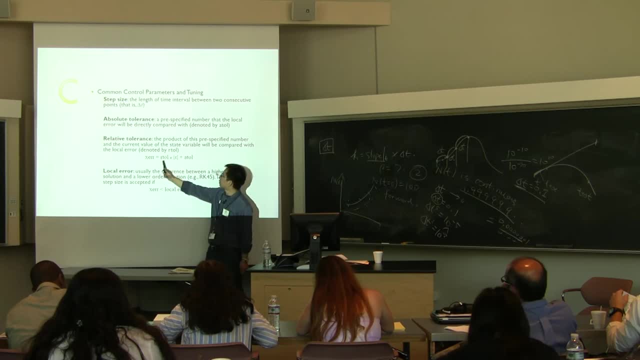 specified by user. Okay, We specify this relative tolerance, We specify this absolute tolerance, And then we'll calculate the error. However, we need to compare this to something Right. Then we know whether it's a good or bad error. 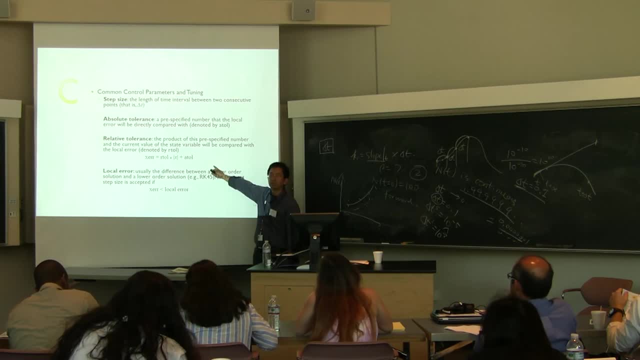 Okay, Whether this error is acceptable or not. Here we just calculate the error. Okay, We didn't actually compare it with anything yet, So if you don't do the comparison, then we still have no idea. Okay, Whether we should increase the step size or decrease the step size. 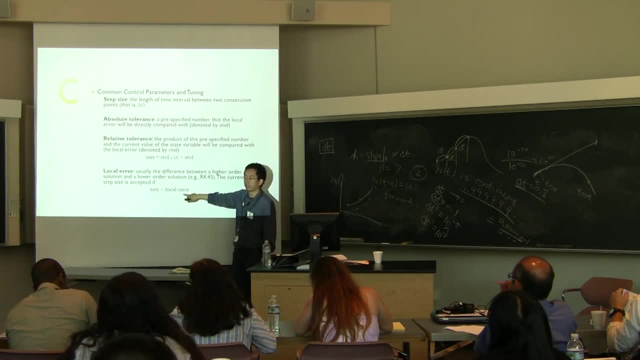 So that's why people also need to calculate when you use the algorithm. Okay, The algorithm actually will do this for you. Okay, You don't need to worry about this local error. Okay, So how we actually get this local error. That's actually a chicken and egg problem, Right? Because we don't know the closed form solution of the ODE. That's why we use a numerical solution. Okay, And if we use a numerical solution and we have no way to actually calculate the numerical? 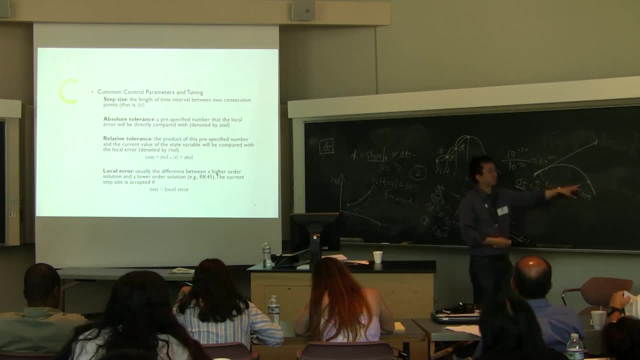 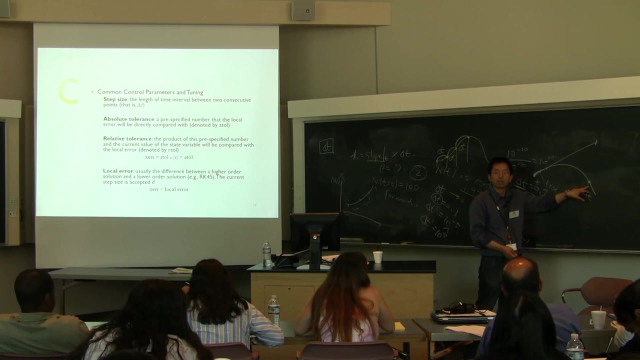 error or approximation error Right From the trajectory, Because we don't know that yet. If I shoot from this point to the next point, Okay, If I have the exact solution or closed form solution, I will actually be able to tell what's the true solution here. 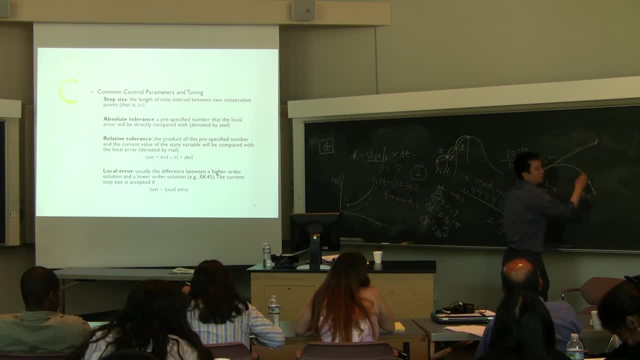 When we use a numerical solution, we can only shoot from this point to the next one. The true solution we don't know yet, Right? So that's why I'm saying it's a chicken and egg problem, Okay. However, there's some remedy for this. 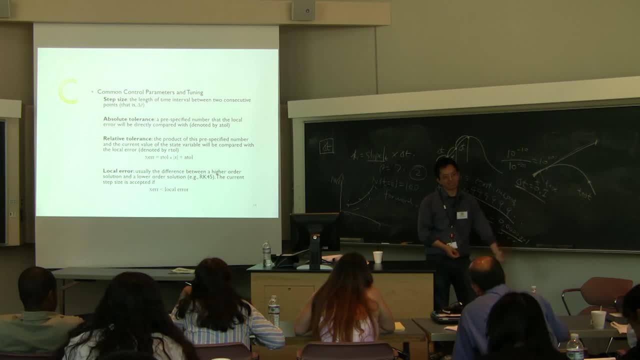 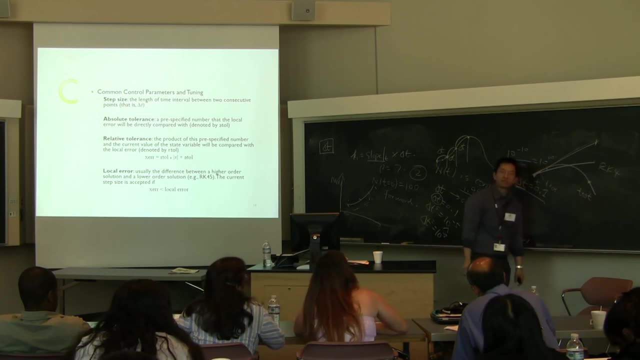 Okay. So the remedy to this problem is that we solve this problem twice. Okay, First time, I solve it with less accurate method, For example RK4.. Okay, Next time, I solve it with No. Here it should be. 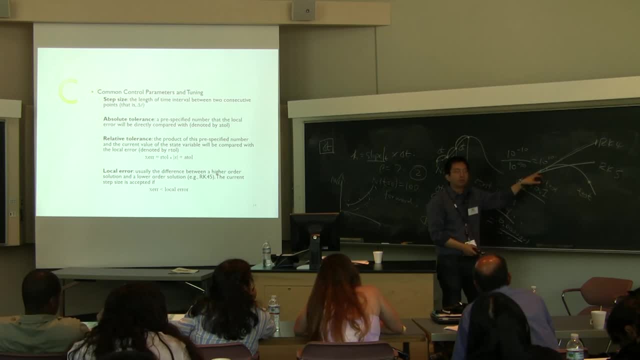 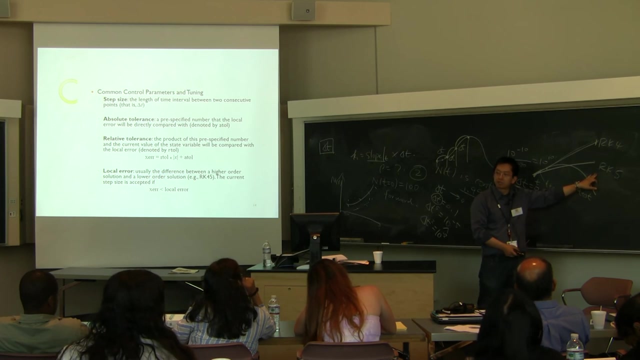 Yeah, Because this one is more close to the true solution. So what people did actually is solve this step using a lower accuracy algorithm, RK4.. Then I solve it again Use a higher accuracy algorithm, RK5.. Then we take the difference between these two as a local error. 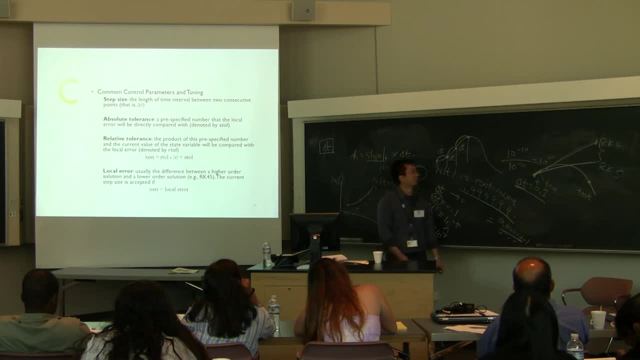 Okay, That's what people do. It's not perfect, but that's how it works. Okay, So you solve it twice actually, But the computing cost is not actually doubled. So there are some strategies actually to save some, you know, computing costs. 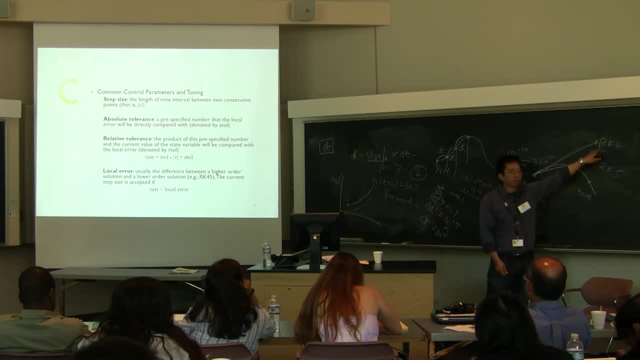 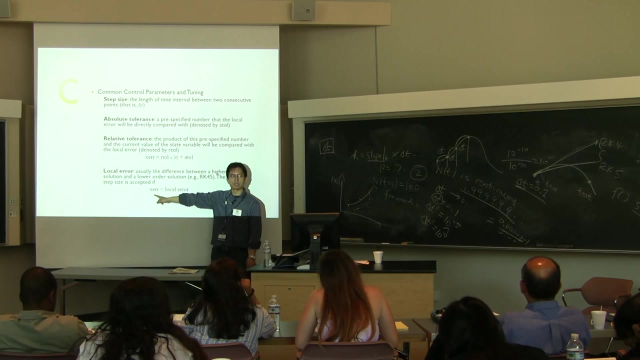 So, Actually, if you use this algorithm, you will evaluate the F function five times only. Okay, Not actually eight times. Okay, It's not eight times, It's actually five times in total. So once we approximate a local error, I can compare to my user-specified tolerance with the local error. 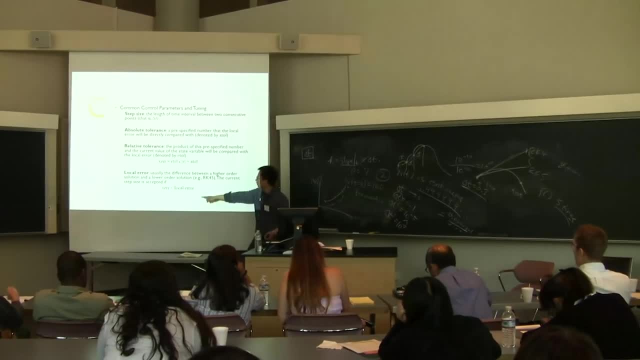 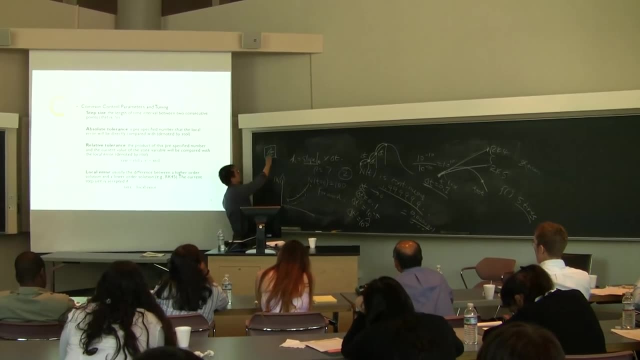 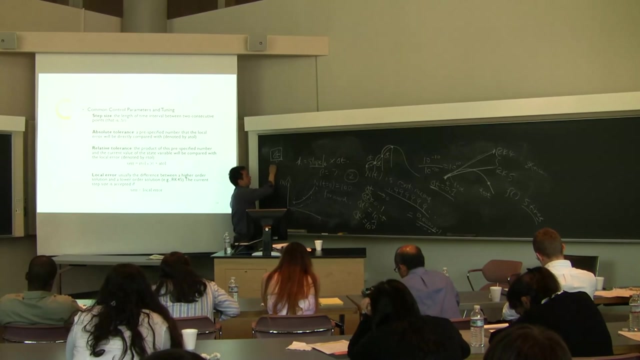 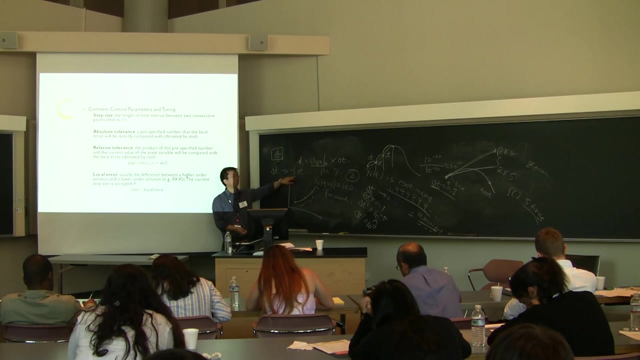 So what I will do is that if My user-specified tolerance is smaller than the local error, I can accept the current step size. If this error is greater than the local error, I will reduce my step size to half of Half of the you know step size. 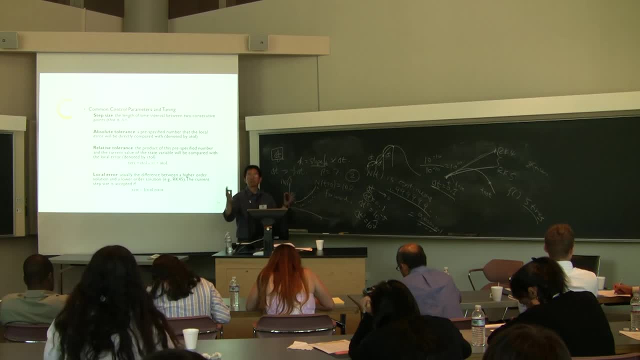 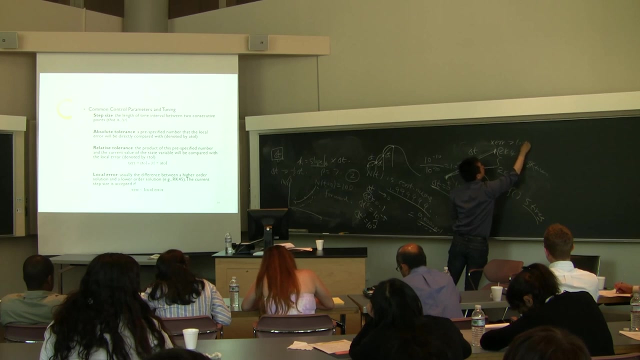 And I calculate again: Okay, That's how the algorithm control. Okay, Automatically control the step size. For example here: If, here, If this step size is too big, Okay, And the user-specified tolerance is greater than the local error, what I can do is reduce the step size to half of the original step size. 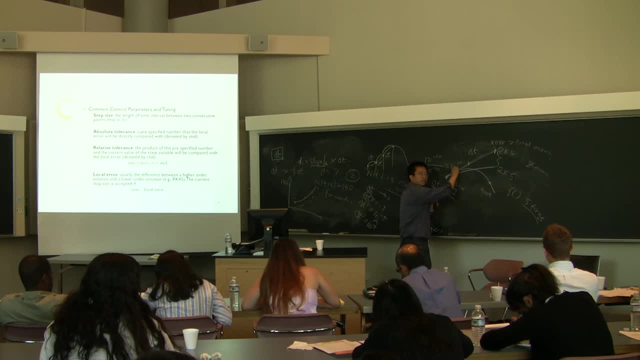 If it is still bad, I can do it again. Okay, So in that way you will find a step size that eventually Such that this error will be less than local error, Local error- And then you accept that step size. 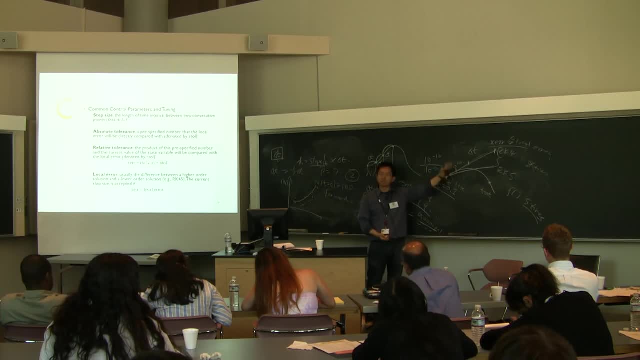 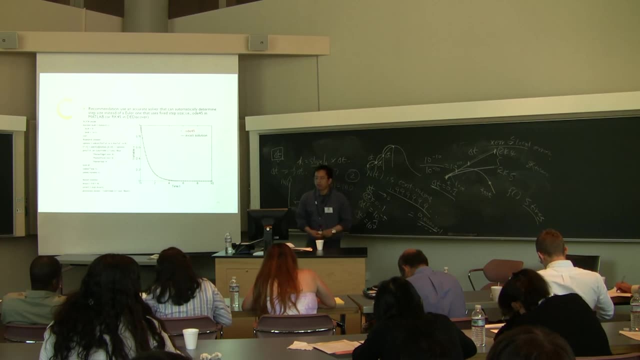 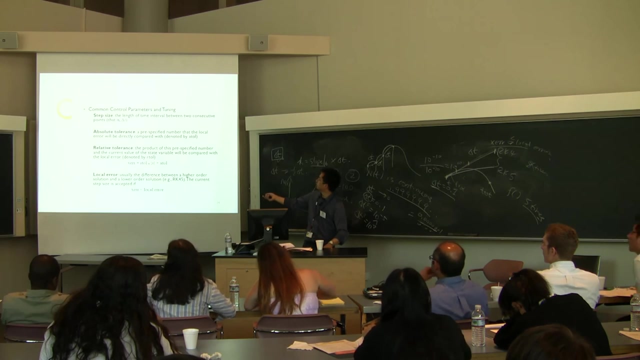 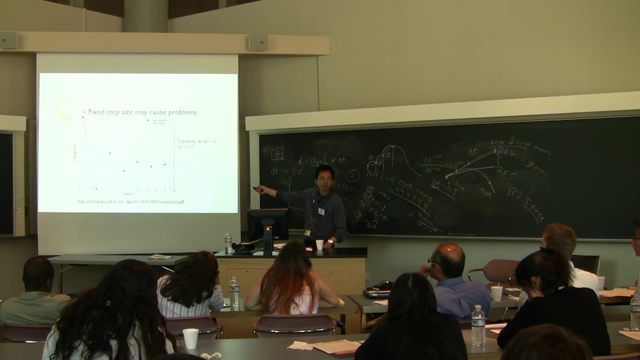 So that's how the algorithm automatically determines the step size for you, Okay. So Now here's an example. Actually, I'm solving the exact same problem, Okay, As in this slide. Okay, In this slide, I used a solver with a fixed step size. 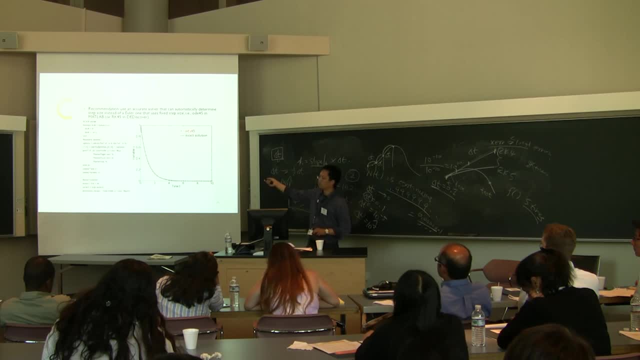 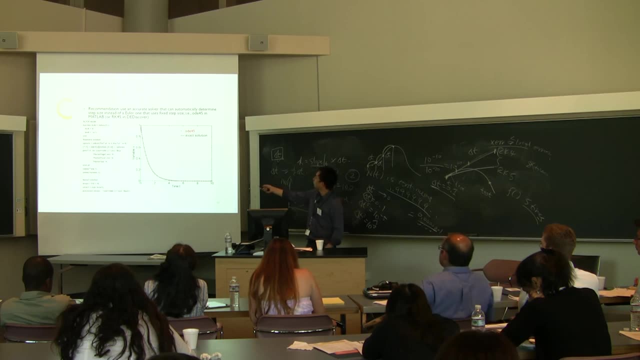 And in this slide I solved the exact same problem with a solver of automatically determined step size. So now you can tell in the steep region the step size is actually varied. Okay, This is not a fixed step size, This is a varied step. 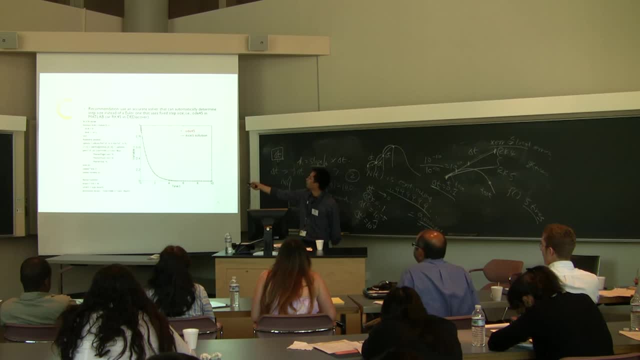 Automatically. you know varied step size. So now all the solution- approximation actually falls over, Falls on the you know exact solution. Okay, You don't get this problem anymore, Right? So now the approximation looks pretty well. 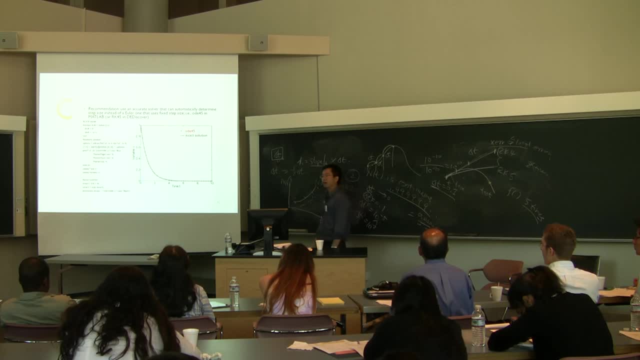 Okay, All right. So that's why, when you use the Whatever package, I will recommend you to use accurate solver like Runge-Kutta method with automatically, With automatic step size option. Okay, So this automatic step size actually increases accuracy a lot. 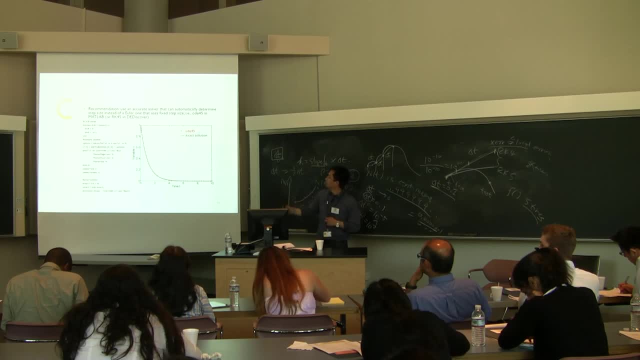 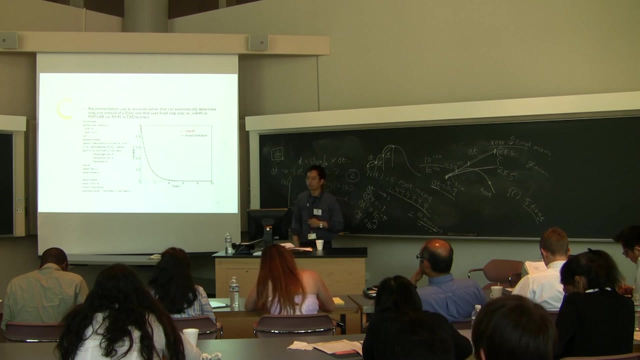 Okay In this region. So if you are interested in, or you have the MATLAB on your computer now try this paragraph of code: Okay, That's the code actually to solve the equation. and the plot: Okay, Do the plotting. 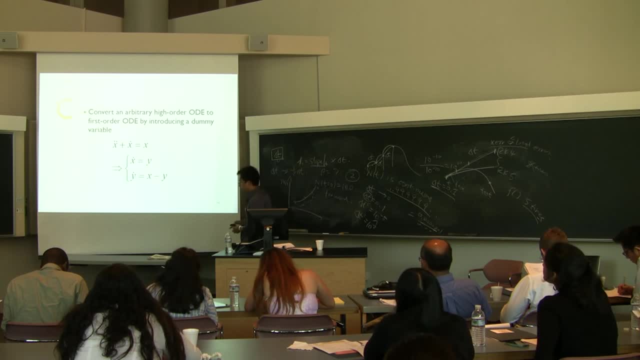 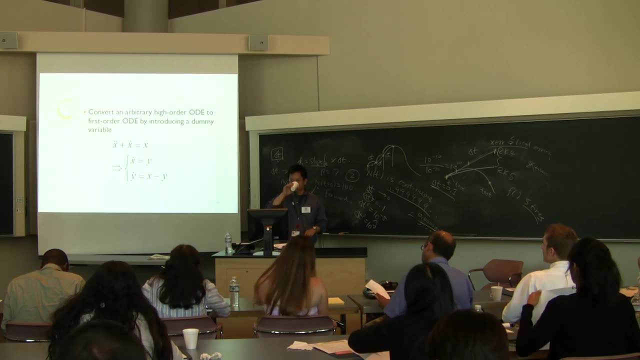 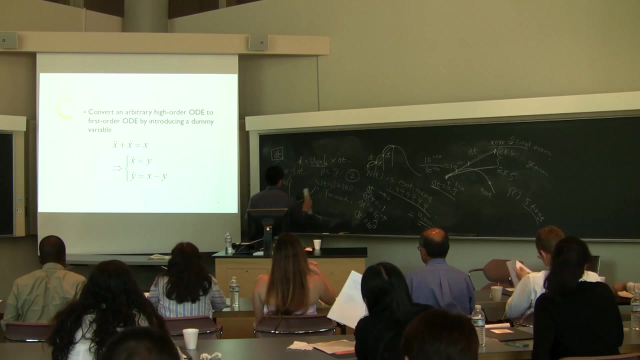 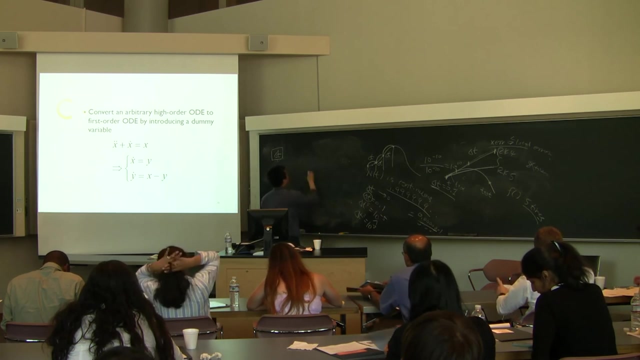 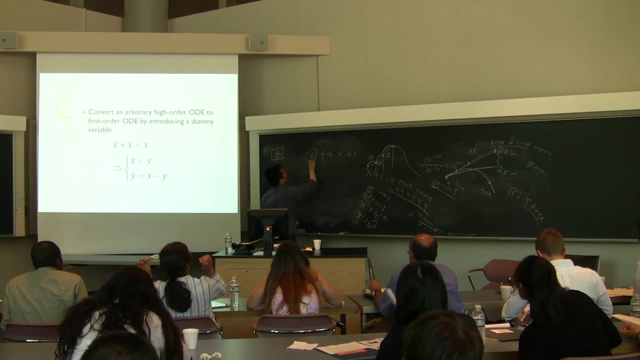 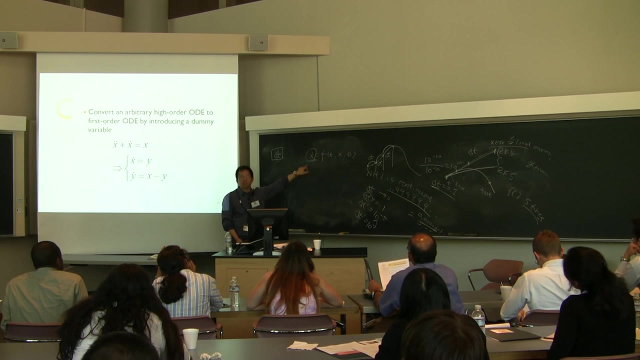 Okay. So now we have talked about ODE's. Okay, First order, ODE's. Okay. We call it the first order ODE's because the order of the derivative is one Okay, Which means we only take the derivative once. 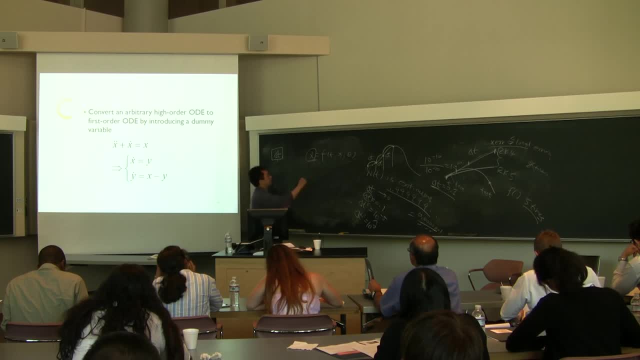 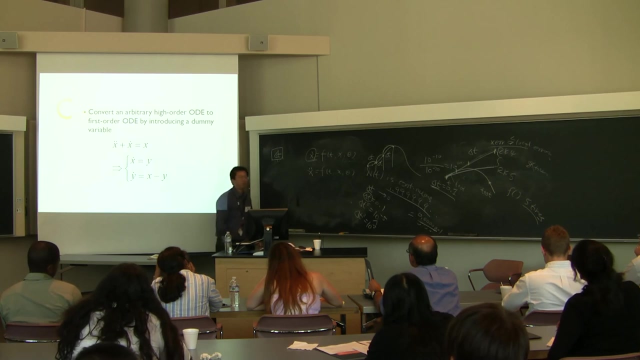 Okay, But you can also get a higher order ODE's, which means I can take the derivative of x with respect to time twice, So you get the two dots Okay, Which takes to. That's also called ODE, Okay. 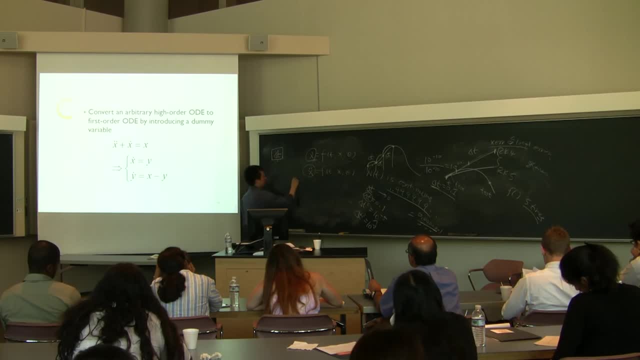 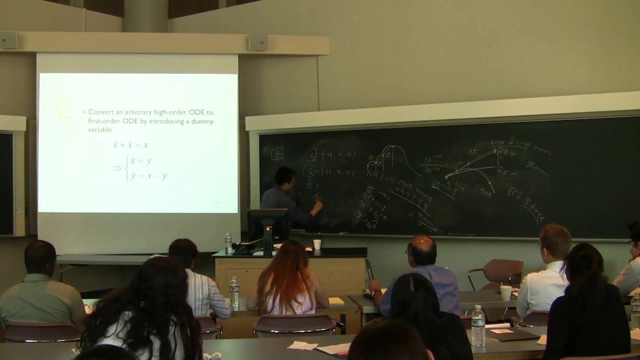 So what does this mean? We know x dot is equal to d dt, x. Right, Take the derivative of x with respect to t. If I put two dots there, actually, what we do is take the derivative of x with respect to t once. 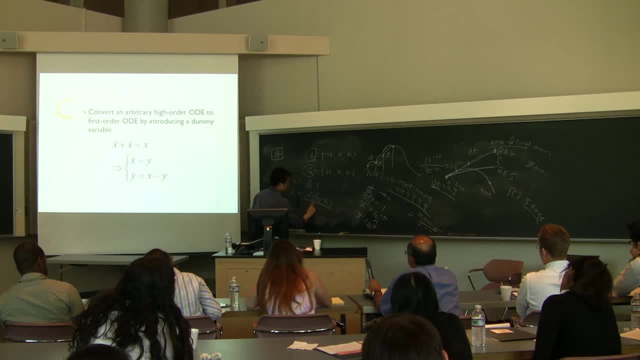 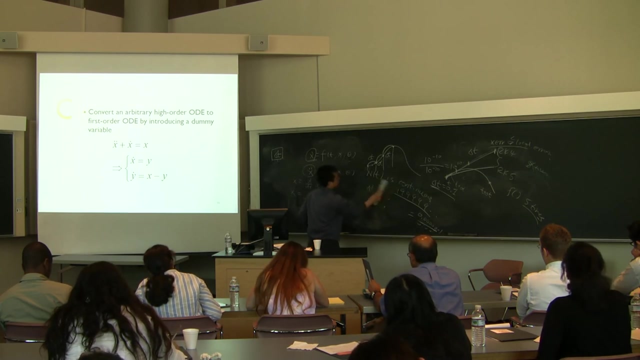 And then take the whole thing. Okay. With respect to t, again, That's what it means. Okay, You calculate the slope of the slope? Okay, So that's the second order version. So if you want to plot it, actually it's not that difficult. 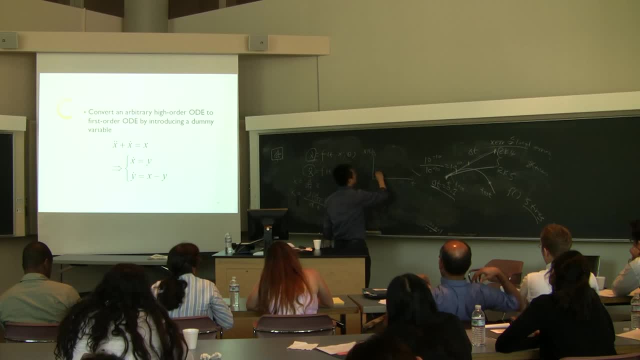 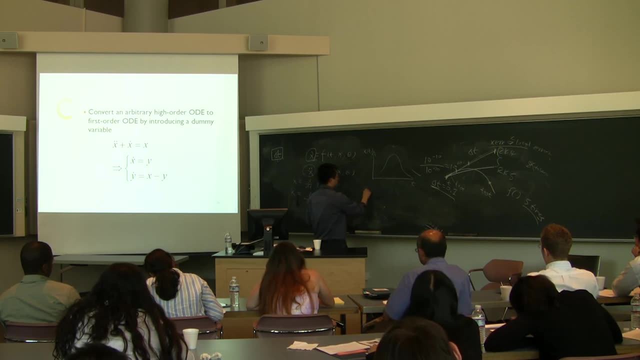 Okay, So If this is my original curve and then if I want to plot the derivative of this curve, then actually I'm plotting the slope of this curve. Right, I have a dot here, Okay, So what will be the slope of the curve? look like: 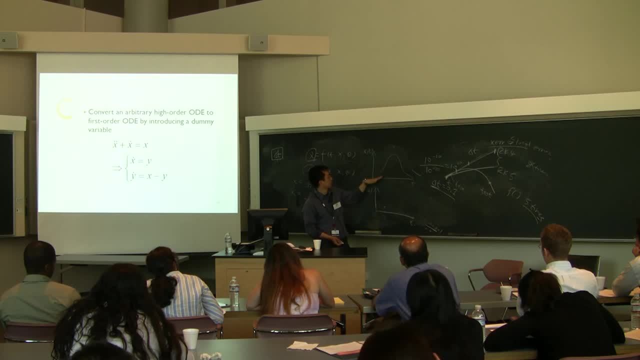 This is a positive slope. Right Start from here. It's a positive slope And gradually it becomes flat. the slope, Because the tangent line of this at this point is this direction- The slope is zero. And then this slope becomes negative. 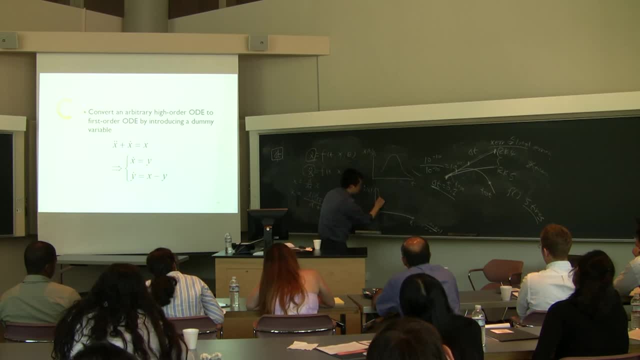 Right, So I will get a curve like, Sort of like this: Okay, So now again, if I want to plot the slope, of the slope I start from here Probably look like this way: Okay, Let's make it nicer. 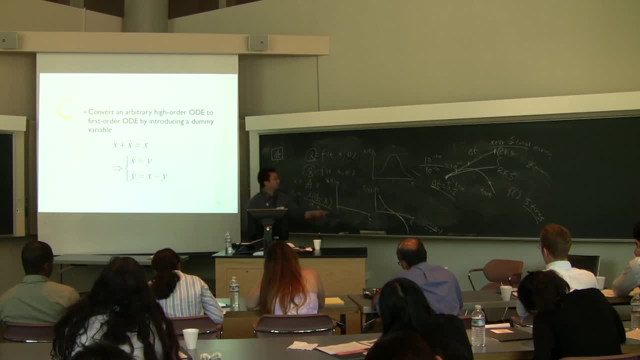 Okay. So what's the slope here? It's a negative slope Right, And gradually it becomes what? Positive? No Negative, Negative, Negative, Still negative, But The, The, The, The, The. 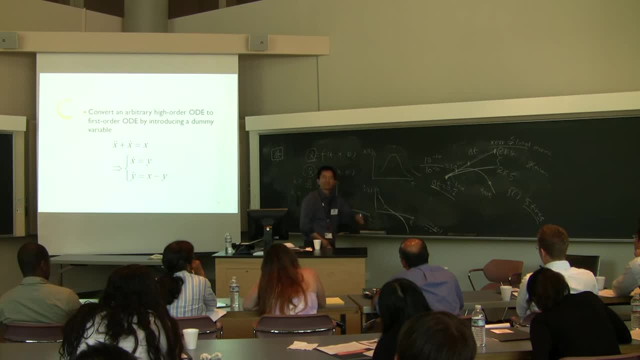 The, The magnitude becomes smaller Right, And then magnitude increases, But it's still negative Right. So if I plot the oops, here's a zero, I will stop from here. It's negative And the magnitude becomes smaller. 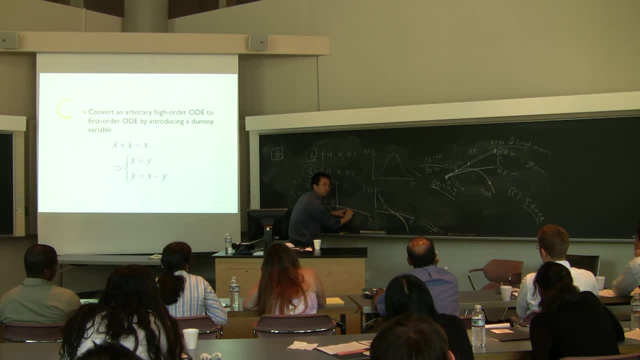 Which means it will be closer to a zero And then the magnitude will increase. Then it will go this way, Right? So it always negative, It's always negative, but the magnitude- absolute value, okay- gets smaller and then getting bigger. 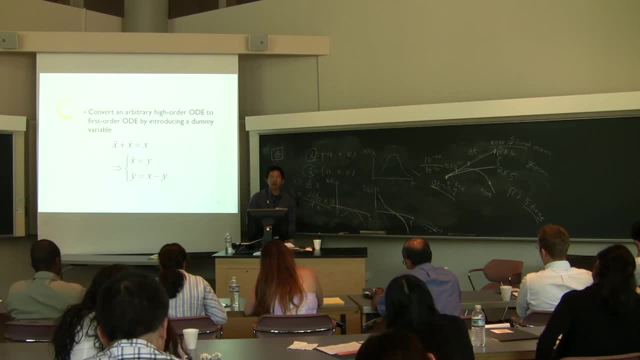 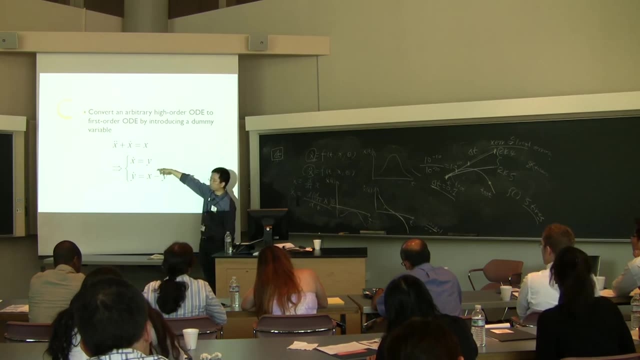 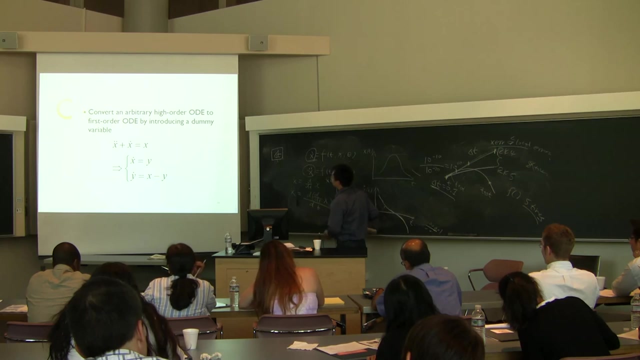 So this will be slope over slope, okay, So the so-called higher order, ODE, okay, is just that kind of thing. okay, Slope over slope, plus the slope is equal to the x, And we actually didn't bother to talk about. 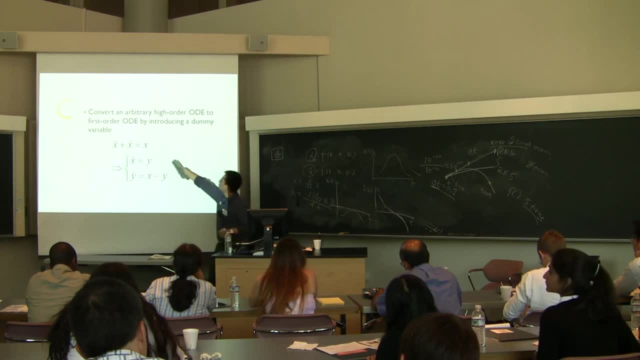 this kind of models, because all this kind of higher order ODEs can be converted to first order ODE okay. That's why people don't bother to develop a specific method for the higher order ODEs, okay. So how we do that? 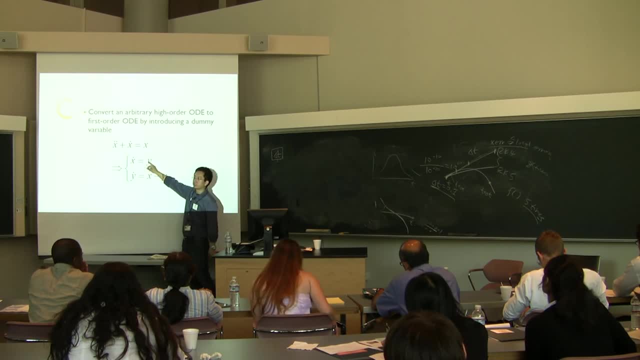 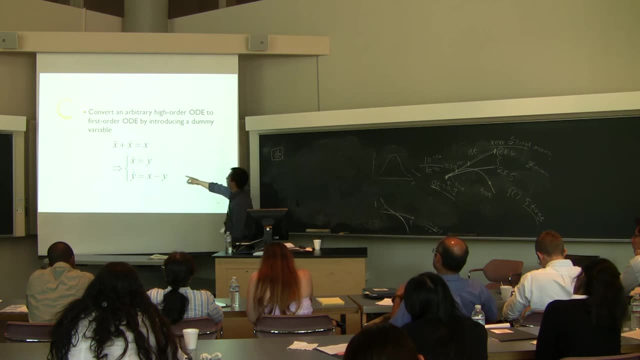 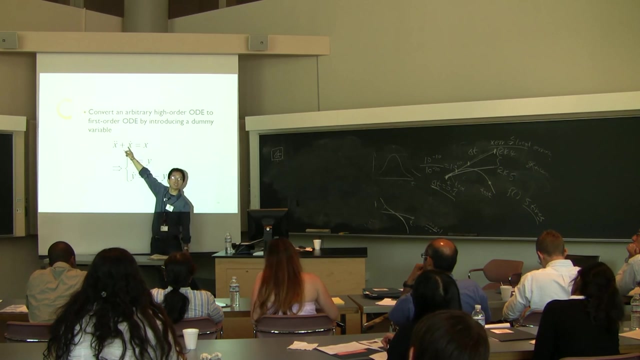 The idea actually is simple. We just introduce a dummy variable. okay, Y here is called a dummy variable, okay. So now y is equal to the slope. Then I plug this dummy variable into the original equation. Then the double dot becomes y dot, right. 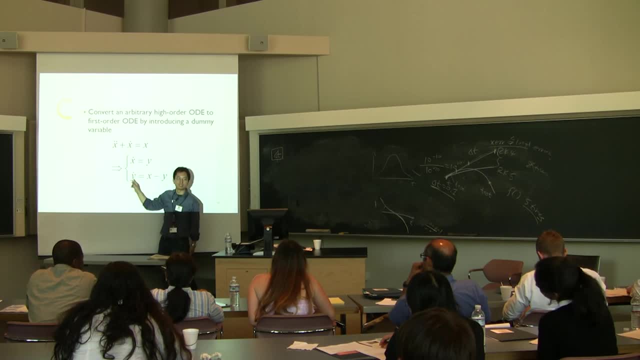 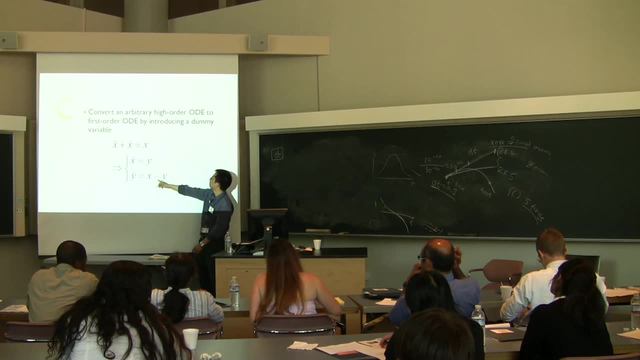 Because y dot is equal to x dot. So you put a dot on another dot On top of another dot, you get x dot. So this y dot, I can use this one, okay. So I do the same thing because y is equal to x dot. 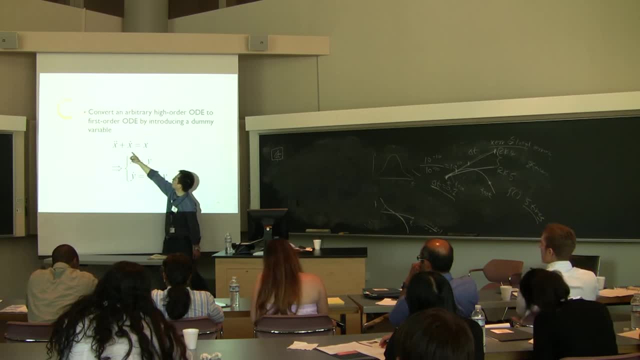 I replace this one with y, Then you plug this one into the original equation, okay, So eventually I get y dot x to x minus y. okay, Now we go back to first order. ODE again. right, That's what it is okay. 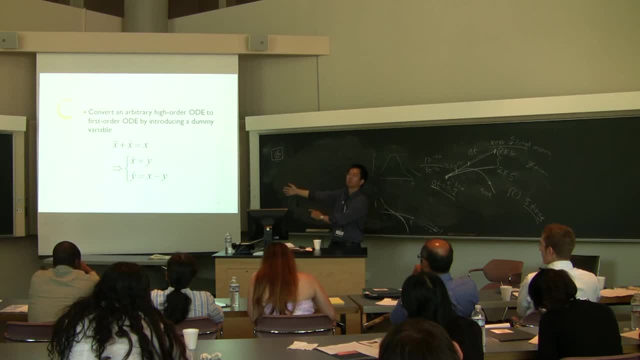 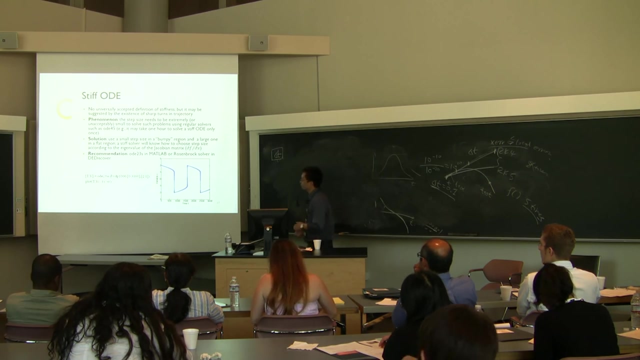 So now all the algorithms we talked before can be applied to this equation. So that sounds great, right? So you develop one set of things and deal with much more problems you expected originally. So okay, Okay, that's good. So now let's relax a little bit, okay. 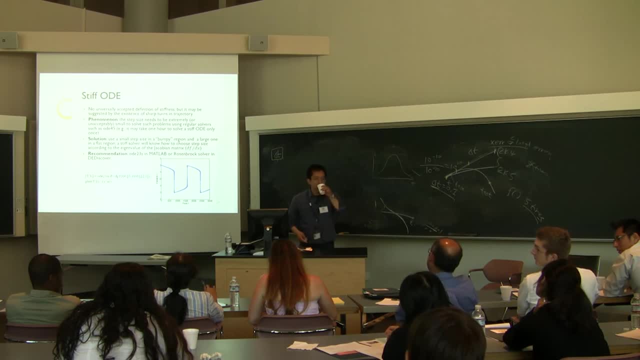 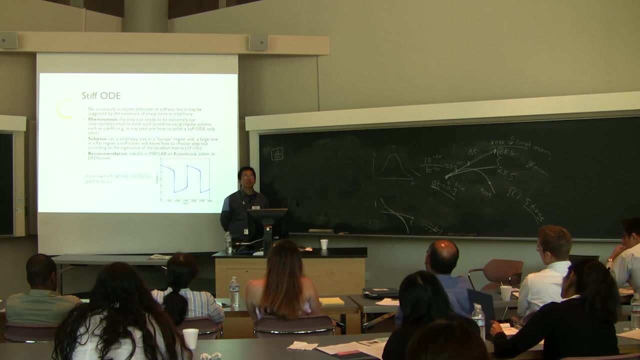 So Can you give us an example of where you would be doing a second order diffusion equation in a biological sense? Yep, Actually, if you're looking at the, for example, the diffusion problem, okay, Let's just talk about the one dimensional, okay. 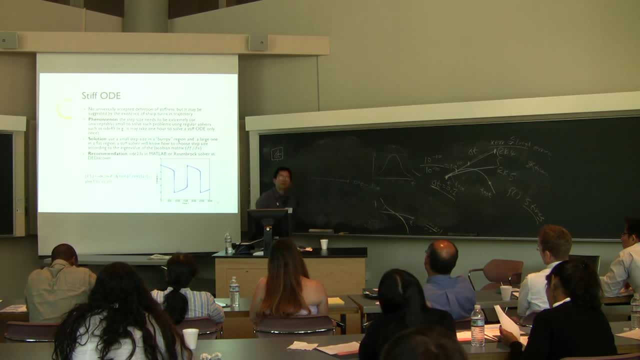 Diffusion problem. okay, The molecule, for example. I have a number of molecules. okay, I want to understand how they were diffused along this direction. okay. So the concentration: let's use x to denote the concentration. Yeah, let's use x to denote concentration. 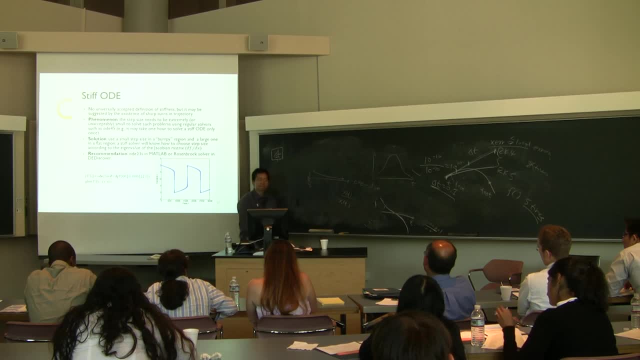 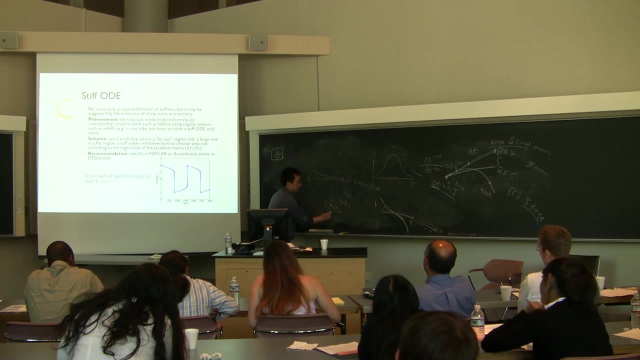 Then the first order derivative will be: what Will be the difference of concentration? The gradient spatial gradient right, And the force that pushed these molecules to move actually is proportional to this one. okay, The gradient of the gradient or the slope of the slope? 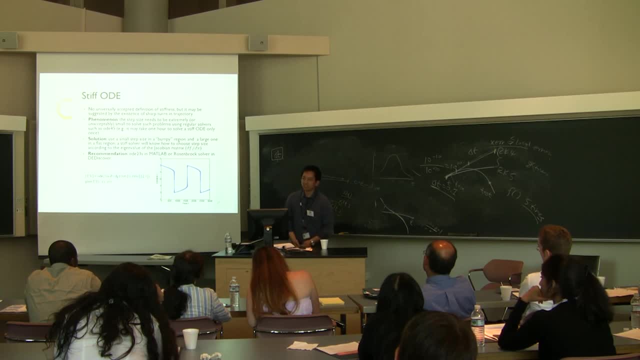 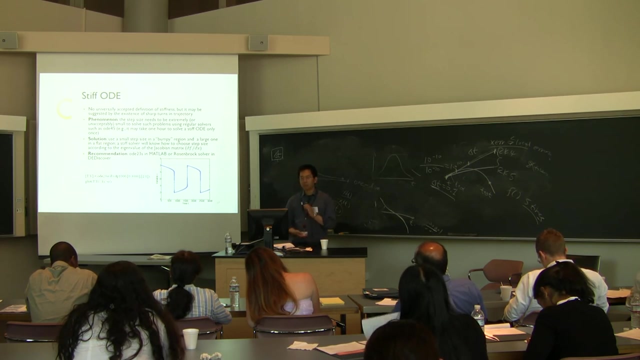 So that's one example, okay, But if you are just doing, you know, setter or lower dynamics, I don't think you have that many chance to actually run into this problem, okay, So now let's relax a little bit, because we have talked about lots of you know. 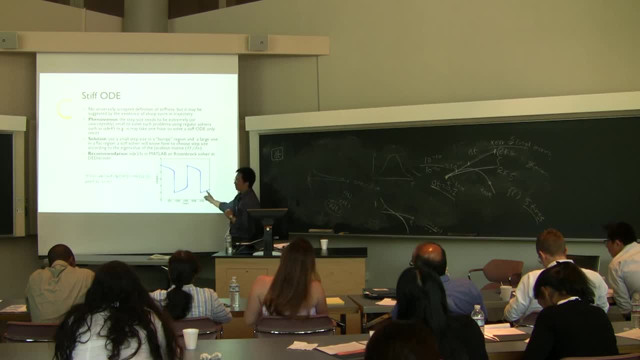 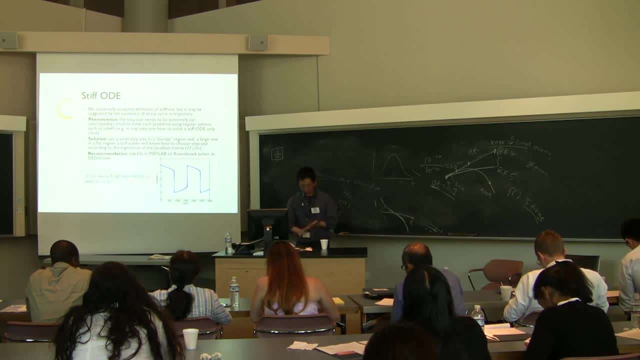 the 마지막 symbols. So there's another set of ODEs. okay, They're called stiff ODE. okay, Unfortunately, there's no rigorous definition for stiffness. okay, Although we call it a stiff ODE, okay. 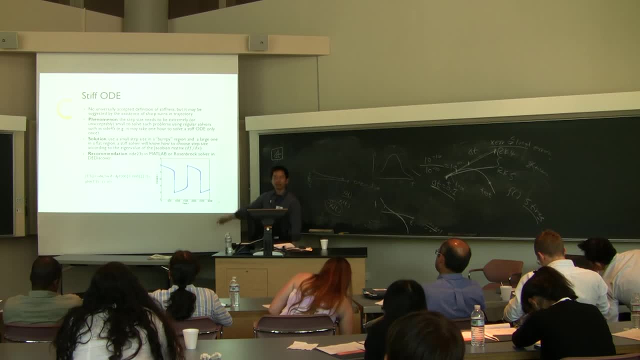 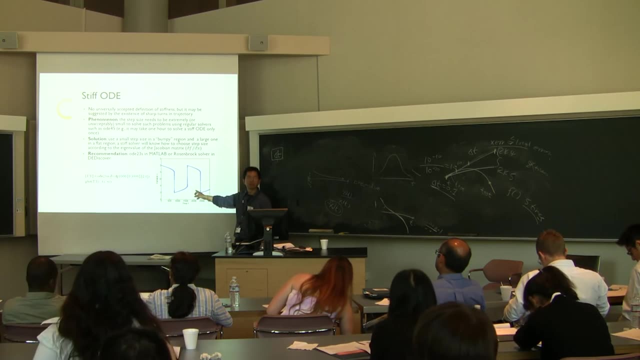 However, by looking at the trajectory you can actually tell the whether there's a high likelihood that the stiffness will occur. So usually, okay, the stiffness will occur if you see a trajectory that has a sharp turn, a sharp corner. okay, like this: 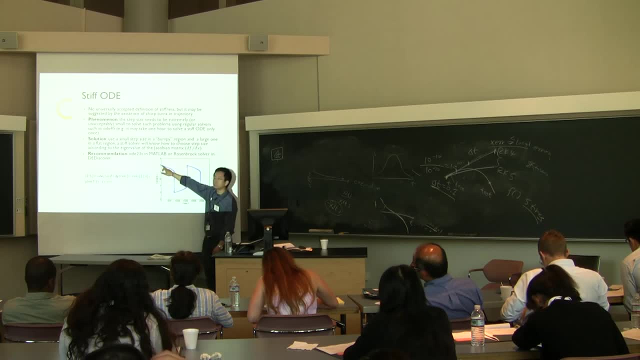 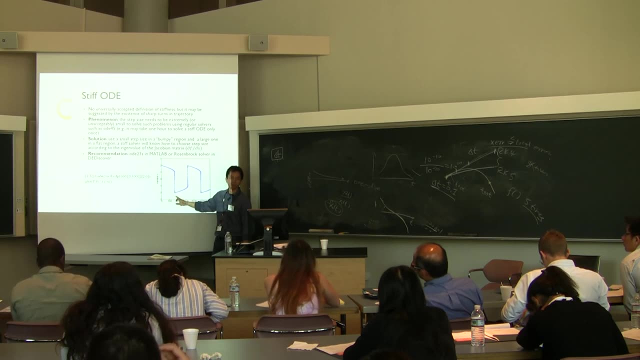 Like this: Okay. so basically this curve has a comparatively flat region, followed by a sharp turn, a jump, okay, then a flat region and then followed by a sharp turn- okay. So what's the big issue about this kind of thing? 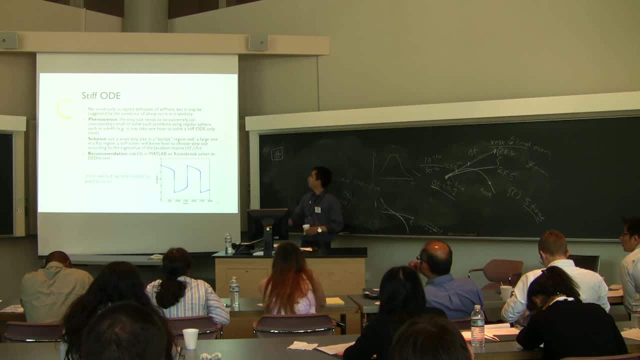 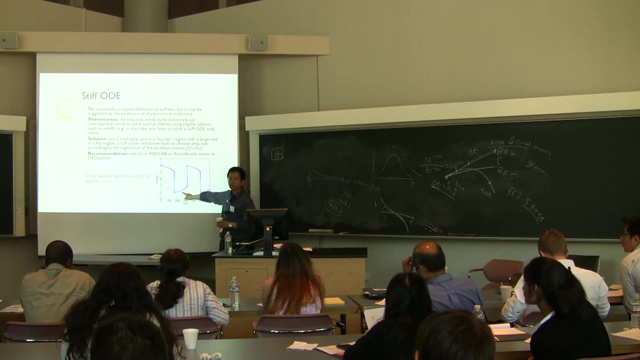 this kind of model. The problem is that we have been talking about how to solve the ODE- okay, but if you have a stiff ODE, okay, the solvers I just mentioned, okay, will not work. Will not work means for this kind of simple system. 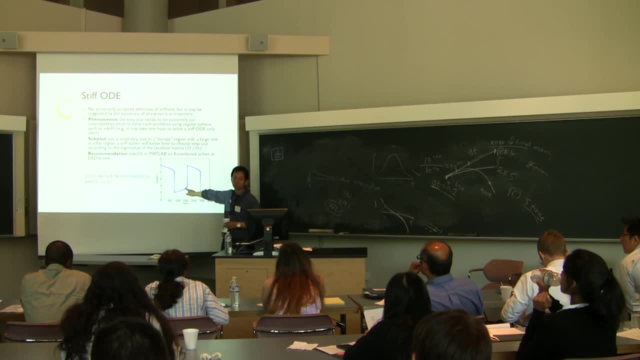 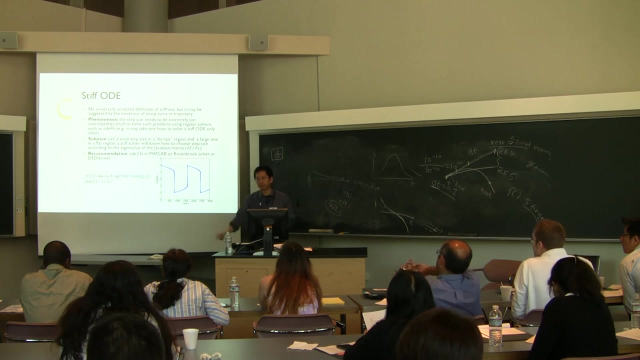 actually, this is produced by a two-equation system. okay, just two equations. So you probably need to spend like eight hours to just solve it once if you use the two solvers I mentioned before. It's not acceptable. okay, for a small system like that. 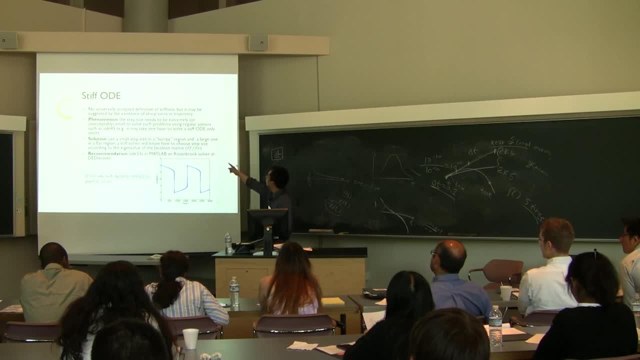 You want to spend eight hours to solve it. So the problem is: remember, when we talk about the step size, we said the solver will automatically determine the step size. Okay, such that in a flat region I will use a bigger step size. 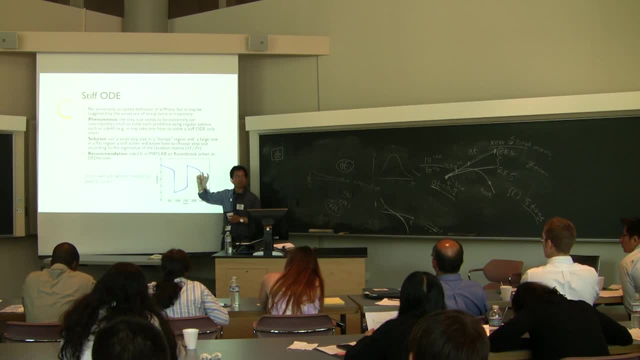 In a smaller in this steep region. I'm gonna use a smaller step size, right? However, because the regular solver okay when they try to do this. okay, around this corner, this density will becomes extremely small, okay. 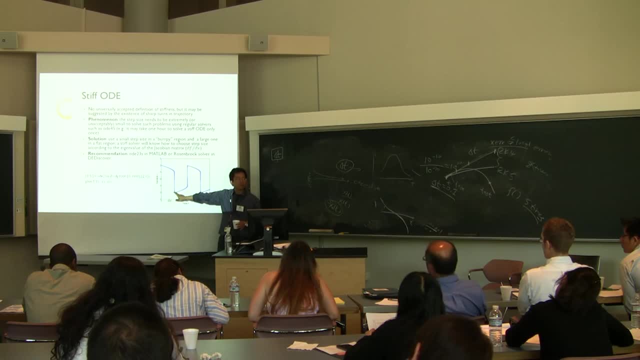 So such that you have to solve this, evaluate the f function, okay, millions of times And eventually, actually, you're gonna just fail. okay, What if you just stuck there? Because you keep reducing the delta t, keep reducing the delta t and then you have to. 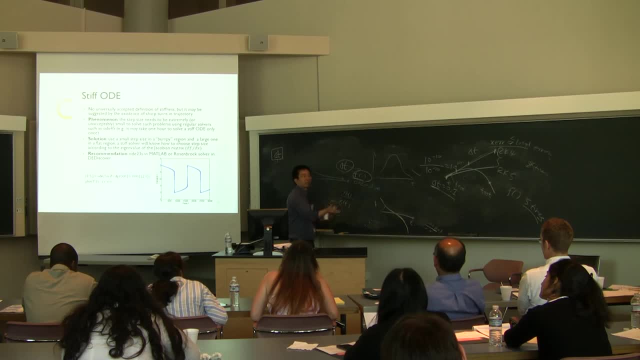 keep evaluating this function, So it will stuck there, You will not move Because the local error- okay, cannot satisfy the criterion we just mentioned. okay, So even if the solver keep reduce the delta t, okay, this one still cannot be satisfied. 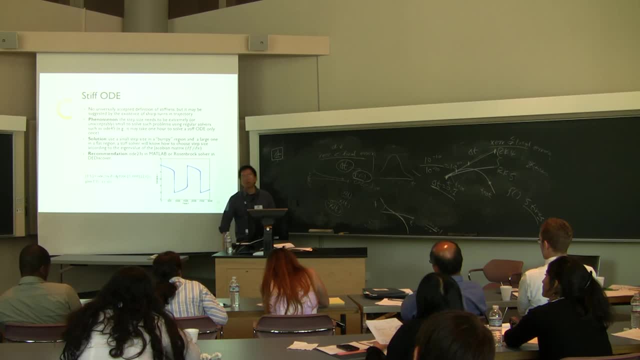 That's why the solver cannot move from one point to the next point. So that's why, actually, people have to use the so-called steep solver. okay, We have a category of solvers that are designed to deal with this kind of a steep problem. 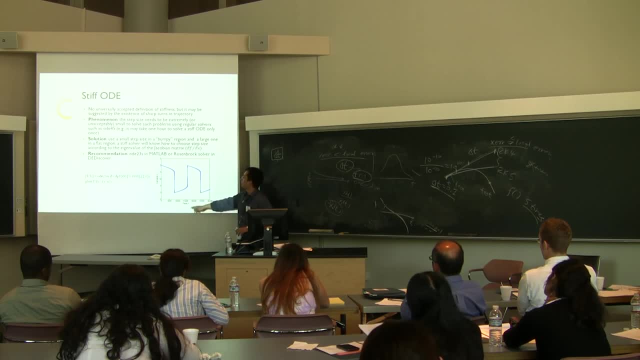 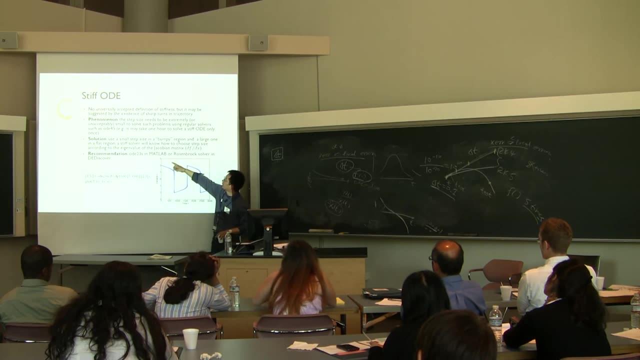 Okay, It's called a steep solver, Mathematically okay. how this solver deal with this kind of problem is by actually by calculating the eigenvalue of the Jacobian matrix. but who cares about the Jacobian matrix? for now, okay. 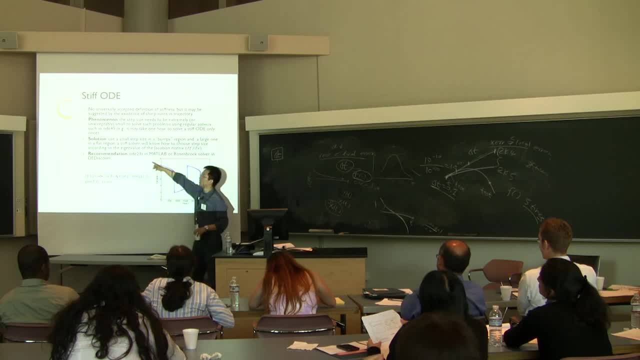 So we just know that it's gonna work if you use a specific solver, okay for this kind of problem. So if you use MATLAB ODE23S, that would be the one you want to try, Or you can use our package, okay. 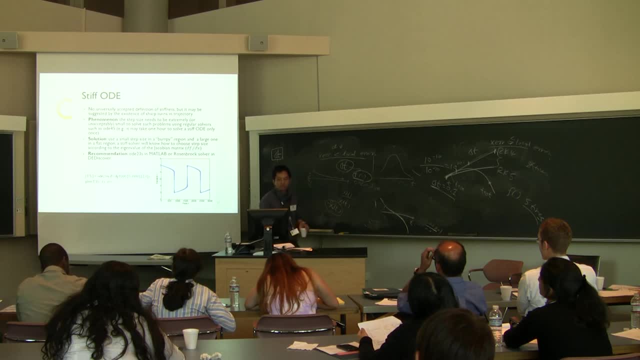 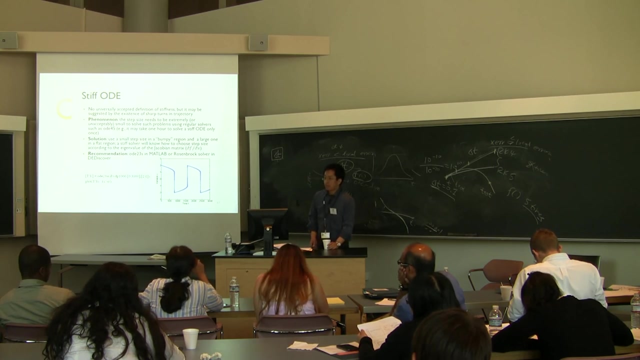 We have a Rosenblatt solver in the D-Discover And if you're a MATLAB user, you just need two lines of code. okay, to solve a steep equation and do this part. Okay, Yeah, there are many other alternatives. 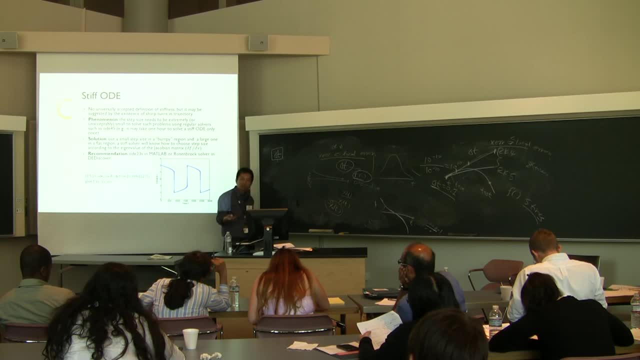 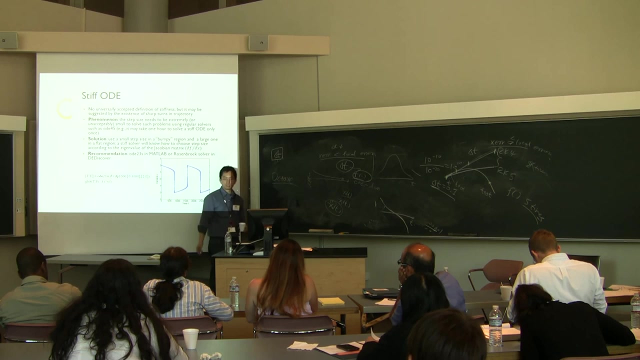 If you're familiar with the grammar of MATLAB, there is a free alternative called you know the Matlab. It's an alternative called Octave. okay, It uses the MATLAB language, but this one is free And many of our statisticians actually. on Wednesday, 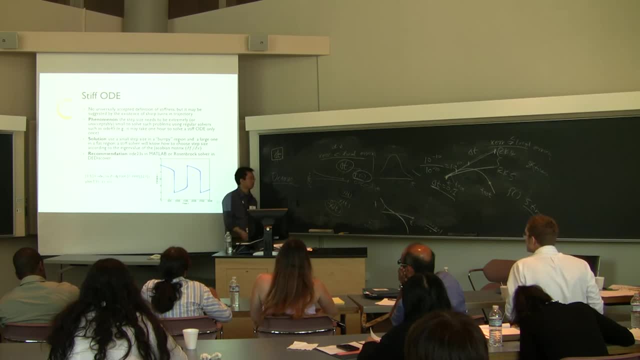 or yeah, Wednesday they're gonna talk about lots of you know data analysis thing. They use R. R also can solve. It's free. yeah, R can also solve it And there are many- I think tons- of packages actually can. 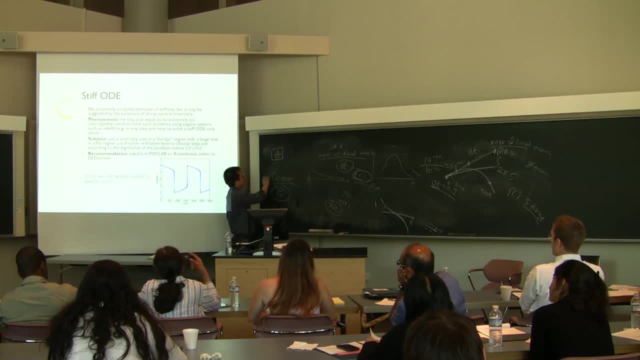 We use MATLAB, but it's a license. Oh, this one. Then. if you are familiar with MATLAB, then this one you can try. Octave, Oh, this one is free. okay, You mean the stiff, stiff solver. 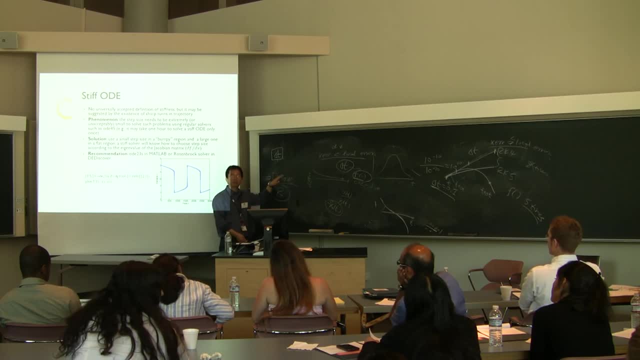 Oh yeah, It has. that has the order you know you, your solver, you need, okay, So you don't need to worry about actually the completeness, okay. Question: The main problem is you have several y values. 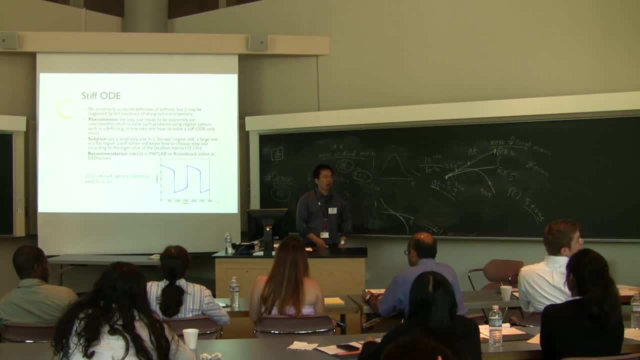 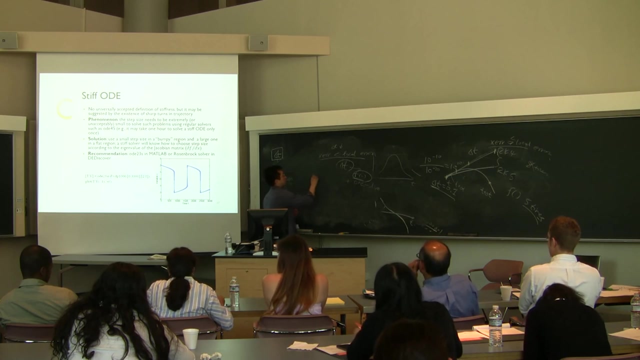 for particular x values. Is that why it takes so long to solve it? No, No, Remember we for now. okay, we only talk. we. I actually used one dimensional problem to illustrate the idea. okay, I just talk about x, dot, x, two f, t, x, theta, okay. 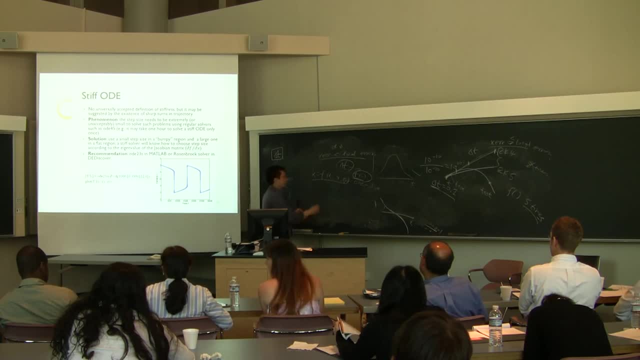 However, the model we used in practice usually is not one dimensional. okay, If you only have x one x two, f one, t, x one x, two x three theta, for example, it's a three-dimensional system. 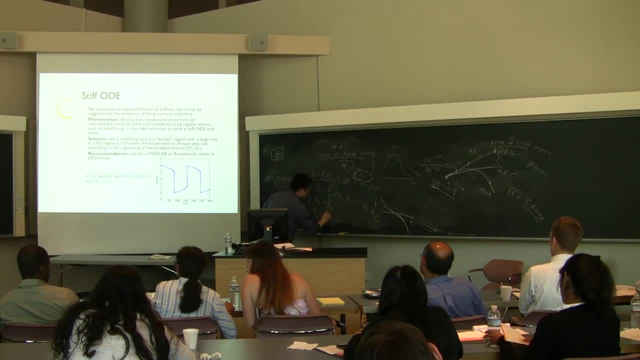 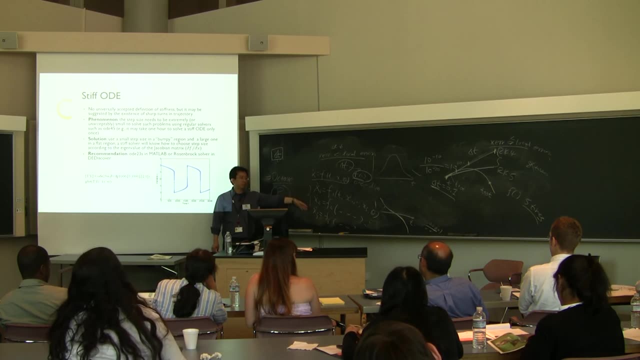 I have x2,, x3,, f2, and f3, okay. Usually you will have this kind of system- multi-dimensional okay system. So it doesn't mean okay if I will spend more time to solve it because I have more variable, okay. 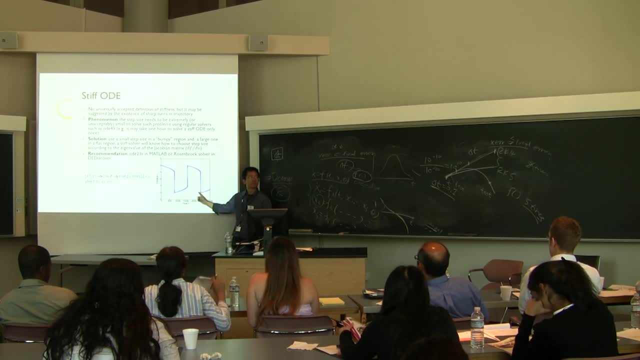 The problem is that if just one of the variable has this sharp turning corner, okay, it will cause a problem. okay, Even if, for example, if the plot of this one looks like this, but this part may look like this: okay, 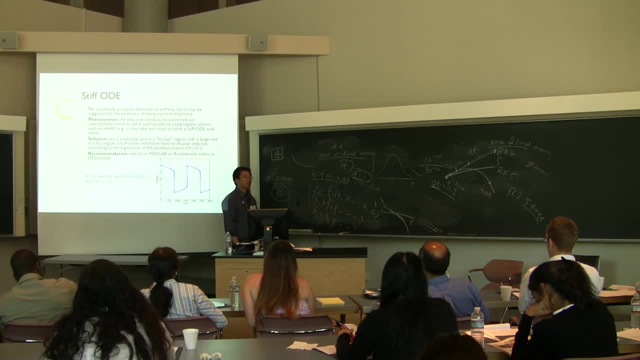 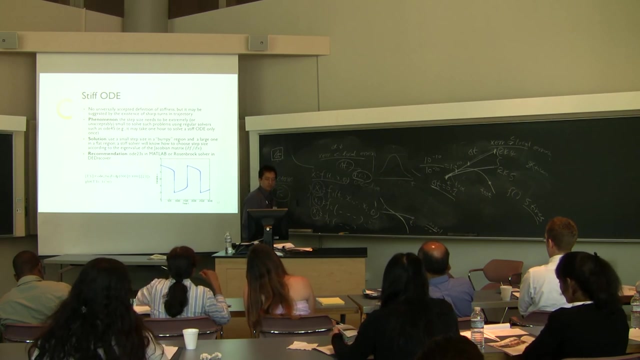 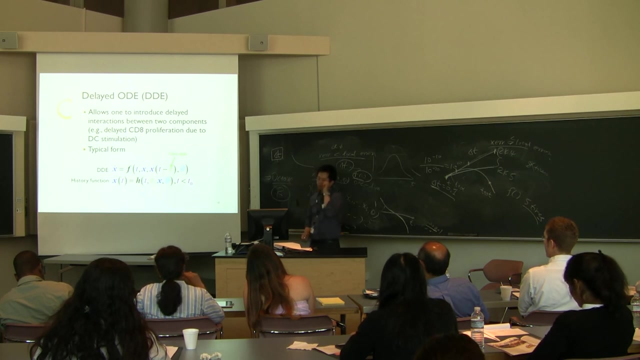 It can be flied sort of. So different variables, they can have very different trajectories, And you can put them together, solve them, okay, Is that clear? Okay? So now let's talk about another category of the ODEs. okay, 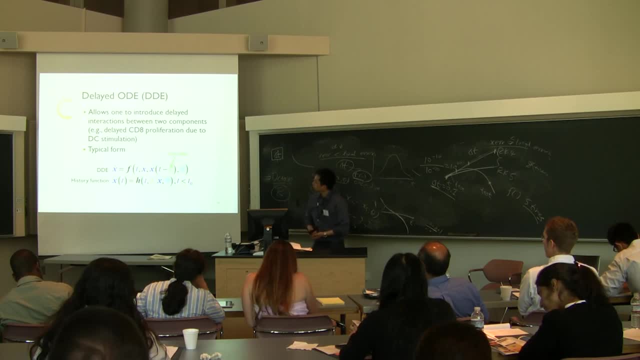 It's actually a variation of an ODE. It's called a delayed ODE. So we have been talking about ODEs, okay, general ODEs. So the problem is, sometimes you need to consider the delay effect. For example, we know that dendritic cells stimulate the CD8 T cells. okay for their delay effect. So we know that dendritic cells stimulate the CD8 T cells. okay for their delay effect. So we know that dendritic cells stimulate the CD8 T cells okay. 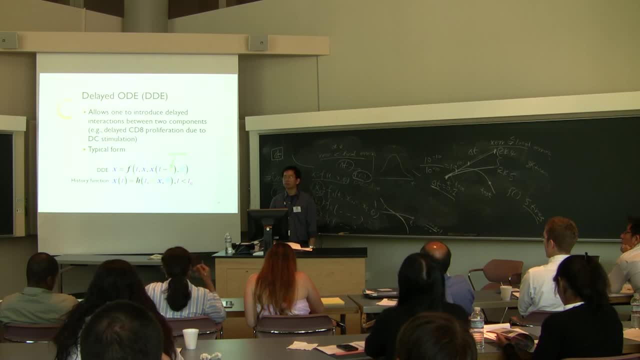 for their delay effect. So we know that dendritic cells stimulate the CD8 T cells also of 1.5 days after the infection. However, the appearance of CD8 virus-specific CD8 T cells is only after day five. Right now I'm talking about influenza virus. 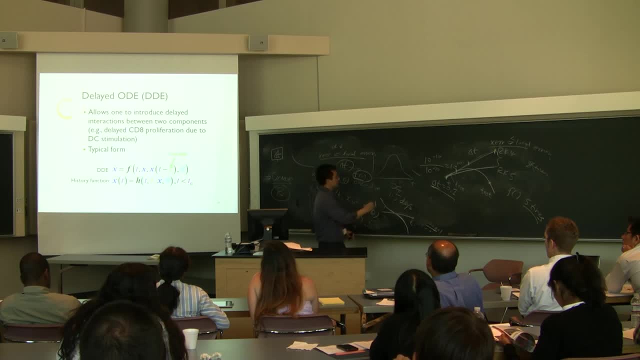 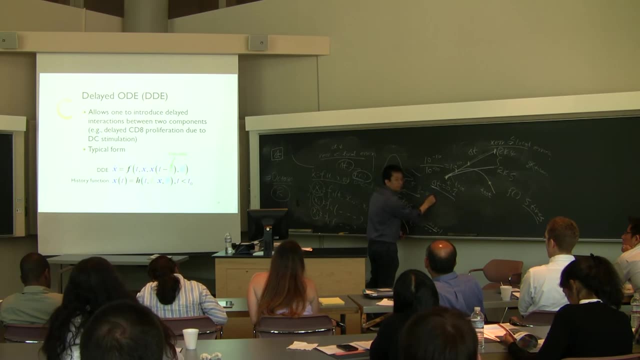 for different reasons, whereas the number could be different. So from the stimulation to the affinity maturation, there's actually a three to four days delay. So if you want to account for that kind of delay in your model, that's the timing. 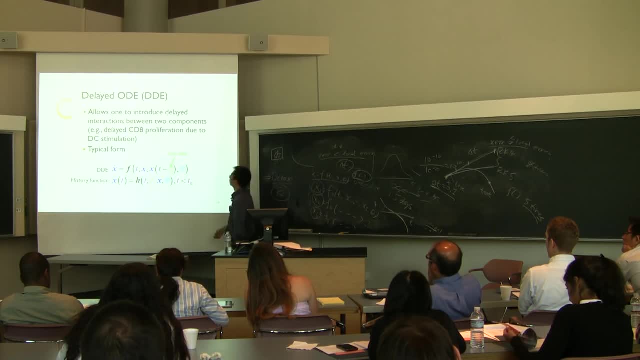 You should use a delayed ODE called DDE. So the difference between the ODE and the DDE is that right now you have a delay term- okay, Tau, here is time, delay, okay. So the problem is that once you want to use the DDE, 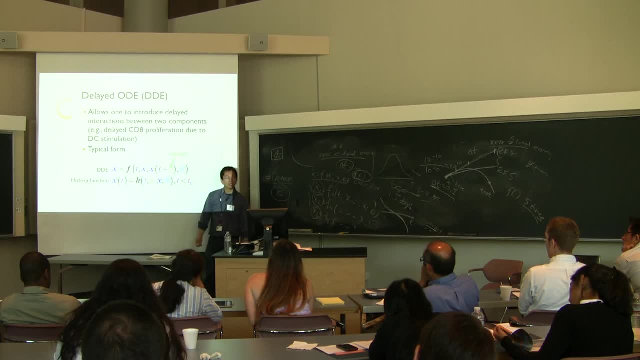 you have to specify the so-called history function. Remember, if I don't have this term, then the left-hand side is x, dot, t. that's the value or derivative at time t, and the right-hand side, we also have the value. 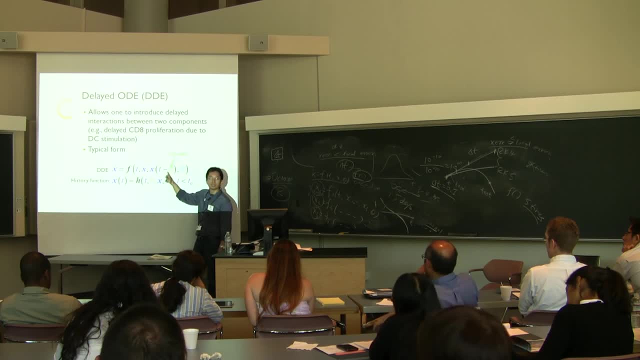 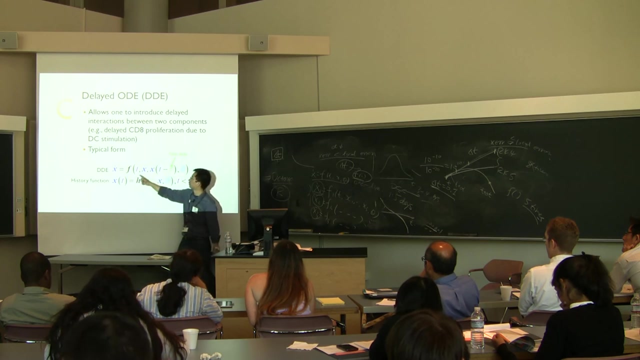 at time t, right. But once you introduce the delay, now the value of x at time t also depends on the value of x at history, right? Or the historical value. You have to plug in a historical value to calculate the current value. 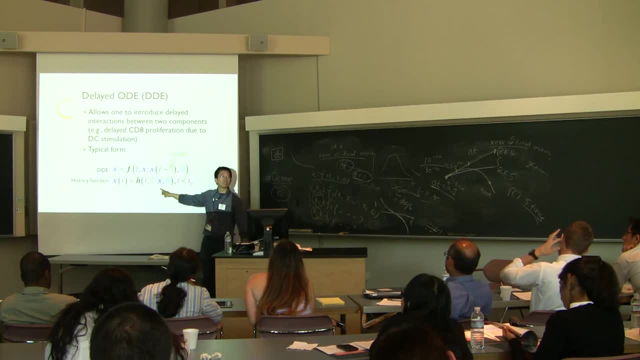 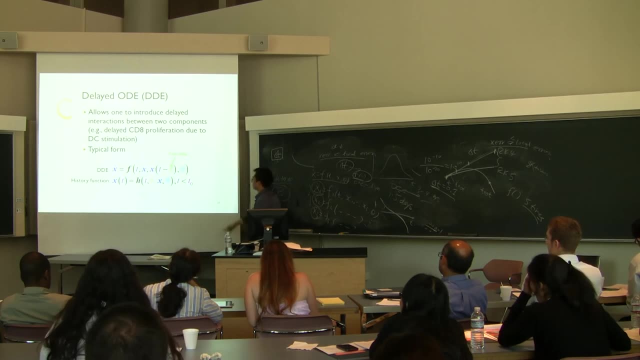 So that's why you need to also specify your so-called history function. okay, If you don't have this one, then you are totally wrong. okay, I have to say that. So if you don't specify the history function before the 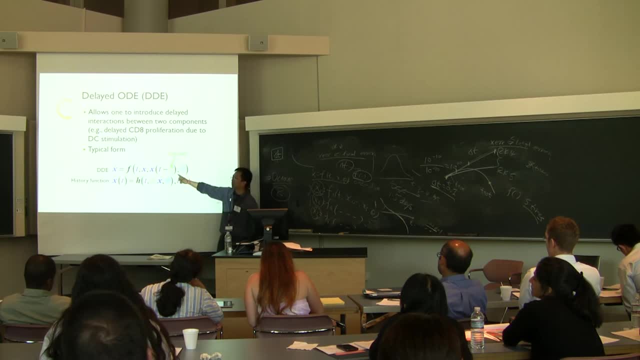 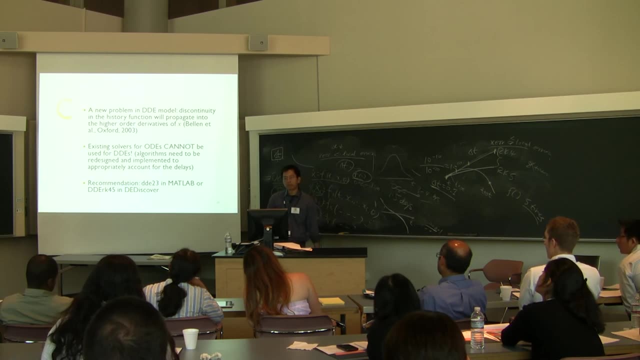 for the initial time point. okay, then you will get this wrong. That's one thing we need to pay attention. Another thing is that a new problem associated with DDE is that the discontinuity in the history function will be propagated into the higher order derivatives of x. 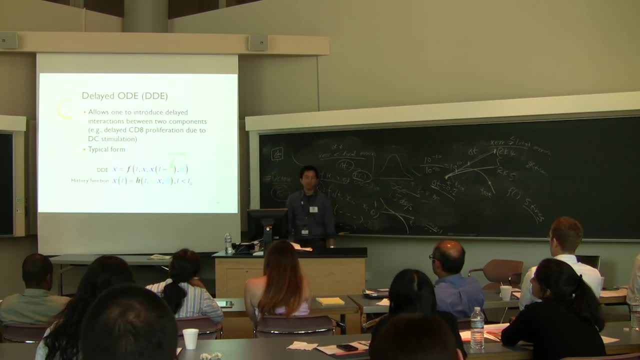 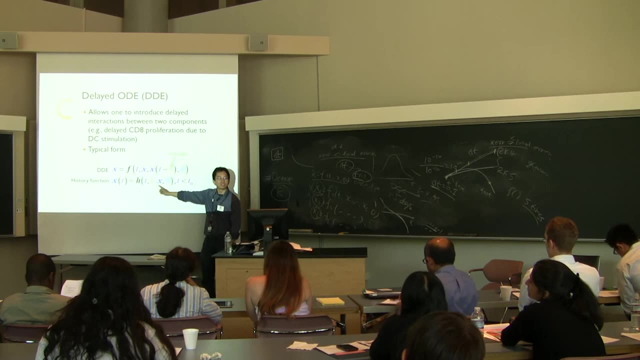 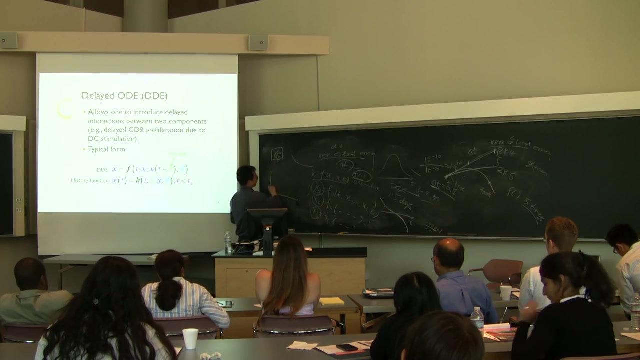 So I bet that you don't understand what I'm talking about. So that's fine, because this one okay when you specify this function. okay, OK, this function can be a continuous curve. OK, up to t0,. 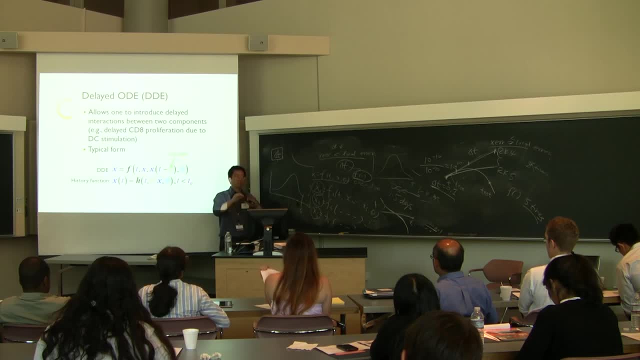 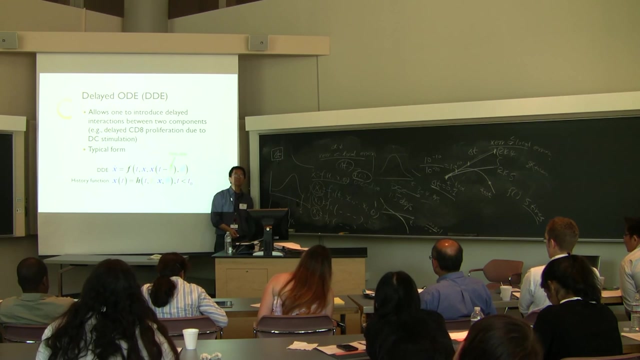 right, But sometimes people also use discontinuous curve trajectory. For example, I may have a history function like this: So I have a jump here And here is my t0.. So you have a jump here. OK, can everybody see it? 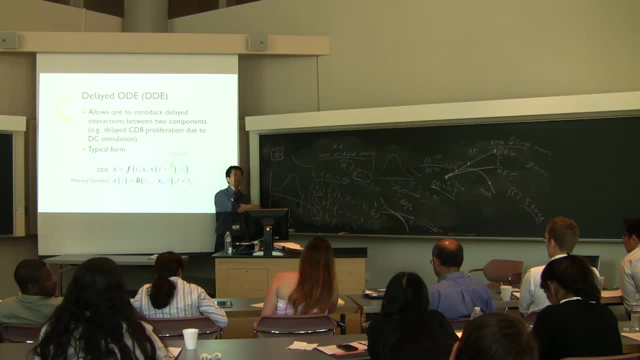 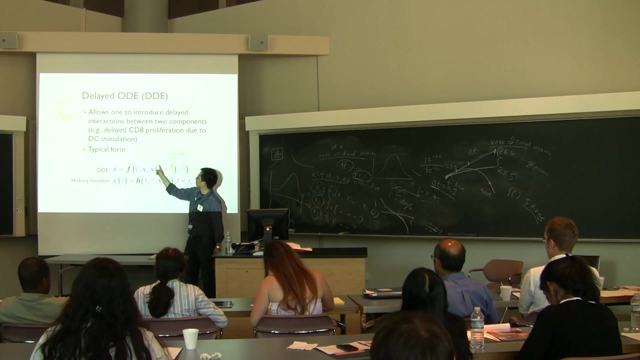 Or I just happen to draw behind the computer. But anyway, once you have this jump, OK, this jump will propagate into the derivative. So actually, just look at the equation. OK, If I have a jump in H, so the H will go to this part, right? 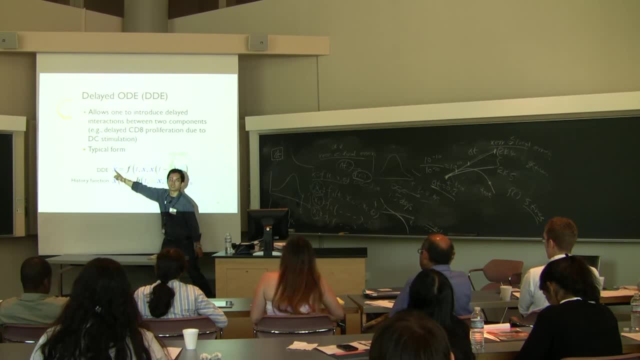 And then the jump will go to here, Because your equation says the derivative depends on this jump. That's what I mean. OK, so why does this jump matter? Because it will change your solution. So either you use a continuous, OK. 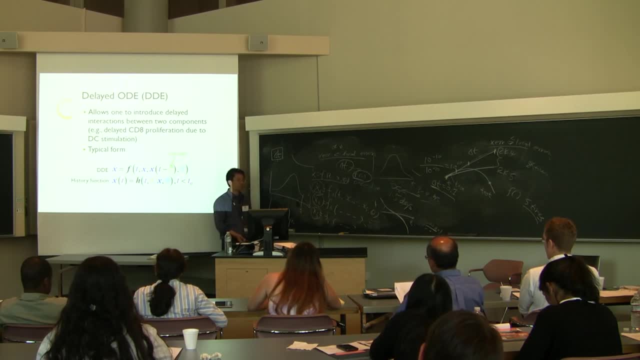 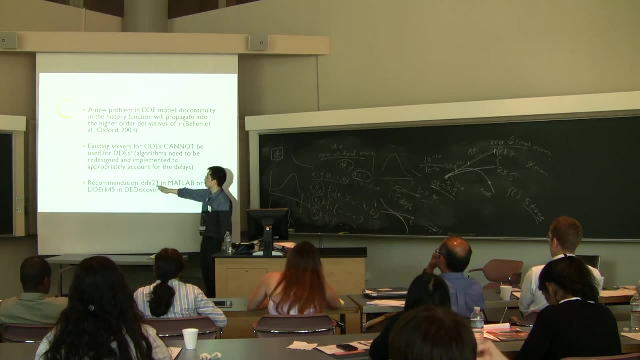 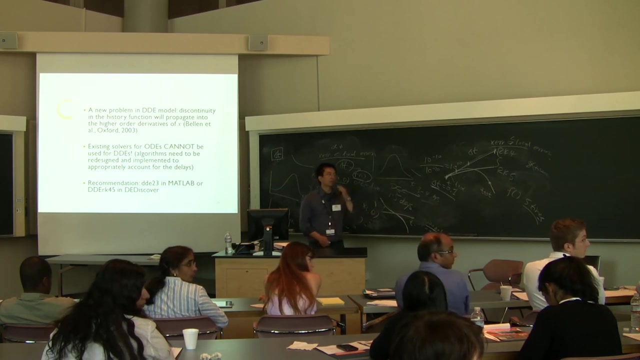 either you use a continuous history function, but if you do have a jump in your history function then you have to use a particular solver. OK for this kind of problem. So in this case the function is not variable in all the time domain. 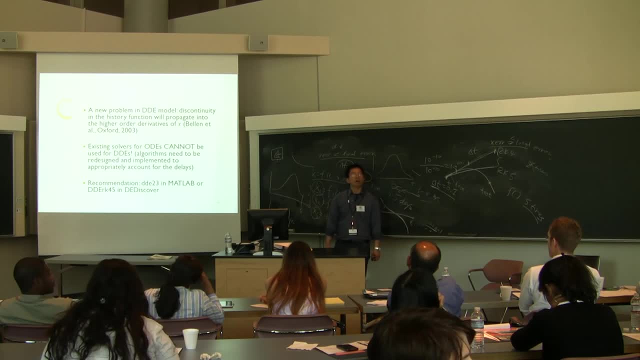 I mean there is a discontinuity. If there is a discontinuity in the history function, you still solve this forward. OK, So I'm not saying that it becomes some other type of problem. It's still a forward problem. The problem is you need to pay attention to that. 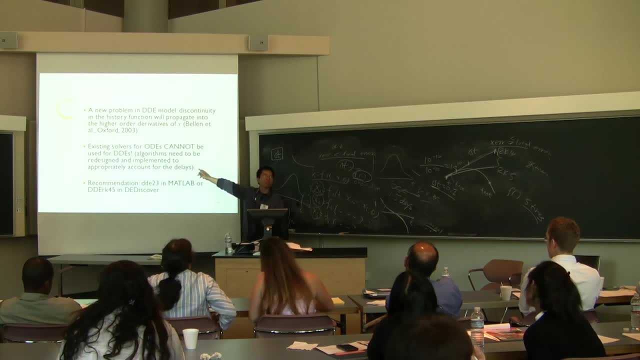 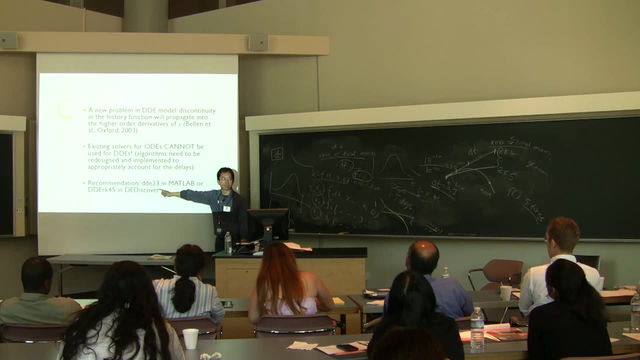 OK, OK, OK, OK, Because if you use the solvers I mentioned before, then we again get a wrong answer. The point is that use the particular solver, OK for this type of particular problem. OK, then you get away from trouble, OK. 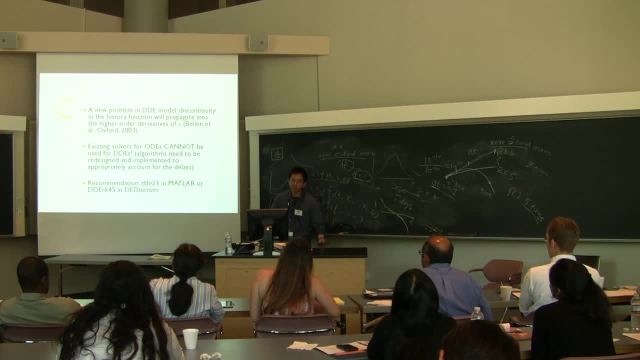 Otherwise you again probably will get a wrong trajectory. So for now, OK, you probably is a little bit nervous, OK? So modeling is not as easy as what we talked about this morning, right? So there are many tricks, OK, and pitfalls, OK. 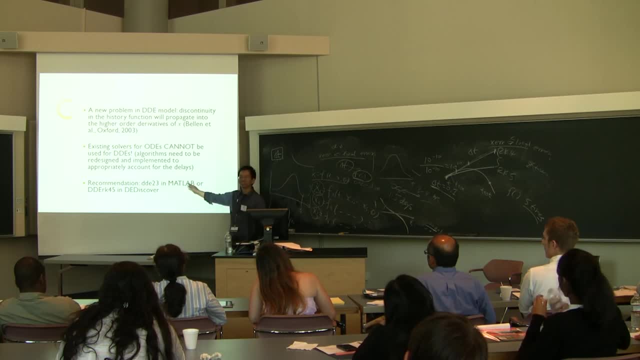 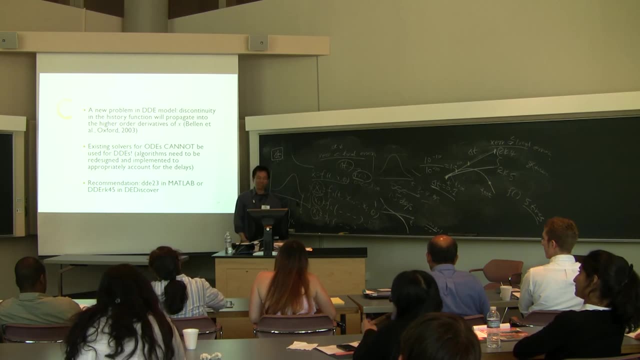 You have to actually to know OK before you use the models. OK, If you don't know OK the issues associated with each type of different problems, then you'll get yourself lots of trouble. OK, That's not actually rare, because when I was going to 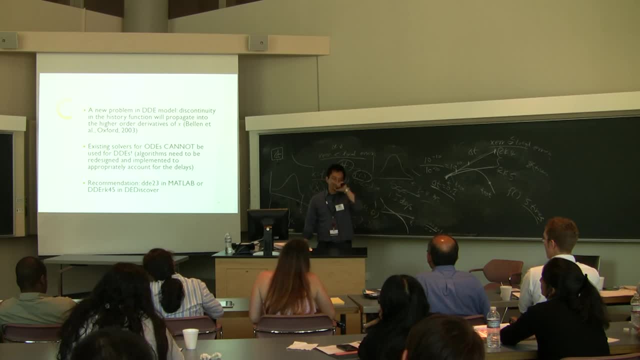 you know some other conferences. OK, I saw actually a simulation work did by some you know lives and they just made some assumptions that she eventually denied it to you know, decide, not to you know, argue with me. 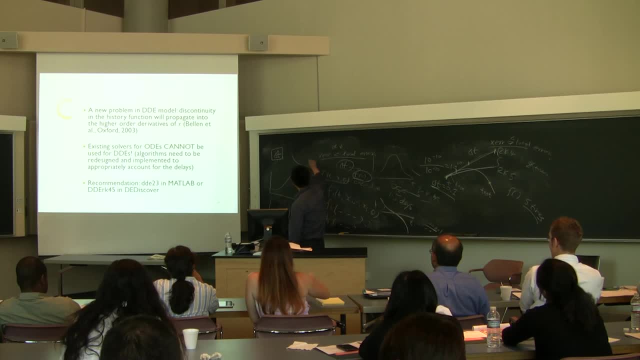 So, because she was looking at the fish population and she made an assumption that there was an infinite number of fish at the boundary, I said: how could that be? It's possible, OK. So again, OK, that's a particular issue, OK, associated with a particular problem. 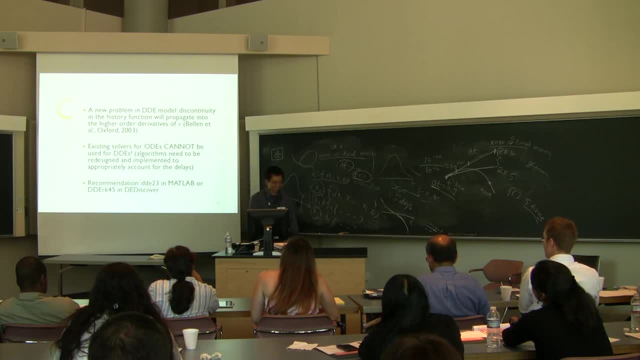 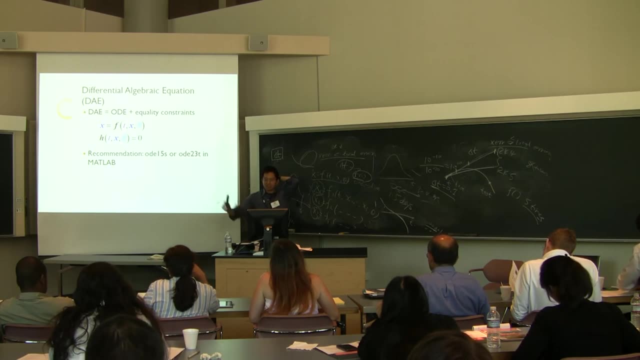 but you have to know that, OK, beforehand. But anyway, the last variation of ODEs is actually the so-called differential algebra equation. OK, DAE. So the concept of DAE actually is simple. It's just the ODE plus some equality constraints, OK, 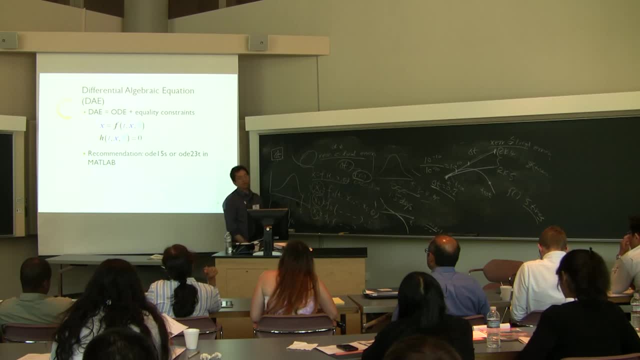 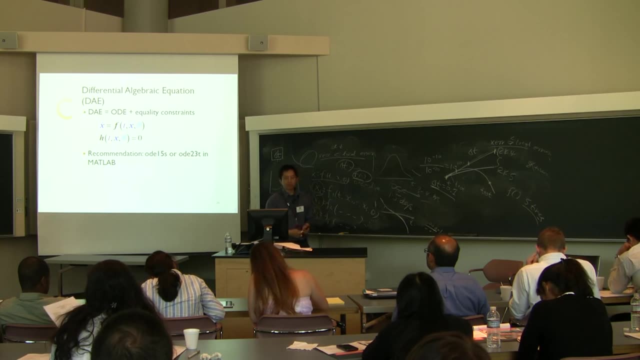 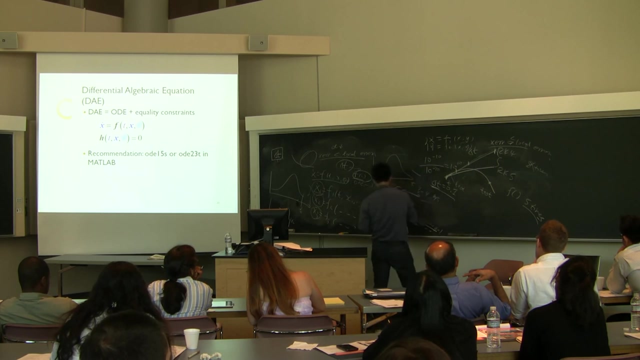 So these are constraints, OK, Although I use the same edge OK at many different places. OK, but here edge means the constraints. For example, if I have x dot x to something, y dot x to, Now, I want to solve this on a circle, OK. 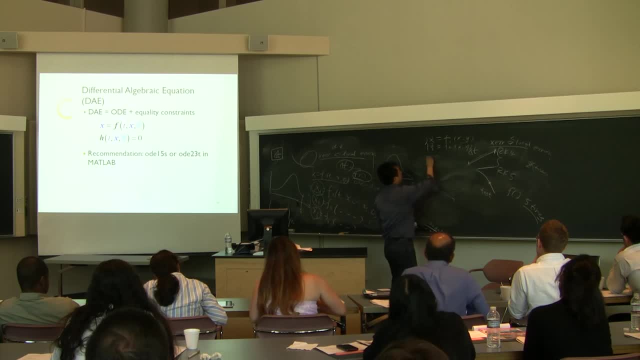 In fact, OK, The only interest in this. on a circle, I put a constraint like this: OK, This is a circle. OK, If you move it, it gives you right x to 0. And if you plot x, y, that will be this circle with a radius of 1.. 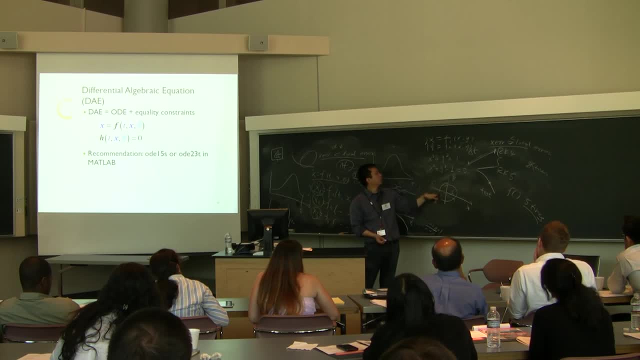 OK. So if I want to just solve this ODE on this circle, that's what we do. So sometimes you have a geometric constraint or whatever constraint. OK, That's how you handle this. Again, you have to use a particular solver. OK for this problem. 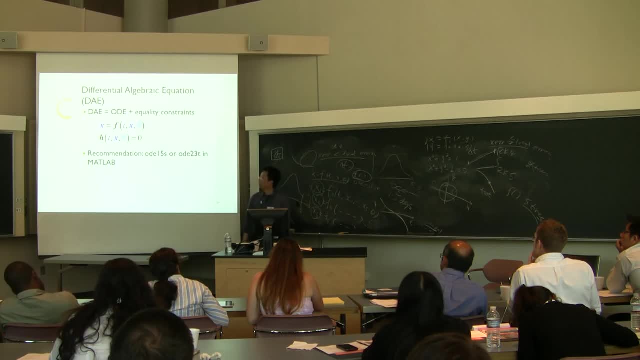 For example, in my lab you use the ODE 15S or ODE 23T. OK, That's the two solvers you can use to solve DAE. OK, Had enough of ODE. Yeah, I'm a little bit sick about it. 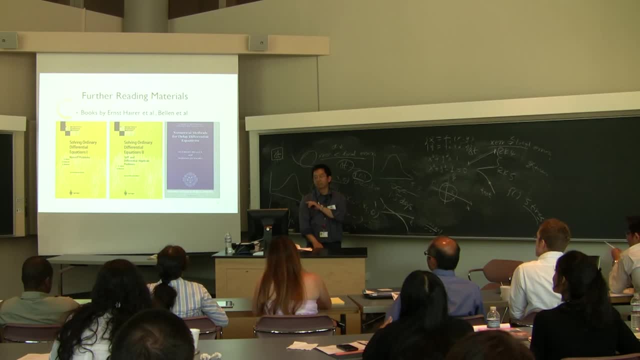 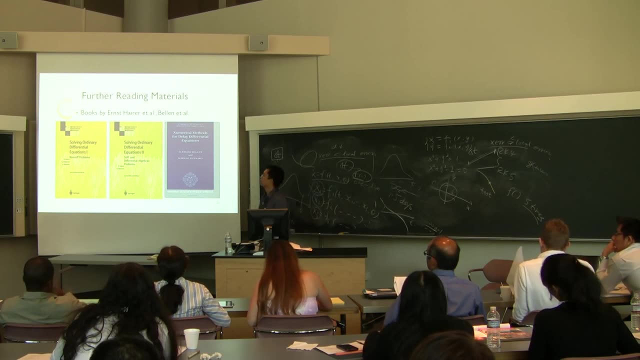 So let's Oh, last thing. Here actually are three books you can read If you're really interested in ODEs and DDEs, whatever DAEs, OK. So this is volume one. volume two: OK. 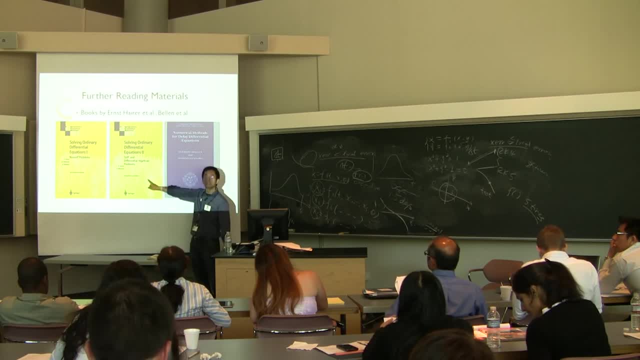 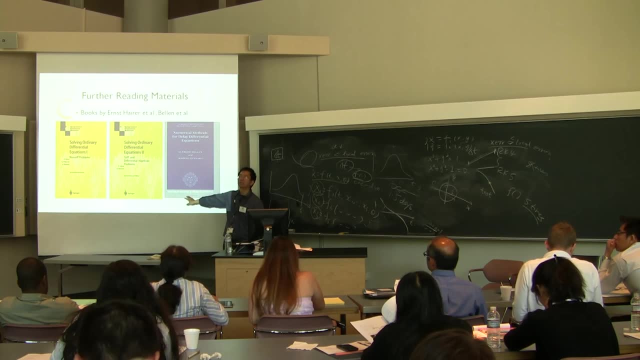 The first one is for the non-STEPH problem. The second one is for the STEPH and the DAE problem. OK, This one is about DDE. OK, Although I have to say this book is not perfect. OK, But that's probably the only book available right now. OK, 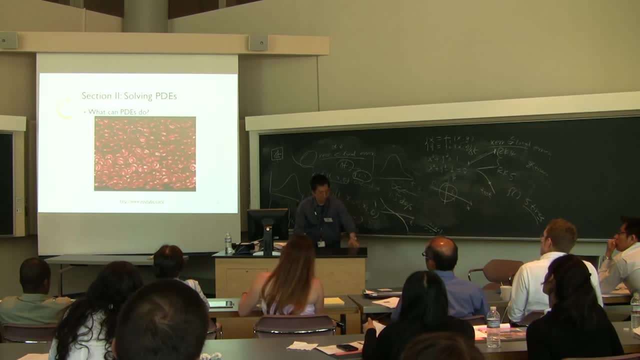 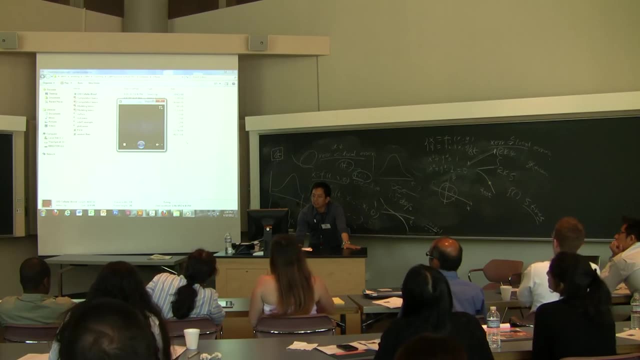 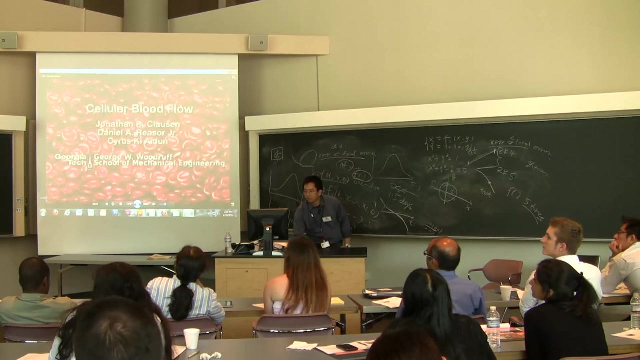 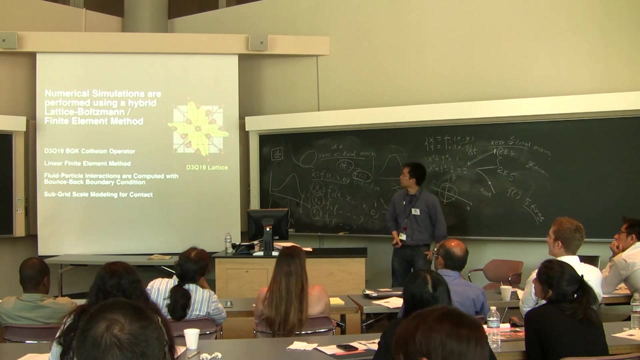 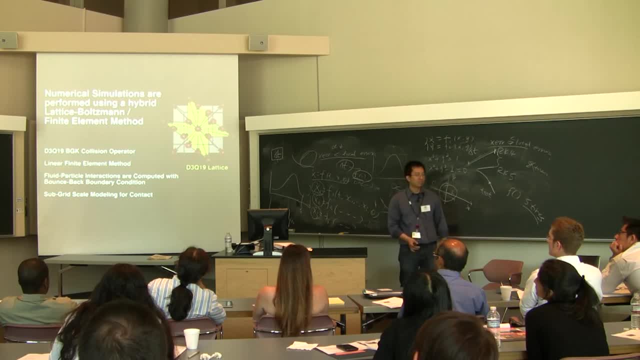 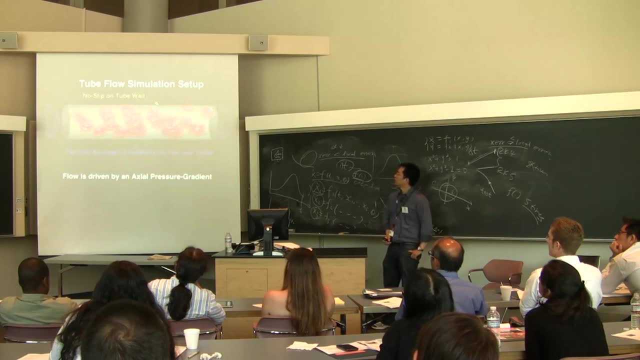 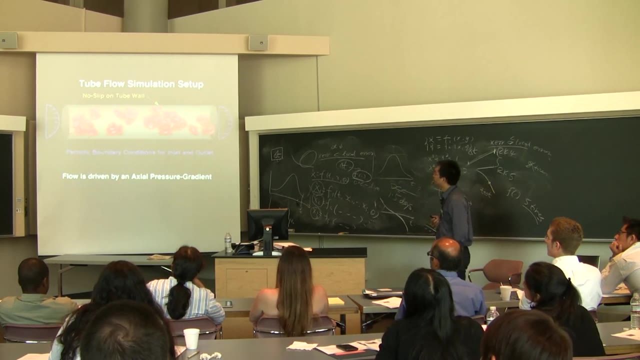 So you want to know what they're doing. OK, So this simulation is about the blood cell flow. OK, You actually solve some equations to get this simulation. Is that fun? Yeah, so now we try different parameters, okay, and we compared with what we know about. 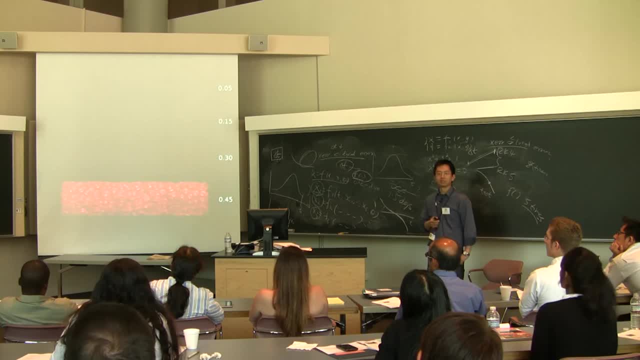 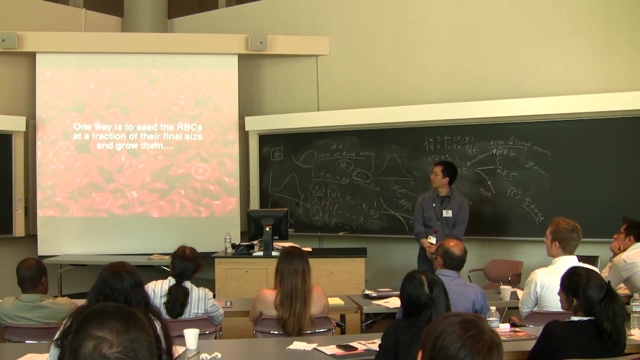 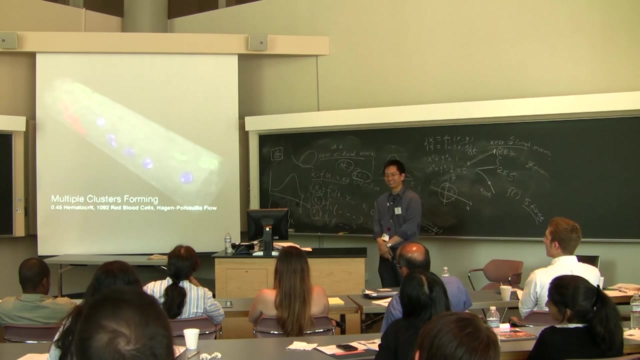 the cell flow and to tell which parameter is more really realistic. okay, so sometimes you know if you don't have music, uh video, just look senior. actually i think the original video actually comes with pretty cool music, but i sort of removed it. and here now we are looking at the clustering phenomenon. okay, in a cell flow. 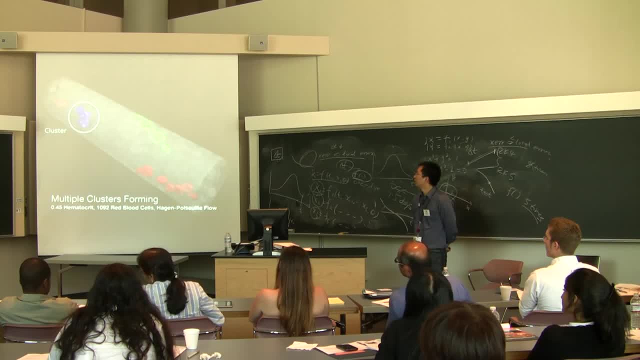 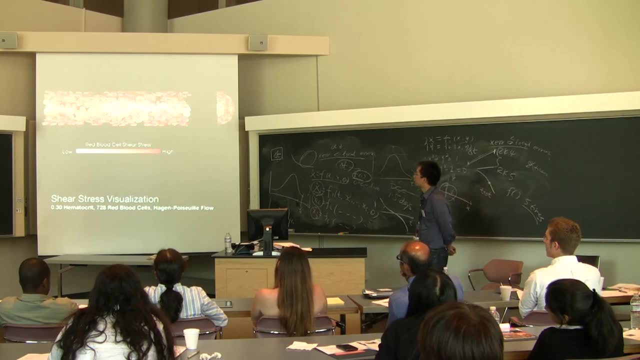 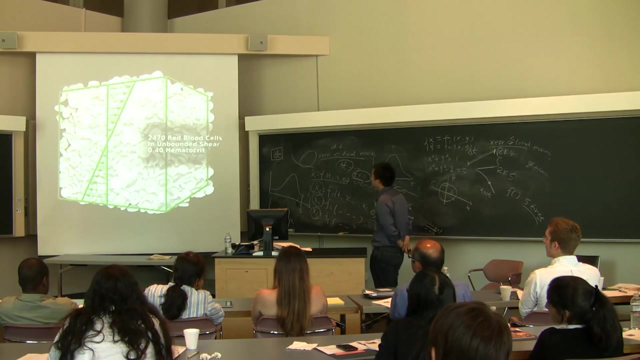 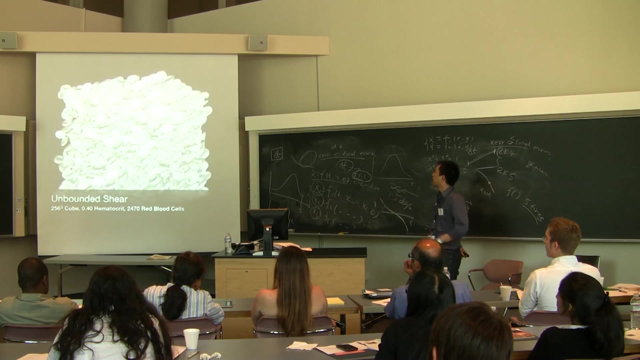 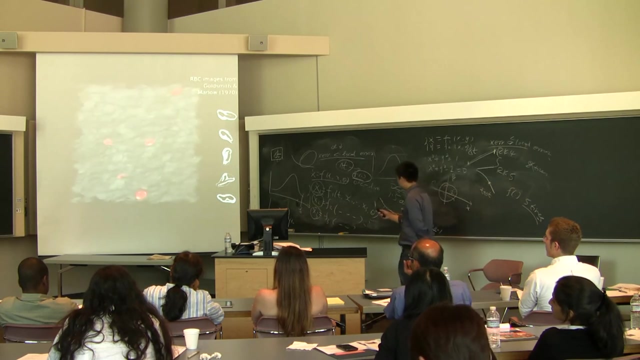 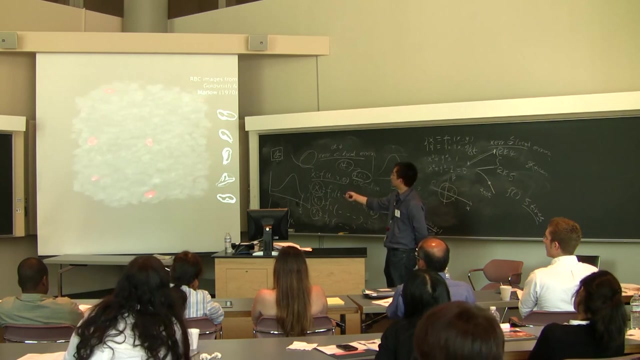 and then Now we're actually looking at the stress on the cell membrane. So red means there is a higher stress, red color- Now this is a shear stress And you see a bunch of deformed cell shape- cell shapes here. They're all the same type of blood cells, but these cells are deformed due to the shear. 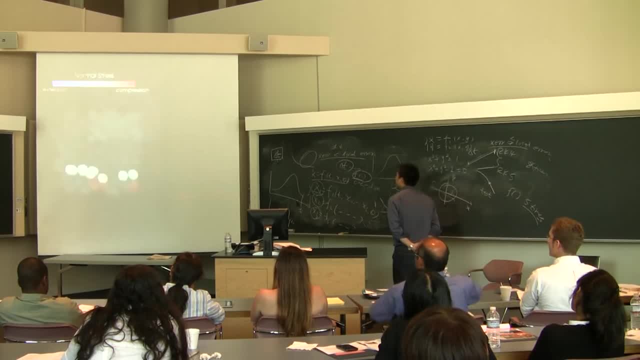 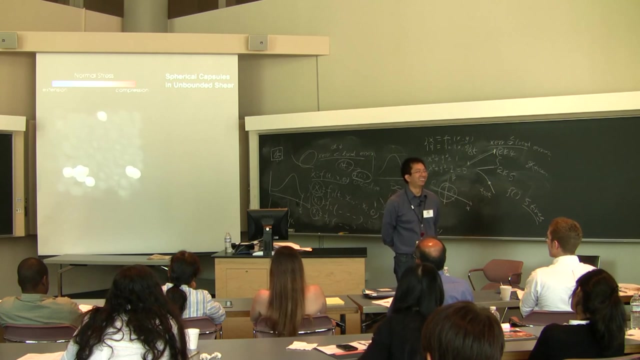 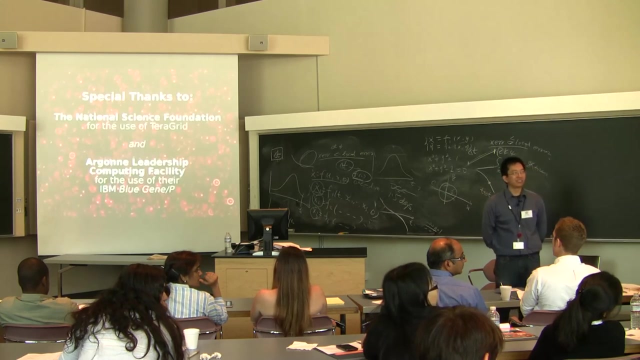 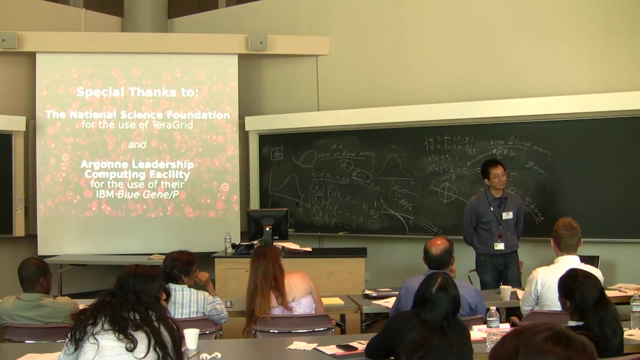 stress: Okay, Okay. Do you want to stop here or do you want to keep watching it, or Okay, Okay. So what kind of literature, findings or data did you use? You don't need data for this. You just create a model and solve it in computer and generate the visualization results. 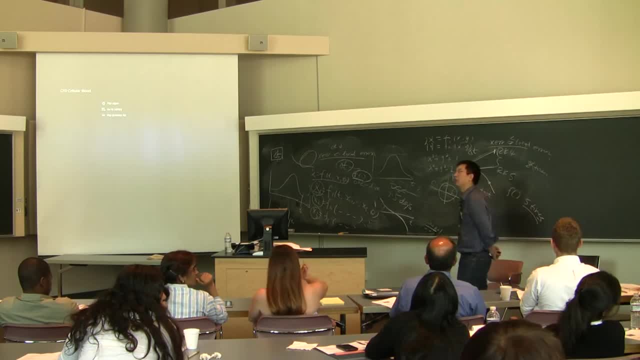 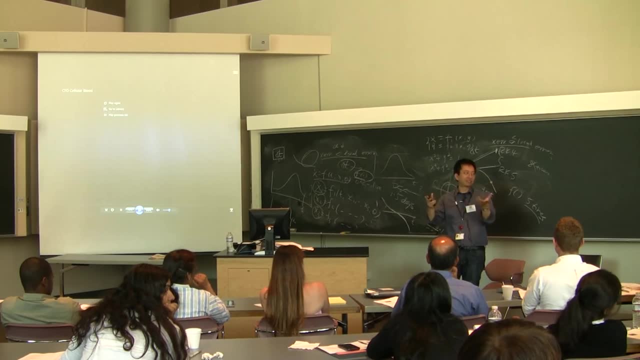 You get a movie, You don't need data. Oh, you do need some data, For example, the physical properties of the membrane or the fluid, Okay, And some value you can take from literature, But you don't actually need to measure anything for now. 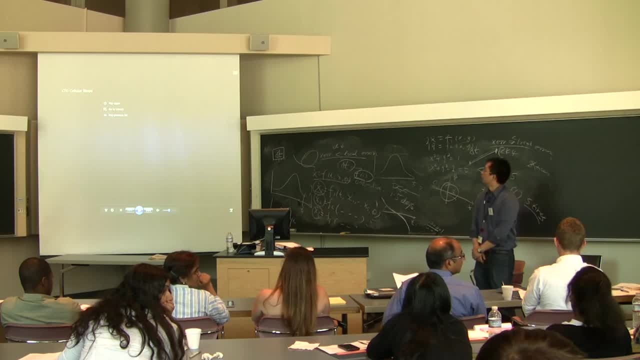 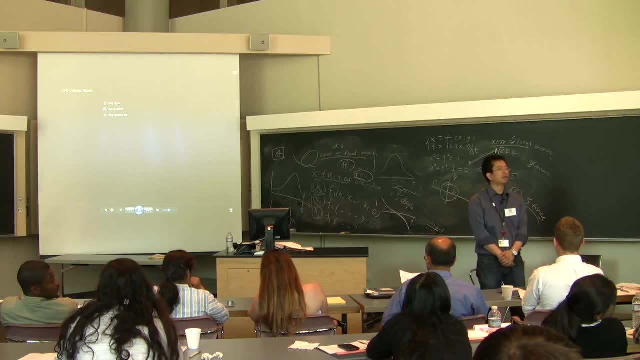 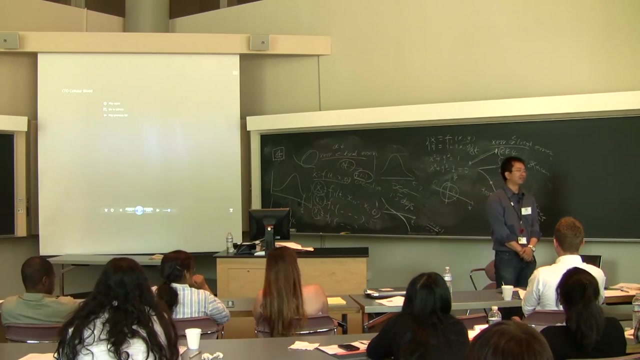 Okay. Do you know if, in this work, the result with this moment match with the prediction by other cells, Mm-hmm. What you just mentioned, yeah, what you just mentioned actually is very, is very, computationally expensive. Okay, But the idea is right. 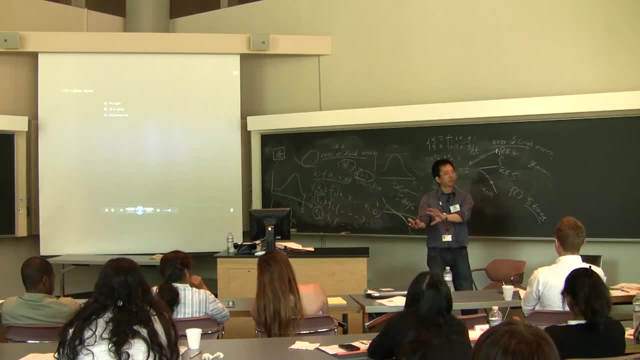 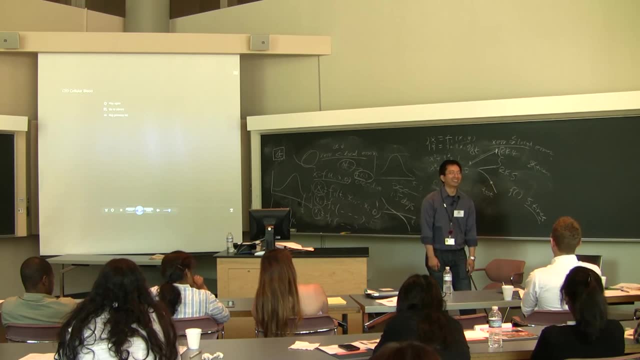 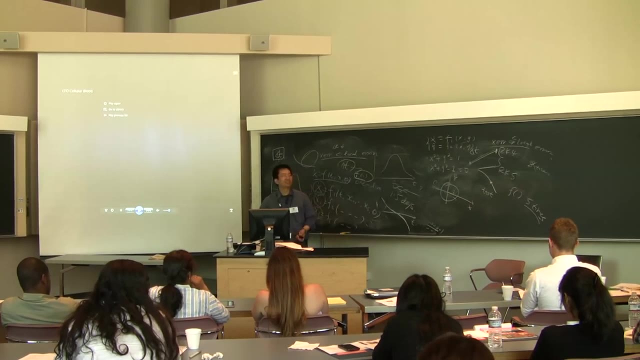 You'll couple the movement of the cells with the fluid dynamics, Okay, But you will not bother to use the Navier-Stokes equation, because that's too much you know trouble, Okay. So this one- actually the way you guys just showed you- unfortunately is not solved. 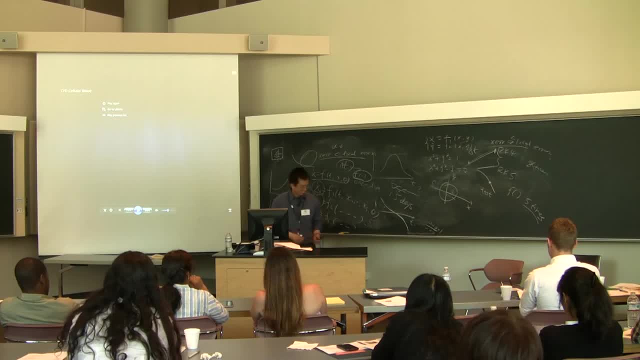 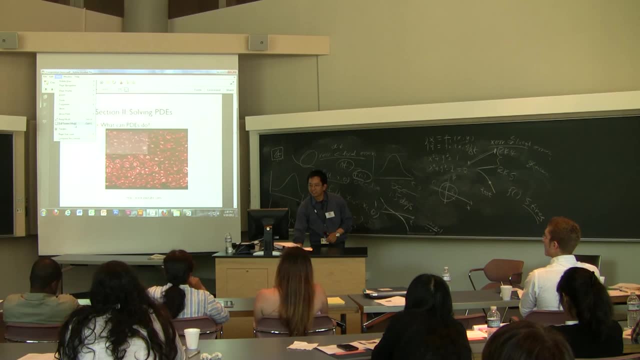 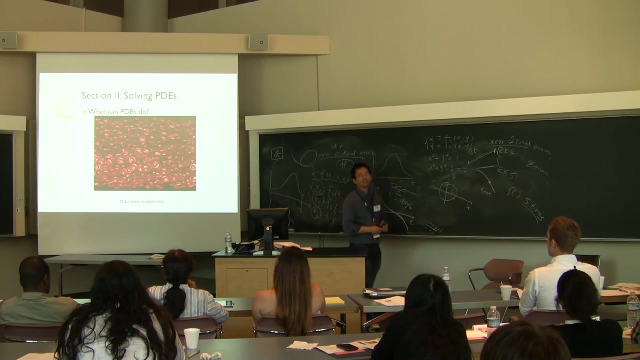 by ODE? Okay, ODE cannot do this, So that's why we talk about PDE, Okay, Okay, So when we use PDEs, okay, as I mentioned before, we can actually take accounting, take the spatial difference into consideration. 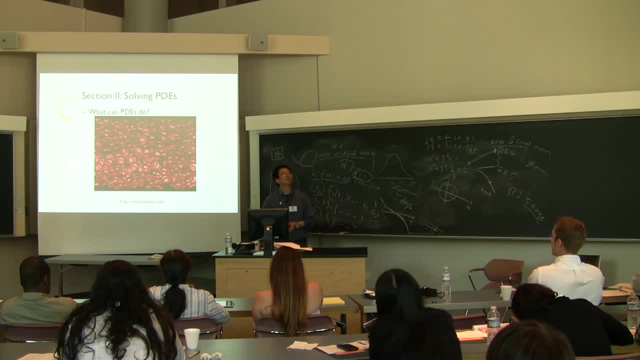 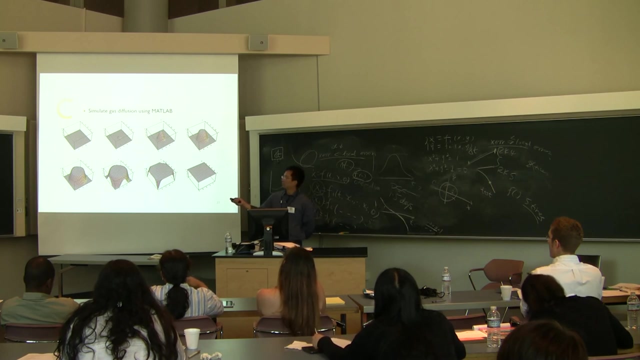 Right, And that's what you can do. Okay, This PDE. Okay, So this is actually. I wrote a simple program to use PDE to simulate gas diffusion. Okay, In my lab actually, You start from a spot and then you look at how long it will take for this gas to diffuse. 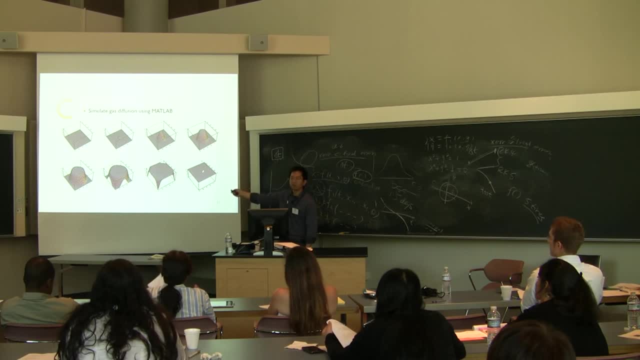 into the neighborhood. Okay, So at different time points you can plot this diffusion, Okay, And eventually this gas covered the whole region you're interested in. So this is also done by PDE. Okay, Now you can tell there is because there is a spatial difference. 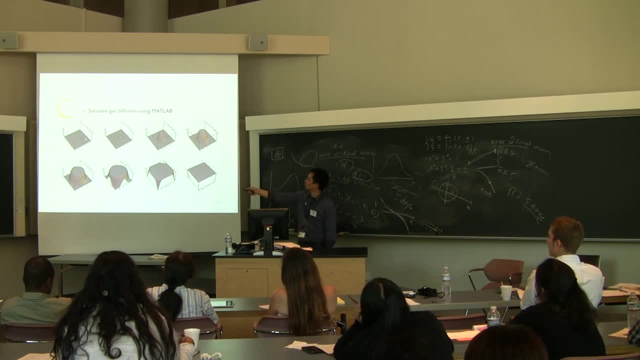 Okay, That's why I use PDE. okay, Because originally the concentration of the gas is very different from the concentration at any other places. right? So eventually, everywhere becomes the same, Okay, So what are PDEs? okay, 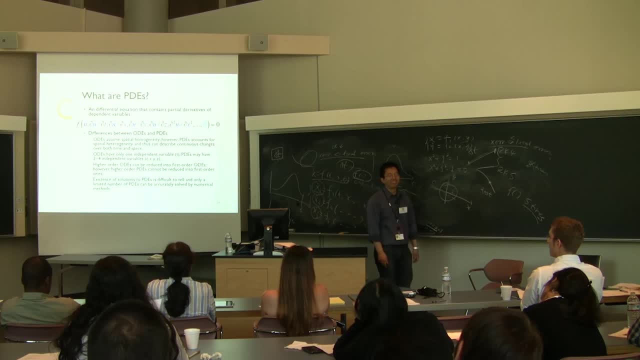 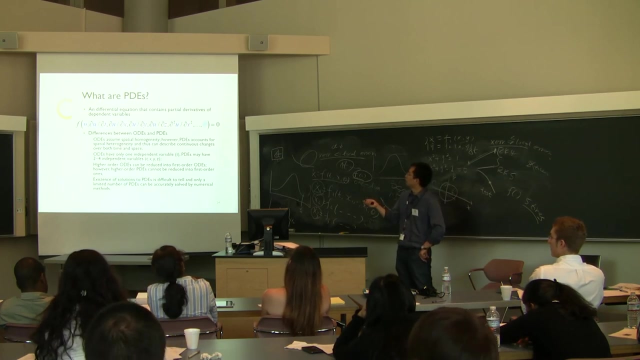 Since we have watched a fancy video, okay, now probably we want to know a little bit about PDE. So PDE itself is similar to OD, but with additional derivatives, So in OD we talk about now. I switched the symbol again. 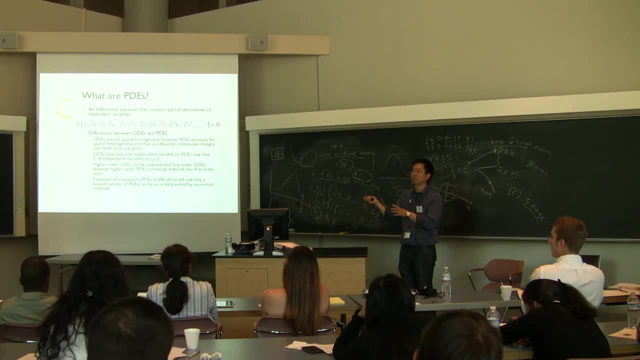 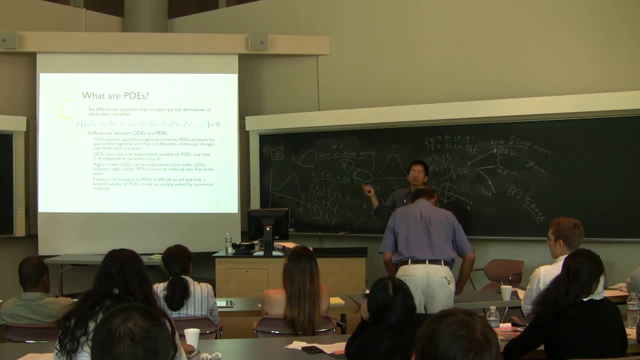 because I have to use X here. okay, for another purpose. So we used to use X to denote the state of variable. By now I use XYZ to denote the spatial coordinates. Okay, that's a three. okay, spatial coordinates- XYZ here. 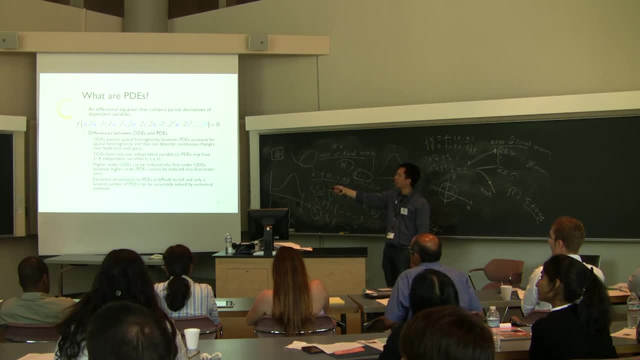 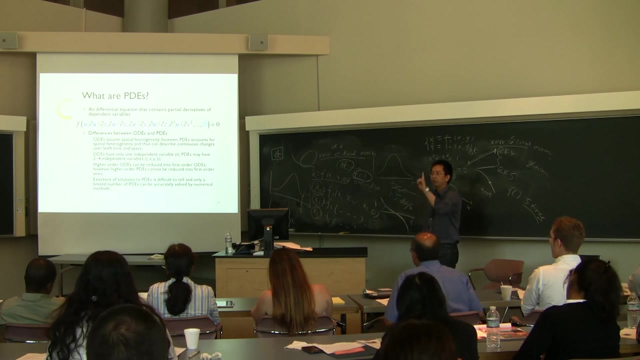 And the T again is our time variable. So our independent variable in this model will be: like how many independent variable? Four We have T, X, Y, Z. okay, Right now we have four independent variable. In OD we only have one independent variable. 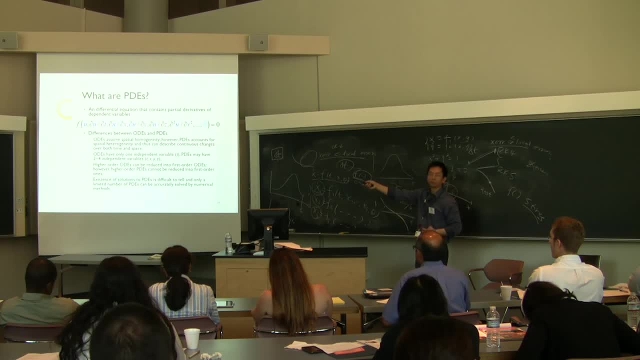 That's T. okay, So now we have the spatial coordinates in the system And also we take the derivative of the state of variable. State of variable right now is U. okay, We take the derivative of U with respect to T, X and Z. 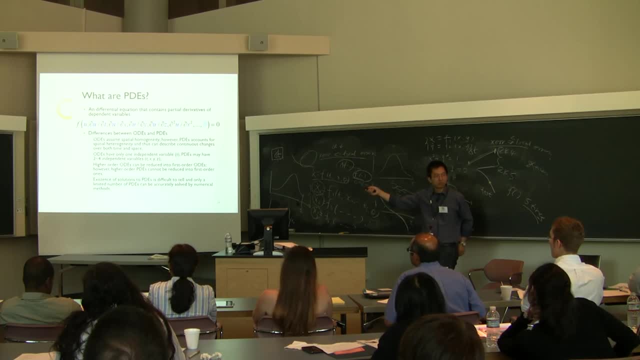 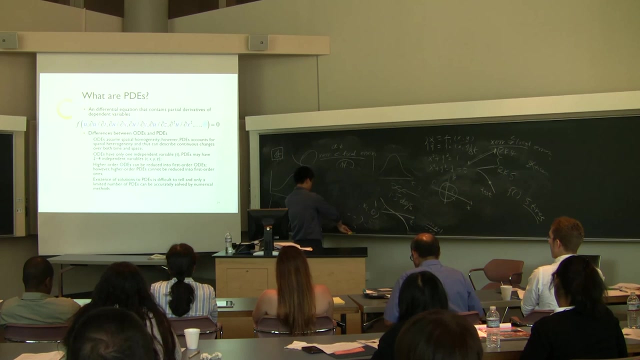 Okay, now you probably also noticed that the notation for derivative changed. okay, So this morning or five minutes ago. okay, we're talking about the derivative and the notation is small d, small d. okay, Now here in this notation it changed to U. 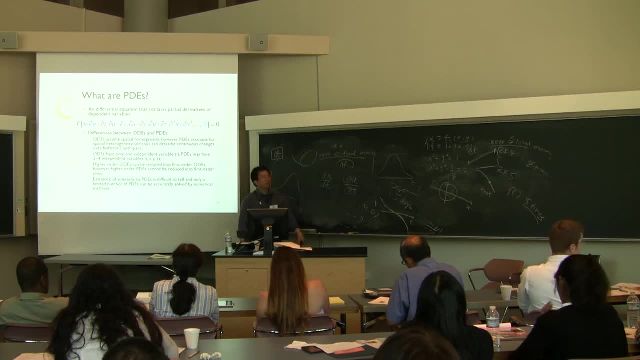 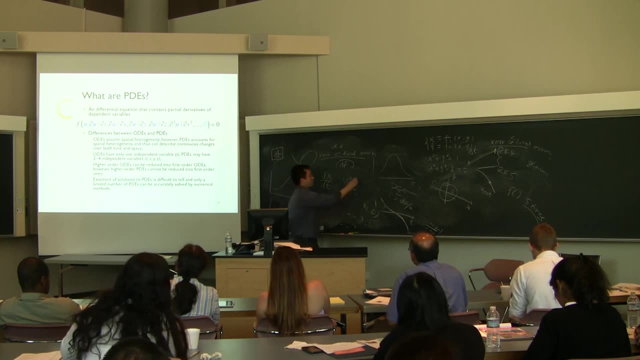 Okay, notation changed So this is still derivative, but it's called partial derivative. okay, Partial, okay, derivative. So what does partial derivative mean? Partial means if I have a function of time and X and Y. okay, 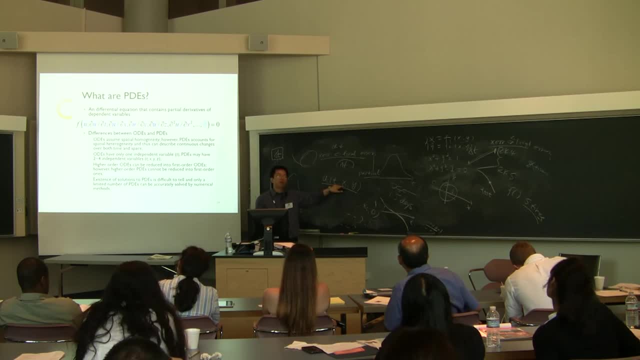 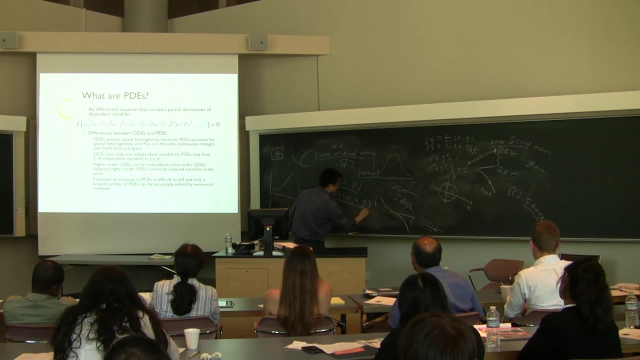 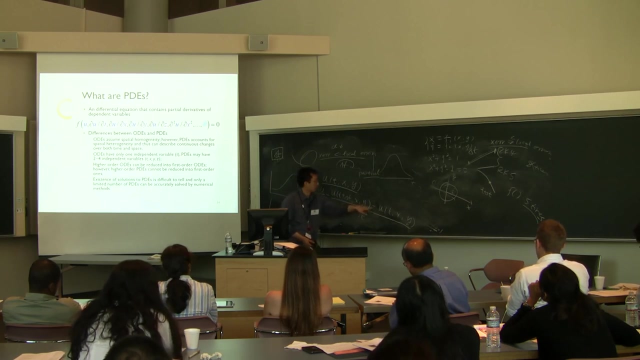 Let's say U is a function of time and also a spatial coordinates- X and Y. So the partial derivative of U with respect to T is that. So the partial derivative of U with respect to T is that I use the same X and Y in these two terms. 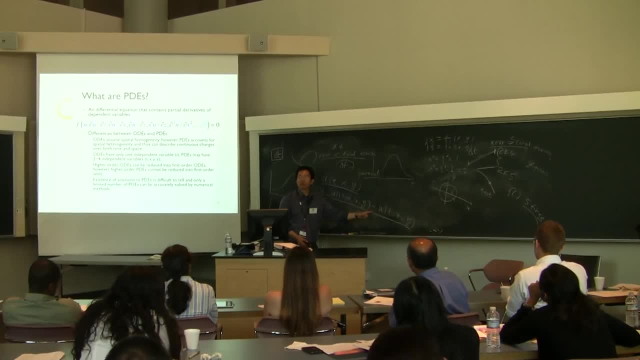 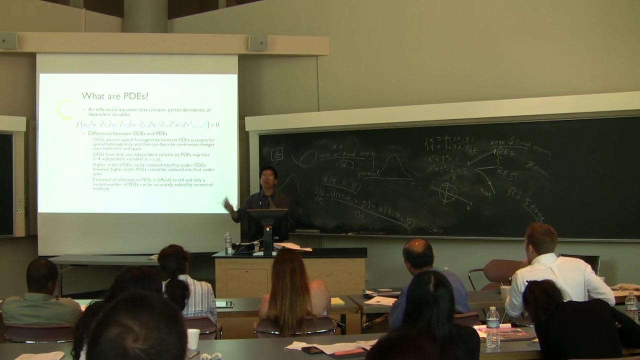 So X and Y keeps the same, okay, I only change the time, okay. And if I change the time, then I calculate the difference divided by the time interval. That's called partial derivative, which means I fixed other variables and only look at the change in one variable. 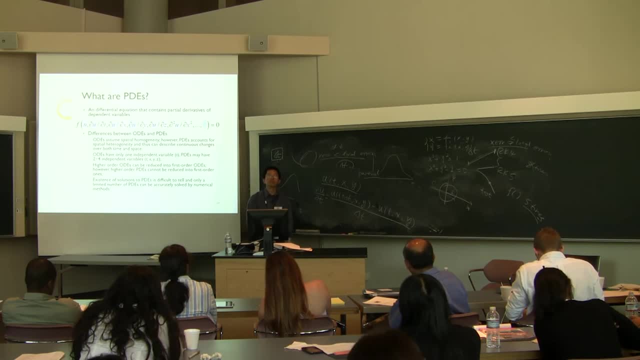 That's why it's called partial derivative. okay, That's the definition. So now let's look at some difference between ODE and PDEs. So now let's look at some difference between ODE and PDEs. 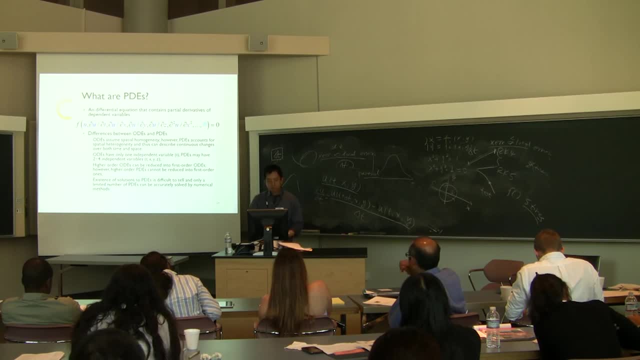 So now let's look at some difference between ODE and PDEs. The first one is that we have talked about this for quite a few times. is that spatial homogeneity? okay, ODE assume that there's a spatial homogeneity. 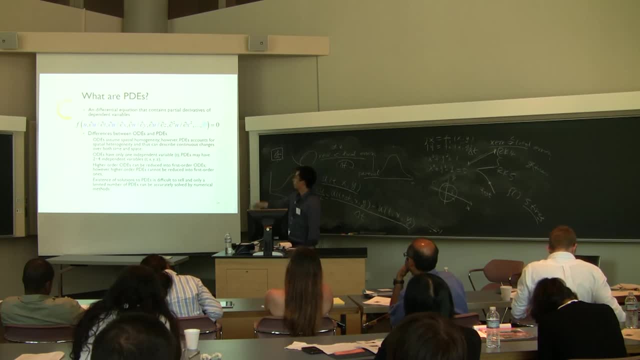 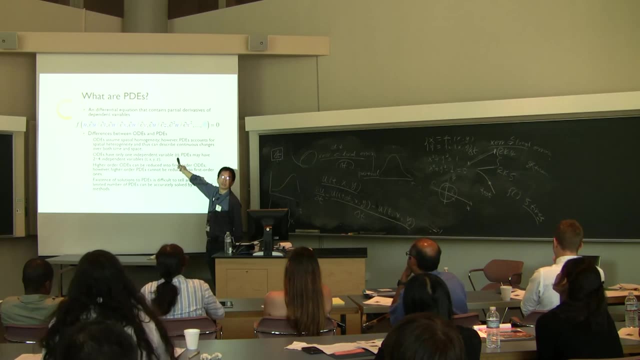 However, PDE does not, So it can actually describe the changes over both time and space. ODE has only one independent variable, T okay. PDE actually can have two, four independent variables. ODE has only one independent variable, T- okay. 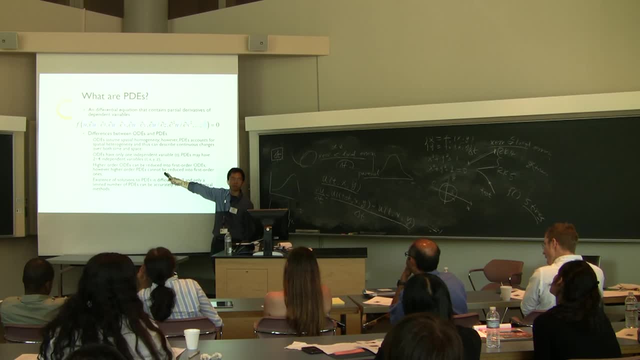 PDE actually can have two- four independent variables. PDE actually can have two- four independent variables. PDE actually can have two- four independent variables. It depends on how many spatial dimensions. It depends on how many spatial dimensions you want to take into your model. okay, 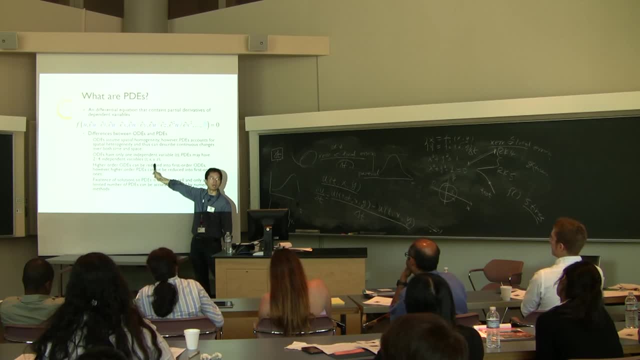 you want to take into your model. okay, You can consider like one-dimensional PDE. okay, You can consider like one-dimensional PDE. okay, You can consider like one-dimensional PDE. okay, That's also fine. 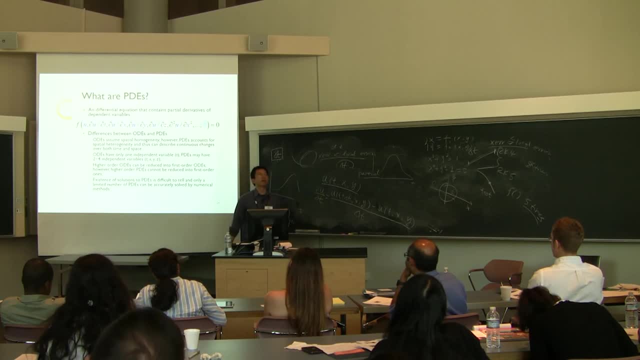 One-dimensional, which means one-dimensional in the space, okay. One-dimensional, which means one-dimensional in the space, okay. So higher orther ODEs can be reduced into first order ODEs, but PDEs can not, okay, unfortunately. 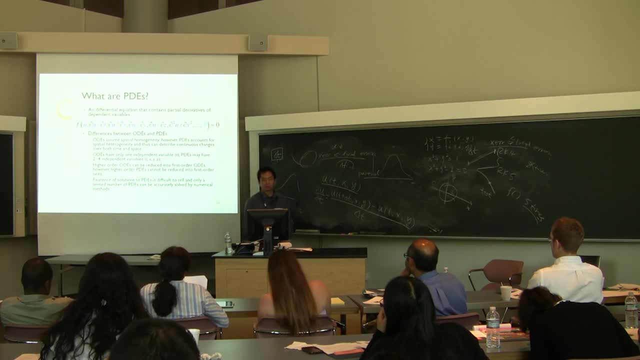 okay, So higher orther ODEs can be reduced into first order ODEs, but PDEs can not. okay, Unfortunately, okay, Unfortunately, okay, Remember, We can reduce this equation,064 01″. Not coaching class intestines. 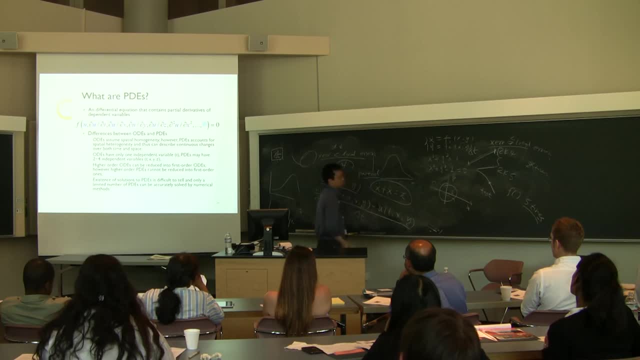 01–1 01″. Remember, We can reduce this equation, okay, We can reduce this equation, okay, Into first-order ODEs, right, By introducing the dummy variable, By introducing the dummy variable for PDE. you cannot do that okay. 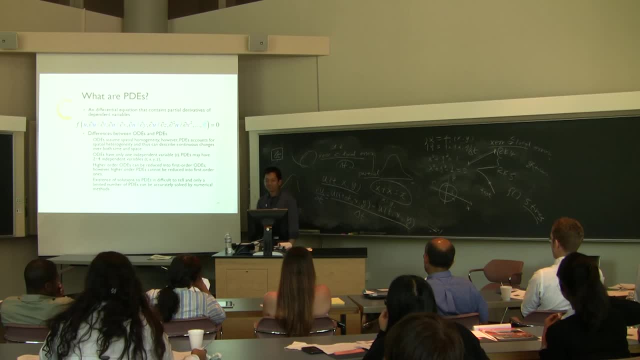 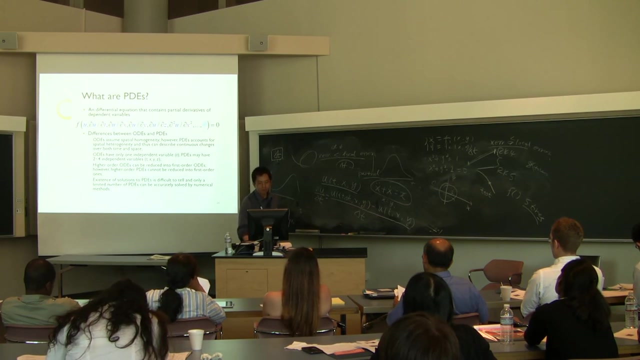 There is no this kind of you know simple way to you know. let you to reduce the simplify the problem. And another bad thing about PDE is that the existence of the solution okay is difficult to tell And so far only a limited number of PDEs can be solved. 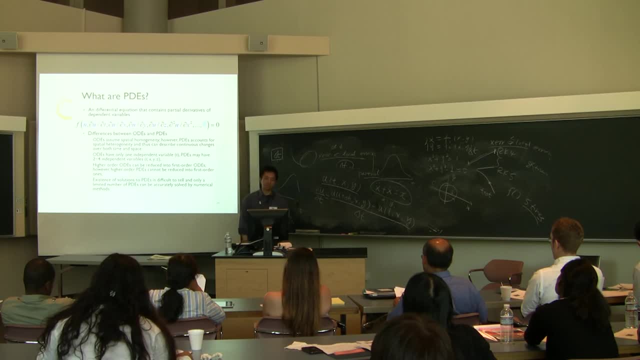 okay, even using numerical method. So that's bad news, but fortunately okay for many of the PDEs. okay, we will use actually in research. We do have tours and you know algorithms to deal with that. 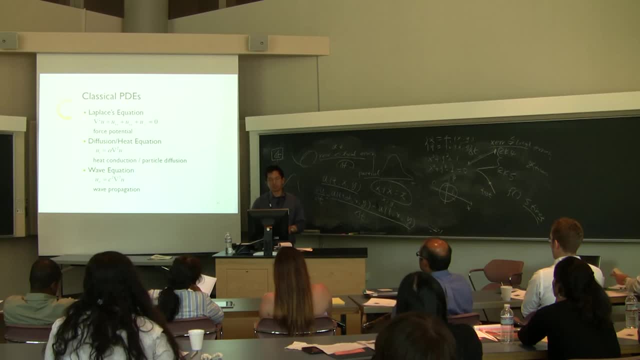 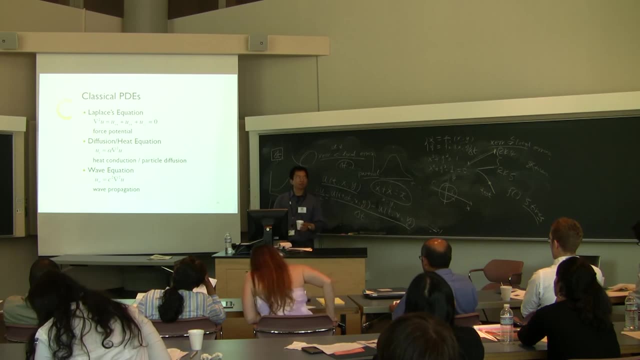 So here is some classical PDEs I want to actually go through. okay, What you need to know is just a name. okay, What's a form? okay, You don't need to bother to understand any of the properties, whatever. okay. 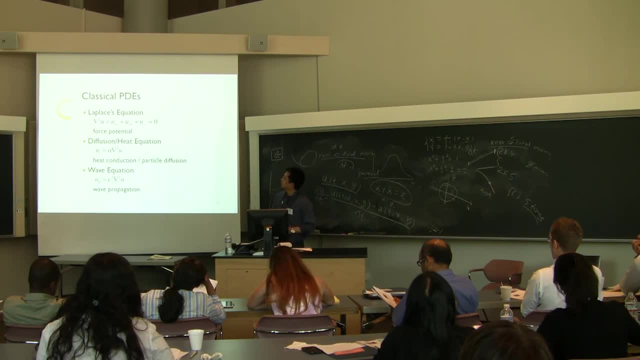 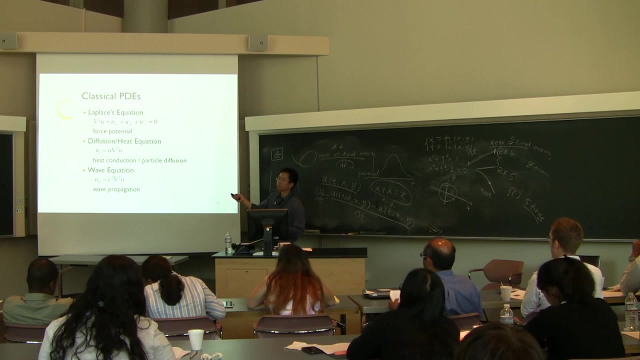 So when people talk about the Laplacian equation, it's just: you add the partial derivative, okay. second order: partial derivative together and the left-hand side then equals to zero. That's called the Laplacian equation, okay. So this notation here means I take the second order. 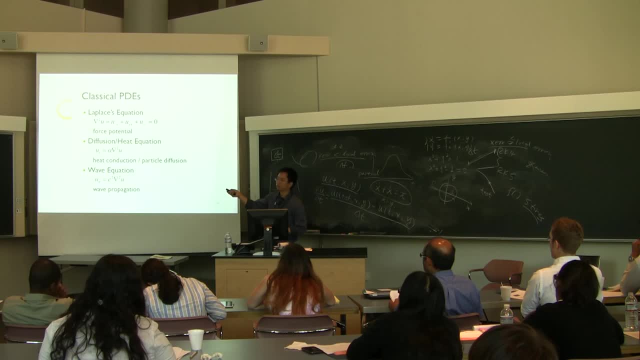 derivative with respect to x, which means I take a derivative once and then again, okay, to the same order With respect to the same variable. okay, So that's what it means, And this one is the diffusion equation. That's actually the equation I just used. 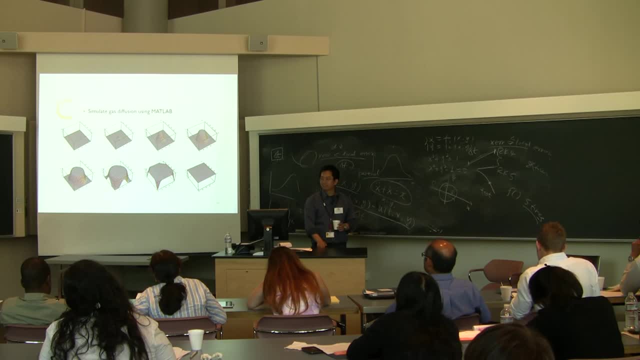 to generate this plot. okay, It's a two-dimensional diffusion equation. okay, You can solve. And here is the wave equation. So I suggest by name, you can use this to describe the wave, water wave or whatever earthquake wave, okay. 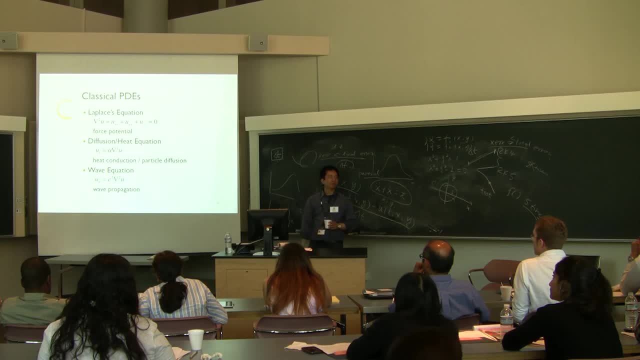 It doesn't matter what kind of wave, okay, Actually people use this equation to evaluate building safety. okay, against earthquake. So once you have earthquake, actually you will get waves propagate in the soil. okay, And then this wave, this vibration, will propagate. 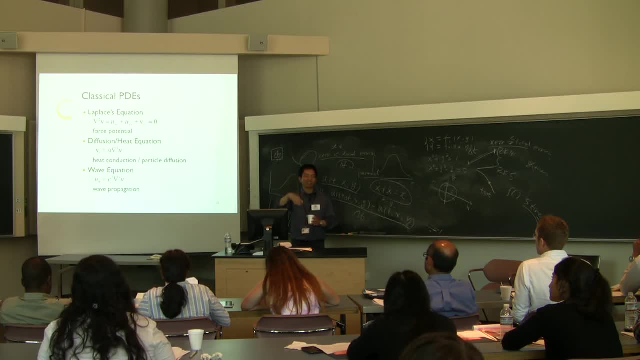 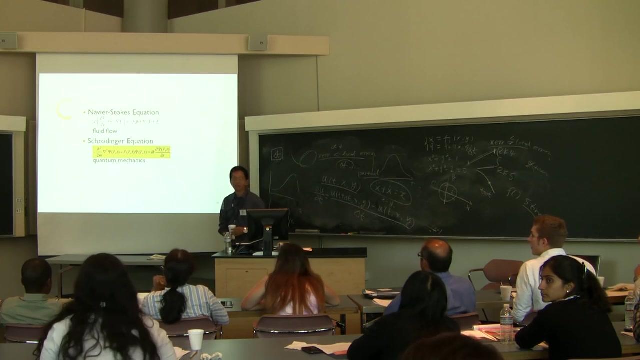 to this building and this building will start to shake And you can actually use this kind of equation, okay, to predict, okay, whether this building will fall apart or, you know, survive What? Oh, This one, this notation, okay. 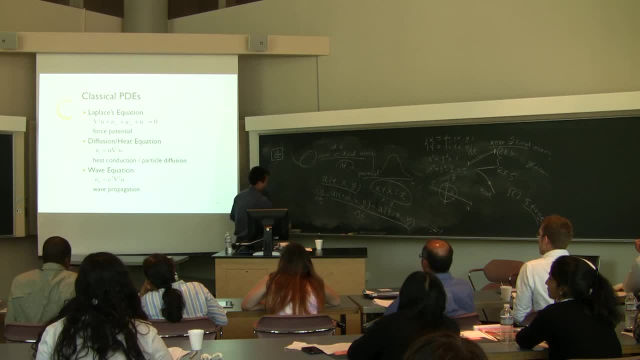 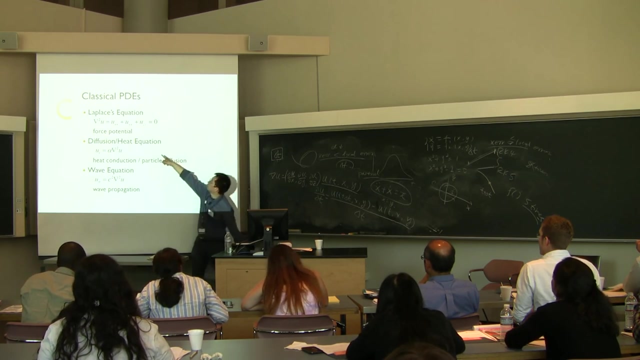 So that's why people hate mathematician. okay, This one means First order right here. Okay, And if I put two, put a square there, then it becomes a second order. Let's see Nothingahan volume system right now. 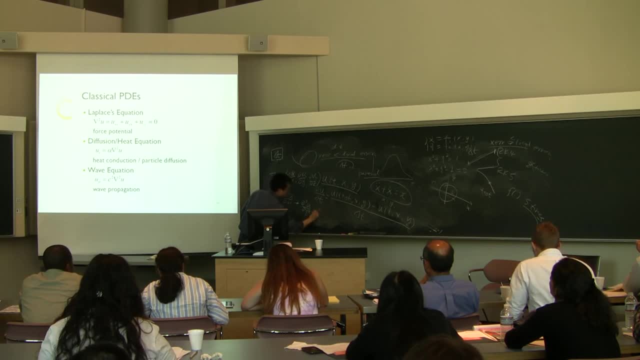 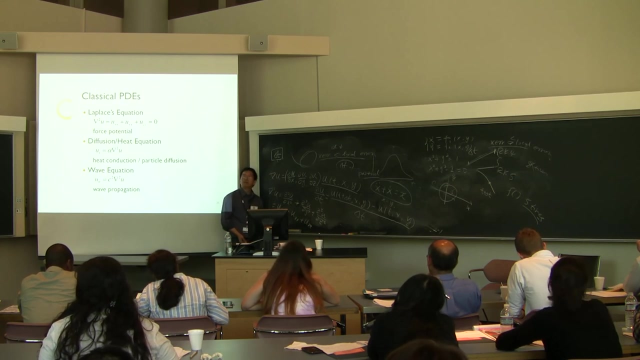 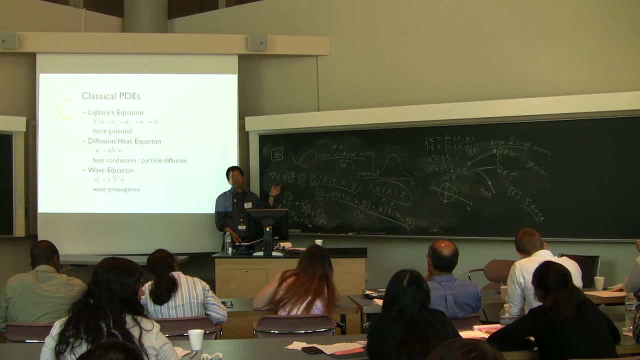 Okay, Now, let's keep our flow unbrake, At least gonna ignore it, okay, Which is what we saw on this slide, okay, Okay. So, since you asked this question, I have to mention: okay, This is an Konzhaler Toll incident. 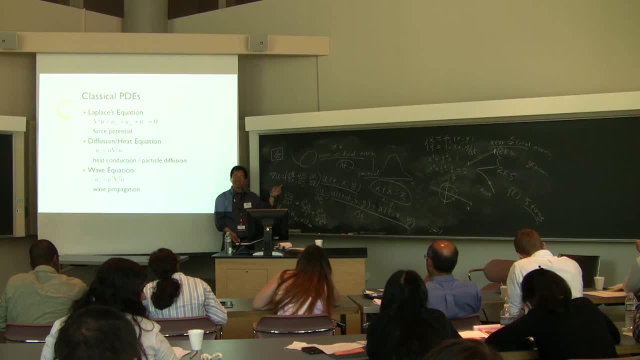 Okay, Sorry guys, It's not Kong dying today. Okay, This is not a summation. okay, This is a vector. You get a vector over three elements. okay, If it's a gradient, it's called a gradient, okay. 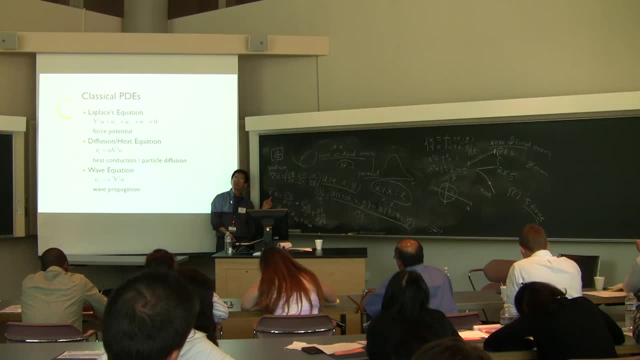 This is not a summation, okay. This one is a summation, okay, So there's a difference here. but if you're saying it's not important, okay, but anyway They're different, okay, So, but it doesn't matter to actually. 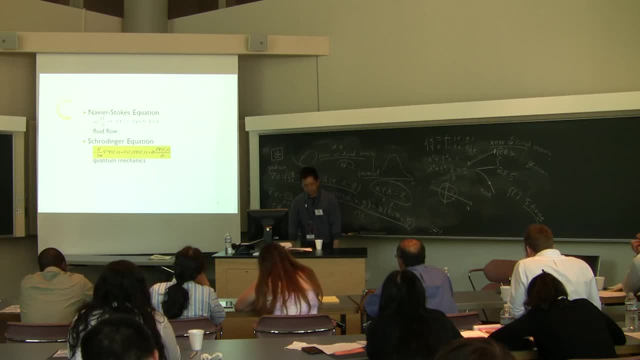 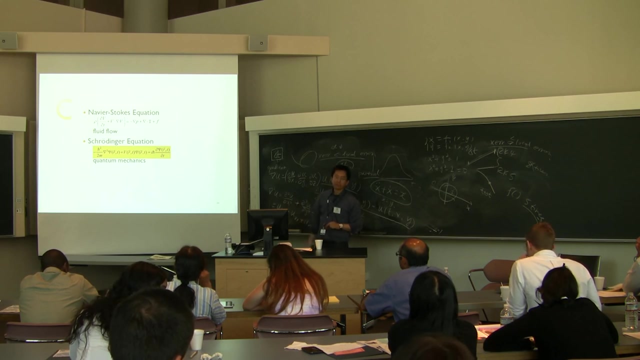 what we're trying to deliver here. okay, I just want to show you some classical PDs, okay, used in engineering or whatever. And the next one is just mentioned by- I don't know what's your name, Anyway- Navier-Stokes equations. 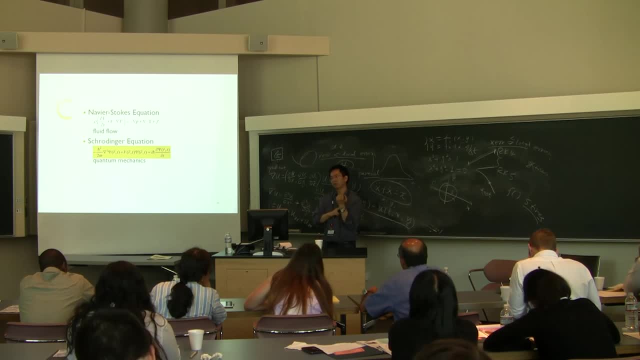 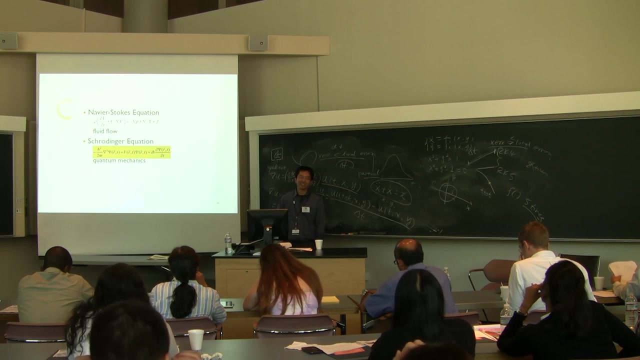 One equation you describe all the almost all the fluid dynamics. okay, Use this one equation. okay, All fluid dynamics can be described using this one equation. okay, That sounds perfect. right, But unfortunately okay for a specific problem. okay, 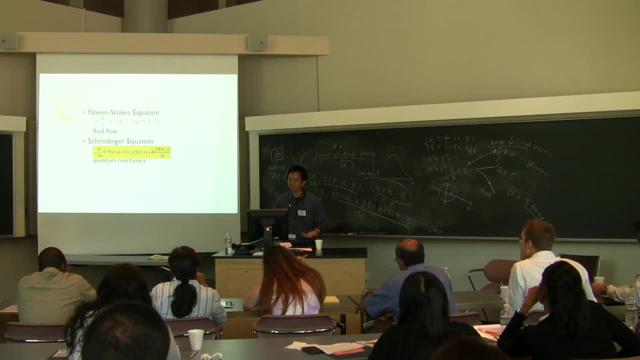 you can actually earn yourself a PhD degree. okay, by solving one specific Navier-Stokes equation. okay, So by play with the boundary conditions or whatever. okay, So that's how I actually get my PhD degree anyway, So okay. 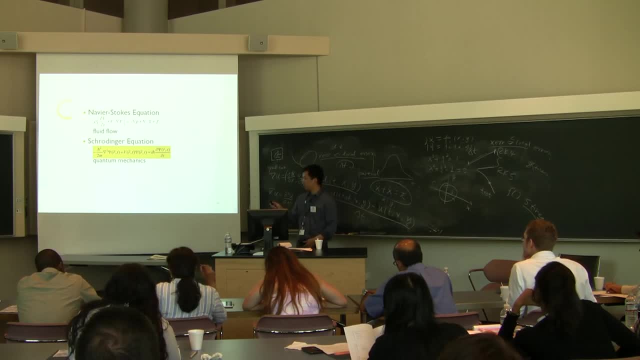 Okay for people who are interested in molecular dynamics: okay. the Schrodinger equation: okay. that's what you should know, Although you don't need to care about the technical details, but that's a name okay. Quantum mechanics: okay. 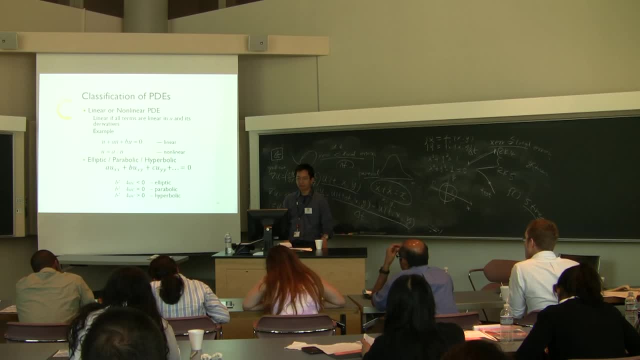 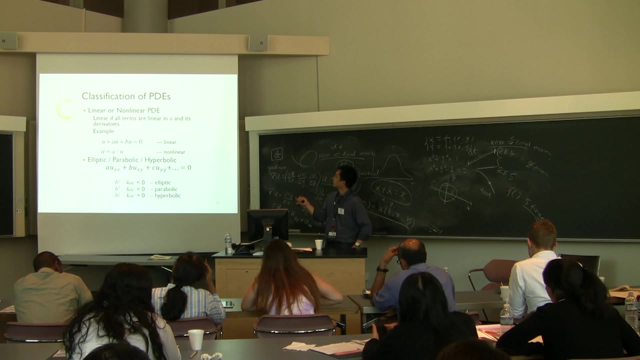 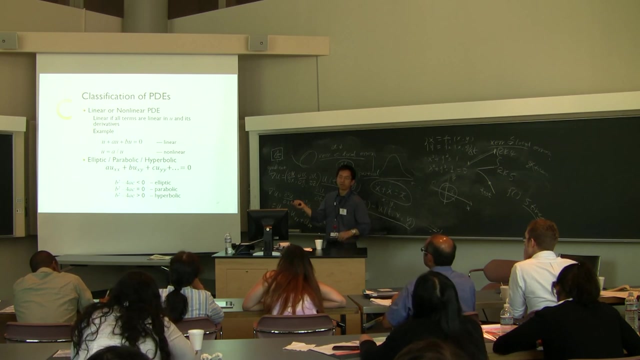 It's also PD, So PDs, for simplicity, we can also actually classify, okay, the PDs, okay, Into either linear or non-linear PDs, okay, And the linearity actually is respect to U, okay, The state variable or dependent variable, okay. 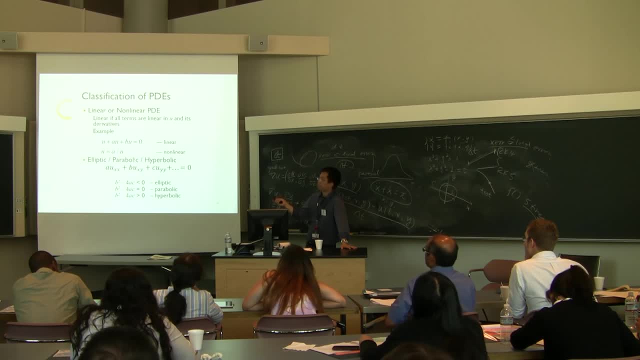 So this one is a linear PD. this one is not Because U right now is in the denominator okay. So also, if you look at PD, you'll probably also will hear people talk about elliptic, parabolic, hyperbolic. 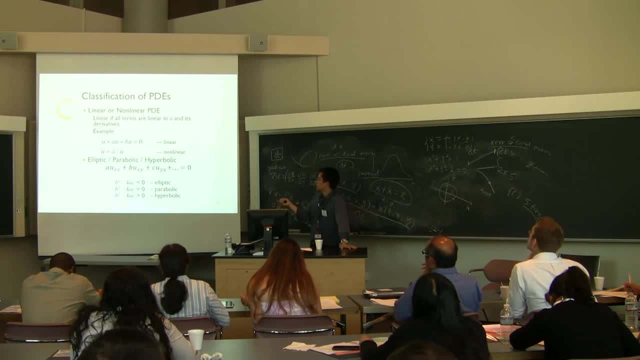 Make it simple. okay, That's just for some historical reason. okay, people would classify the PD in this way. But when you solve a PD, okay, you probably can. I don't need to pay attention to this. okay, Just some terminology. okay. 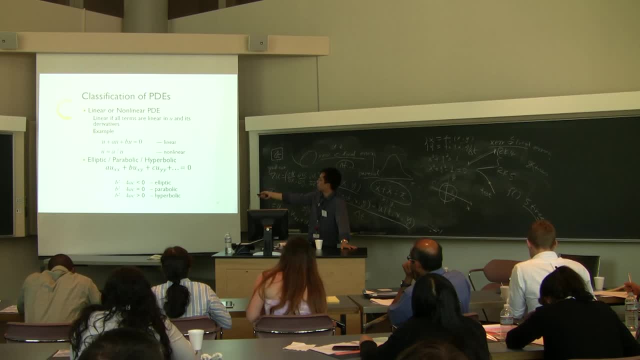 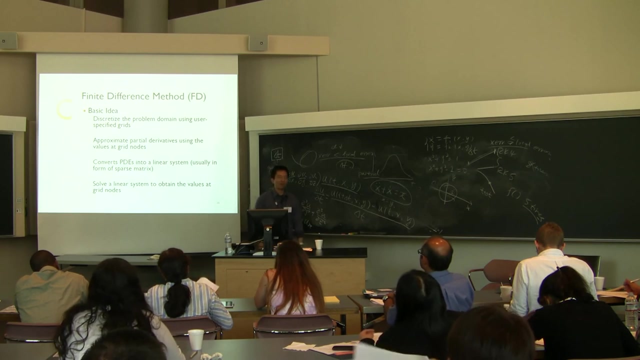 So if you have a second order PD in this way, you just look at the coefficients, okay, If this relationship holds you equate, the holds you equate, elliptic or whatever. So that's just some terminology, Okay. So now I'm gonna talk about how to solve it, okay. 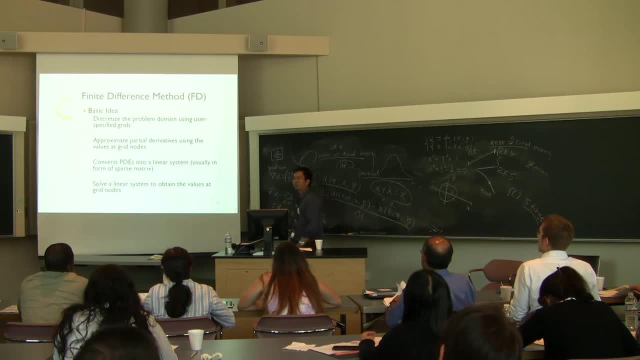 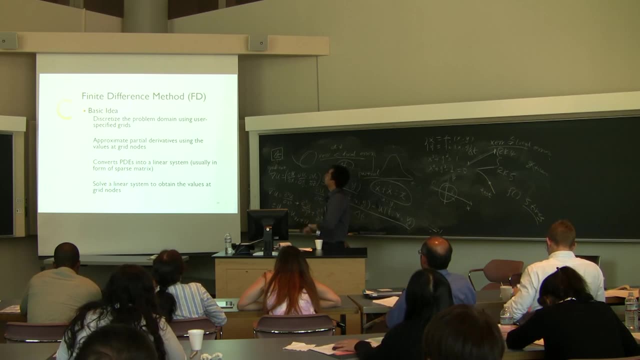 We have talked about the PDEs. we watched the video. okay, Now we want to know actually how to solve them. So to solve the PDEs, the first classical method is called the finite difference. Okay, actually we have talked about. 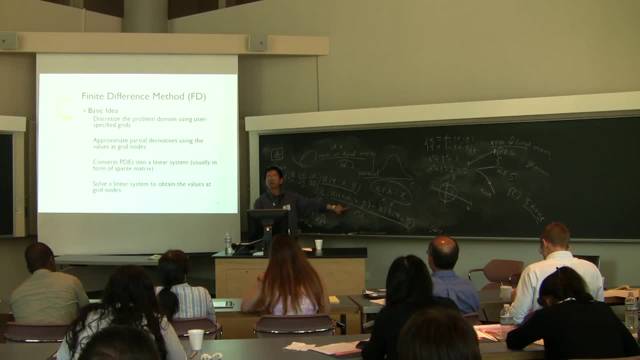 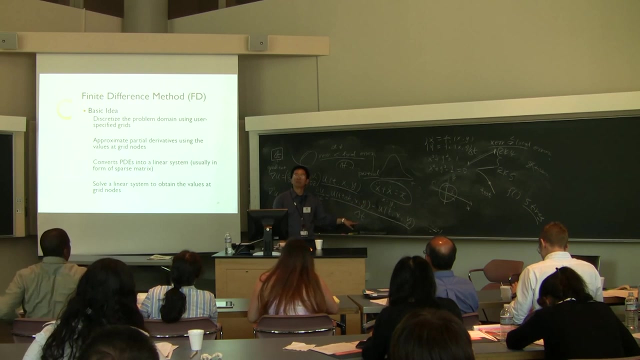 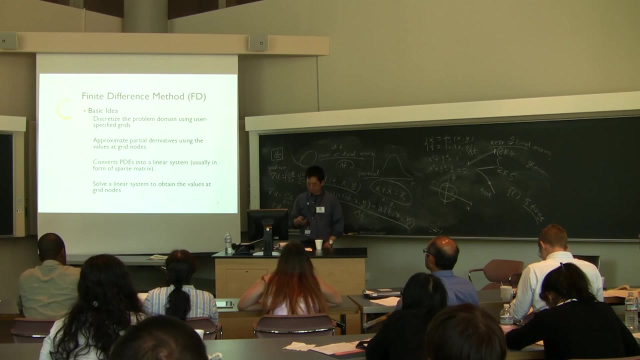 the finite difference method already. This is finite difference method, okay. So the partial derivative is approximated by the difference after the interval divided by the interval, And that's called finite difference. So there's nothing magical about this method. So by doing this, okay, the advantage is that 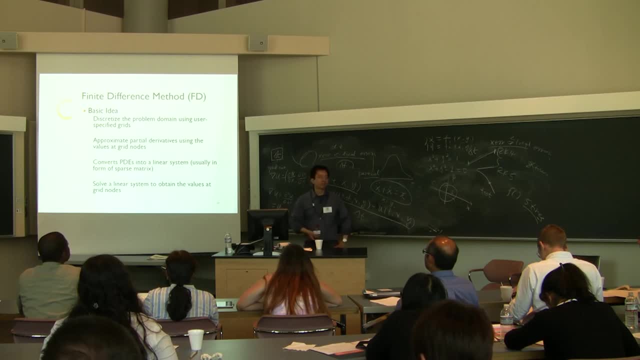 you can convert the PDEs okay, into an inner method, Into an inner system. That sounds good, right? PDE itself looks pretty complicated. okay, as we show here, right. But now, if I can convert this one into a system like this, 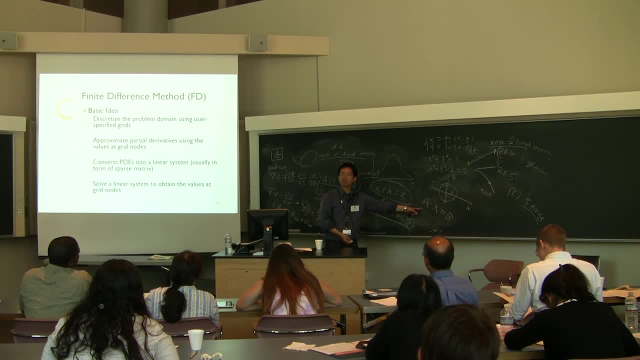 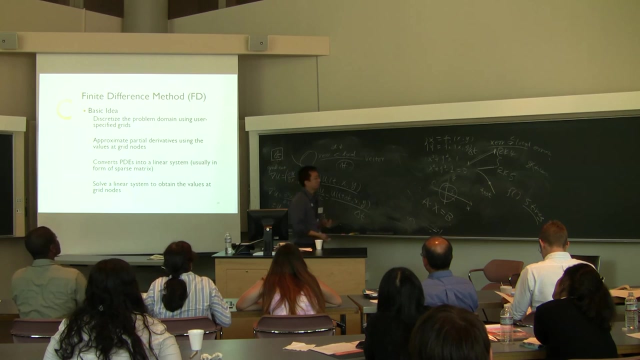 This is a matrix. Is there anyone who doesn't know what is a matrix? I don't think so, right? Or there does? Okay, I got an answer. So What is called a vector is actually a bunch of a number. 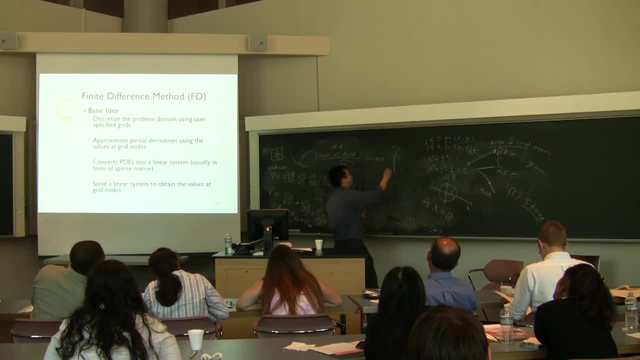 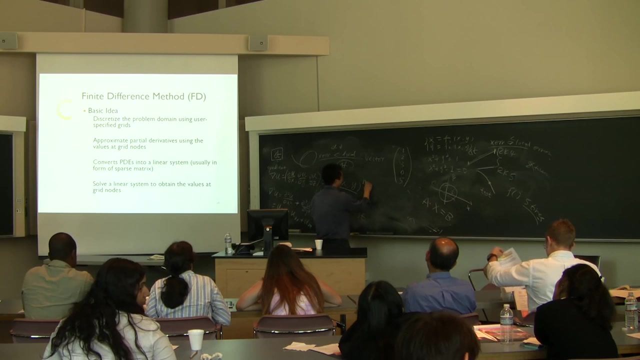 okay, you put them in a column That's called a vector. okay, That's a vector. So you put some numbers in a column That's called a vector, okay, And when we say matrix, matrix, it actually is multiple columns of numbers, okay. 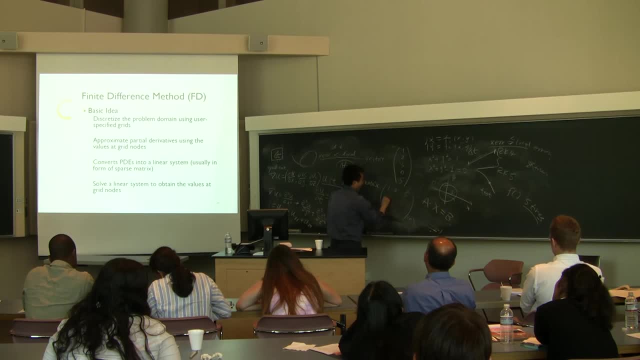 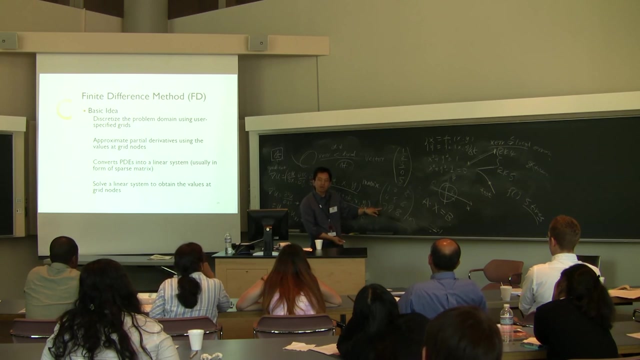 So there's nothing you know mysterious here. This is a matrix, okay, A matrix that has eight, nine elements. This is a vector that has five elements- okay, Or five, because we have five numbers, okay, And this one has nine elements. 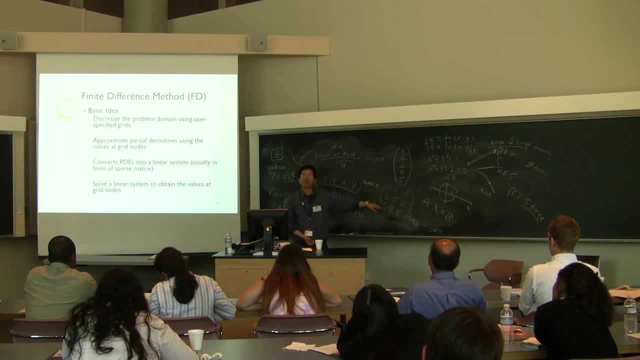 Or we call it a three by three. okay, Because we put the numbers in this way: Three rows, three columns- okay, So that's a matrix. So now what I can do using FD method is that I can convert a PD into this kind of equation. 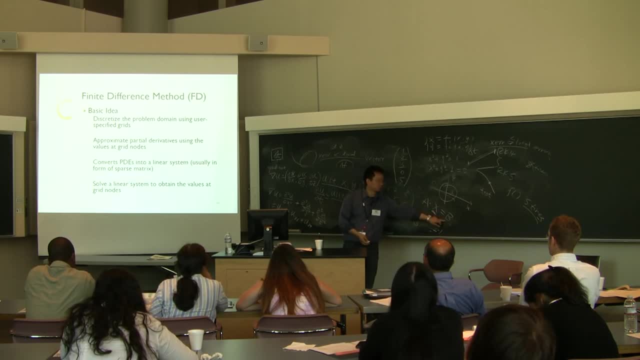 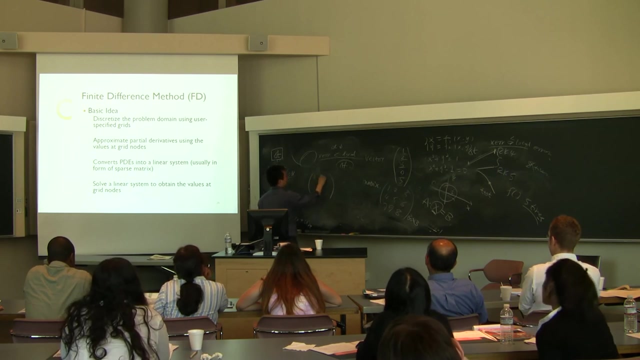 So a matrix: multiply unknown vector X to another vector. What I need to solve is X, For example, one, two, three, zero, one, two, zero, zero one. that's my A matrix, And what I want to solve is X, one, X, two X, three. 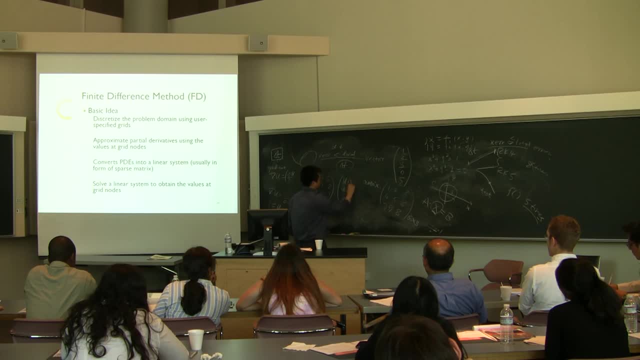 Or let's use U okay, U, three, And this one is equal to, for example, four, five, six. Okay, this is what I call the linear system. okay, This is unknown And you probably understand that this is a linear system. 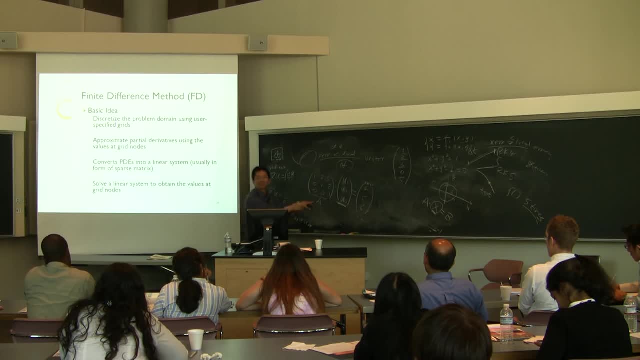 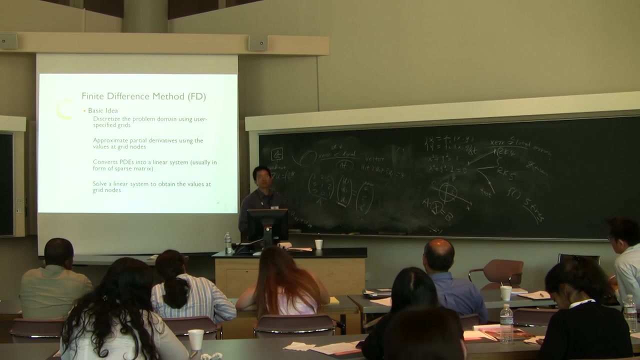 So you can ask: okay, what the hell is this? okay, This one can use the equivalent to what: Mu one plus two, mu two plus three, mu three, Which is to four, See row by column, equals to this element. Okay, that's a product of matrix and vector. 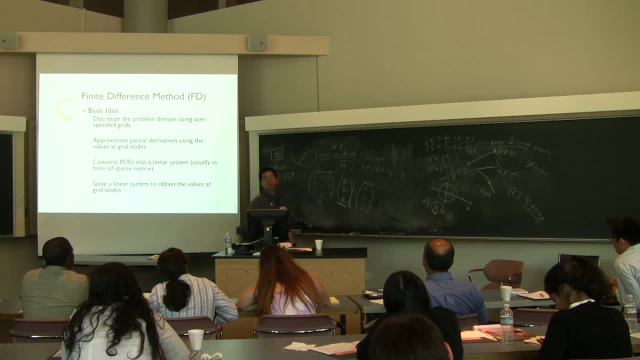 Row by column. okay, you put one with mu one, two with mu two, three with mu three And add them together and you get four. Similarly, for the second row, I can put zero with mu one, you get zero. 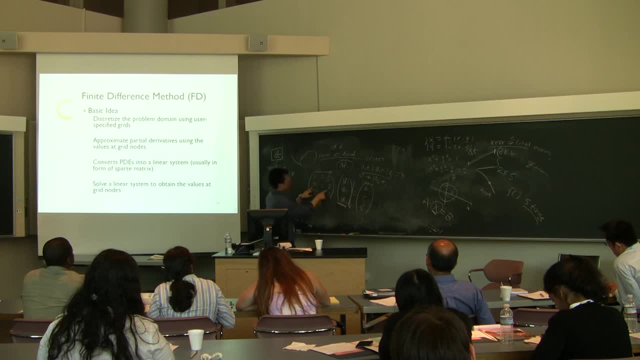 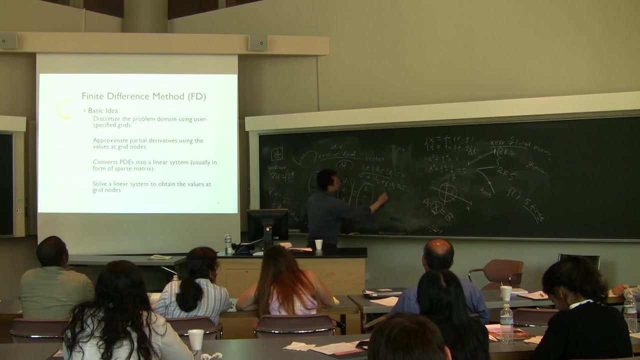 One with mu two, you get mu two, And the two with mu three, and then X to five. So I can also do the same thing right for the last row: Zero, zero, U three, X to six. 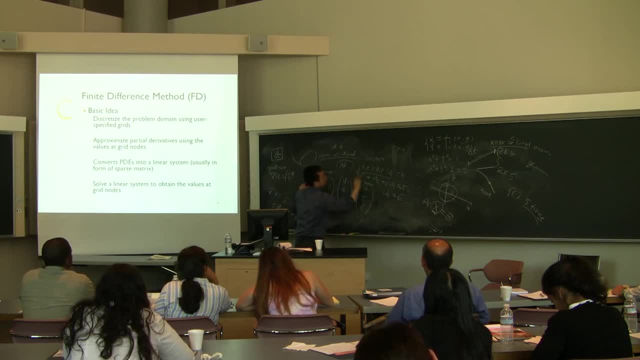 So this system is equivalent to this system. okay, It's just a notation. okay For simplicity, okay of notation, People write it in this way, But indeed, okay, These are three equations And you know how to solve it right. 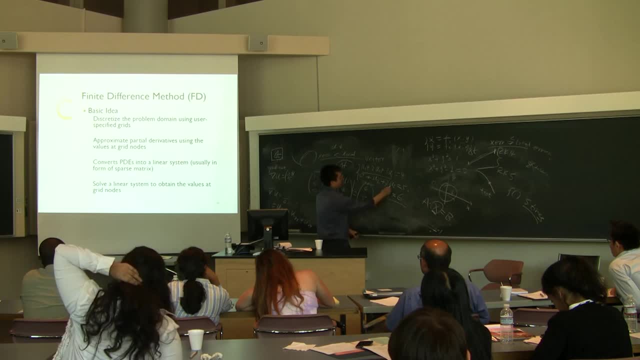 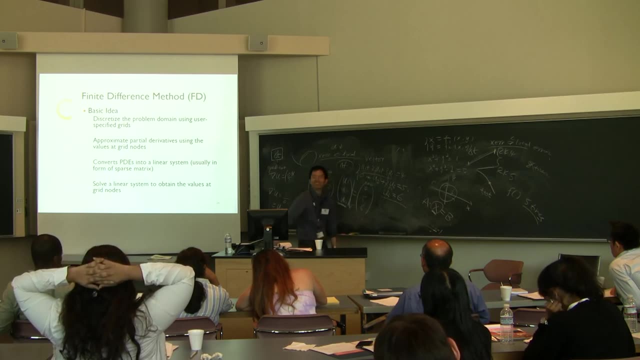 Because this one is pretty simple. U three is X to six. Plug this back to here. you can solve it for U two. right, When you plug U two back here, U three back here, you can solve U one okay. 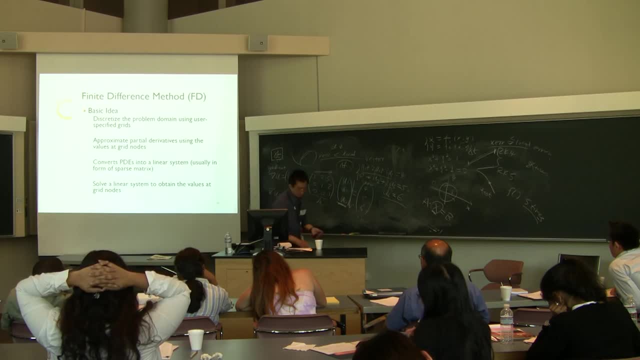 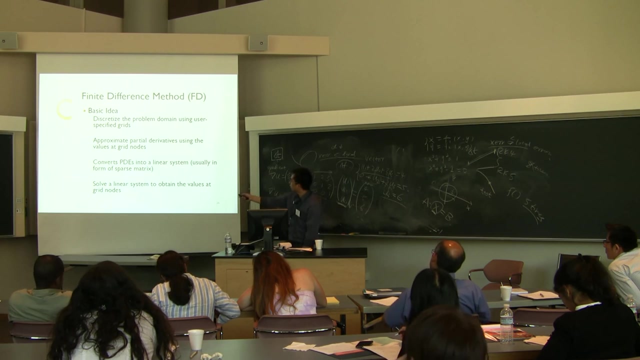 So that's a linear system and how to solve a linear system. okay, So a key step in a finite difference method is that we actually divide the problem domain into, you know, grids. okay, That's how we can actually generate this linear system. 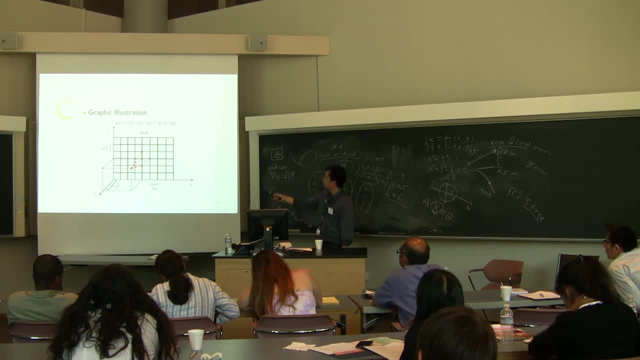 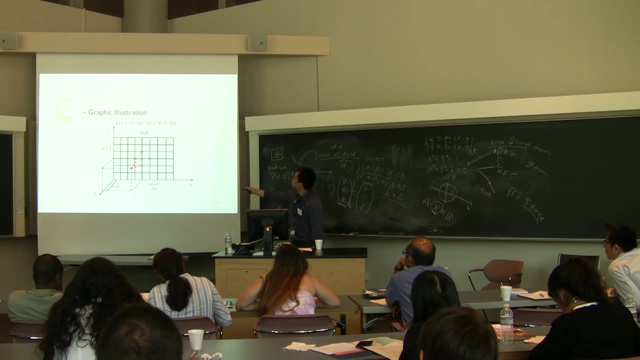 For example: okay here, If our problem domain is a square, okay then if I want to solve it, I actually divide this problem domain into smaller, much smaller squares. Then what we want to know is U right? Then we use the value of U at each grid node, okay, 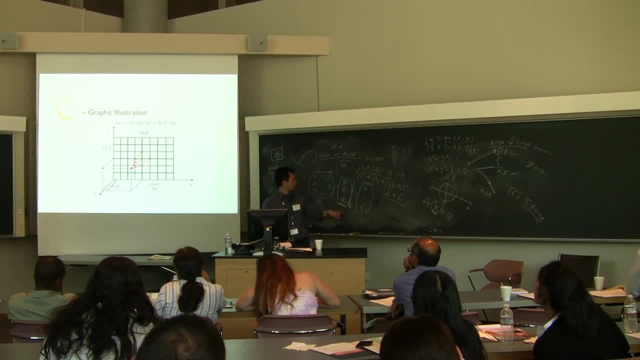 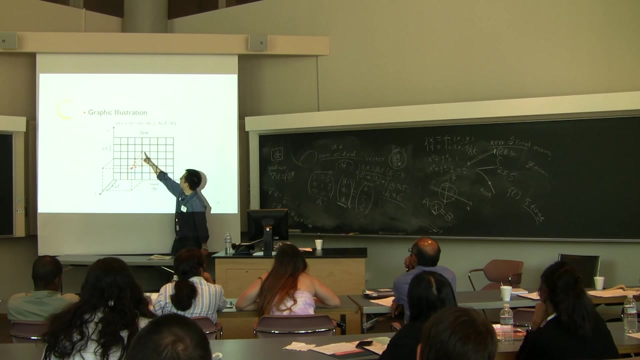 to approximate the derivative. Remember- Oh, I erased it- but For example, DX, right, We can actually use this to use this to nodes To calculate the derivative here. right, The change in the value divided by the interval. 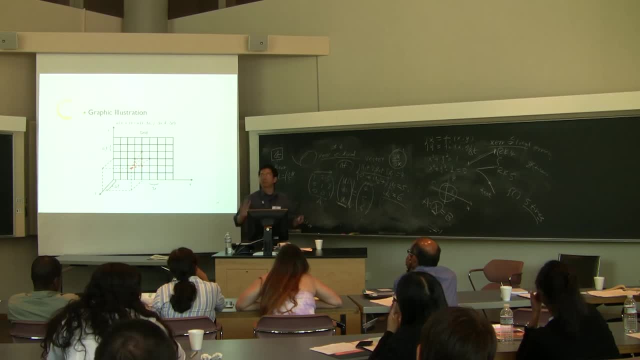 you get the derivative here, right. So that's actually the idea, okay, Totally the idea. You can do the same thing in the time domain, okay, And so if we look at an example, remember, we have a Laplace's equation. 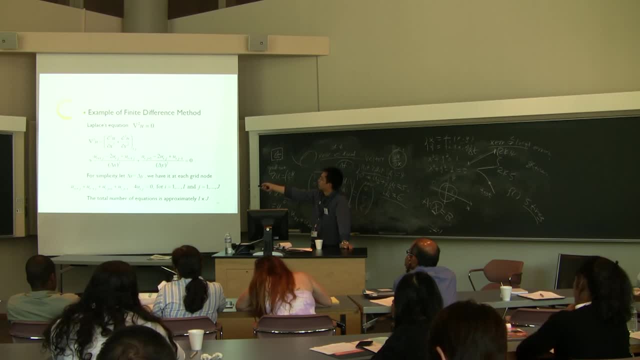 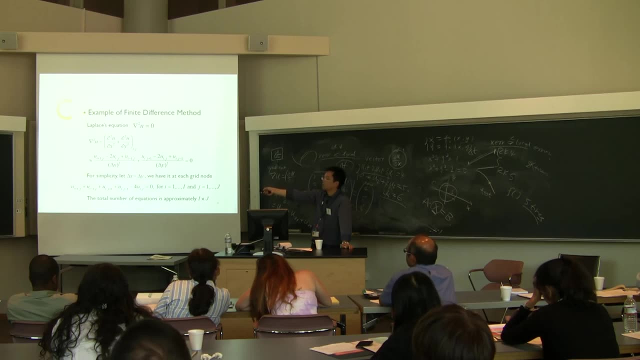 That's a second order partial derivative, And we just use this approximation. okay, Calculate the slope. okay, The slope of the slope. okay, It's just the approximation to the slope of the slope. So you know how to do it right. 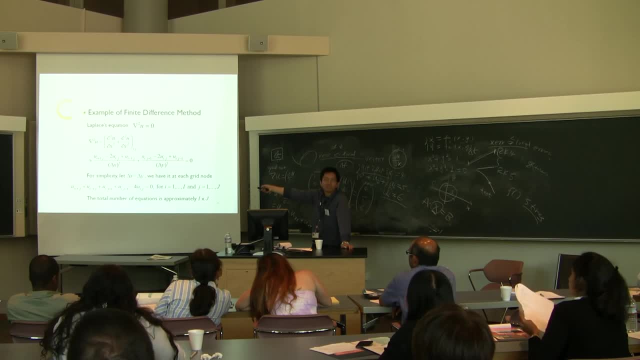 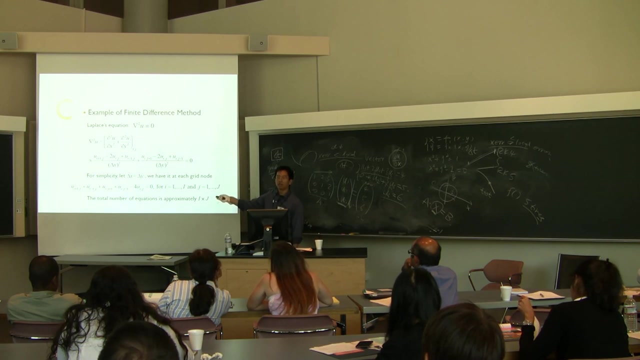 We have talked about it okay before. So you just plug in this approximation into the original equation and that's all Okay. So, for example, if you let their X X to their Y, you can get an equation like this: 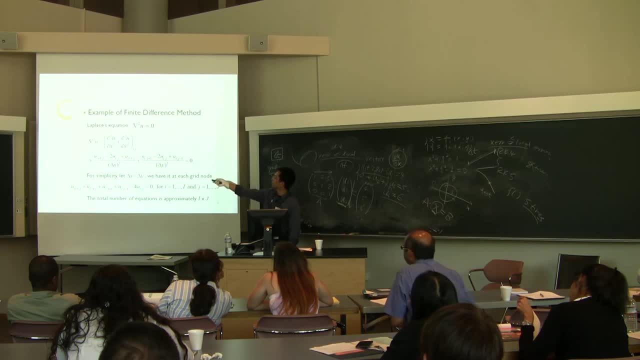 At each grid node. okay, That's what you actually come. that's actually okay. That's actually come from here. okay, From here to here. If you don't mind, do some. you know simple mathematics. This is, there's nothing. you know difficult here. 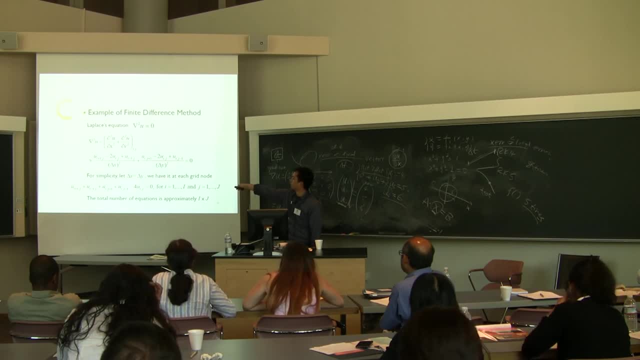 You just let this two equal be equal and then this two can be canceled out, right? Then you just rearrange the nominators and you get this one. okay, So also that here the? U, all of the? U are unknown, okay. 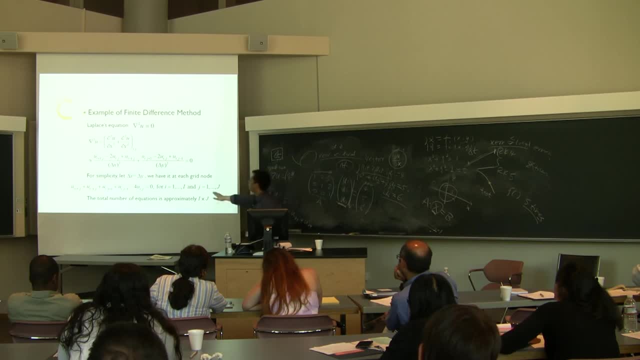 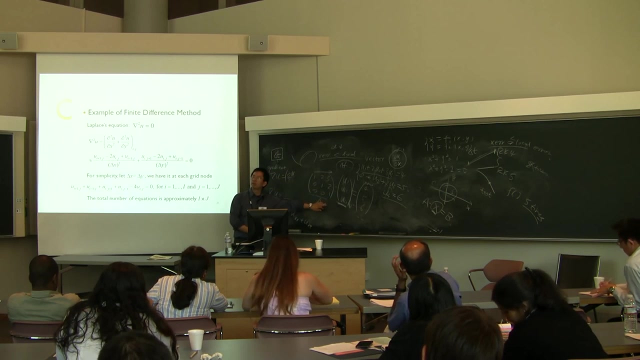 We don't know. That's U yet. However, at each node we can get one equation. In total, I will get- I multiply J- equations, which means hundreds of equations or thousands of equations, And that actually can be right in this form, okay. 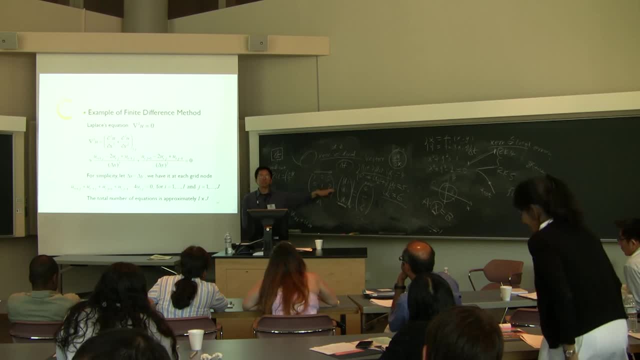 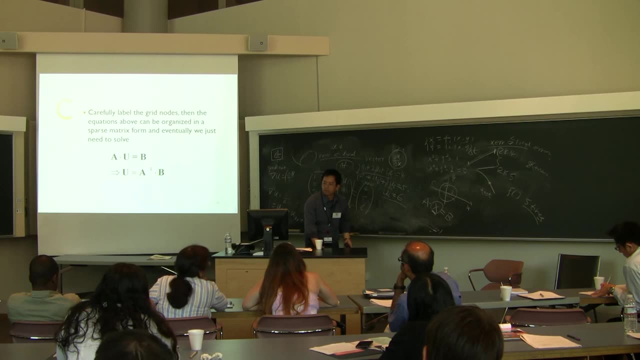 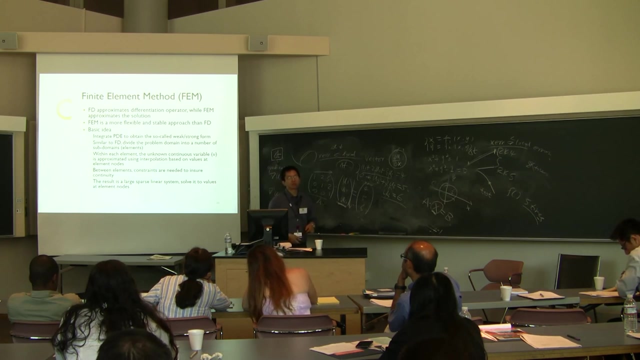 These hundreds of equations eventually will be arranged into this form, And then you solve for the U. okay. So that's a basic idea. However, I personally just don't like the finite difference method, because there's something called the finite element method. okay. 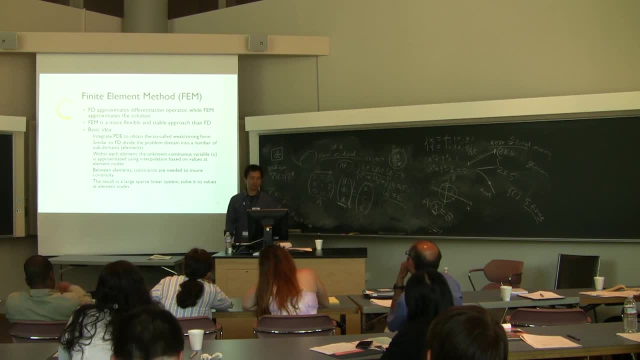 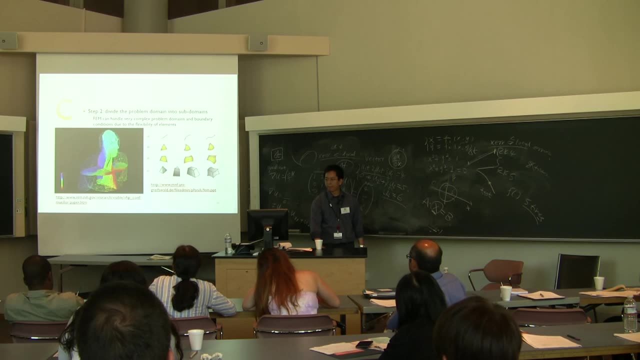 which is way more flexible and stable than the FD method. okay, And again, the finite element method: actually proximate the problem domain, Using something they called elements. That's why they called finite element. okay. For example, here is the model that actually model. 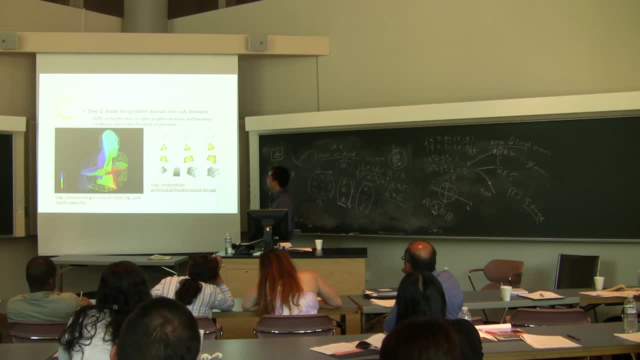 the stress. okay, in the human body. You see a color here. okay, That's a distribution of the stress. And now I use actually the pyramid- okay, element to divide the whole problem domain into smaller elements. okay, thousands of elements. 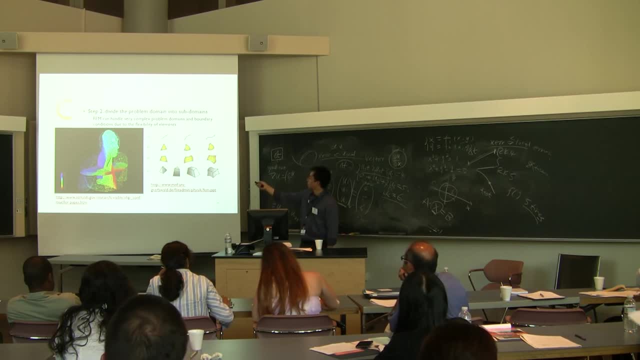 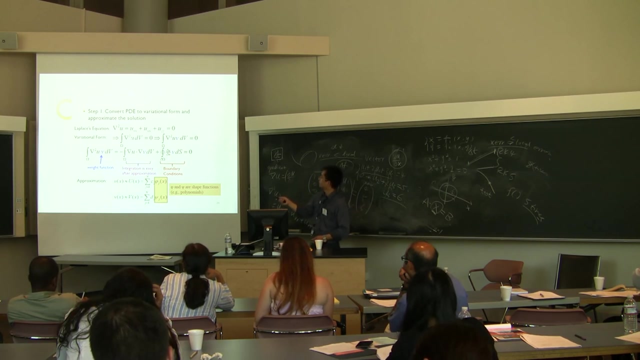 So of course, for different problems you can use different elements. okay, to divide the whole problem domain. And then what I do is not actually like what I did in the finite difference method. Instead of approximate the derivative, okay, 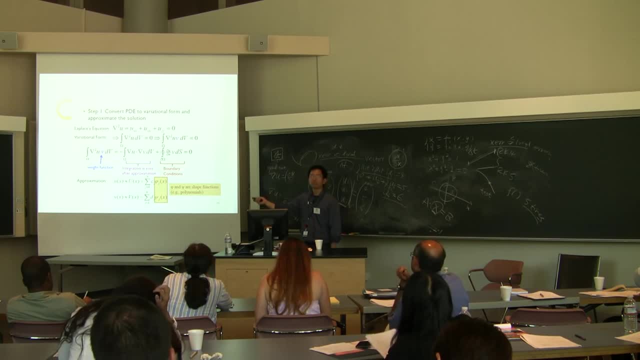 I actually do an integration. okay, I do integration and then use some mathematical techniques. You can actually reduce, sort of reduce, you know, reduce the order of the derivative, okay, by introducing a weight function And this kind of trick. okay, is not important for now. 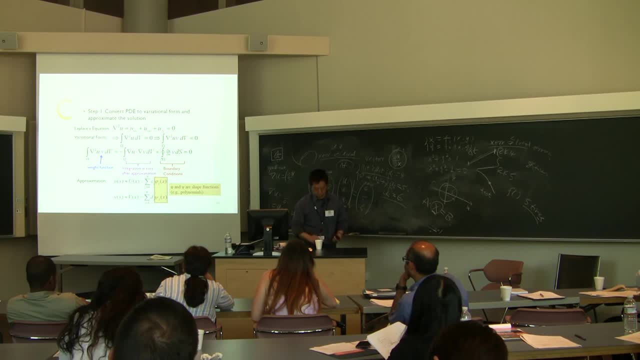 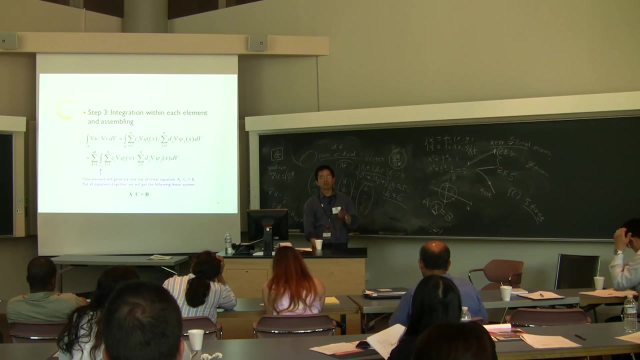 okay, because that's not what we want to learn. okay for now, But eventually I also get this kind of linear system like the finite difference method. okay, There are two different methods, because one method is the FD method, directly approximated the. 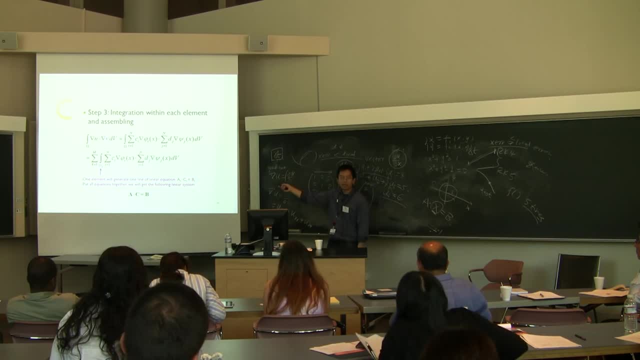 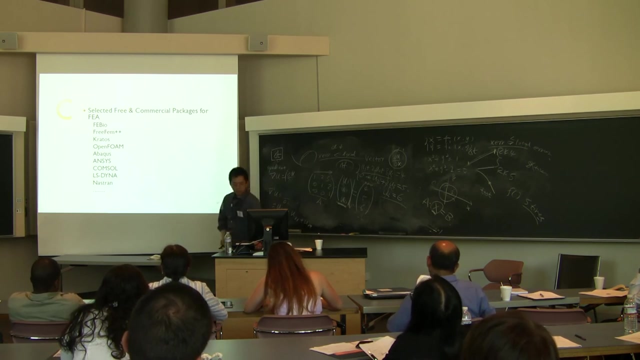 bounded differentiation. okay, operator and this one finite elements method actually do integration. okay, And that's also the reason I talk about integration at the very beginning of this talk. okay, So fortunately okay, like ODEs okay. 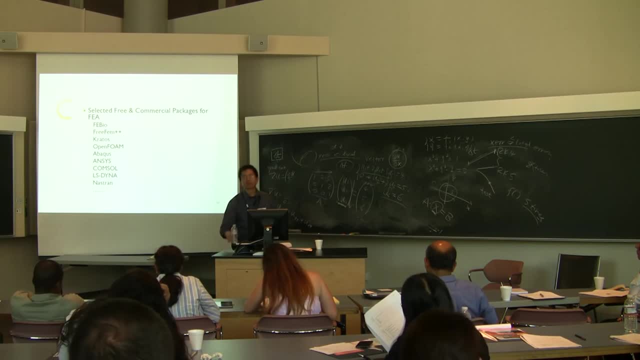 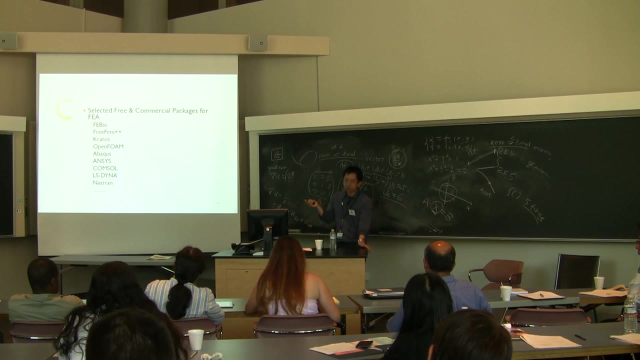 you don't need to struggle with the implementation of FD method or finite elements method. Okay, available packages okay and they can actually deal with very complicated problem. Probably some of you know the FeBio. It's a package designed to simulate the bio tissues. okay, or blood flow. You can use this package And this. 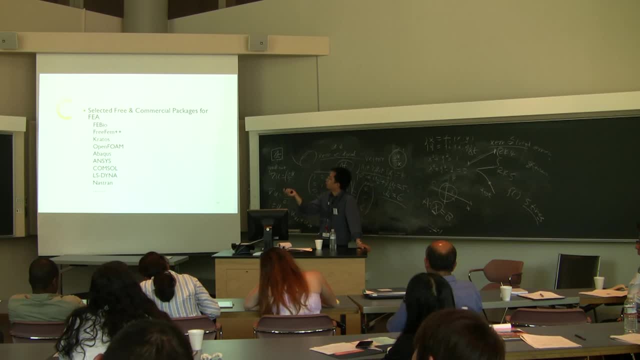 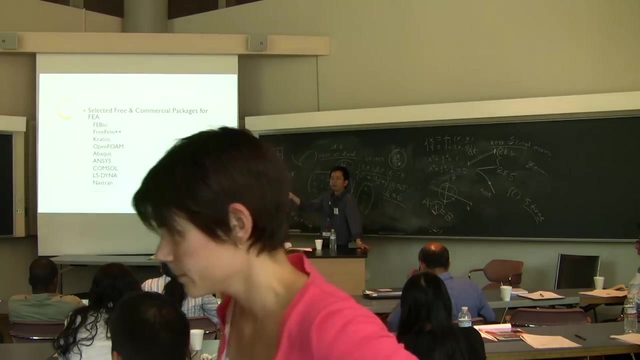 one and this one and this one. they're all free, okay, These four packages are all free, okay, And I think they're all written in C or C++. okay, And here are some commercial packages. okay, If you have the grand money or whatever money. 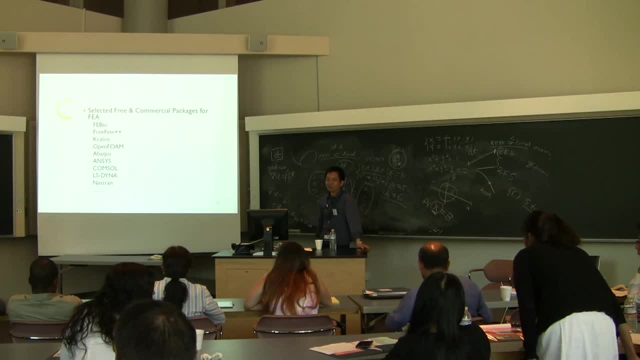 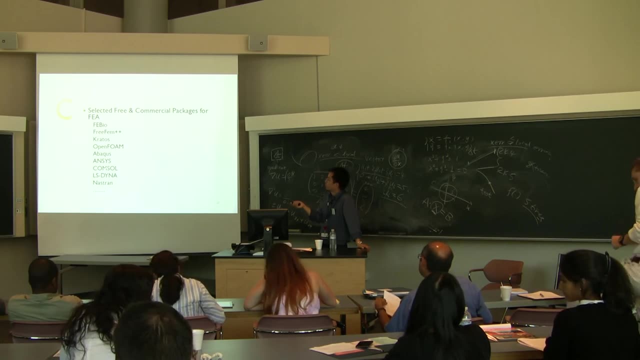 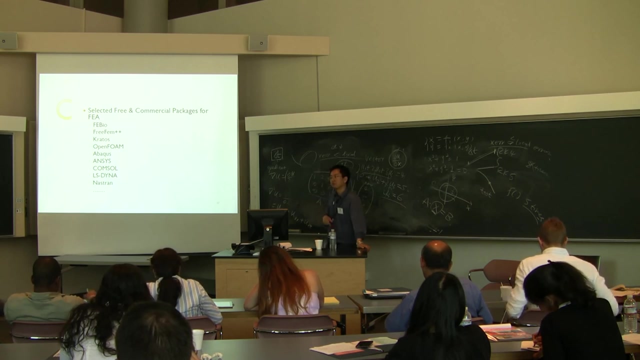 okay to pay for the license. okay, although I have to remind you it's pretty expensive. okay, The package I will recommend actually is something called Comso. Okay, Comso is an amazing package. okay, You can use to model many, many, many. 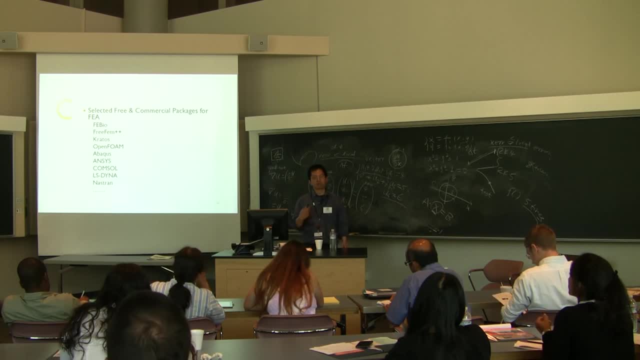 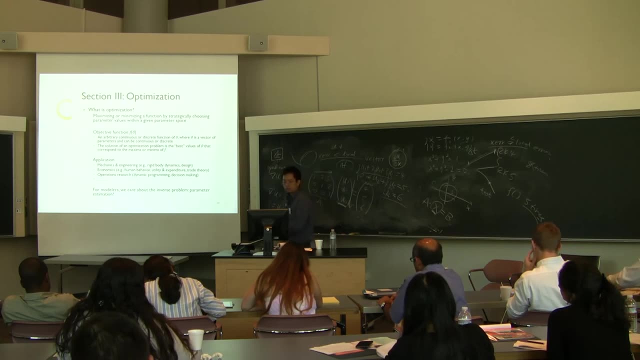 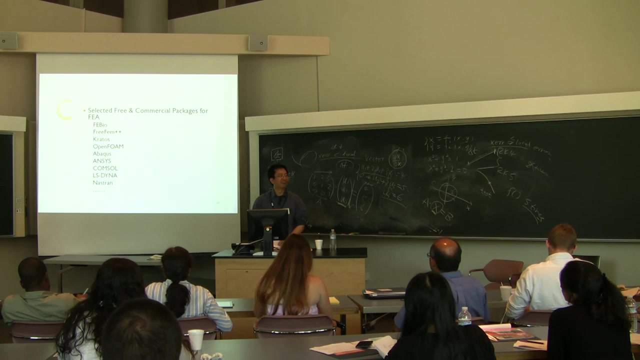 you know dynamic problems, okay, So now let's move away from differential equations, okay? Is that too fast? I had a thought I should have a 10-minute break, but anyway, let's try. I mean two hours, you. 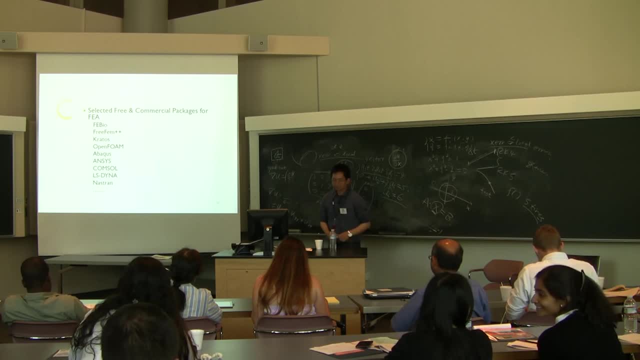 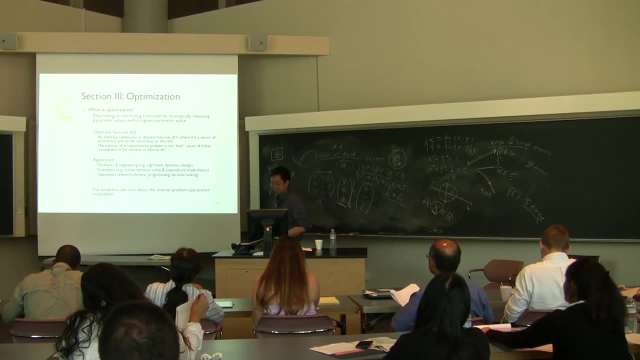 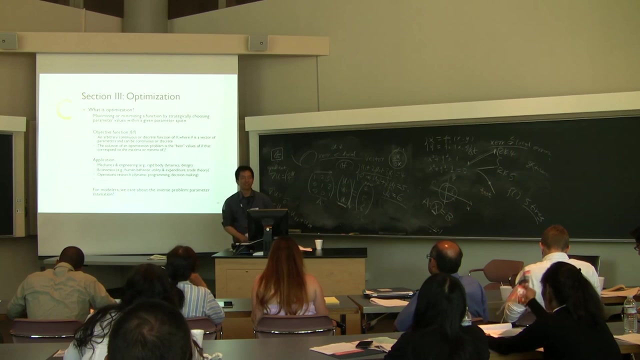 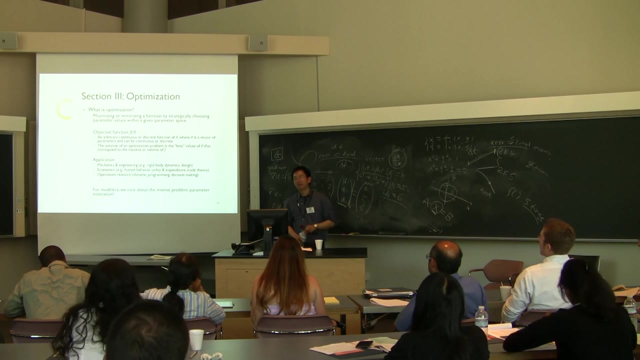 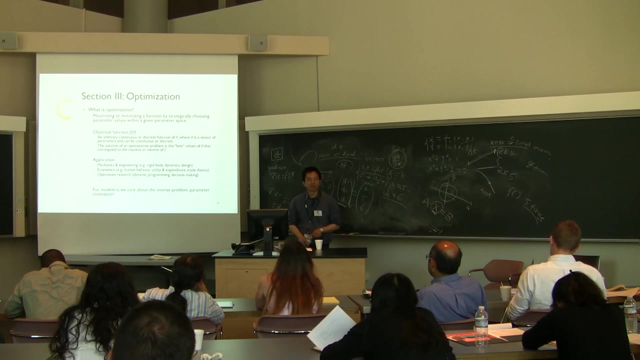 know. So optimization, okay. So what do we mean by optimization? Optimization, because we want to find out the optimal balance between something: optimal cost, which means minimal cost, right. Or we want to maximize the productivity- okay. So optimization means minimization, or. 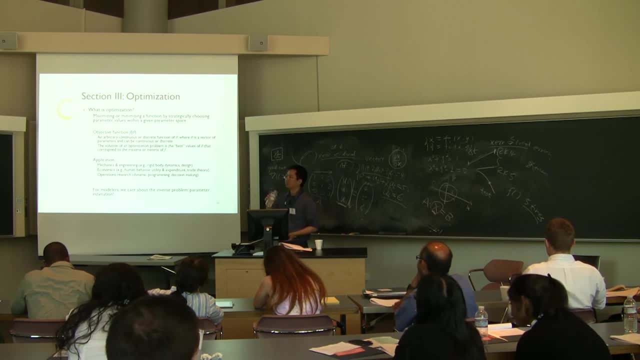 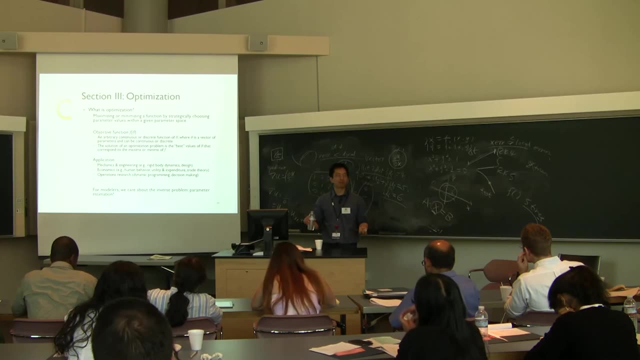 maximization. okay, That's just optimization. So, but to minimize or maximize, you have to have something to minimize and or maximize, right? So what do you want to minimize or maximize? That kind of thing is called objective function. okay, We have a name for that Objective function. So what we want to do to this function is: 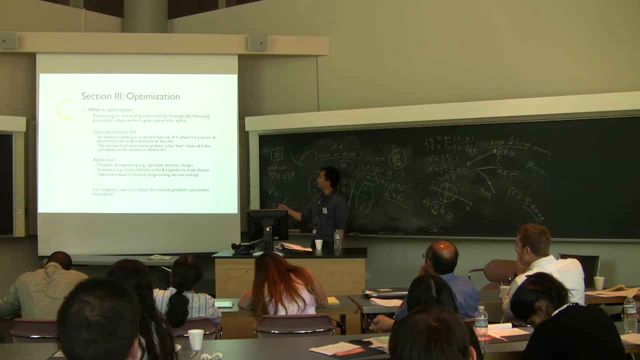 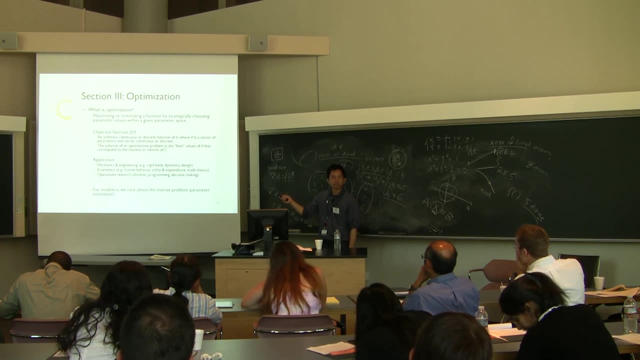 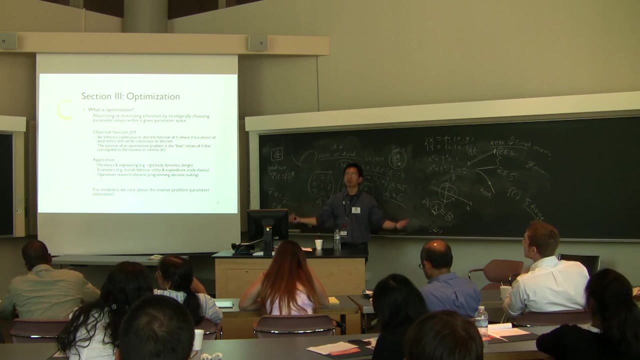 to either minimize or maximize this function by changing or search and best set of parameter value. That's it. For example, we want to know what's the best parameter or best material that I can use to build a house- okay, Given the total amount of money I have, For example, 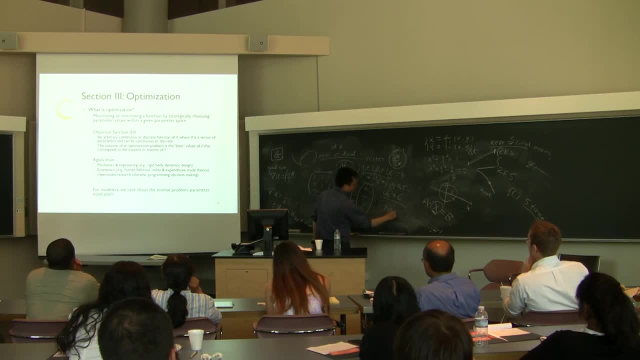 what's the best house I can build, Given 100K? okay. Then you have a model that is, parameters to choose, right? for example, what's the percentage of steels you want to use? what's the percentage of wood you want to use as building blocks, right? so 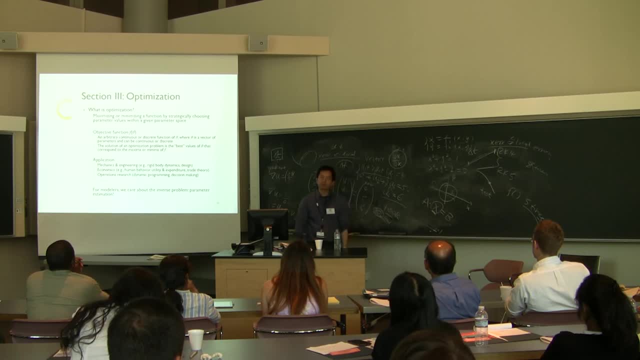 this, this problem: percentage actually becomes your parameter. okay for our problem. okay for modelers. okay, what we really care about is so called model fitting. okay, we don't care about our other things. okay, we care about model fitting. which means: how can I infer parameter values from data, given the 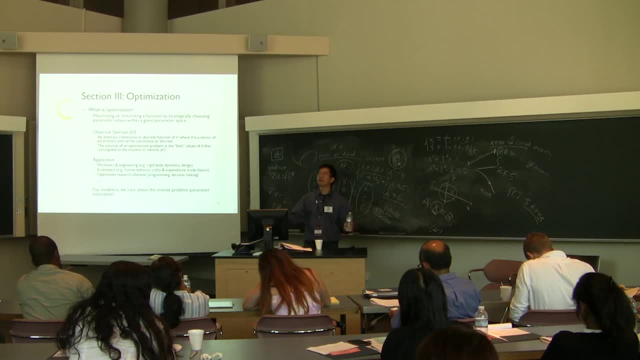 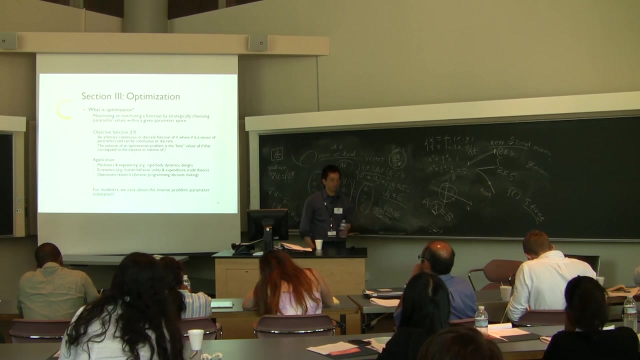 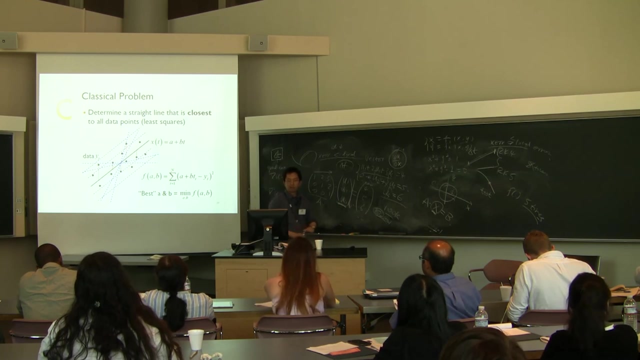 model structure. okay, what's the best parameter values that I can best have my model prediction be closest to my data? okay, if I interpret the optimization problem in this way? way, okay, so here is a typical problem of optimization. it's called least squares. how many of you have heard but least squares before? okay, 50% approximately. so 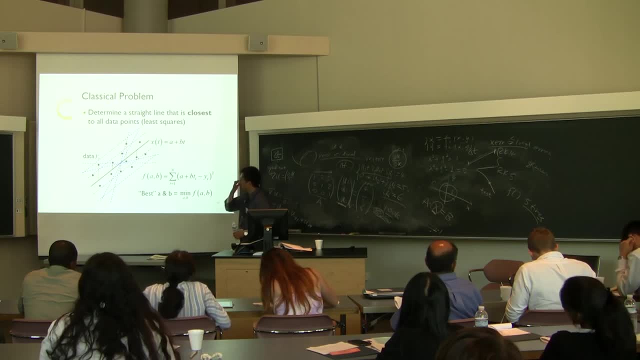 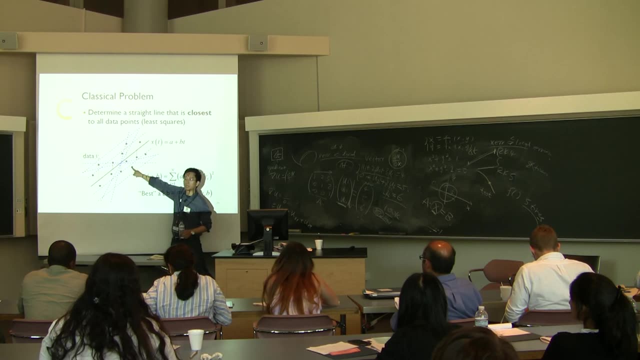 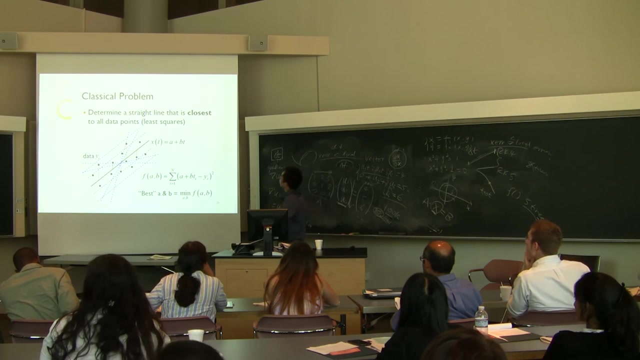 there what's least squares, least squares, which I use a simple example to explain: okay, if I have a bunch of data points with black dots, okay, and now my goal is to find out a straight line that is closed to all the data points. okay, not to just one single data point. okay, I want a straight line that is close to 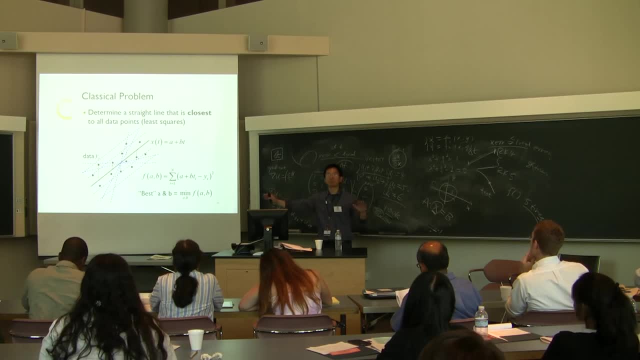 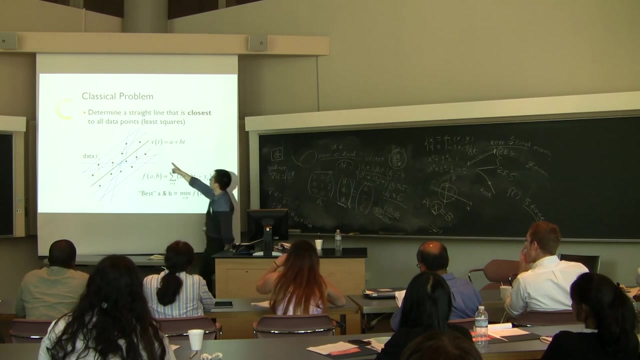 all their points. okay, which means this line fit my data the best. now, how many possible, how many possible candidate straight lines are there? I can have infinite number, right? I can draw a straight line here. right, I can draw a straight line here, here, here, here, okay. 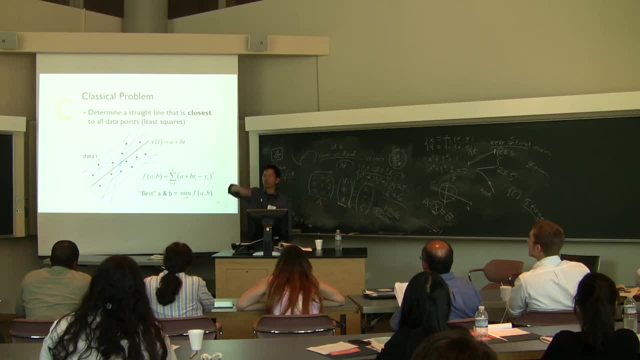 So I shift it okay in the vertical direction. I can also rotate the straight line right, Change the angle, change the slope, So I can have actually infinite number of straight lines that can describe the data. However, there's only one line. 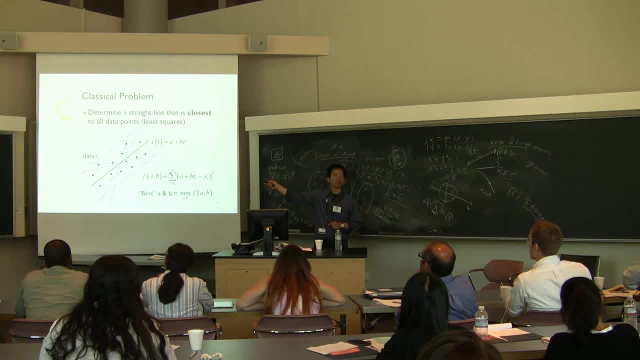 that is closed to all data points, And what we're trying to do is find out that straight line okay. So what we do is actually that we actually we know that we can use A plus Bt to actually model a straight line, right. 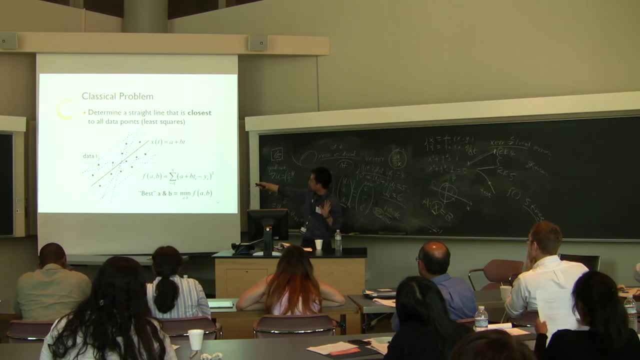 That should be. that would be the first agreement we should have, right? Okay, Okay, Okay. We are saying we have to use a different model. okay, to model a straight line, Then we are in a different universe. okay. 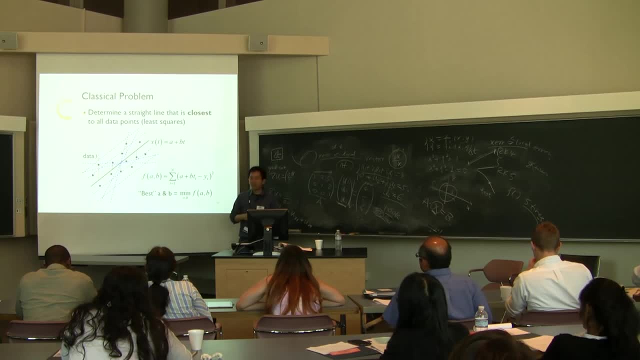 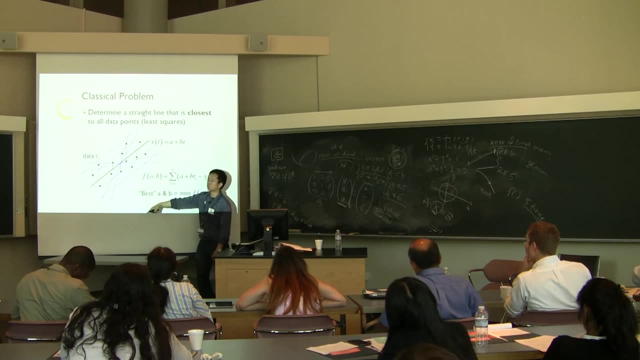 So, but anyway, use A and Bt. okay, We can describe a straight line. So what we want to find out is what's the value of A and what's the value of B, that I can actually draw a straight line that is closed to all data points. 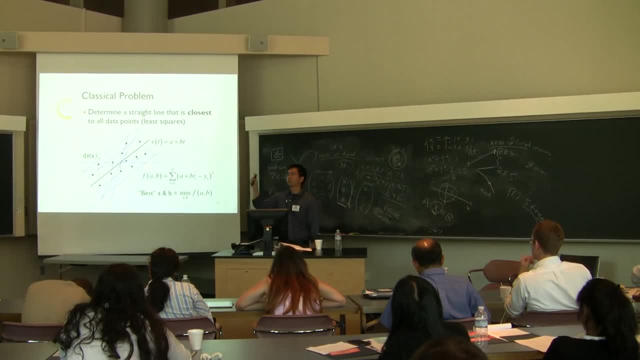 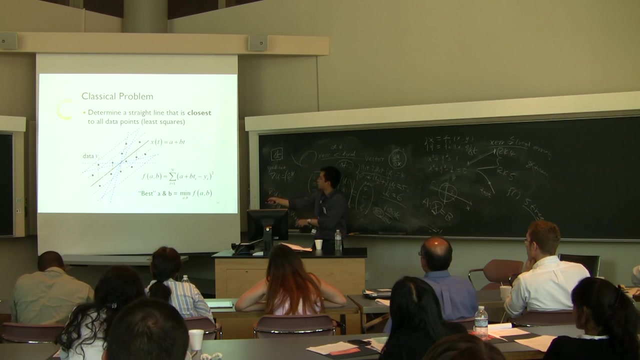 So now I have to define an objective function right To minimize or maximize. So here, since I'm talking about closed, so I want to minimize some function right. So minimize what? Minimize the distance from the data points to the straight line. 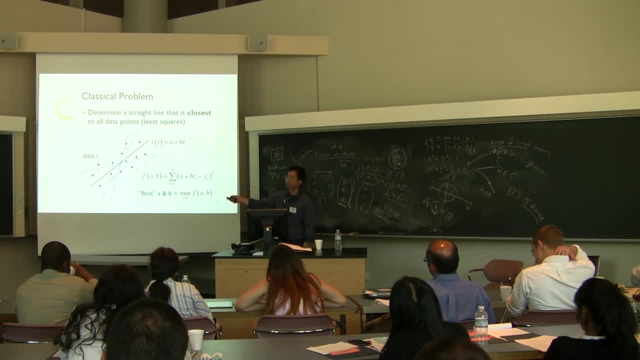 Okay. So what's the distance from the data point to the straight line? So here to here, that's distance. right, So here to here, that's distance. So all this, you know, red dashed line, they're actually distance. 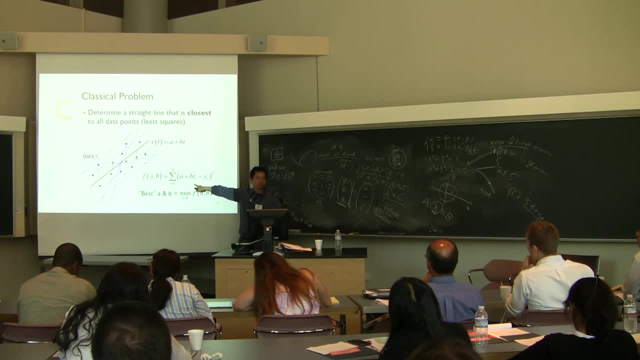 So now, if in mathematics, okay, the distance actually is, this is a straight line. Subtract the data: okay, Yi, here is our data. I use a notation of Yi, So this is a value on the line right. This is a value on the line A plus Bti, okay. 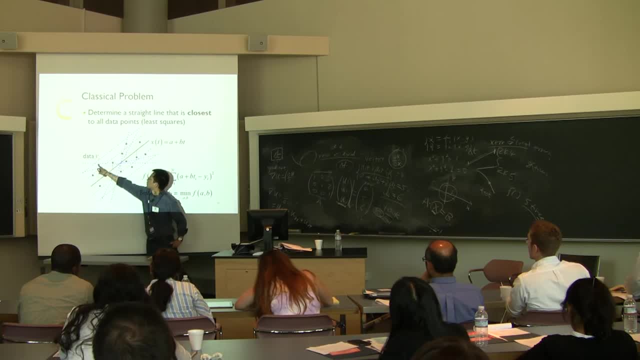 This is a value on the line, This is the data. So I subtract these two, Subtract one from another, Negative, So this is the distance right, And then I put a square there. So this distance can be positive, can be negative. 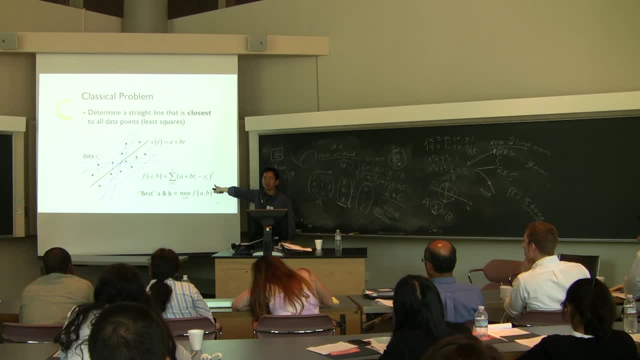 but after I put a square there, the square will be always positive, right? So now I'm okay to minimize it. Minimize this function and then you will get the best A and B you want. So that's called, at least, square, okay. 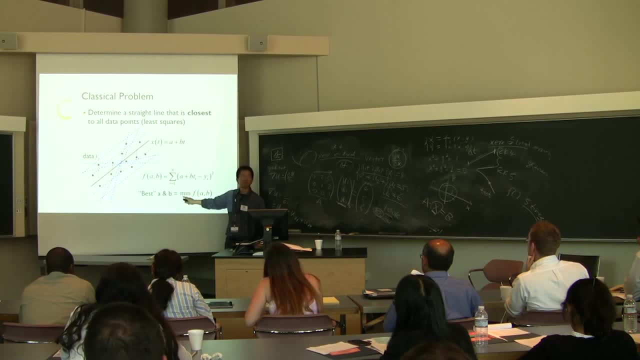 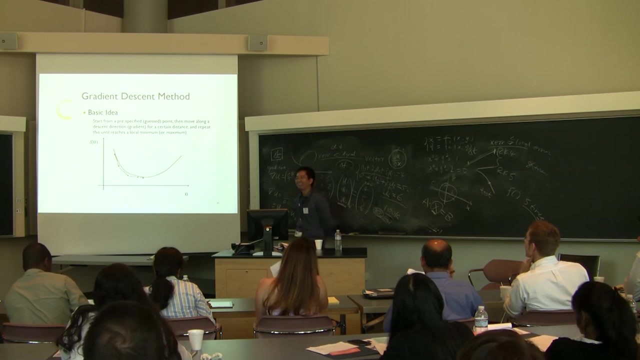 Square. Square part is here, Least part is here. It's called least square. okay, So is that clear Question Good? No question is good. So now let's talk about, okay, how to actually find out the best A and B. 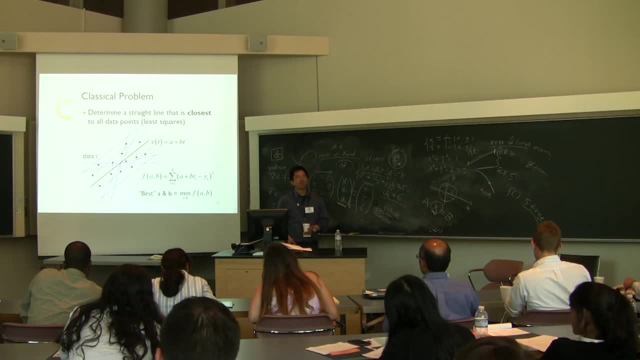 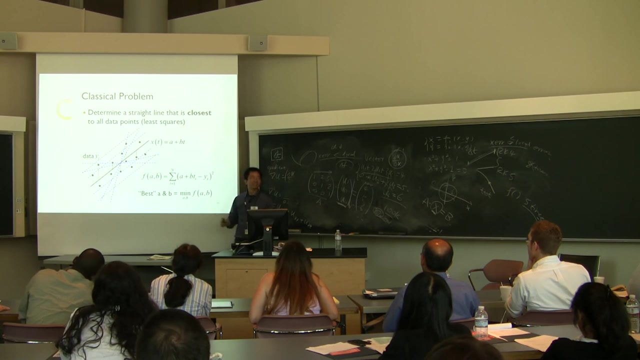 So one brute force method will be. what will be the brute force method? I just try many different A and B right And I compare them and I find out the minimum one right. So, for example, I can generate: 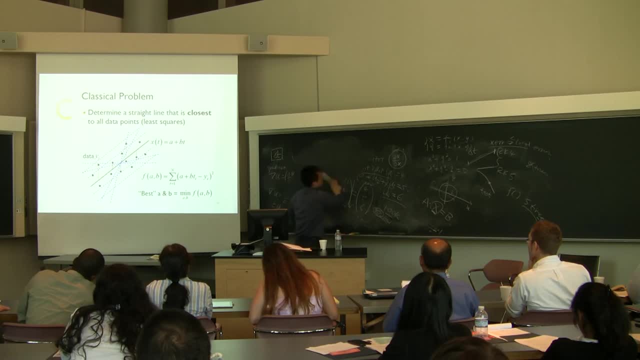 let a computer generate a list of A and B. I can let A and B, and here's my F A B. I can have a one, two, one point, one, two, one point, two, two, Two, two, two right. 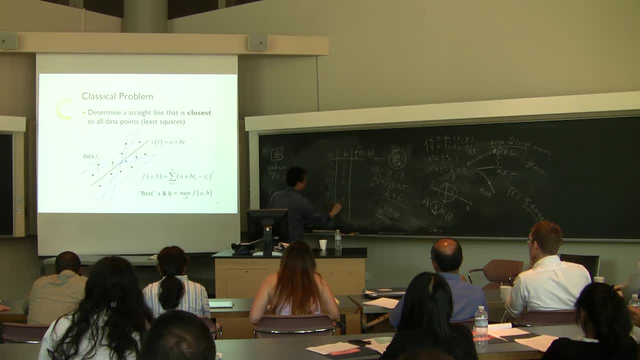 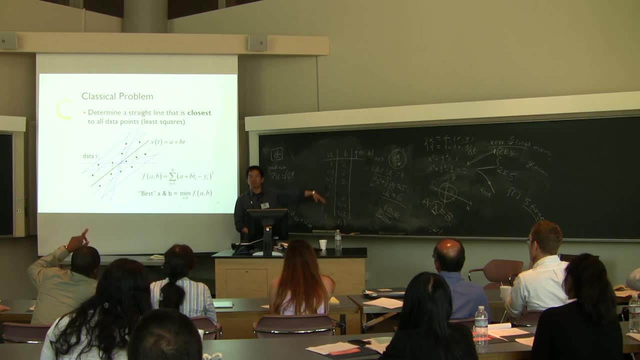 I can have a one, one point one, one, one point two, one point three. I can plug in many different pairs of values into this function. Okay, Okay, In these squares, are you determining the distance from the dot to the line? 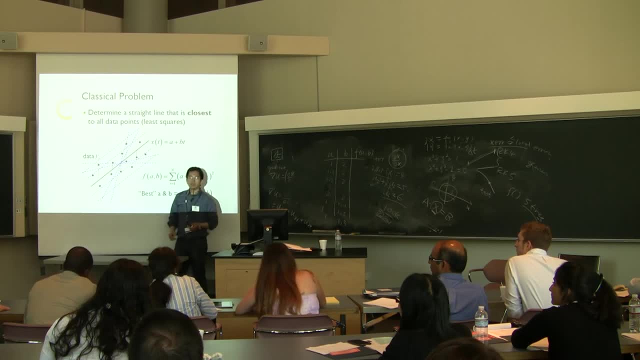 is it the closest distance from the dot to the line in terms of perpendicularity, or just you're just going to be? it has to be. for this case it has to be not perpendicularity, It's just in a vertical direction. 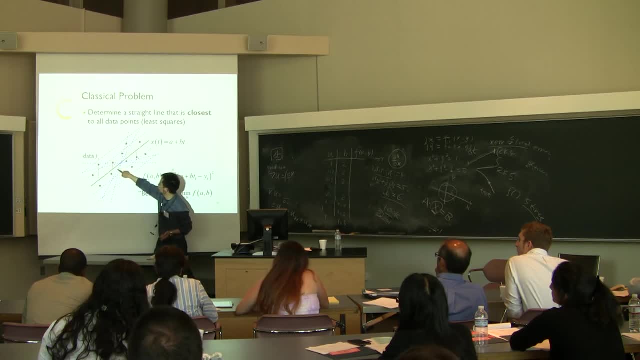 Okay, It's in a vertical direction. It's not perpendicular. Perpendicular will be in this direction. Okay, Here now we only calculated the distance in the y-axis. Okay, All right. So because we assume the distance in the x-axis actually is t here. 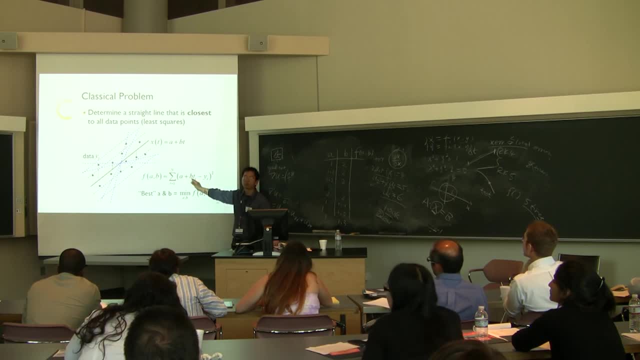 We, we, we fully specify the t, so we don't want to bother to you know. you know, include this one into the distance. Okay, So you only calculate the, the vertical, okay, distance. So now let's talk about how to find out a and b. 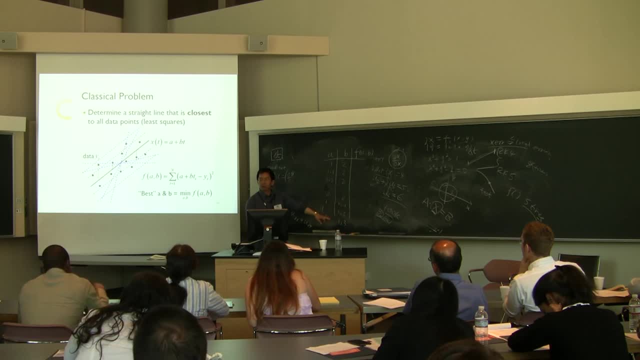 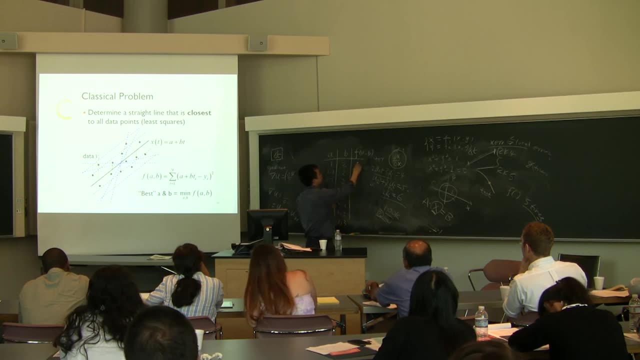 Okay, I can generate this table, Okay, Okay, And plug this number, the parameter values, into the function. Probably, this one, I get a five, this one, I get a 10,. this one, I get a one, this one, I get a 30,, 30,, whatever. 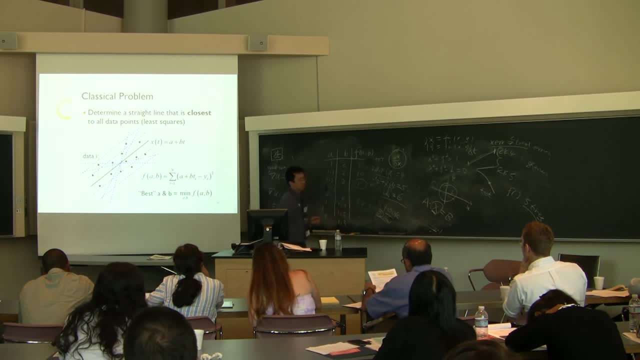 Now I compare them, Because this one gives gives me the smallest value. Okay, I think. okay, my parameter should be 1.2 and 2.. Okay, Let's minimize this function Right. However, this method is stupid. 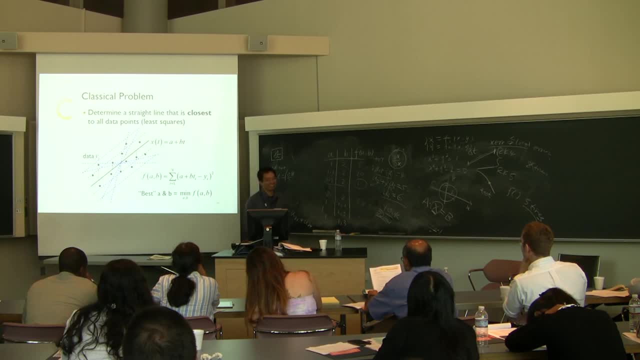 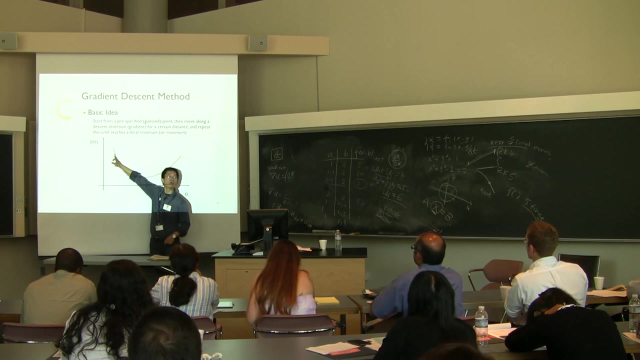 Right, Because there are infinite combinations. you have to try to figure out The answer. Okay, That's why people derive this, the so-called gradient descent method, This kind of a. so the idea is, if I move from one starting point, okay. 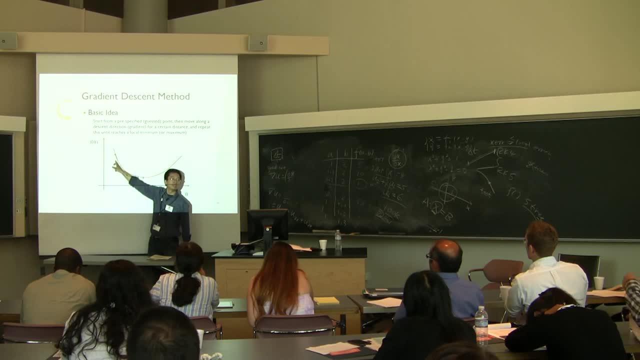 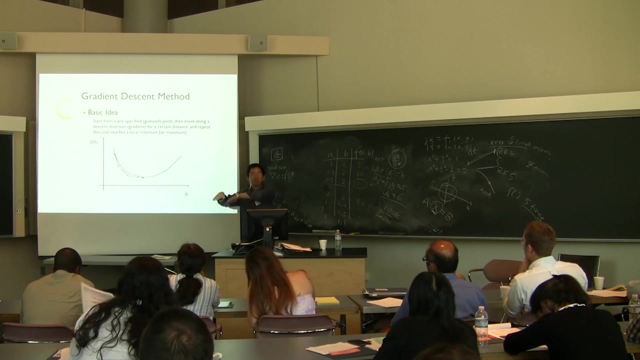 because here the slope is negative. right, the slope here is negative, So I just move along the slope direction, So I decrease the value a little bit. Right, Because right now I want to minimize my object function, So I will move along a direction that leads to a smaller object function value. 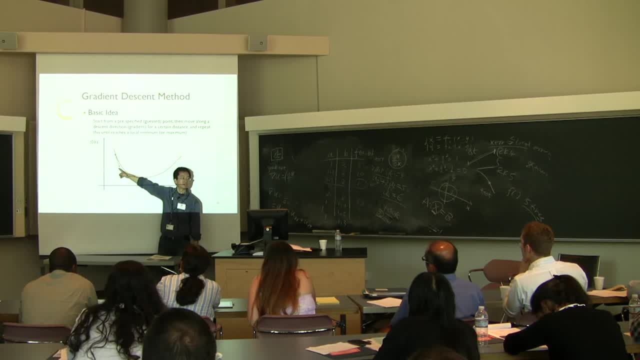 So now I move along this direction. That makes sense right Now. I start I from here, I get to here And my object function value becomes smaller Again. I start from here and move a little. Does that look? does that look like the ODE solver? 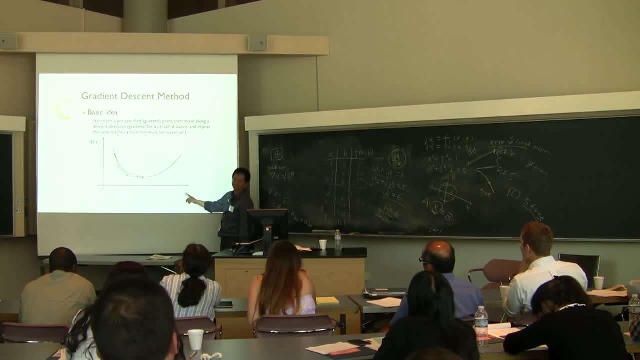 A little bit right. Okay So, but now the independent variable is theta. okay, instead of f, instead of t, okay, So, actually, that's exactly the same idea. okay With solver ODE. we start from one to the next. 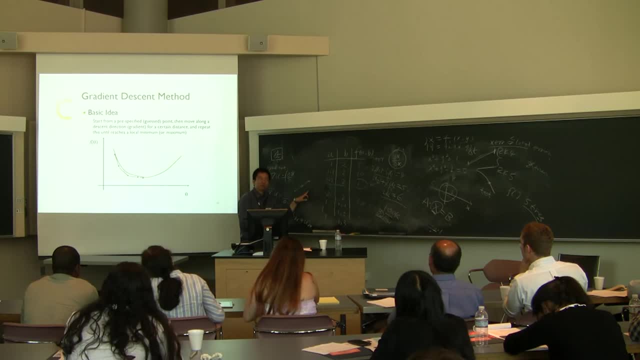 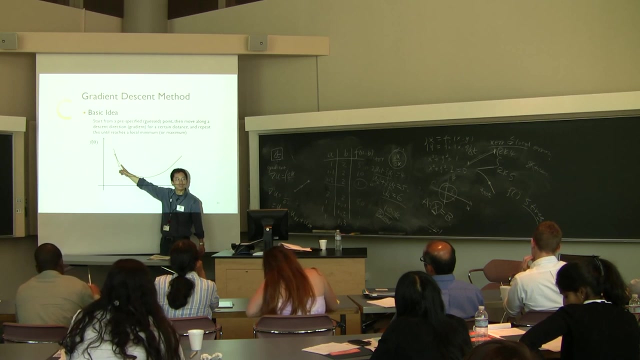 by calculating the slope. right After we calculate the slope, we move along the direction of the slope and get the next point. Here's the same thing. I move in a slope in this direction because the slope is negative. I do not move in this direction. 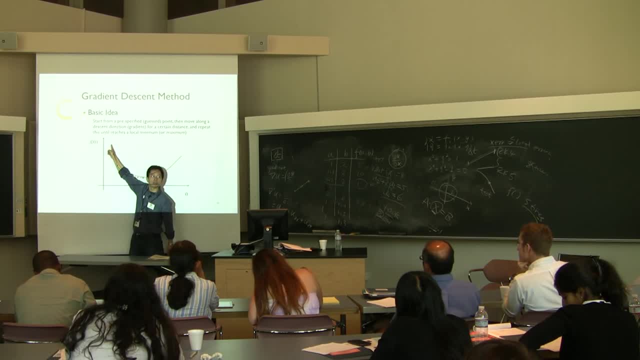 because if I move in this direction, that will increase my object function value. So you know, this direction will lead to a smaller object function value. That's why you move in this direction And I do the same thing here, do the same thing here. 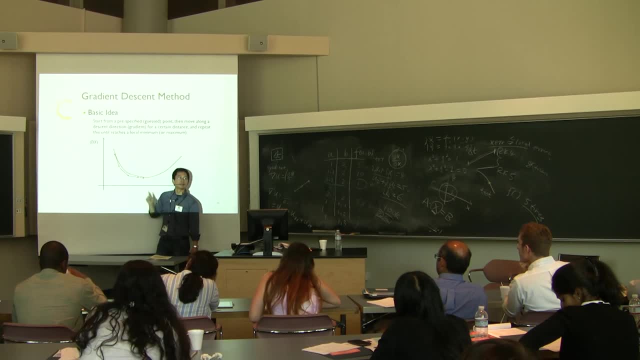 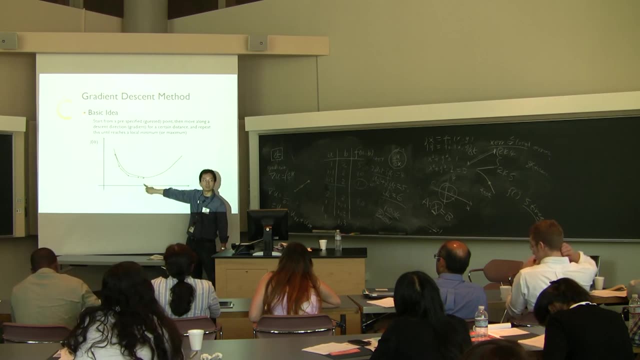 Eventually I got to the nadir. okay, That will be the point I want. okay, So my best parameter value actually corresponds to the nadir. okay, in the object function curve. Does that make sense? That's the basic idea, okay. 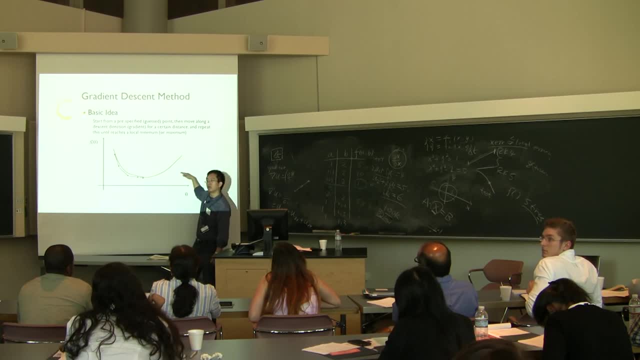 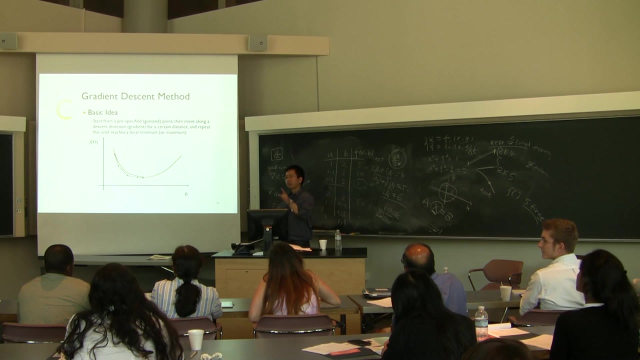 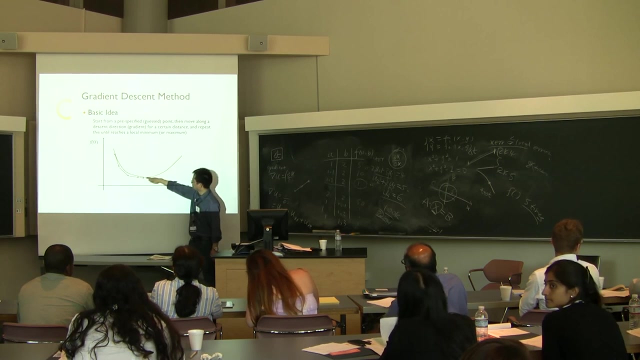 You want to draw a horizontal line. What, What, Where the slope will be your t, Where the slope will be your t. That's true, That's very true actually. So if you have not just this one, okay. 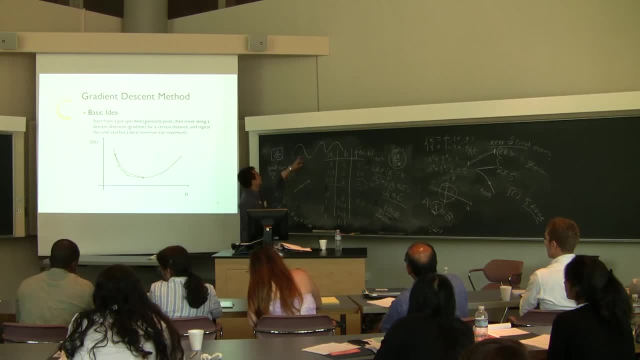 an arbitrary curve, okay. the minimum and the maximum always occur at places like here, here, here, here. And one common property of this point is that the derivative here, the slope at these places, are always zero, Because if you draw the tangent line, okay. 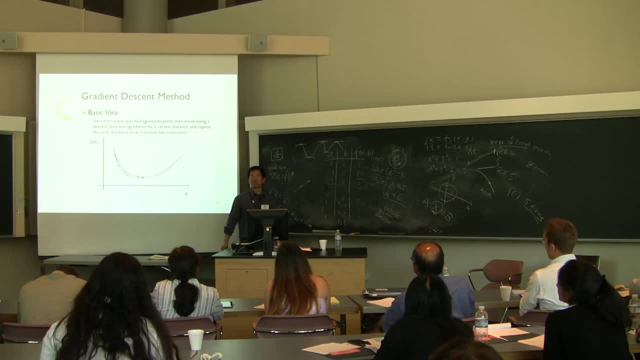 you actually get this. But the problem is, if I have multiple this kind of points, which one you want to choose? Right Here I just do a simple case. This one has only one, you know place that has a zero slope. 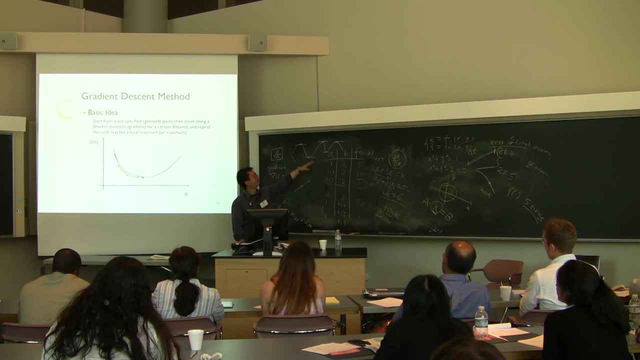 But this one. if I have multiple, you know zero slopes. you solve this equation. but you get a multiple solution. You have to choose one, right? So this will be the so-called gradient measure. Okay, you start from one point. 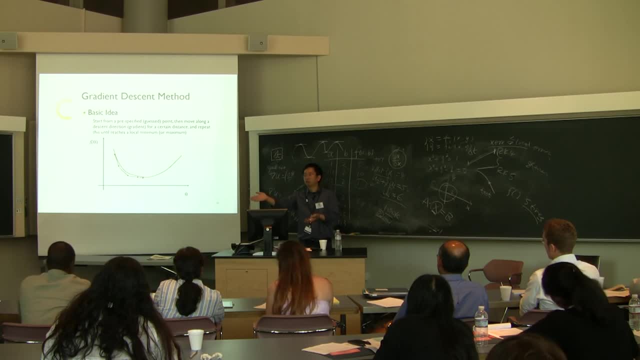 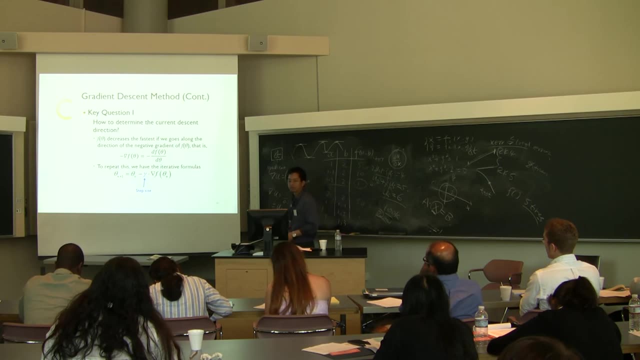 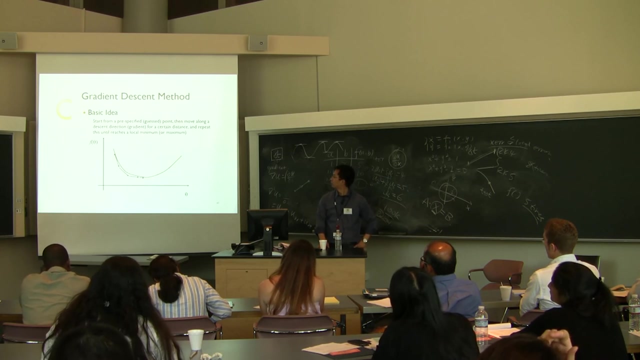 then move along, move in a favorable direction, And then you search the minimum. The key problem is that. so what's the problem? you can tell okay from this plot. The first problem is: where should I start? Right, How about I start here? 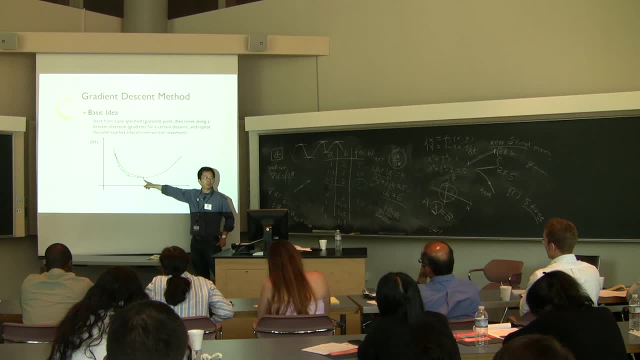 When I just move, one move once, I get a solution. But do we know where to start beforehand? No, we don't okay. You only okay for the problem we have. We don't know where to start. 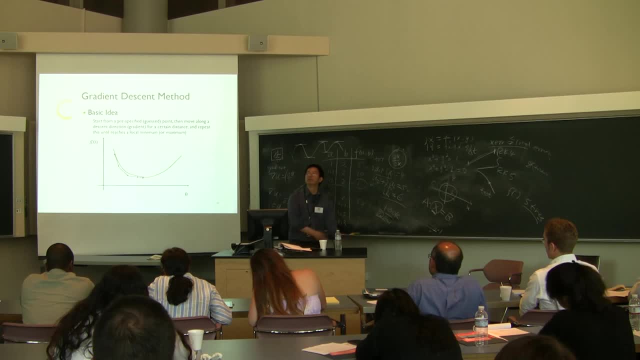 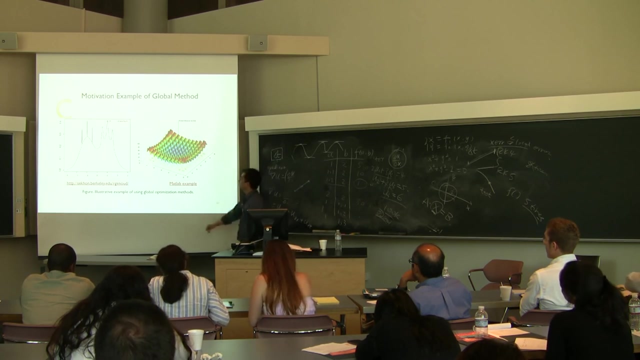 We have to guess. okay. That's the biggest problem for this kind of method. If my guess is wrong or too far away from this solution, you get into trouble. Okay, For example here: okay, This is actually a real object function. okay. 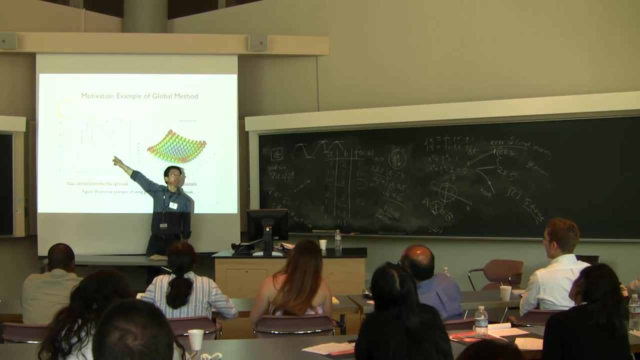 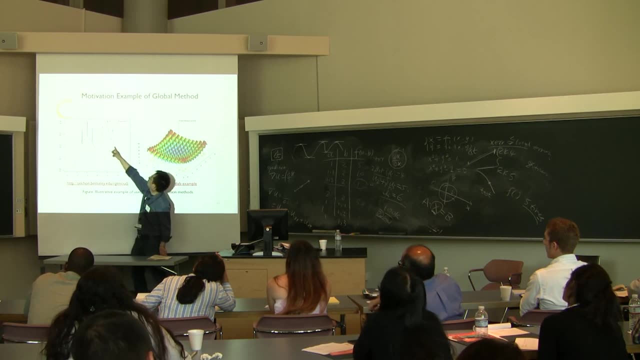 If I start from here, Let's say here I want the maximize, okay, maximize my optical function. If I start from here, then follow the gradient direction. I probably will just stop here, right, I will not move away from this point anymore. 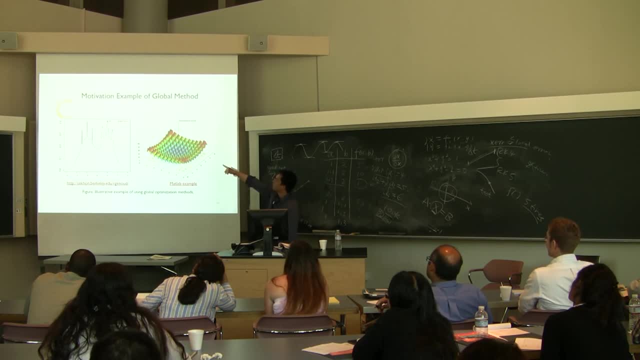 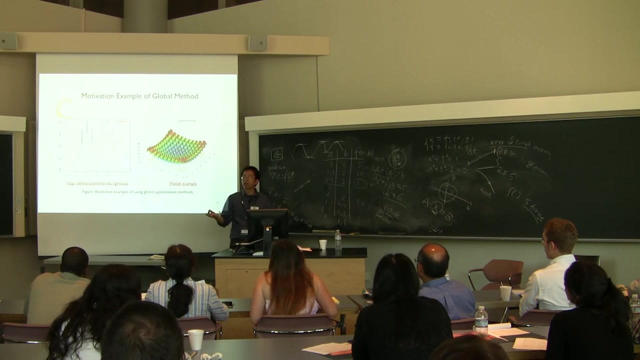 Because- Yes, Because I think that's already my answer- The gradient method will take that one as the answer. Okay, it will not search for a better solution. Okay, once it reaches a local minima or maxima. So that's the same problem here. 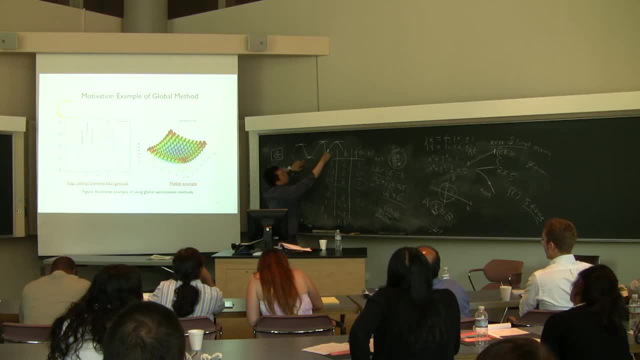 If I, if the true solution is here and but if I just start from here, I go along in this direction and then I get this solution, then the gradient method will stop here. It will not move anymore. Okay, once it finds a local minima. 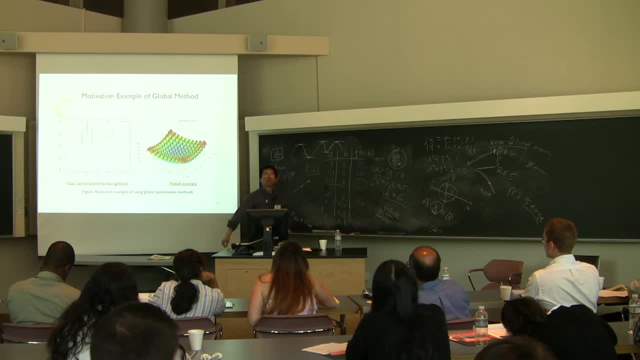 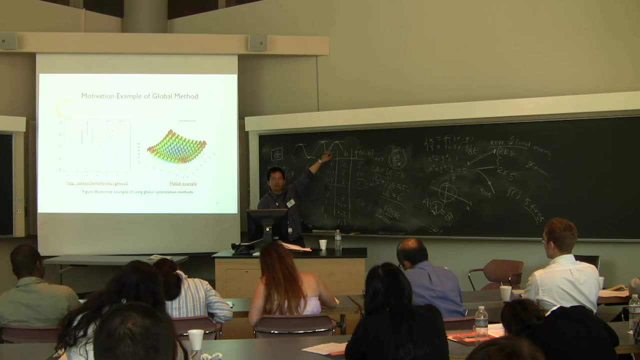 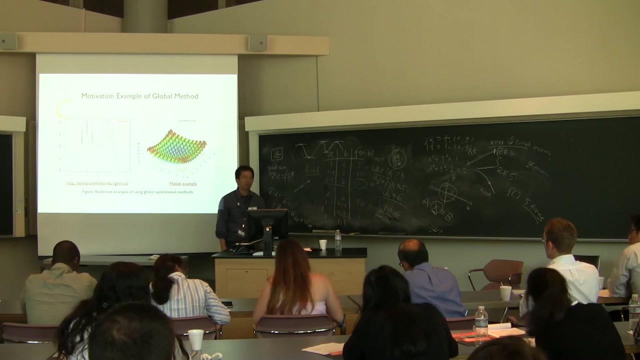 So gradient method is a local method. okay, If you, if your guess is far away from the true solution, you will get a wrong answer. And how did you find the global minima? Thank you for that question, because this is a motivation, okay. 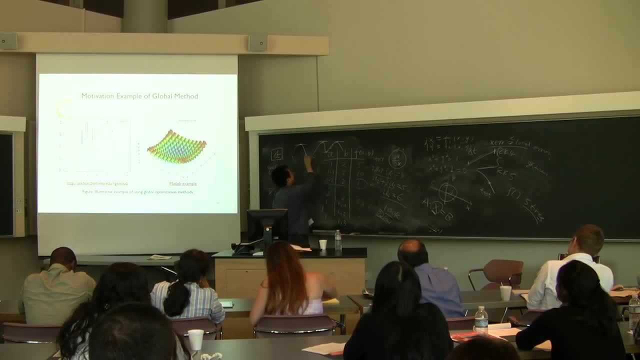 for the global method. okay. So we want to find the global solution, okay, instead of a local solution. So this is another example. okay, you can actually check the help file in my lab. okay, It has an object function that has this many bumps. 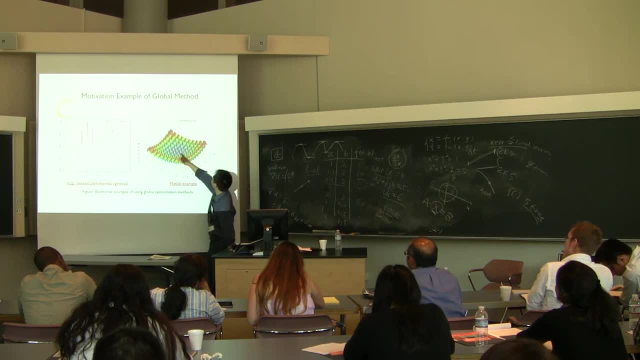 and you know, and the true solution actually is here: Okay, if you start from here, you never. actually, if you use the gradient method, you will never get from here to here. okay, That's why people actually developed the so-called 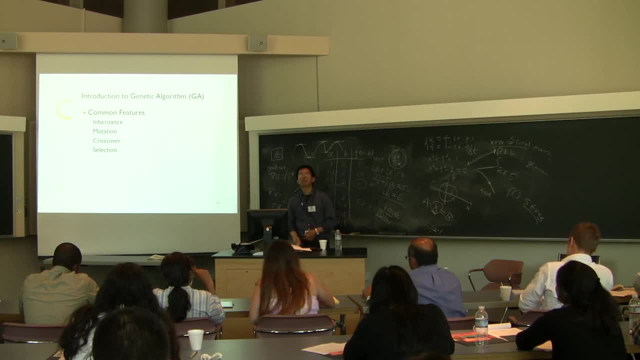 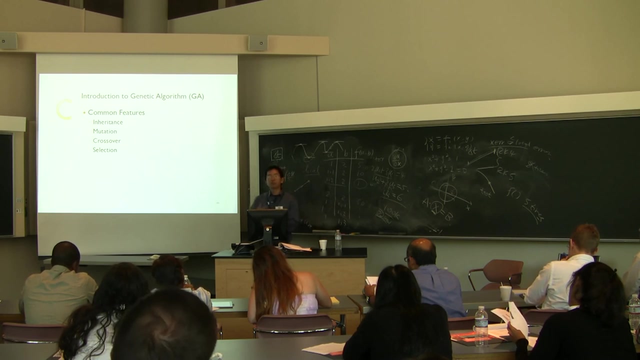 global method, global optimization method. One typical algorithm is called a genetic algorithm. I think all of you should have heard about it. okay, before genetic algorithm. So the genetic algorithm actually mimic the evolution of a genes. okay, That's how it works. 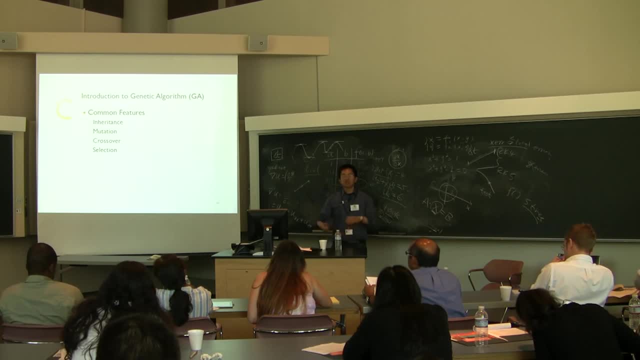 So you have four steps. The first step is the inheritance, which means the next generation, or the children or parents, is already free of inheritance. tenho a PhD in it. That is the result. у насur jaét, у насur, je мıs entend которую. 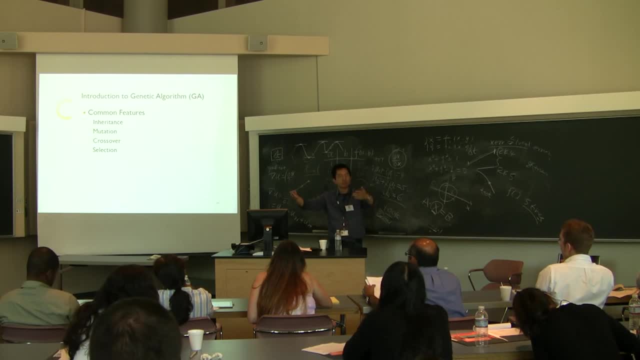 children will be generated from the parents. okay, That's called inheritance. And the second step is called mutation, which means the genes of the children will be mutated, so they will be different from the genes of the parents, or they're not exactly the same, right? 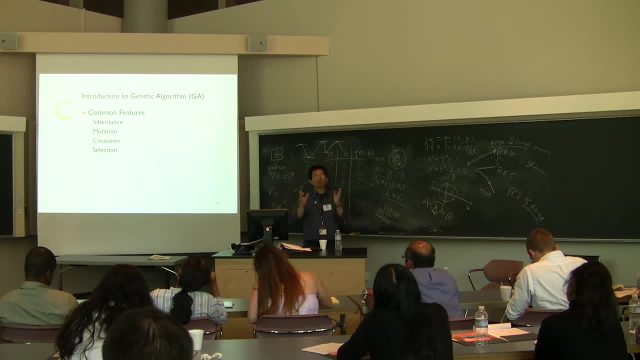 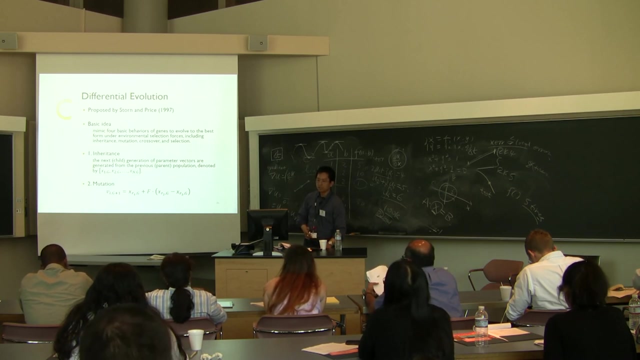 The third one is crossover, which means after mutation by the selection force, you may keep some of the mutation, but you may just keep the genes from your parents, okay. So you have a crossover, And the last one is selection. So 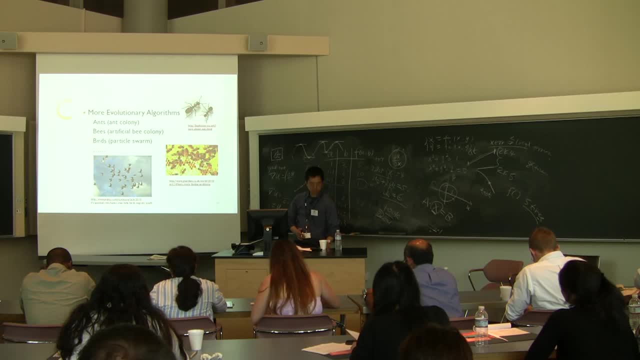 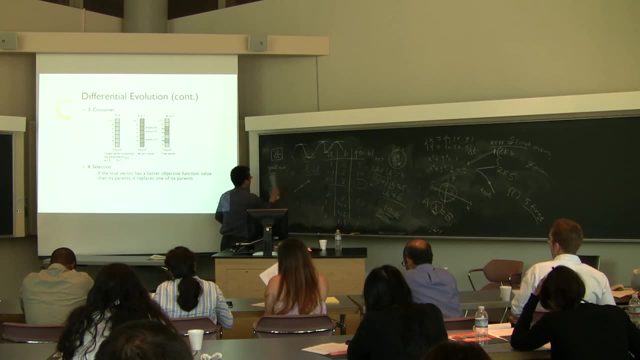 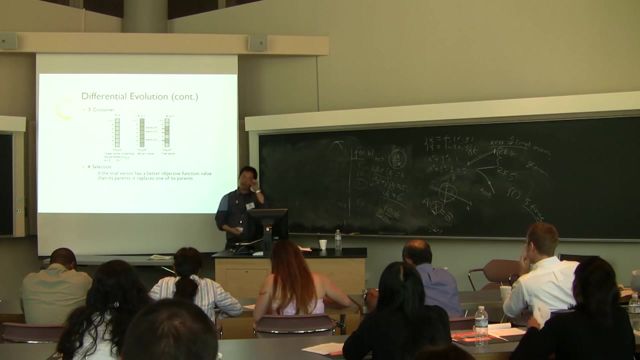 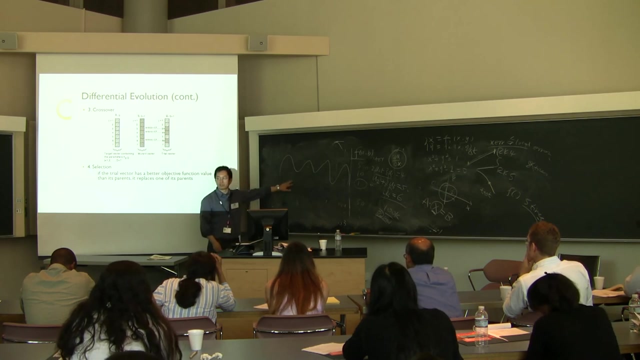 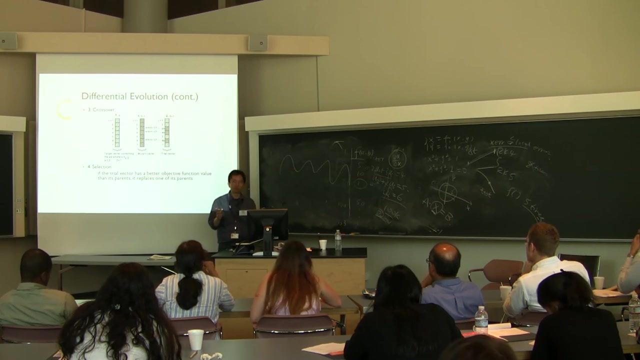 let's skip the technical details, okay, And then instead I want to actually draw a plot to explain why this genetic algorithm can find the global solution. okay, So I still have object function like this, okay, Now, instead of start from one particular point, 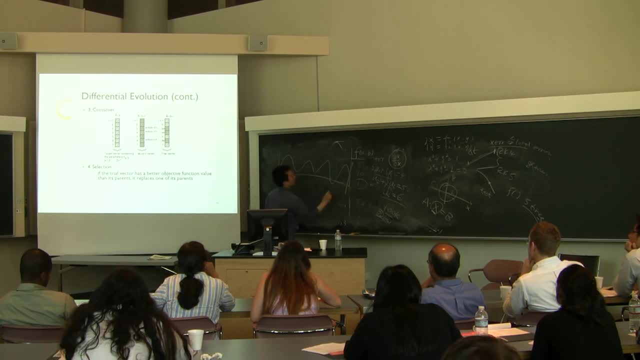 I will randomly generate many points spread out. okay, For example, I put points everywhere. For example, if I allow one hundred search agents, okay, Let's call this point search agents, because they are searching the global solution. okay, So let's call this point search agent. 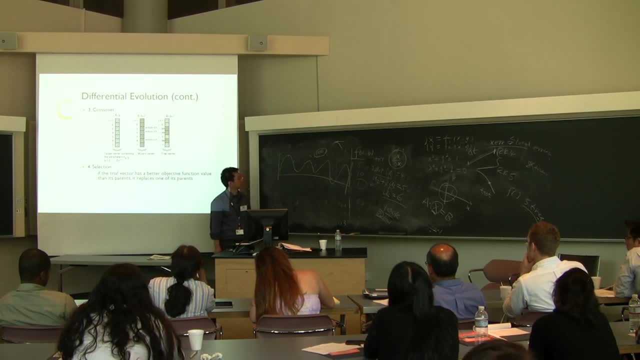 So I let this search agent spread out, okay, In the whole parameter space. okay, You can do this easily by generating uniform, distributed random numbers. okay, You can do the first step. Then you will say: okay, now I have many starting point. 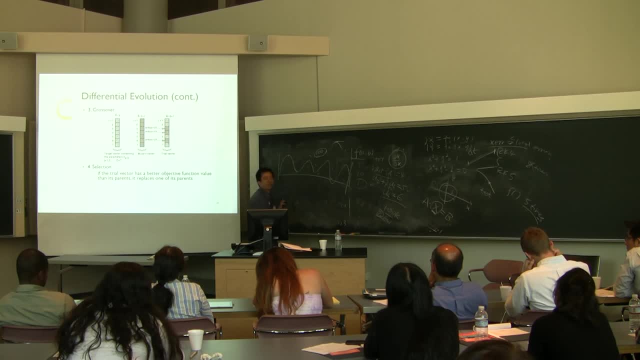 okay, then I, one of them, will. I can move along the direction and get to the global solution. okay, That's a good, that's actually a good wish. okay, The problem is, if you have a function like this, okay, 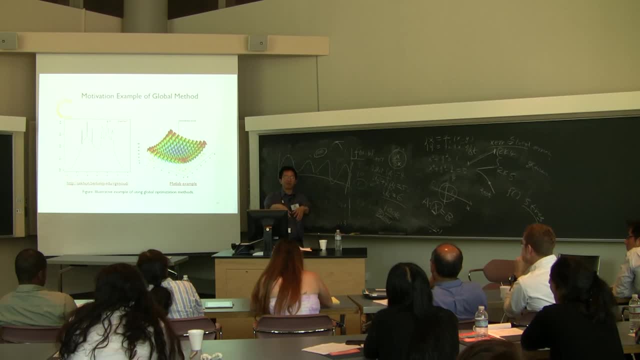 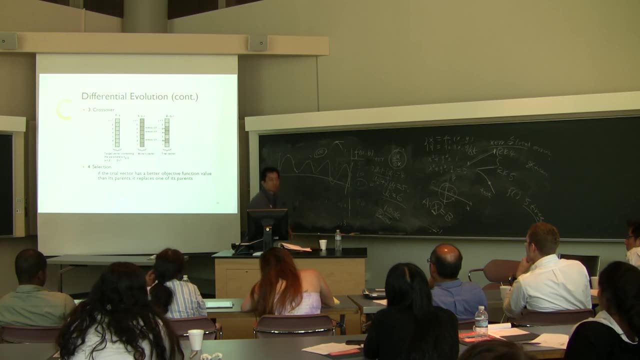 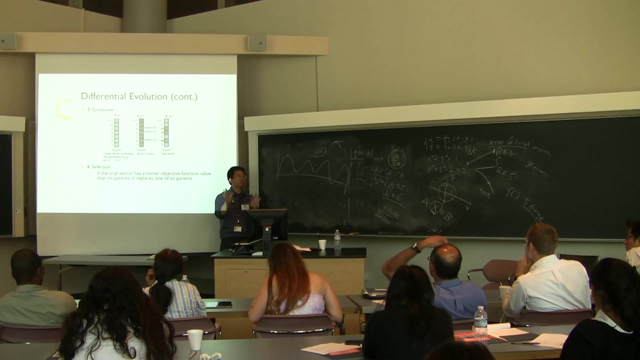 Most of your searcher agents were stuck by the local minima. okay, You still will not have a global solution. So the solution actually is we need a certain strategies. okay, To explore the whole parameter space. okay, Instead of randomly. okay, let them, you know, search. 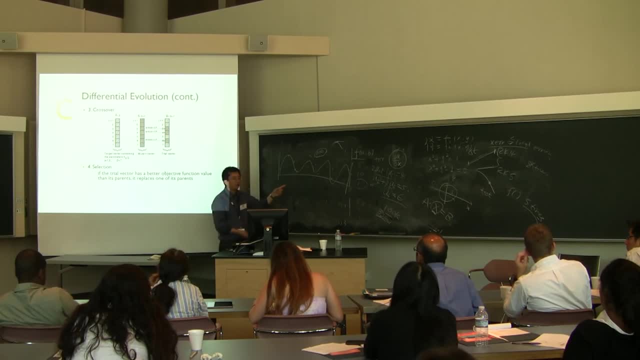 we need some strategy, okay. So strategy is that I, after I put a, generate the initial search agents. okay, I generate the next generation. okay, So I generate the next generation of agents. They are children of the previous generation. 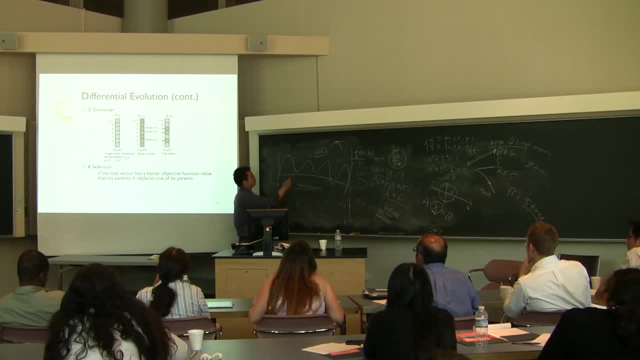 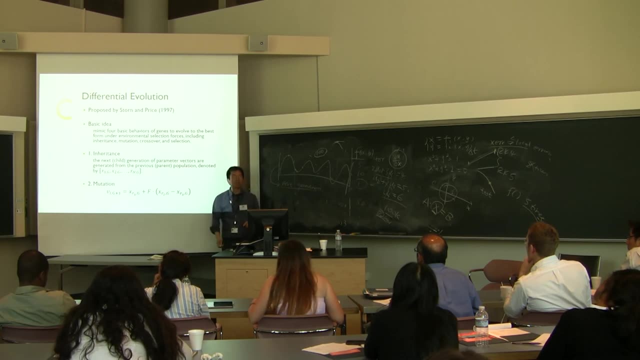 And these search agents actually will update themselves from the parents, not only by mutation- okay, You see, here is the mutation- but also selection and crossover and selection. So mutation here is simple. I just randomly select the three search agents, okay. 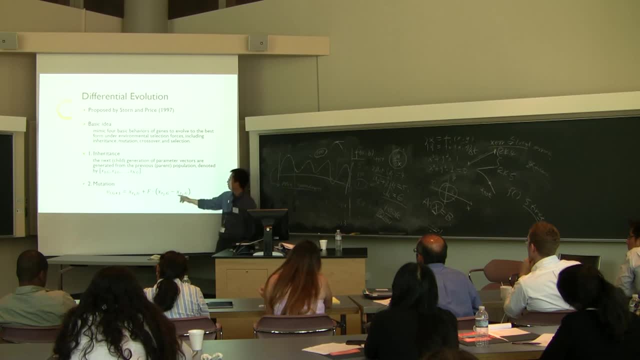 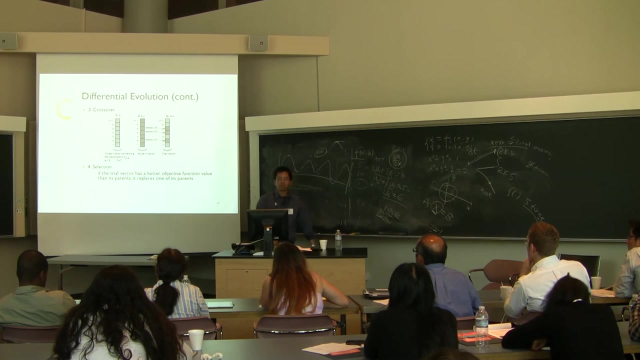 And then I add the genes in the previous generation And I add them together. okay, Basically this is a difference between two. Amplify the difference, add them together, You get a mutation. But a mutation could be good, could be bad. 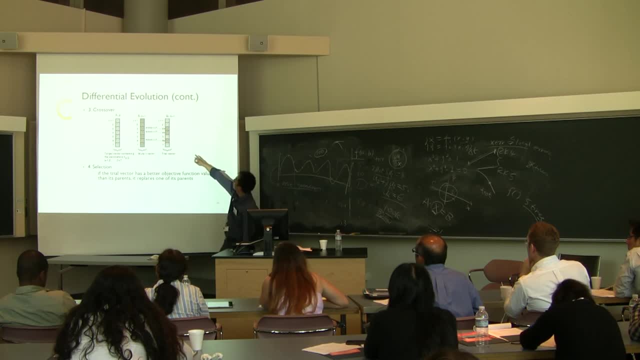 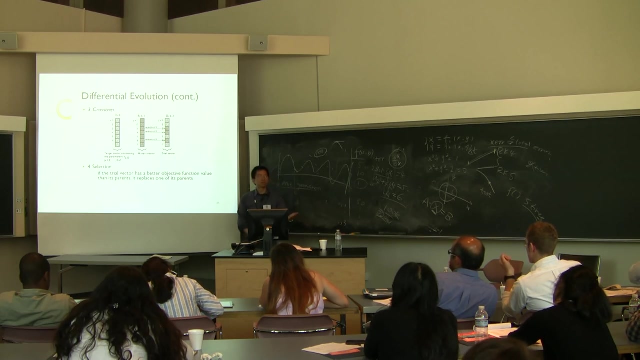 And then you do the crossover. Crossover means you mix the genes of the mutated genes and the parent's gene. okay, Mix them okay. Next step is that if the children are better than the parents, then we replace the parents with the children. 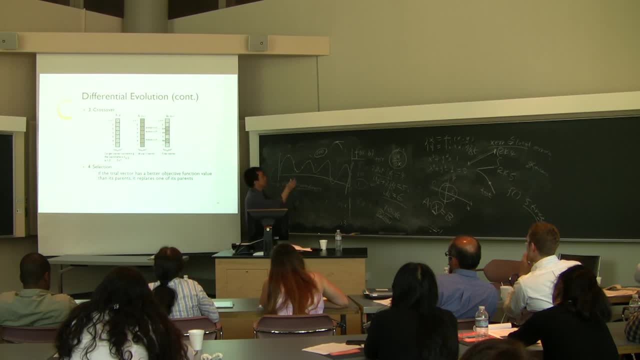 That's selection. So in that way I will generate my search agent eventually will get better or get closer and closer to the solution here here here. So basically what I'm saying is that all the local minima or maxima. 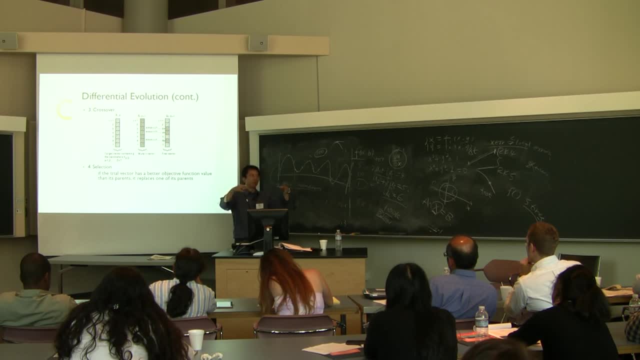 they will be. the search agent will get crowded there, okay, And then you have a best one, okay. So in that way I can search the whole parameter space And then one of them are the best is the best. 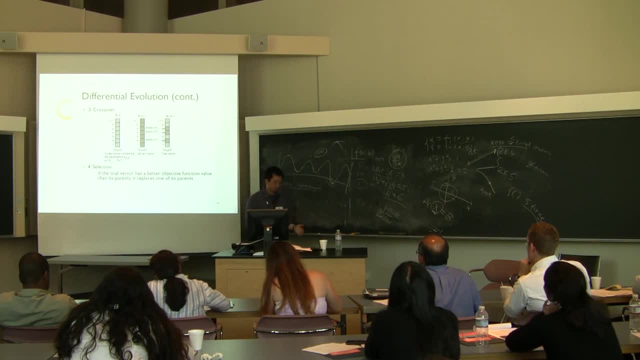 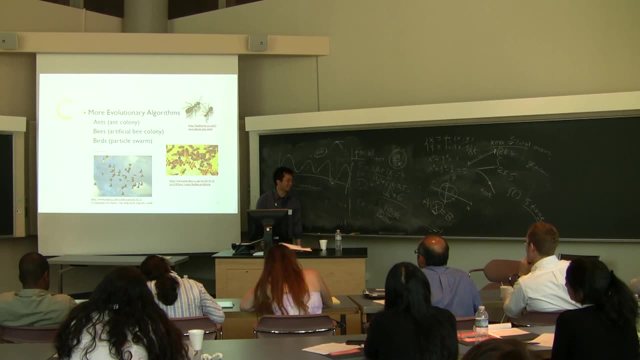 So that's how this kind of genetic algorithm get the you know global solution. So, instead of a genetic algorithm, people also do many other things, okay, Interesting things. You can mimic the behavior of ants. That's why you get the so-called you know. 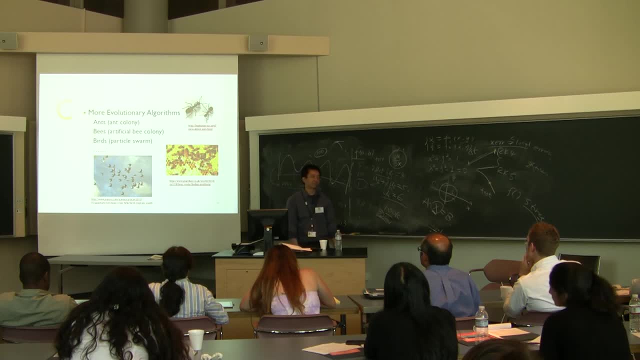 the so-called ant colony algorithm. You can mimic the behavior of bees- That's why you get that facial bee colony algorithm- And you can also mimic the behavior of birds. That's how people actually develop the so-called particle swarm. okay, So we are actually. we are- inspired by nature. okay, a lot. 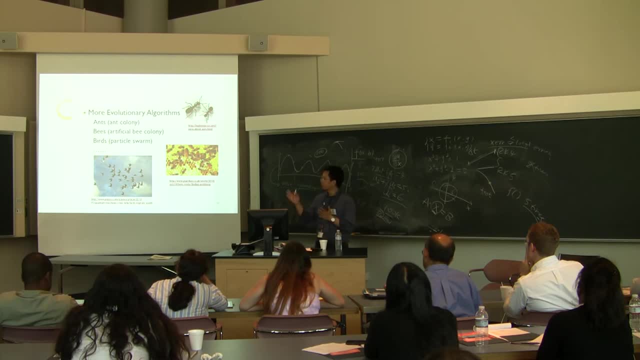 So, but in nature, okay, these algorithms called evolutionary algorithms, okay, the concept, okay, is actually similar to what we just described. okay, You use the parents. okay, generation, generate children and follow some strategy and do a selection. okay, 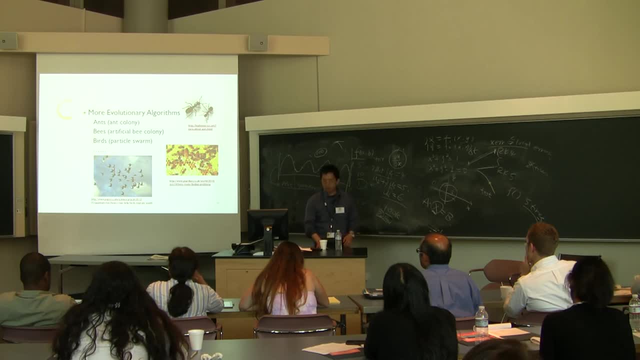 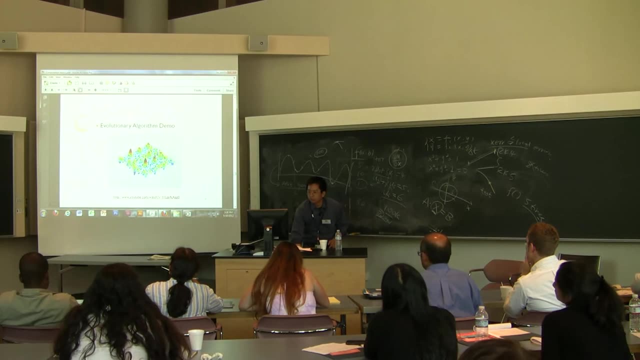 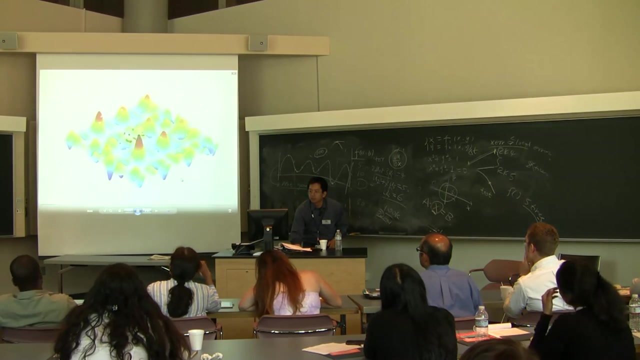 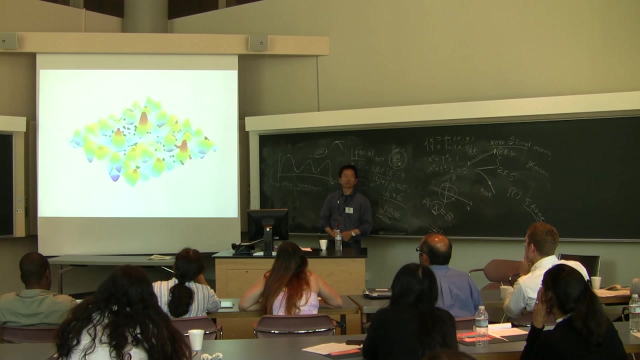 So they are similar thing. They can all be used to find out the global solution. So now I actually want to show you some movie. So how they, how the global algorithm, work? okay, You see, the surface actually is there. 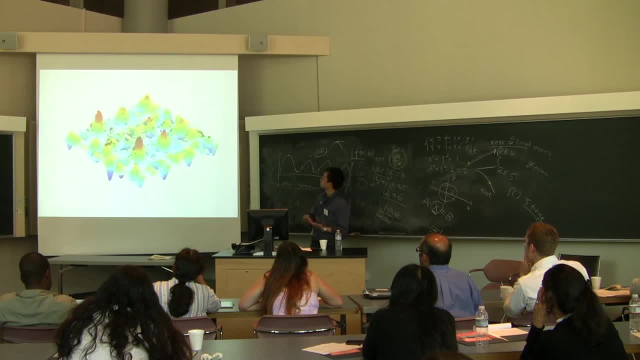 object function surface. okay, It has many, you know, bumps, And what we really want actually is this one, And I have many, you know, search agents And they're, you know, exploring the whole parameter space. 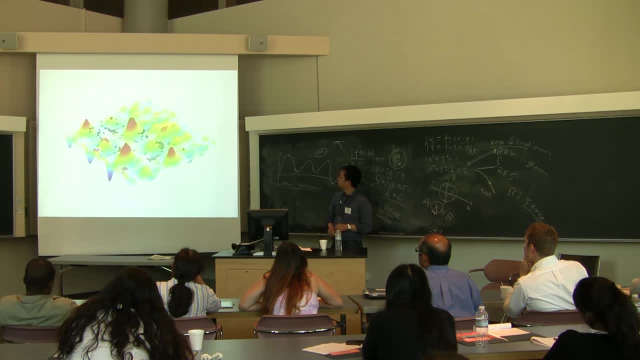 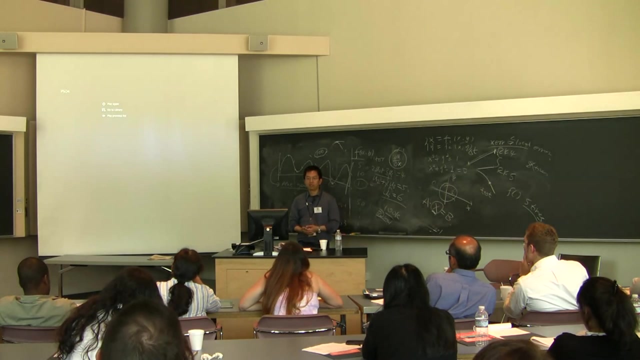 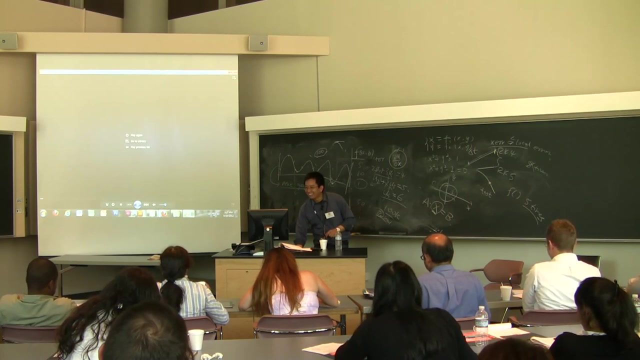 And eventually it goes to that solution. Okay, now it will converge, okay, So that's how it works. So the important thing is the idea, right, It doesn't matter the technique details, okay. So Well, I think I have two minutes. 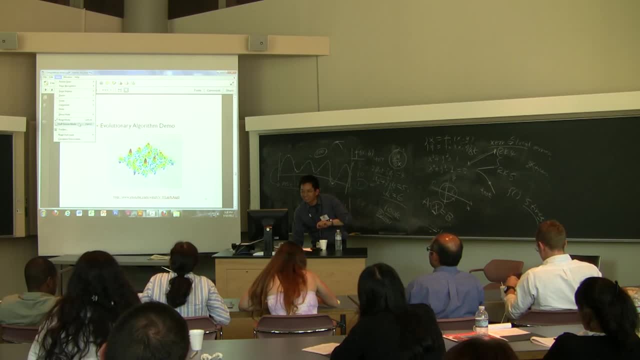 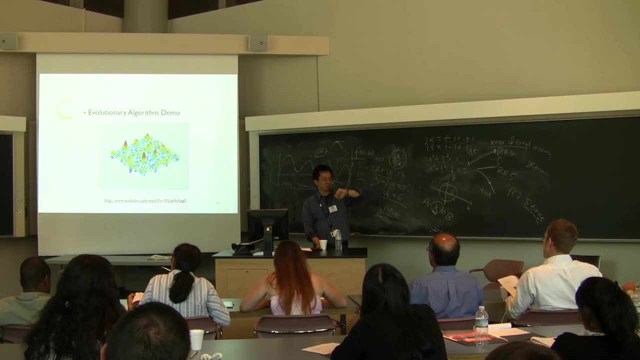 but probably I will not take advantage of it. Fifteen minutes, Huh, Fifteen. Fifteen minutes, Fifteen. You want me to talk two hours and 15 minutes. No, you're braining, You're braining. 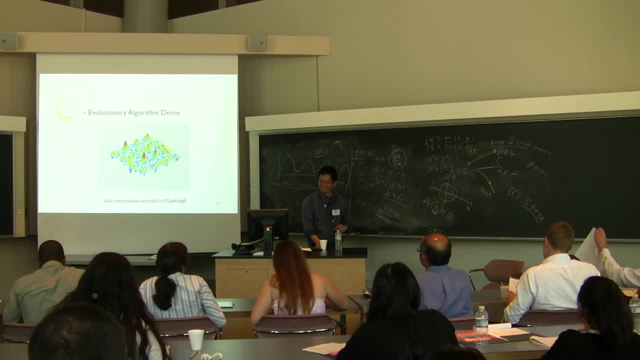 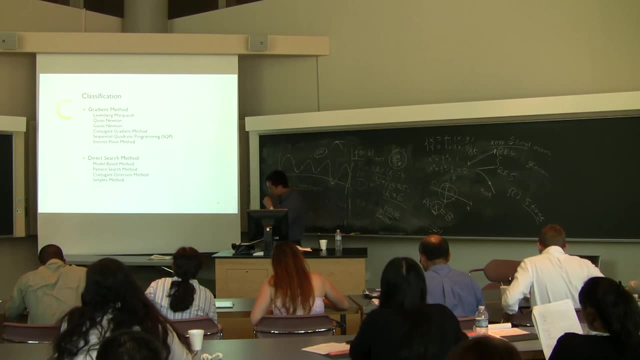 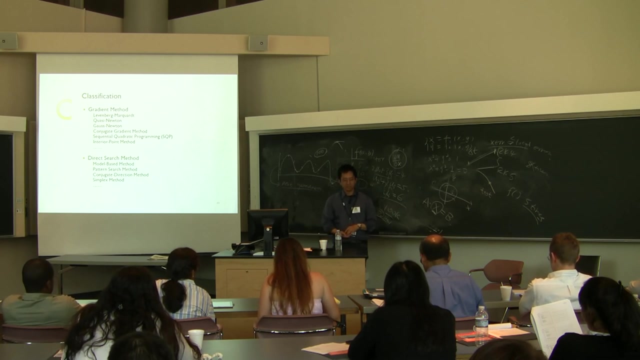 Okay, that's fine, That's not humane, okay, But anyway. So Let's talk about the different types of algorithm. okay, We talk about the gradient method. We talk about the global method. right, Actually, there are more methods, okay. 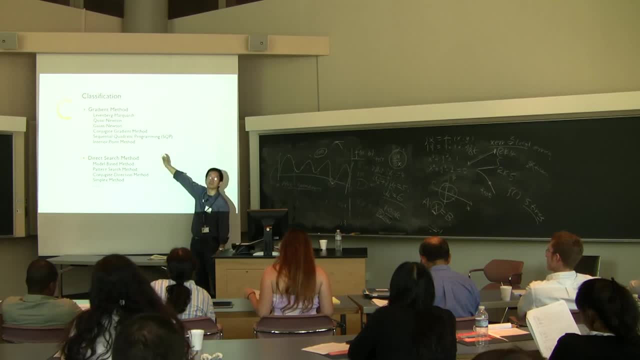 This category is called the direct search. okay, Here I just put a bunch of names. okay, here You don't need to care about the details, But once you met them, you know what they are. okay, That's enough. 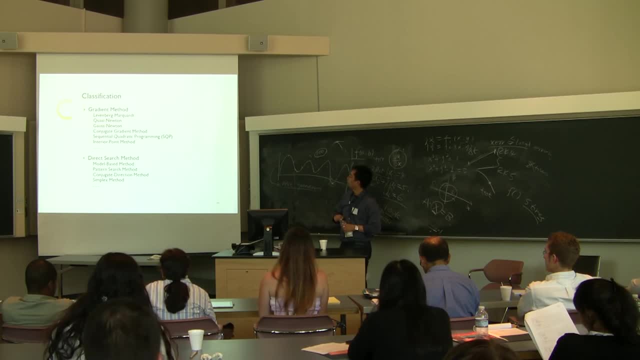 So for the gradient method we just talked about, okay, I will recommend the sequential quadratic programming. That's the algorithm I always use. okay, But I actually do not directly use this one. okay, I combine this method with some other method, okay, 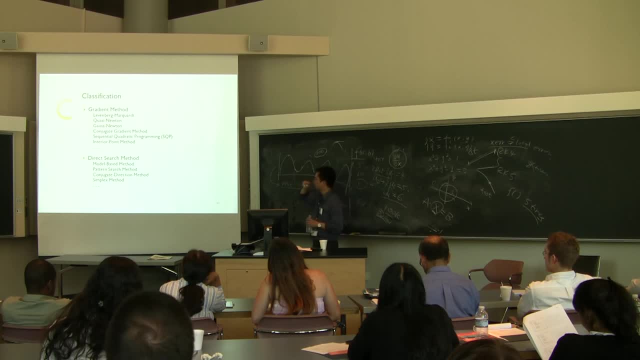 That's how you get the reliable results. I'm gonna explain that in like two minutes. So the second category of optimization algorithm is called the direct search. They're slow, they're a local method, So don't bother to use them, that's all. 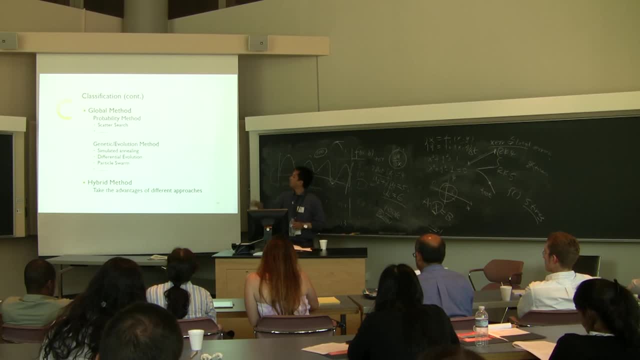 And the third one is called the global method. I just talked about, right, The differential evolution method, a genetic algorithm. So there are many variations, okay, But you just remember the video, okay, That's, oh, okay. 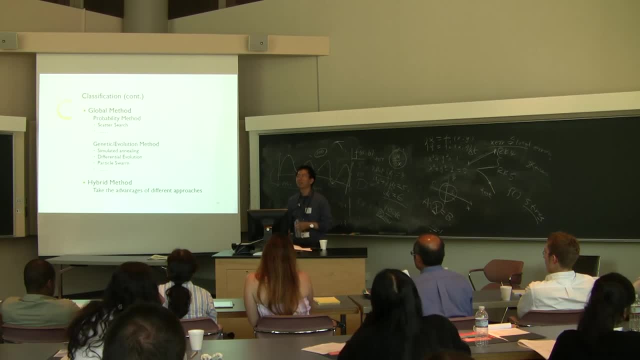 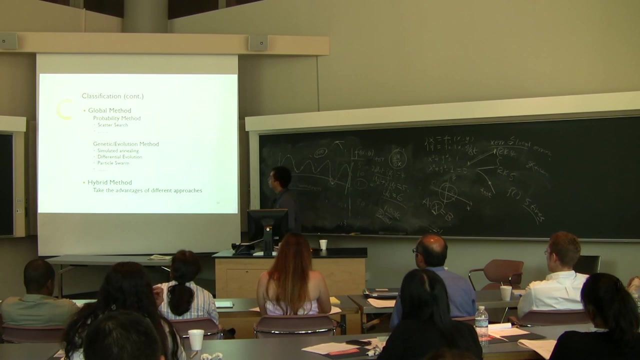 The video tells you how they search the parameter space and get the global solution. Then we are okay. okay, So this final set of algorithm is called hybrid method. That's actually what I used in research. Basically, you know that gradient method is not reliable. 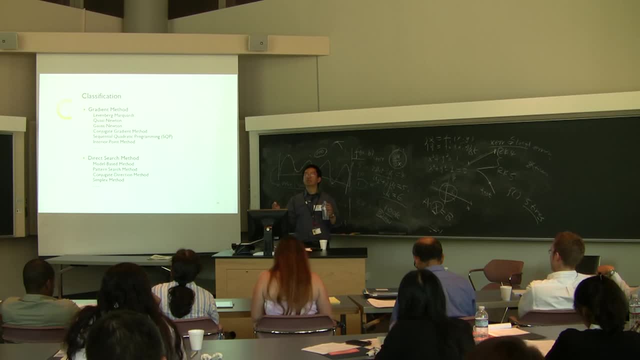 because you need to pick a starting point and which you have no way to know how to pick that, okay, You have to guess, totally by guess in many situations. okay, Also, the gradient method will just converge to a local minima, okay. 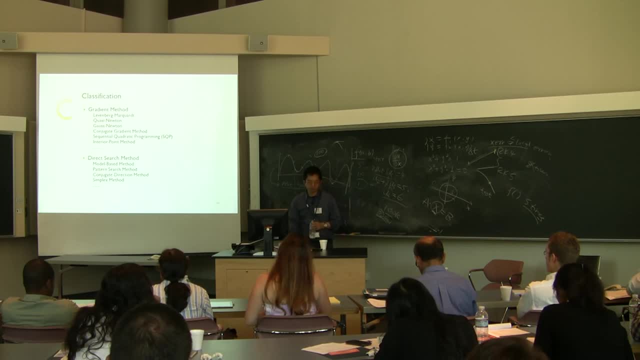 So that's another thing you don't like: You don't have a global solution. Now, if I use global method, I can have a global solution, but one thing I didn't mention is that this kind of method are extremely slow. okay. 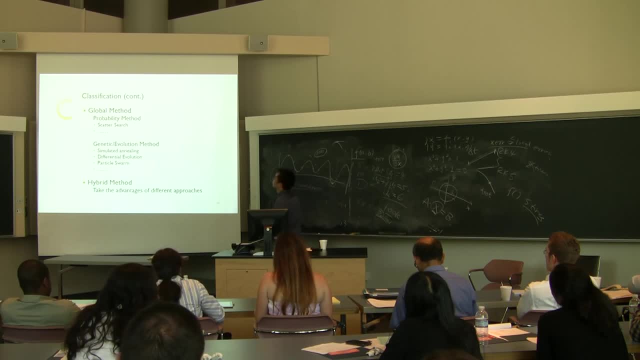 The computing cost is very high, So you don't want to, like, wait one week to get an answer. So that's why people actually develop the hybrid method, or called the memetic method. Okay, Now, the idea is that let's just combine, okay. 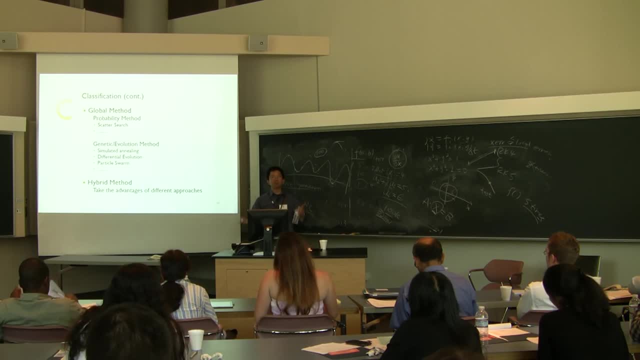 the gradient method and the global method, So you can get a global solution with much improved computing efficiency. okay, But this kind of method is still slow, but much faster than the pure global method. okay, And also, since you introduced the gradient method, 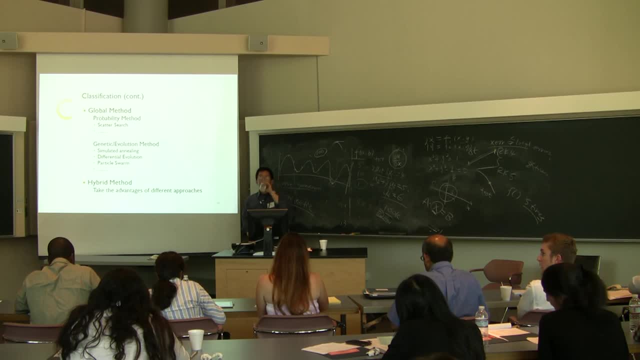 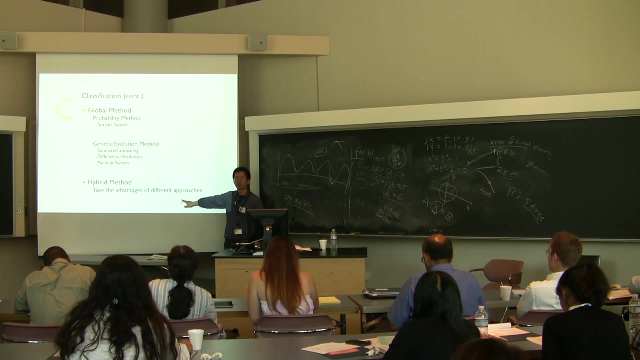 into this kind of approach, then you are guaranteed to converge to the local minima Right, And also, since we have some strategy to ensure the search for global solution, then you get both okay. That's one good thing about this one. 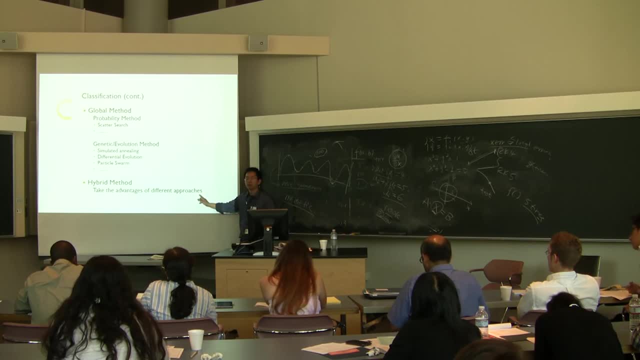 And tomorrow we're gonna talk about D-Discover. We actually have all the three types of, four types of algorithm implement and you can try it. You can try different, you know method to see which one works better. okay. 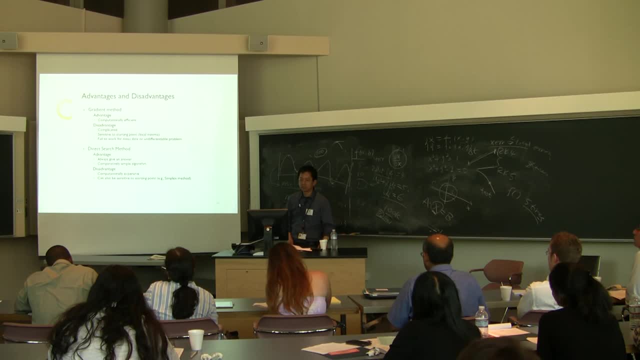 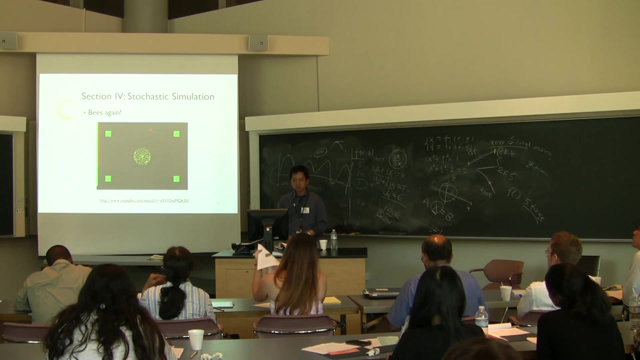 So that's actually the advantage and the disadvantage I just talked about. okay, Basically just the global solution versus the local solution and also the computing efficiency problem. okay, So now I have 10 minutes, So let's see. 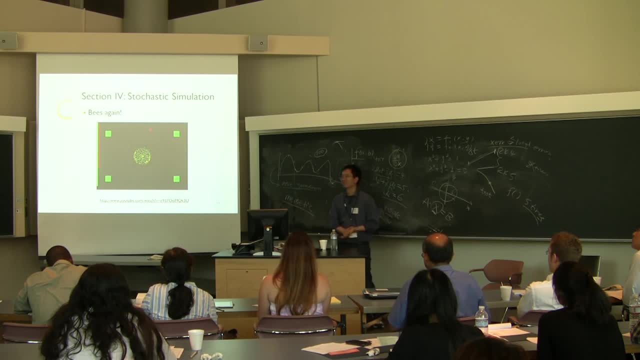 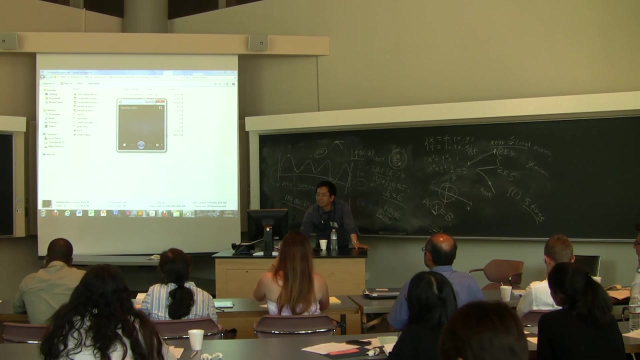 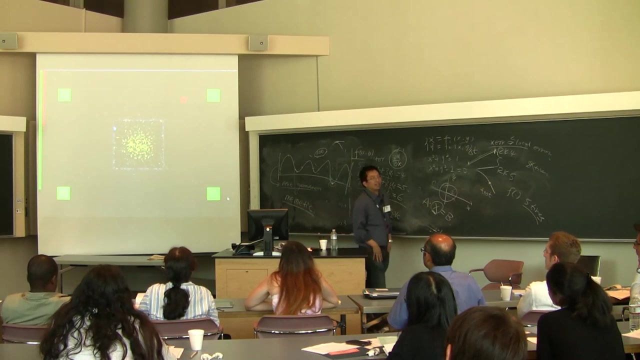 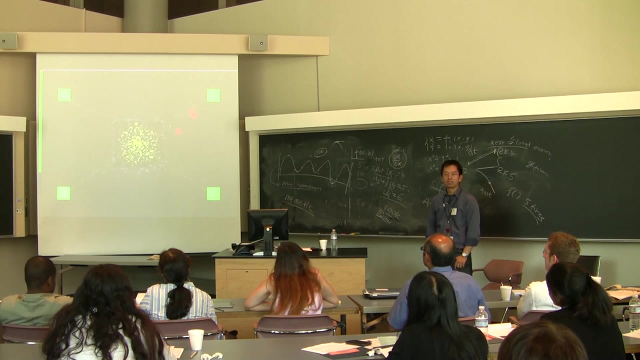 Let's start with the stochastic simulation. okay, Let's look, watch a video again. okay, Ah, this time I got a video. I got music. Okay, While you are watching right now there, which point I will try to show you. 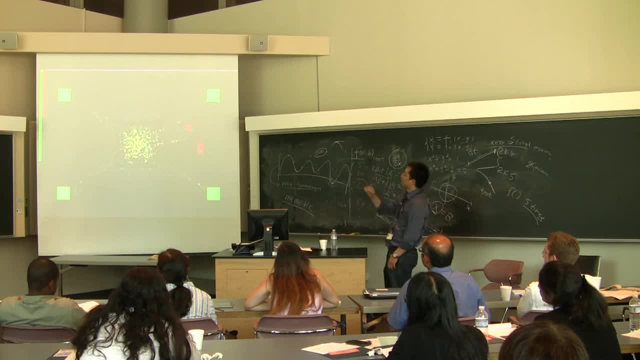 You can see that I'm looking at. I'm looking at the red blocks- They are intruders okay. And the yellow dots- they're bees okay. And this green bar is the total amount of food available to bees. 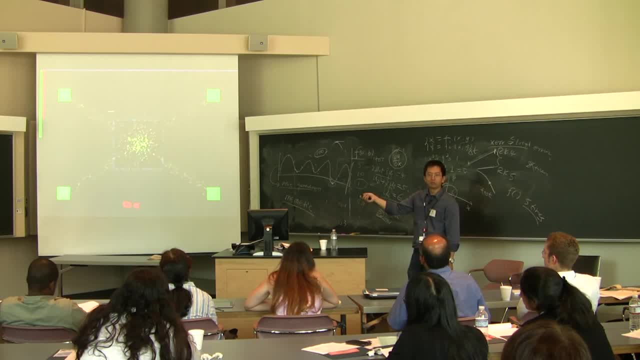 And the red bars are total amount of food available to the intruders. So the intruders are trying to steal foods from the hive, Okay, And once they get closer to the hive, to the hive, they get some, you know, guards, okay, fighting against them, okay, you see. 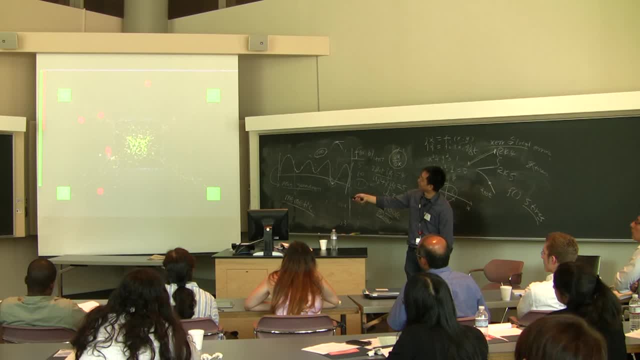 the purple. there's some purple. you know dots here. that's actually the guard. so the number of bees actually depends on the total amount of food. okay, similarly, the total amount of intruders depends on the food, but also their- you know, migrations or something. 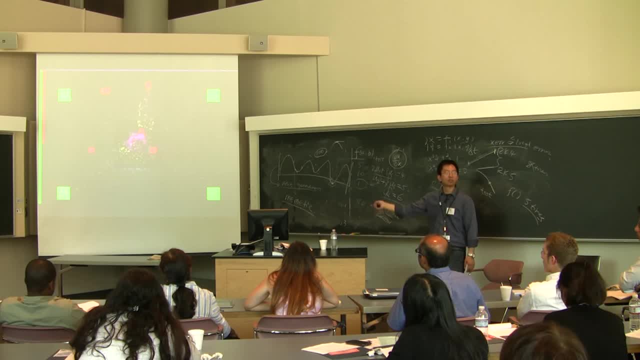 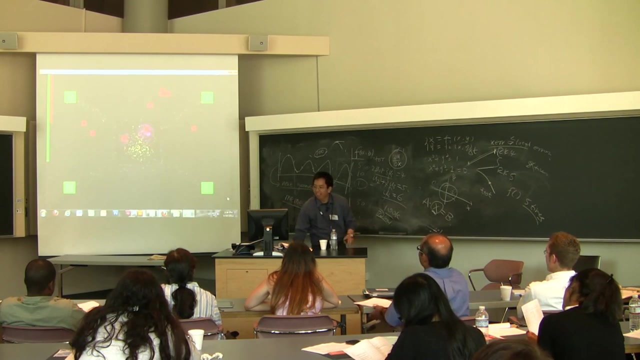 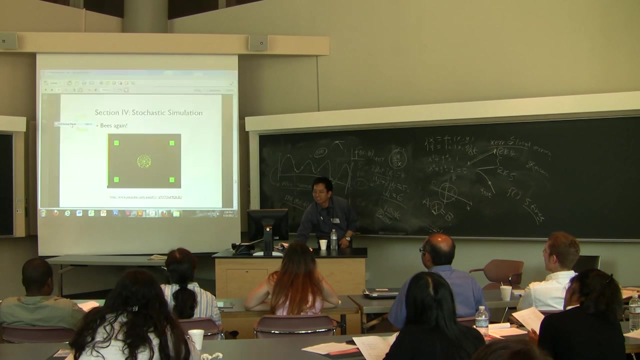 so sometimes they will just move away from the frame means they find another place to start over. okay, and these green squares, they're actually flowers, okay, where the bees can get, you know, flower powder, okay, Okay, so I guess that's a highlight of my talk, okay, but anyway, to generate that video, 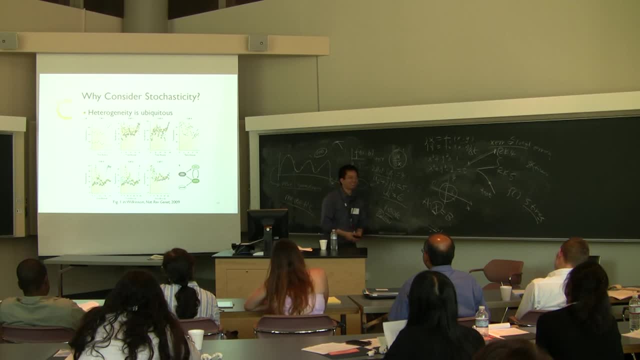 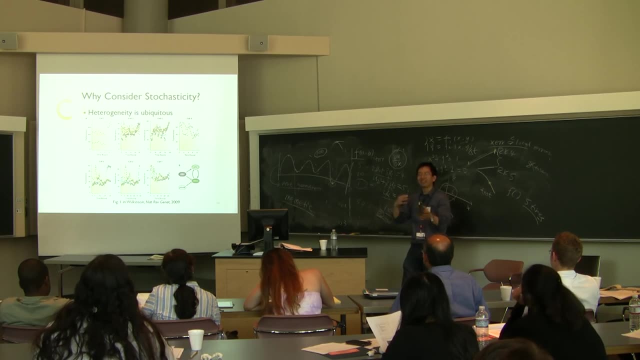 is actually extremely simple. okay, I have to tell you, okay, visualization is complicated, but generating that data, okay, Visualization actually is very simple. you just draw random numbers. okay, keep drawing random numbers. okay, that's actually the basic idea of stochastic simulation, okay, 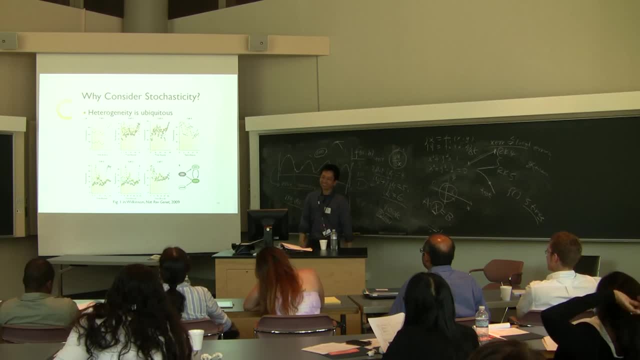 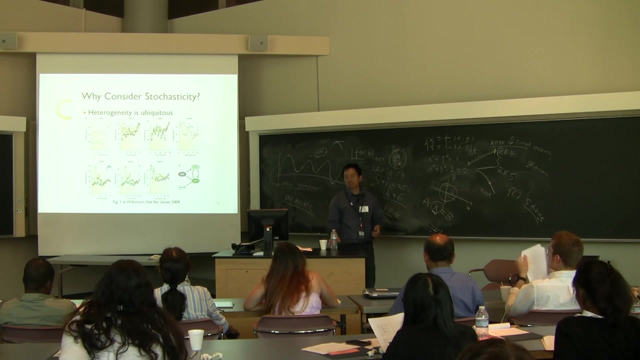 stochastic simulation is just drawing random numbers. okay, that's all so, but I since I still have a few minutes, so I will not stop here, so I have to talk about some details of how to draw random numbers. okay so, but before that, let's look at this plot. so that's. 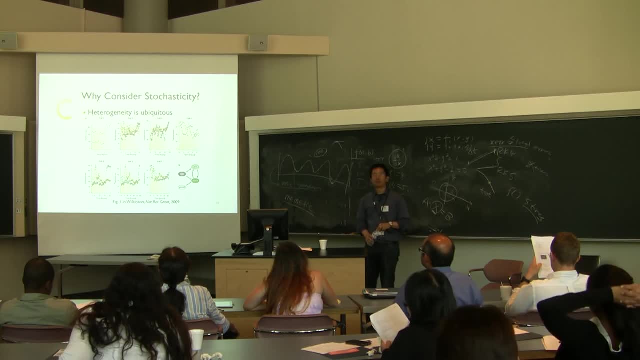 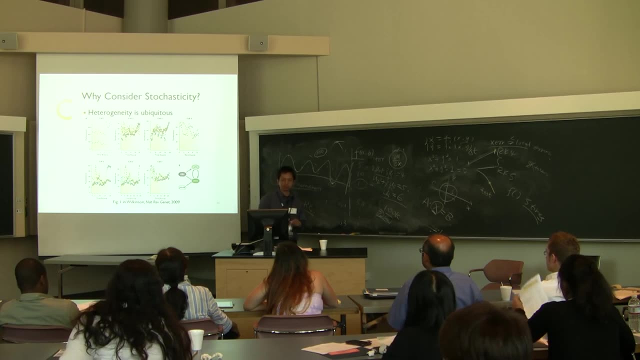 actually the case that randomness will become very important. This actually comes from a nature review paper that looks at single-cell data. so that's the same type of cell, seven cells of the same type, and they're undergoing the same biological process. however, if you measure the protein, okay, one type of one certain. 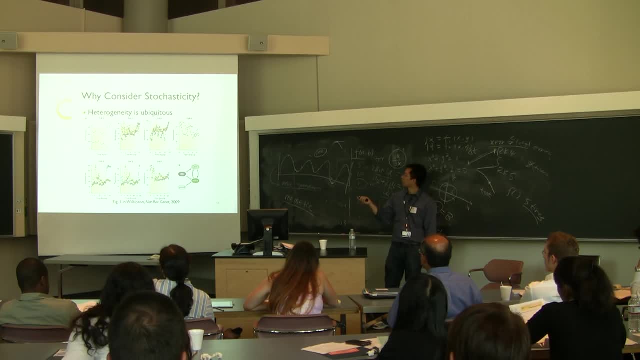 protein concentration within each cell, the data pattern looks totally different. Okay, So since there are there are same type of cells that are undergoing the same biological process, we expect that we can use the same model to describe the data, right. however, 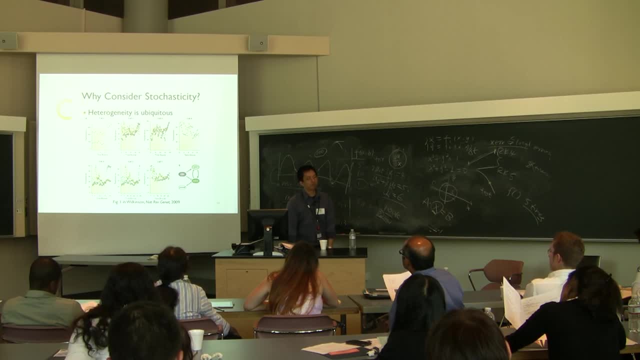 the data pattern looks totally different. so are we going to create a model for each cell or what, or we just introduce some randomness to the same model? in that way I can account for the variation. so which one you prefer, I will prefer. 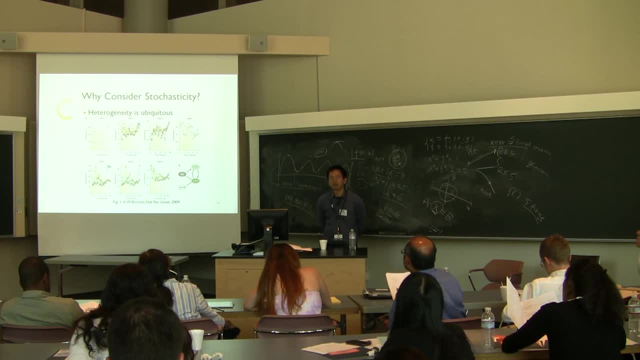 I will prefer the latter because they're the same problem. okay, the mechanism is the same. the variation is just due to the between-subject variation. so I can use the same mechanics mechanistic model to model them, but I can add some randomness right in that way. I. 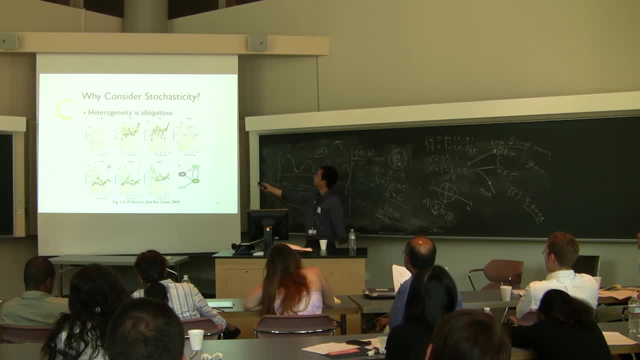 can account for the uncertainty. so that's the idea of stochastic modeling. okay, I do do stochastic modeling. Okay, I'm not only, I'm not an ODE guy, okay, 100% ODE guy, okay. so now I want to actually. 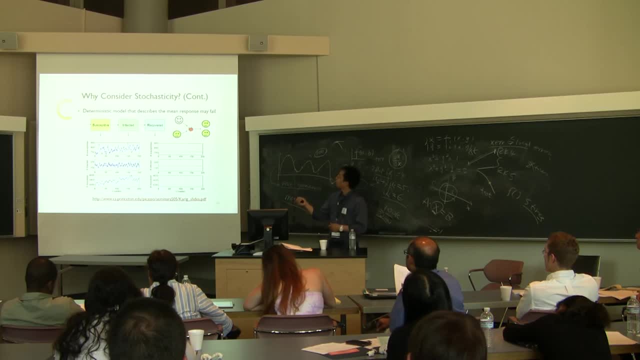 give you another example. okay, so this is just a very typical SIR model. okay, people use this to model the epidemics. okay, so susceptible, infected, recovered or removed. okay, people also call this removed sometimes. 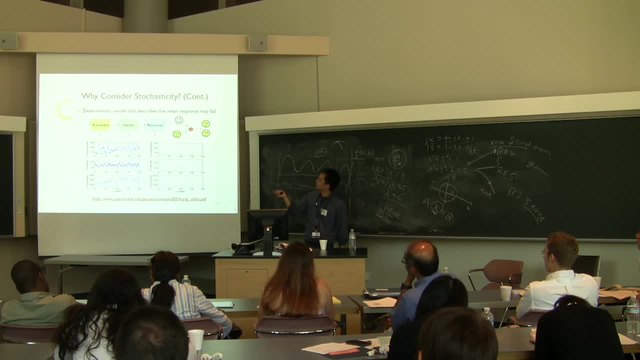 So if I do a stochastic model, I see this very interesting oscillations, okay, and that actually means something which means there's a cycle, okay, from the burst of the disease to the eradication- eradication, right. so if I use the ODE model, okay, you just get. 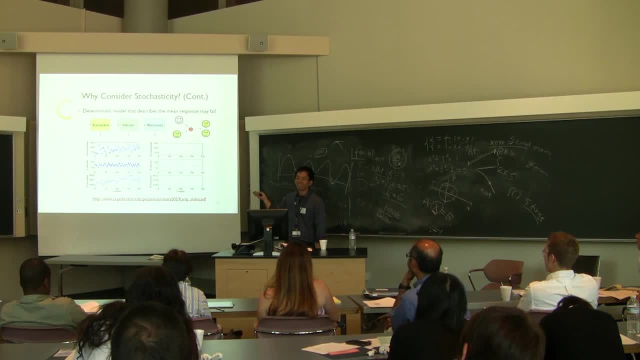 a flight tail tails do nothing. The only interesting part will be just this beginning part. okay, so that's one example. if you don't use the, you know, static model, you get totally wrong. okay impression about the problem. 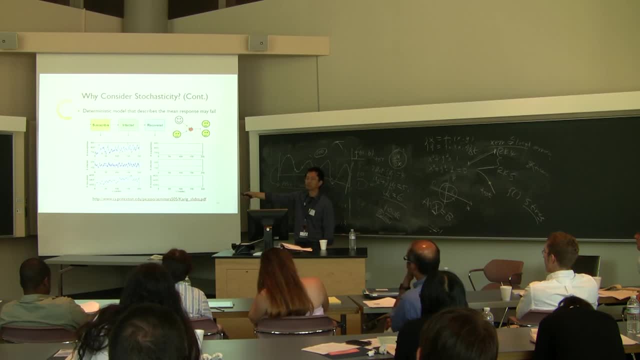 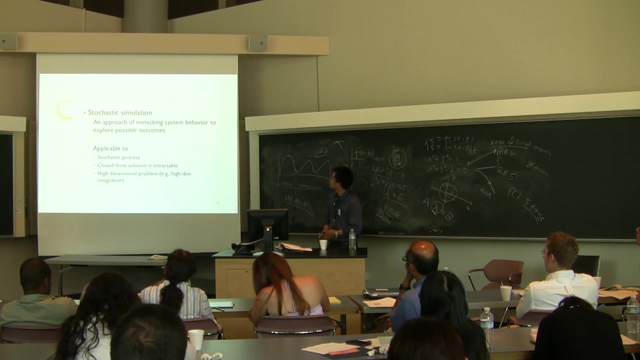 Here I have randomness, I have noise, but I also see this prominent, you know oscillation. okay, that oscillation, I think, is important for this problem. so that's why people actually use the stochastic simulation. okay. 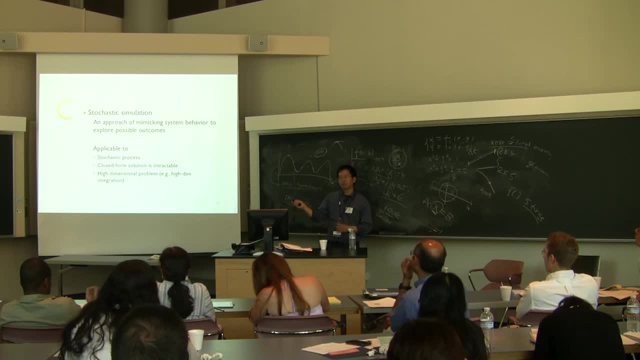 Okay, To mimic the system behavior and the ultimate goal is to actually explore the possible outcomes. okay, You can run the simulation multiple times and get a sample of all the you know- possible outcomes. then you will understand the distribution of this outcome and that will tell you some. 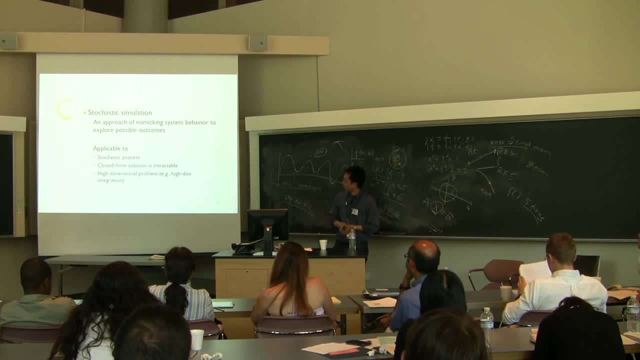 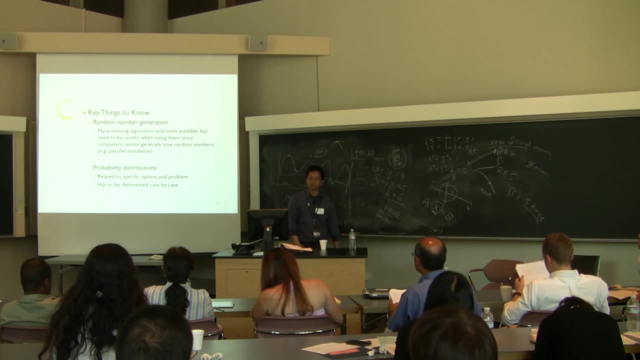 useful information. okay, So the key thing is, in this kind of stochastic model you can use the stochastic simulation. okay, the stochastic simulation is that random number generation and probability distribution, Random number generation: you remember, computer cannot actually generate true random numbers. 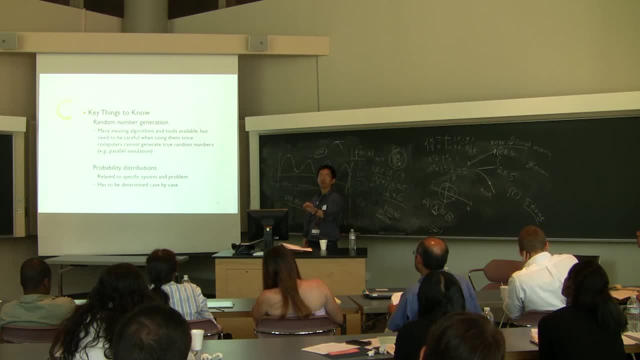 okay, computer just do what you tell it to do. okay, so computer in nature is deterministic, so they cannot generate a true random number, but they can generate pseudo random number. okay, So these pseudo random numbers actually can work well. 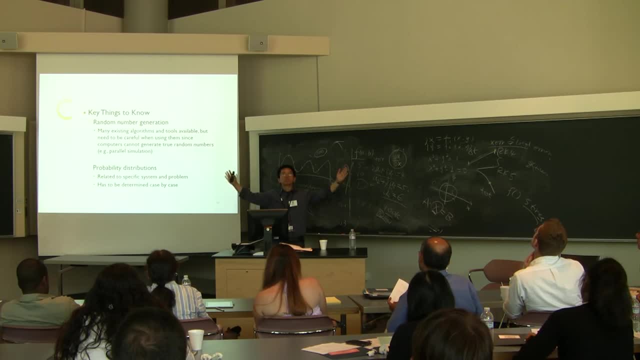 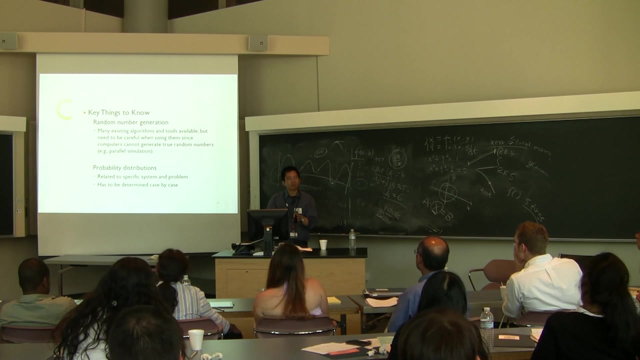 Okay, They can work well if the algorithm is well designed. so the period is long. When I talk about period, which means if you use a random number generator, for example, if you draw one million random numbers from this generator, it may start to repeat itself. 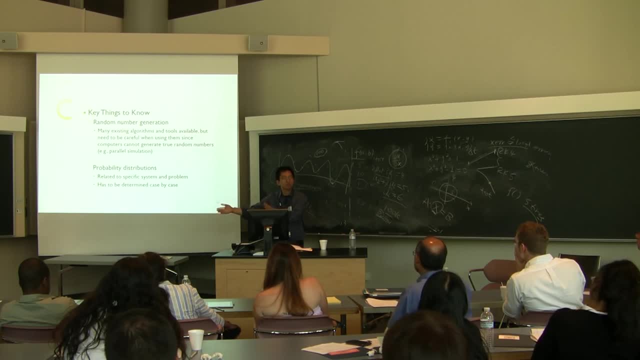 okay, after each one million random numbers. So now this pattern will become predictable. then it's not random anymore. Now people have designed generators that actually have extremely long periods. So for your research purpose I think probably you don't need to worry about it, okay, because 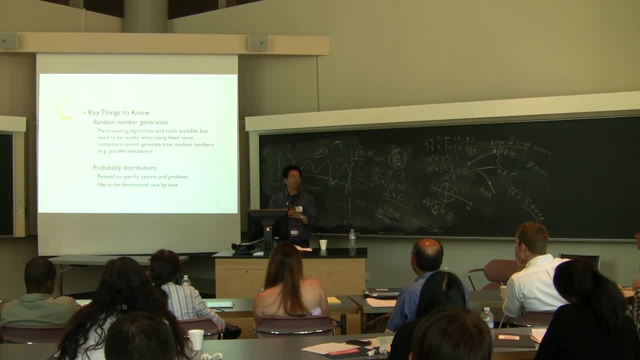 the period is too long. Okay, it's not one million, actually it's, I forgot. it's actually a huge number, like 10 to the power of 23, or even more than that. I think it's more than that. 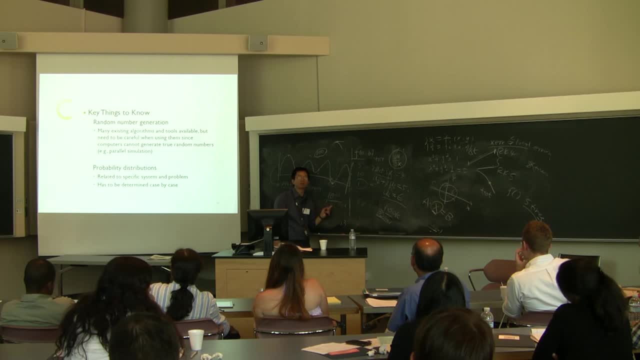 So usually in your simulation you will not draw that many- okay, random numbers, okay, at one time. Okay, The second thing is that you need to specify the distribution of the random variables. okay, That is problem. problem specific: 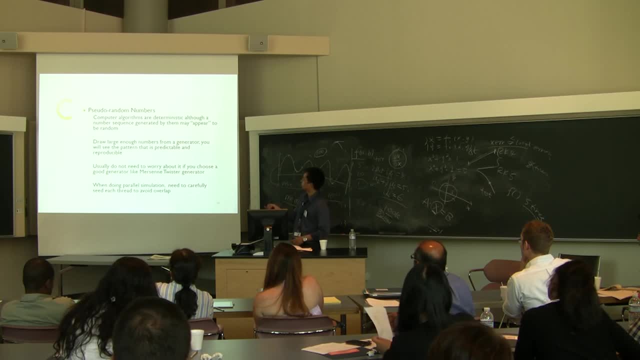 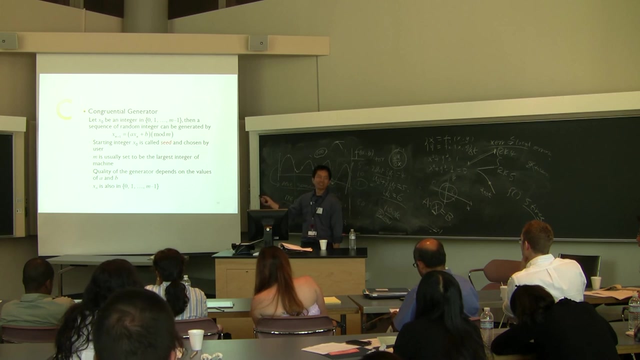 So to generate the pseudo-random numbers, I will recommend this Mercenie twister generator. okay, It has a very long period. okay, and do not use the congruential generator, okay, although that's a very classical generator. Okay. 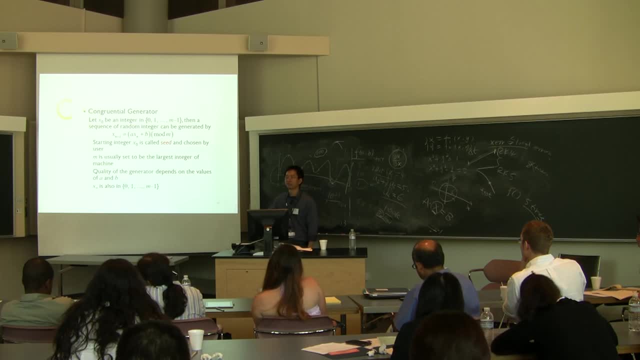 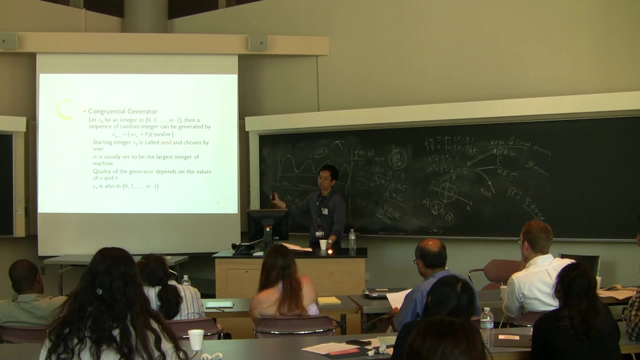 For the first generator. you will learn in a computer science course, okay, but the performance is pretty bad, okay, and its period actually is short. okay, it's just actually m, okay, if you specify m beforehand. okay, that becomes m. 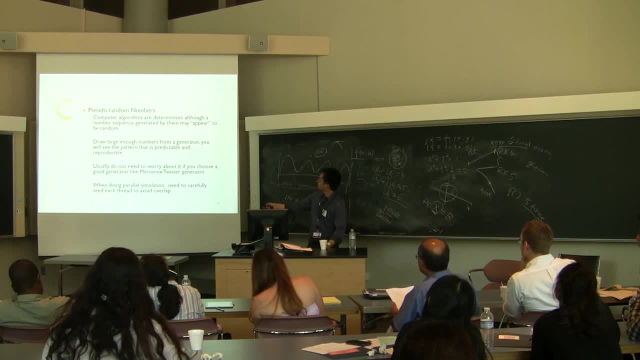 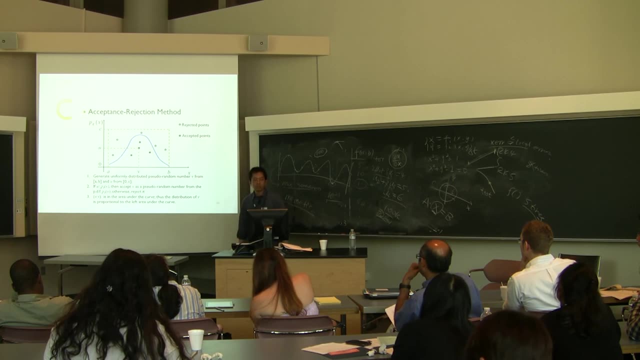 So the Mercenie twister actually generator, I always actually use it okay in my own implementation. So far I haven't tried other generators, although I read some papers that claim there are generators that are better than that one. 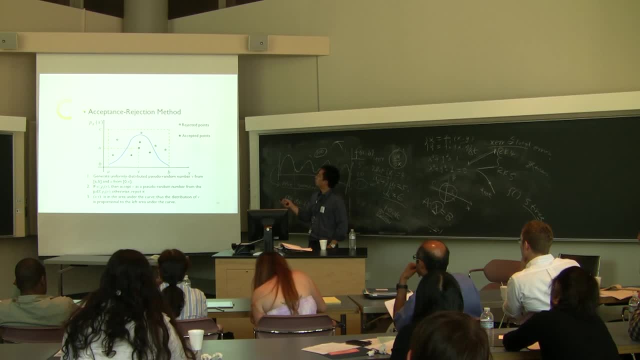 Anyway, when you generate random numbers, you probably will use something called acceptance and rejection method. okay, So the acceptance and rejection method, the implementation of this method is simple. okay, So let's see. Okay, So I want my random variable. my random variable is x, okay, 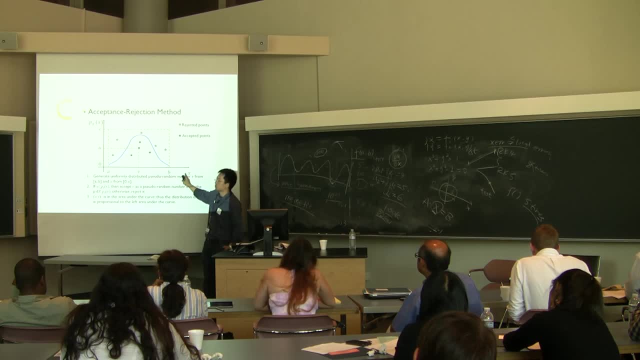 I want to generate random numbers from the distribution of x. So this is a distribution, okay, a blue curve. So what we do is actually generate a uniform random number, v- okay, within a and b. And then I generate another uniformly distributed variable, u- okay, from zero to c. 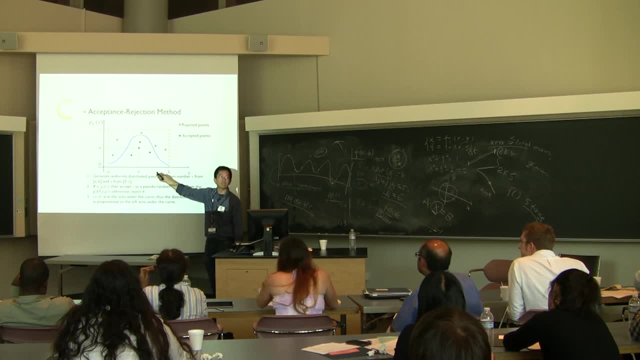 C is actually greater than any constant. okay, Any constant you can specify That is greater than the maximum value of this curve. okay, above this curve. And you see, once it's above the top of the curve, it can be used. 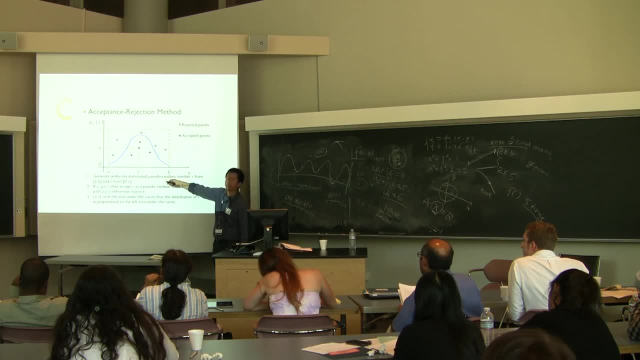 Then if this point- the pair of u and v- actually is a two-dimensional point, if this point falls under the curve, you accept it. If the u and v falls outside of or above this curve, you reject it. In this way, you will generate a two-dimensional point. 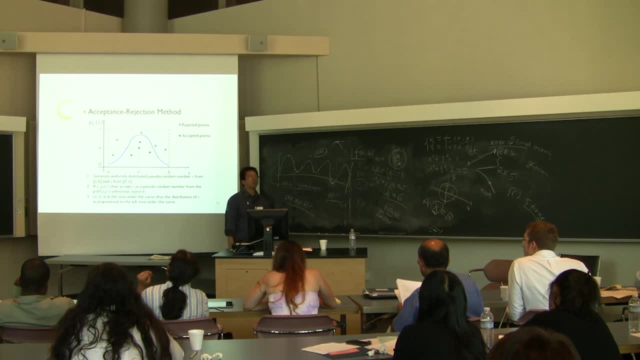 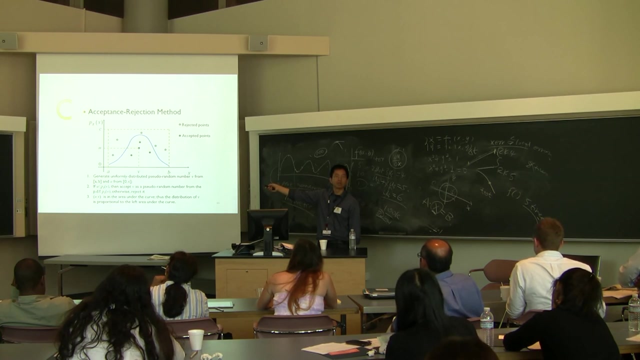 Okay, Okay, How can you run a number? Follow the follow this distribution. Okay, So I? I don't think I have time to talk about why is that? okay, But simply speaking, this is the idea of acceptance and rejection method, okay. 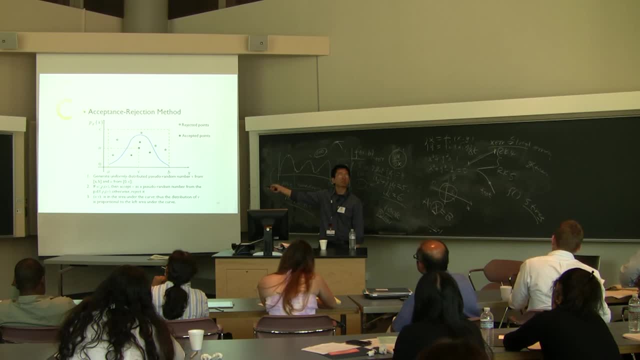 And it works for arbitrary distribution. Now, this is a good thing about this method. okay, because there are many other generators that you need to know the mathematical details. For this one, you don't need to. Okay, You just need to know the distribution function. 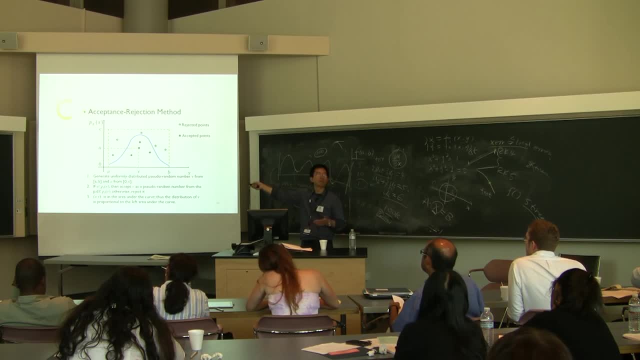 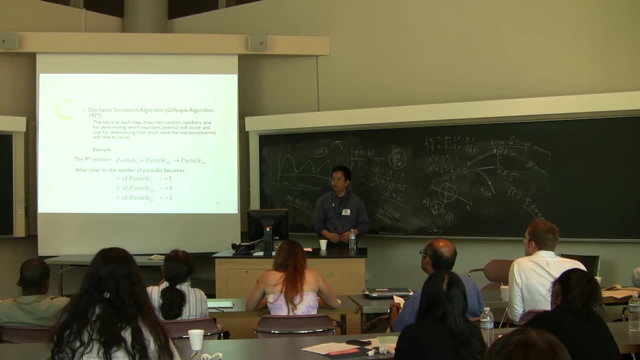 That's all. Then you can just use this measure to generate random samples. Okay, It's gonna work. So another thing I have to mention is that I have to mention is that the so-called SSA- okay, Stochastic Simulation Algorithm. 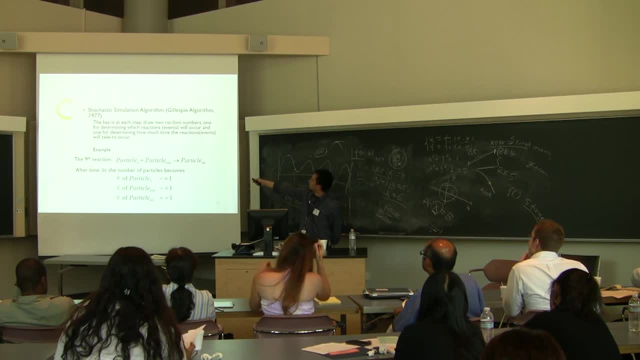 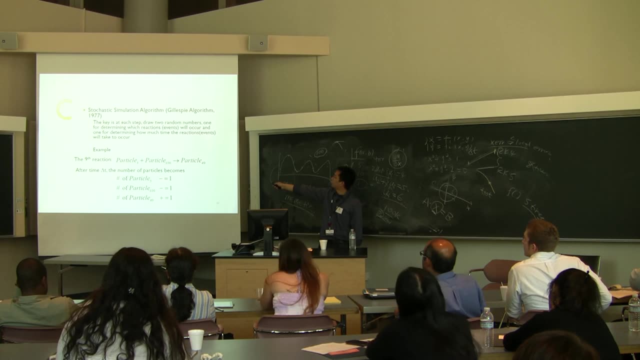 And the concept is extremely simple: At each step, you draw two random numbers. So, based on the first step, you draw two random numbers. Okay, So you draw two random numbers. You can determine which reaction will occur. It's like a lottery. 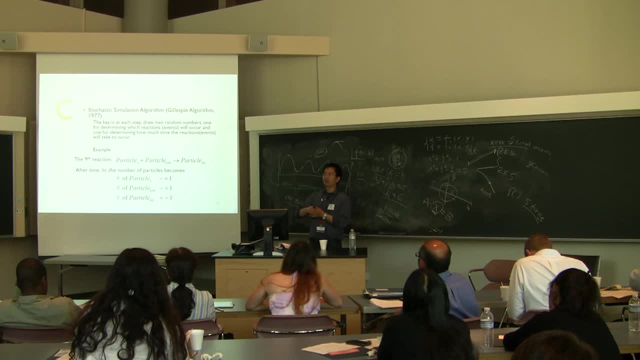 Okay, So there is one reaction: win lottery, then it will occur. The second random number. you actually draw another random number to determine how much time the reaction will take. Okay, Then that's done. Okay, You just repeat these two steps. 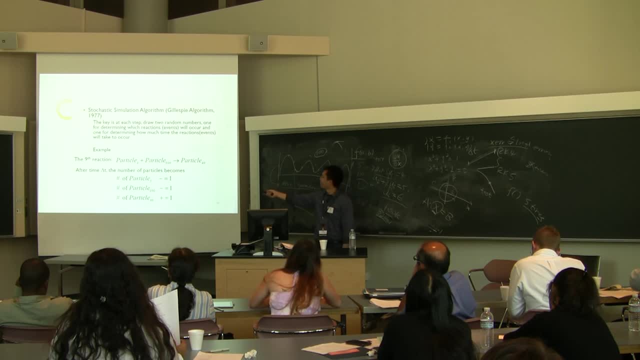 And that's called SSA. Okay, Extremely simple, right? So, for example, at this step, okay, you just repeat these two steps And that's called SSA. Okay, Extremely simple, right? So it happens that the ninth reaction will occur. 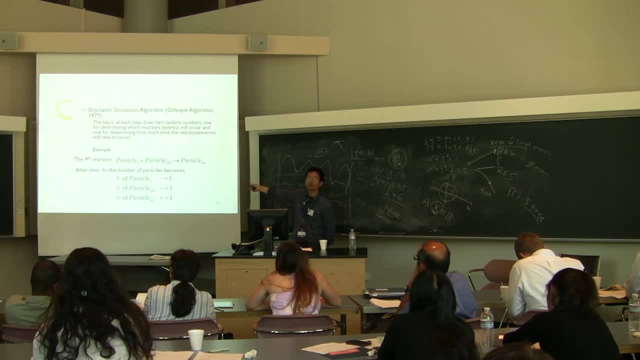 So the particle 3 and particle 100 will form particle 49.. Okay, You get a complex, So you draw another random number So to determine what the time, what's the time it needed to finish this reaction. Then, after that, the number of particle 3 decreased by one. 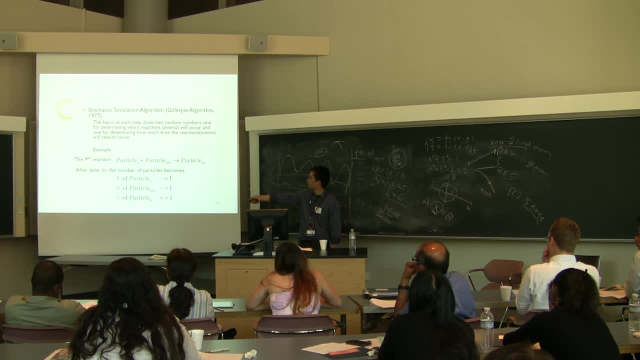 The number of particle 100 decreased by one, But the number of particle 49 increased by one. Okay, So in that way you simulate the changes in particle numbers, And here is an example. Okay, So here what I draw actually is the total number. 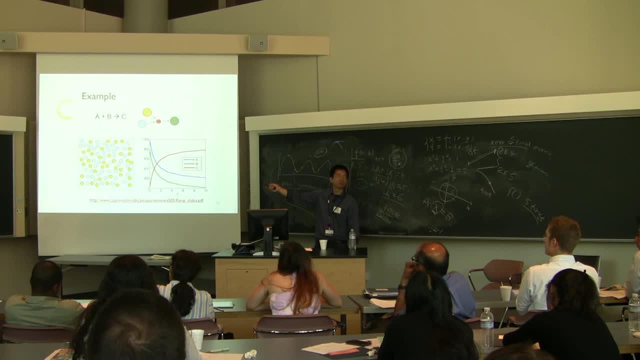 Okay, I have, I start with many A and B particles. Okay, Then I get a C particle Complex, So the. I think the number here, the color here is wrong, Okay, Color here is wrong. The red actually is a C, Okay. 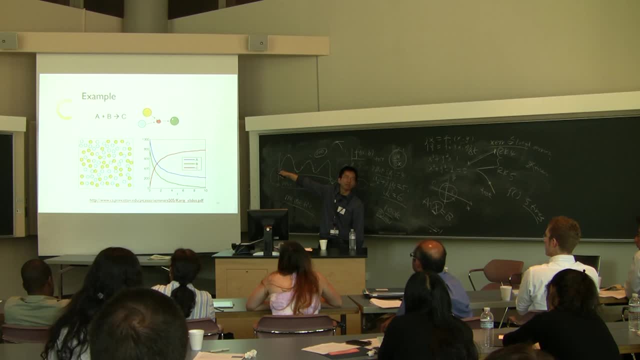 The C actually will increase. So it's different from the color here, Okay, But here here is consistent, Okay, But these two are not. But anyway. So C will increase, A and B will decrease, Okay. 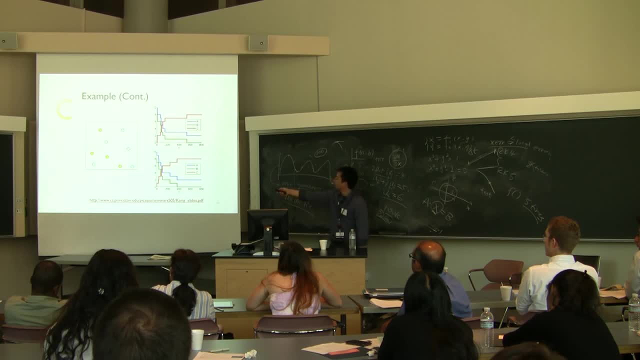 If you use a random simulation And if I reduce the number of particles in a system. now you see what I mentioned this morning. Okay, So this one, this curve looks pretty smooth. I can use ODE. Right, I can also use ODE to model this one. 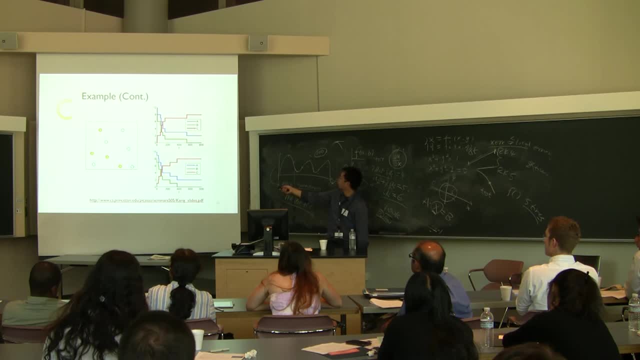 But if I reduce the number Down to like five or you know, six, now you see the curve just become stepwise And now it will be a big, big problem. if you still use ODE, Okay, The approximation will be bad. 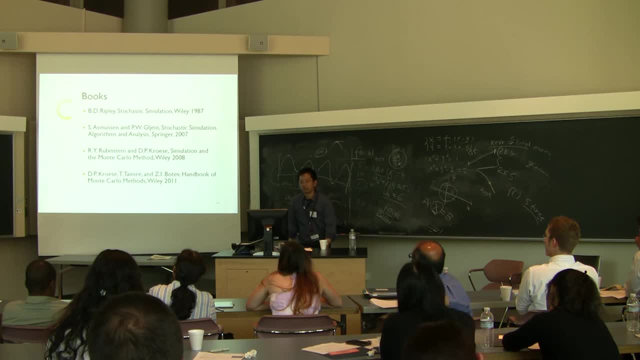 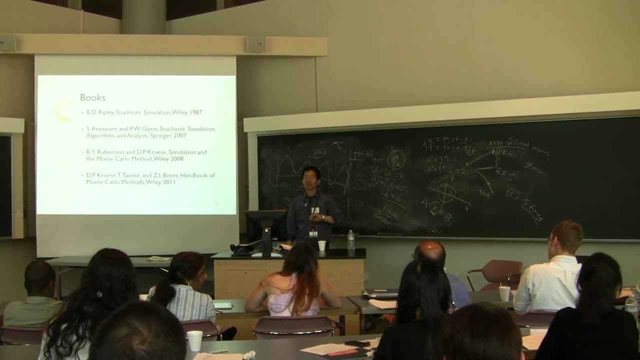 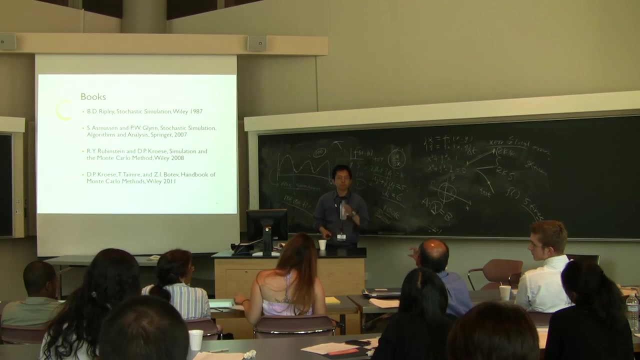 So I I think that's all I want to talk about today, And thank you. Do we have time for questions or Any questions? Okay, I have a question. Uh-huh, When you're talking about the example with the number of different cells, is it possible? 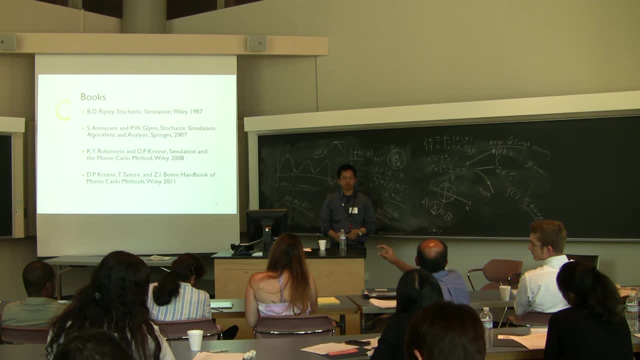 to figure out. you know, I know it's random. There are some places where it could be Like, for example, some of those cells could be going through cell division. Yeah, So, So you want to find those cells? 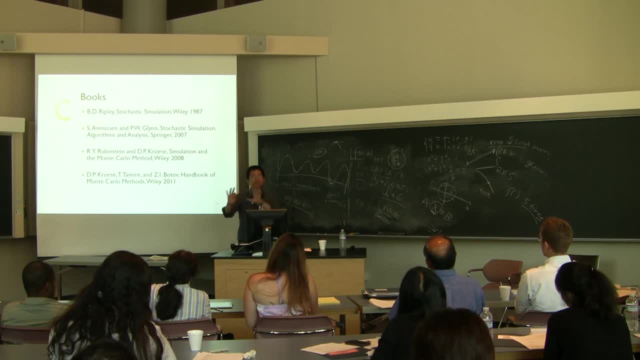 That's what I'm saying. I can use the same model to model all the cells, Right? So, for example, I have the same model for all cells, However my parameter they are different for each cell. Okay, Right.